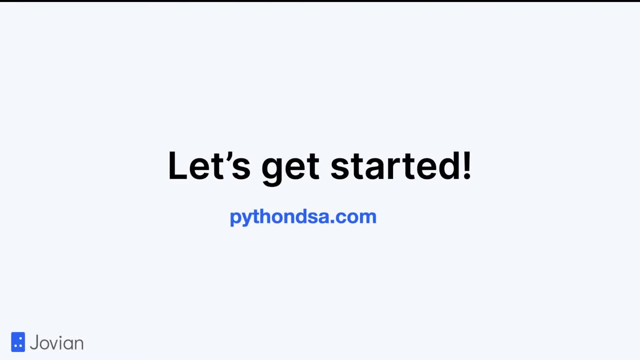 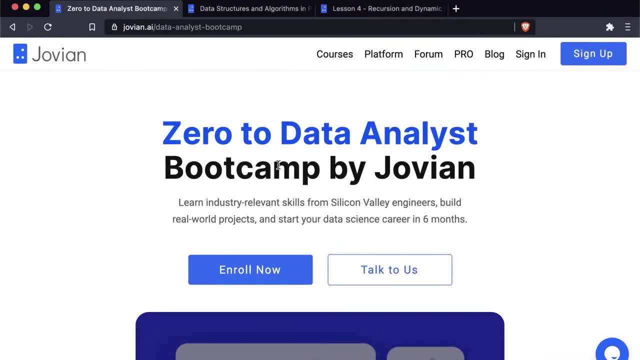 So let's get started Now. before we start, I have an announcement to make. We're launching a new bootcamp called the zero to data analyst bootcamp by Jovian. This is a 20 week program where you can learn industry. 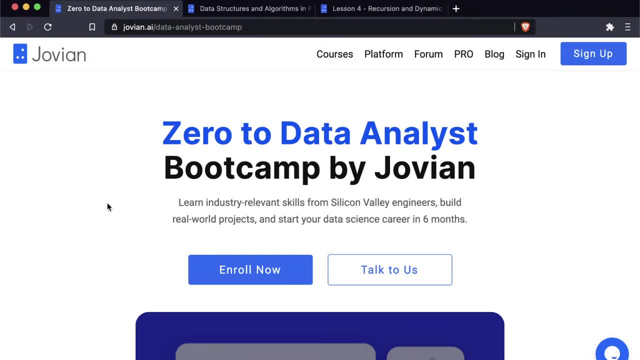 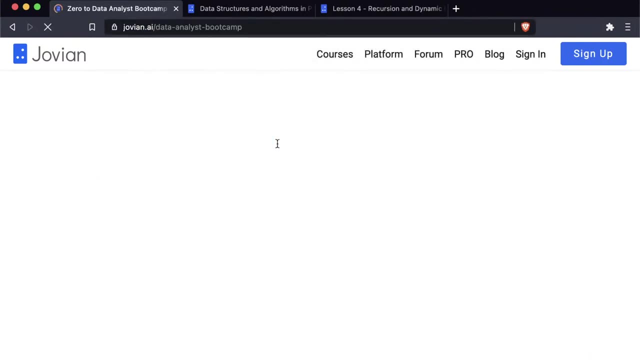 relevant Skills from us, build real world projects and start your data science career in six months. Now you can find this on the site zero to analystcom, That is Z E R O T O- analystcom, And we will also post the link in description. 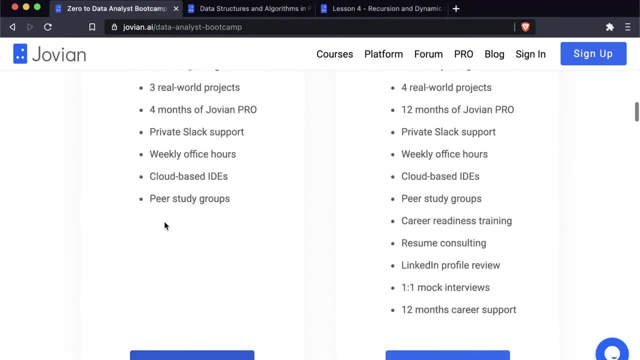 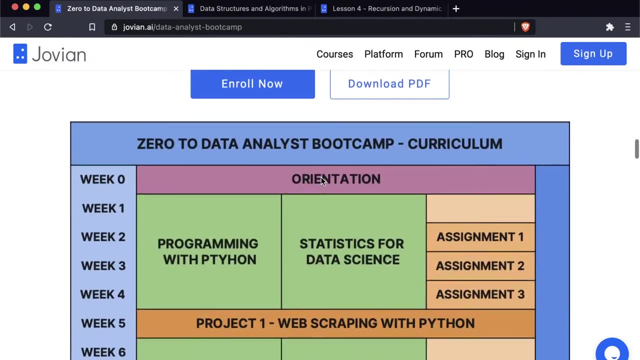 You can learn more by watching this video here or by checking out the benefits. These are the two options you have. You can take a 16 week Or a 20 week online program, And this is what the curriculum looks like over 16 weeks. 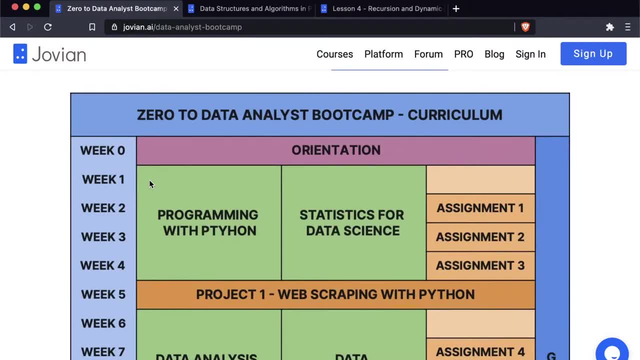 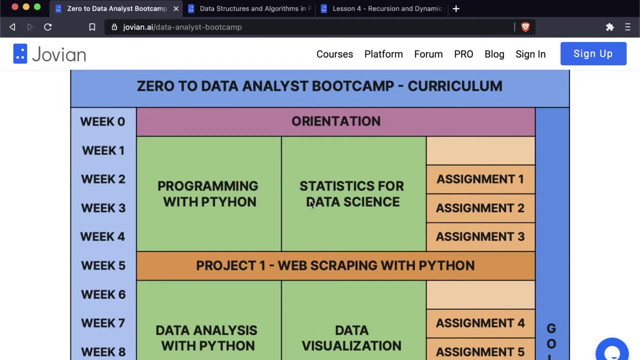 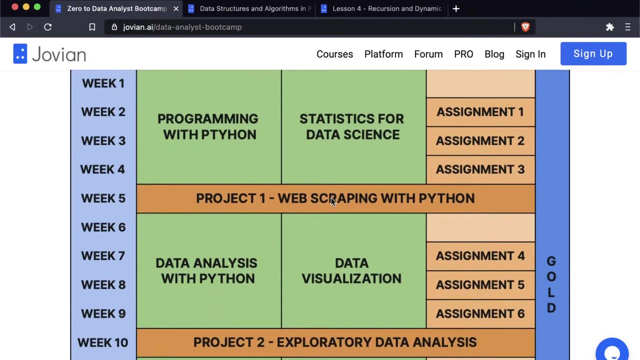 We will have classes on weekends, on Saturdays, and we will cover two courses in battle. So over the first four weeks we will cover programming with Python and statistics for data science and you will work on three real world assignments. And on week five you will build a project on web scraping with Biden. in week six to nine, 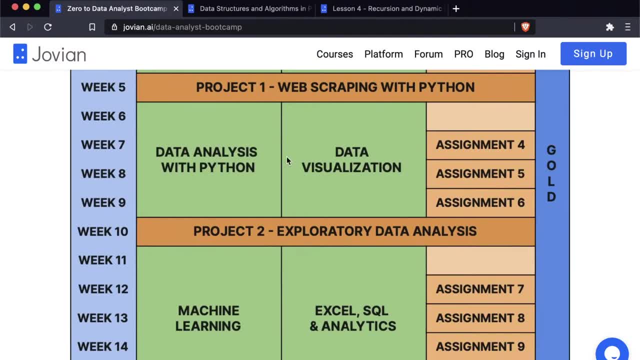 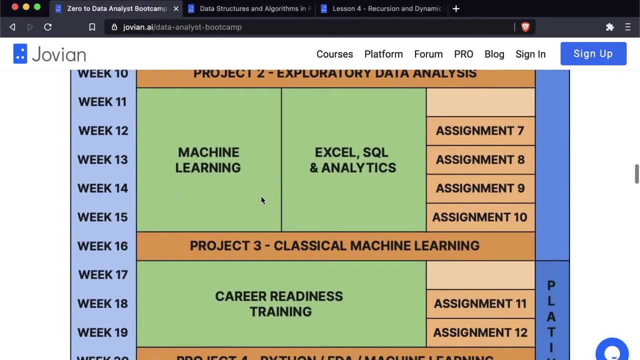 We will Cover data analysis with Python and data visualization, And here you will build a work on three assignments and build a project on exploratory data analysis. Further, we will have a course on machine learning and another course on Excel, SQL and analytics. running in battle. 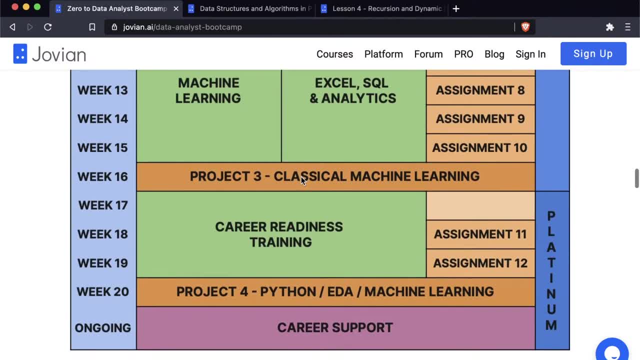 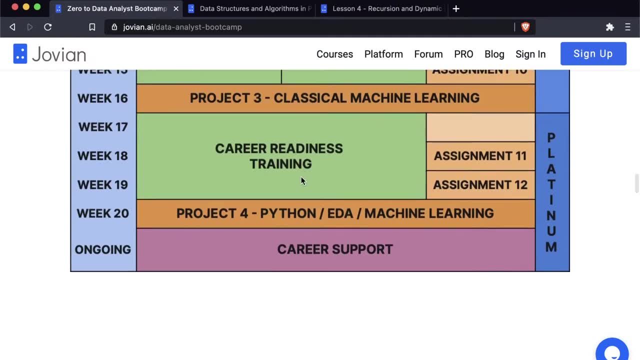 You will complete four more assignments and build a real world project on classical machine learning. And finally, we have a specific and dedicated portion towards career readiness training, which will help you prepare for interviews, build a solid professional portfolio, create a great resume and learn how to apply to jobs and get. 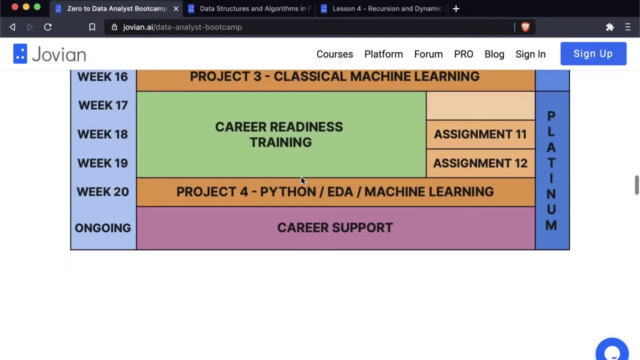 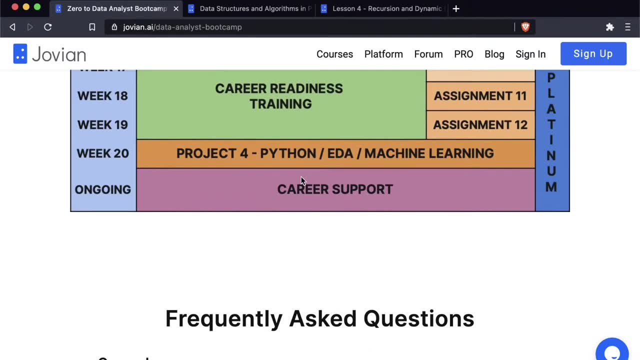 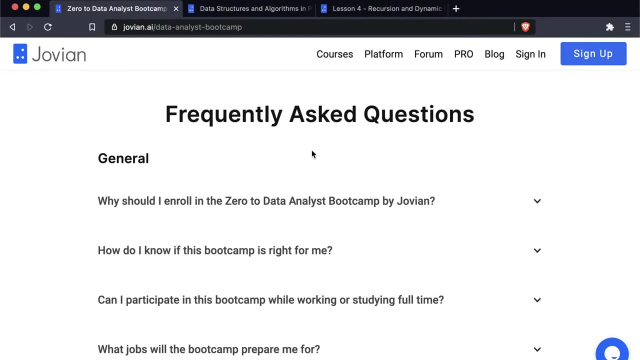 shortlisted and ace interviews. Apart from this, you will also receive ongoing career support or several months after the program. So do go to zero, to analystcom, to learn more, and you will find a list of frequently asked questions here which you can go through. 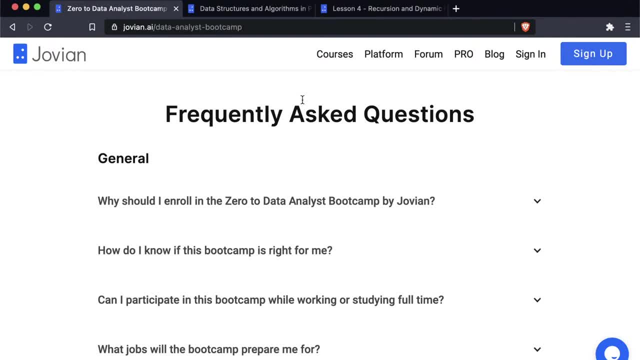 And you can also share. You will call with us If you want to learn more about this program. this is a limited program and we are only accepting a hundred participants, So do reach out to us or enroll If you're interested. all of this is happening on weekends. 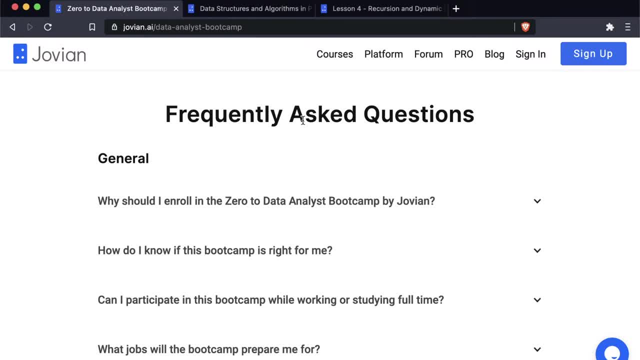 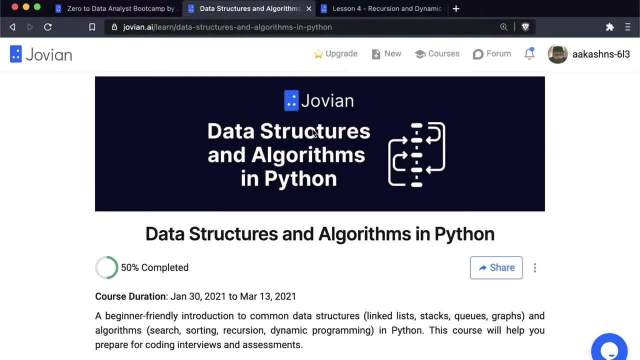 So this is part time, You can take this while working or studying and you will have ample time. Even if you have a week or two busy, you will have ample time to catch up and complete the program. Okay, So do check this out and let's go back now to the data structures and algorithms course. 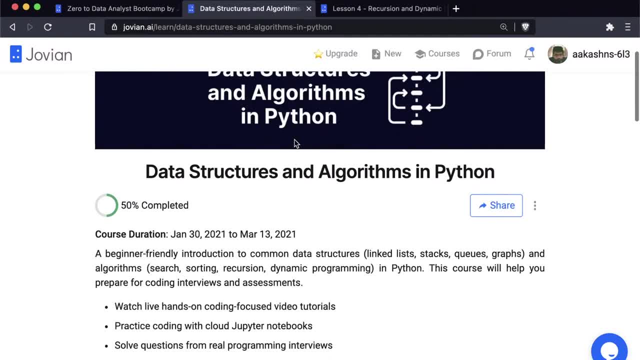 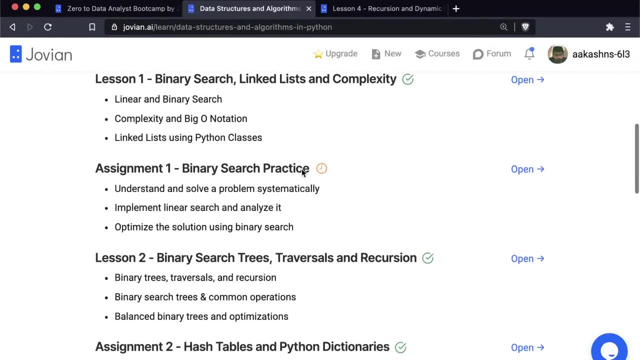 This is python. DSAcom is the course website and on the course website you will be able to find all the information about the course. So you can view the previous lessons- lessons one, two and three- and you can also view the previous assignments. 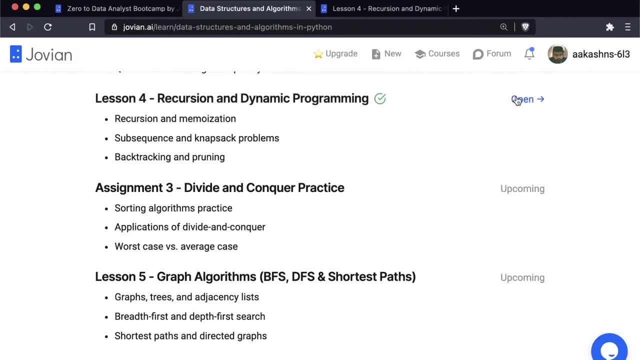 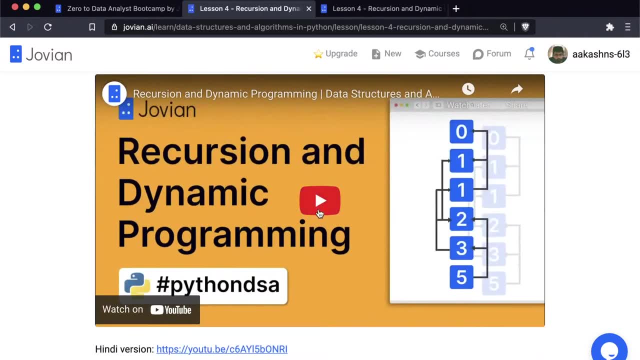 assignments one and two. Today we're on lesson four, So let's open up lesson four. The topic is recursion and dynamic programming. Okay, You can find A recording of the lesson here and you can also watch a version in Hindi. 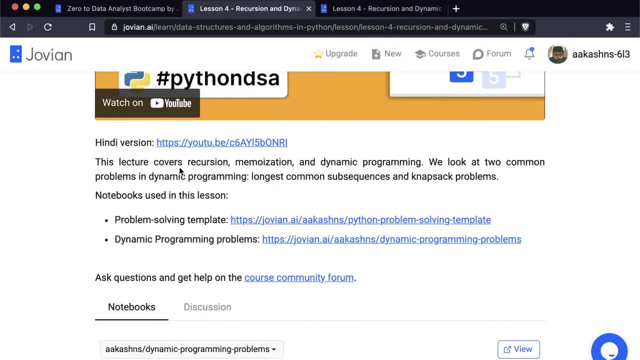 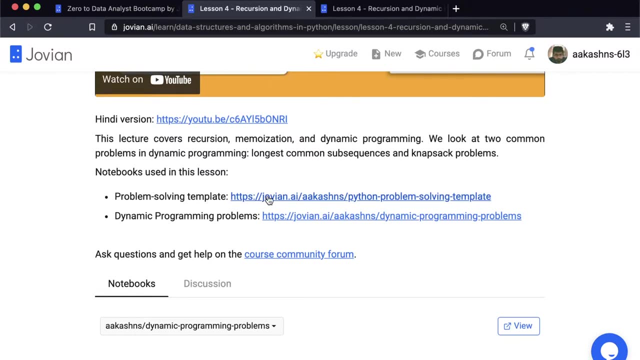 If you would prefer that in this lecture we will cover a recursion, memorization and dynamic programming by looking at two common problems in dynamic programming- the longest common subsequence problem and then the knapsack problem. And we'll do this by coding these problems live using the problem solving template that we have been using one in one. 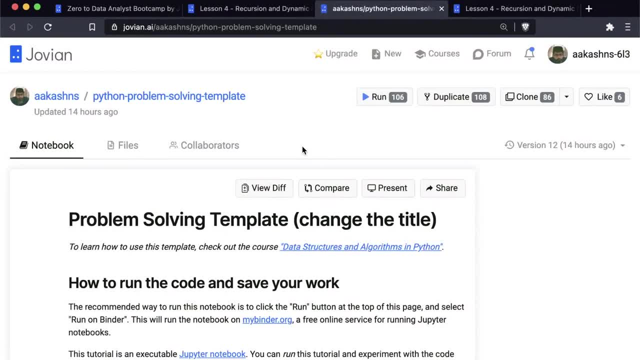 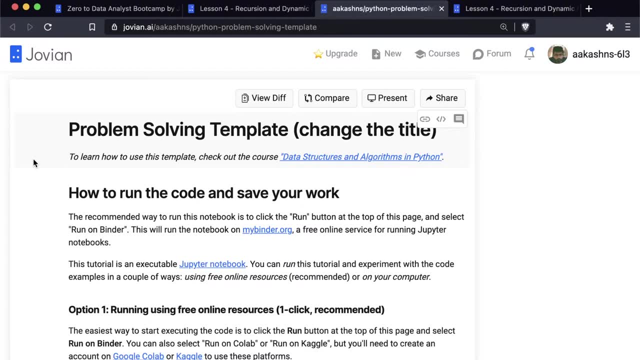 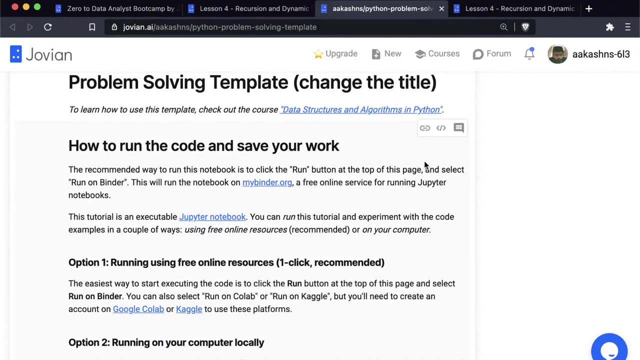 way or another since lesson one. So let's open up the problem solving template. This is a template that you can use to solve any coding problem, And we will illustrate this by solving two problems using this template today. So the first thing we need to do is to run this template. 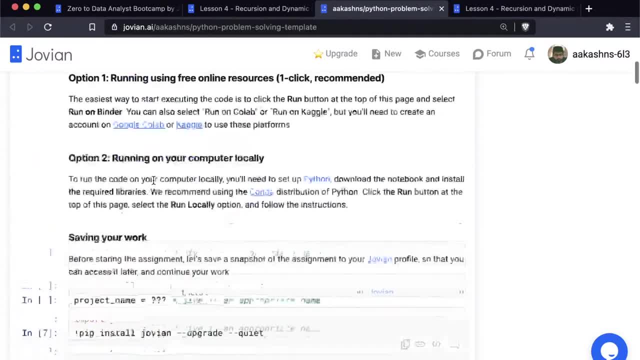 You can see that there is some explanation and then there is some code here as well. Now, to run this code, you have two options: You can run it using free online resources or you can run it on your computer. Okay, Okay. 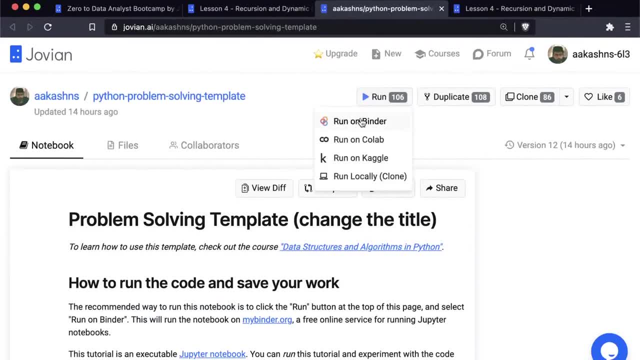 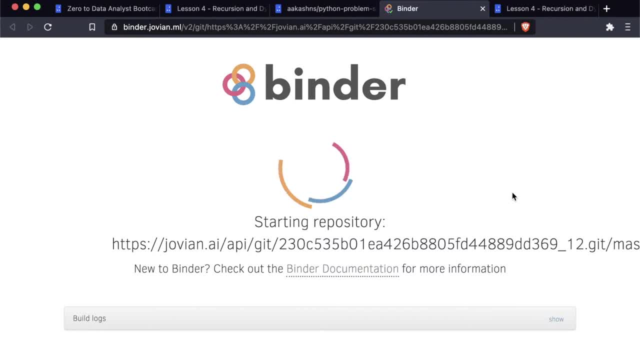 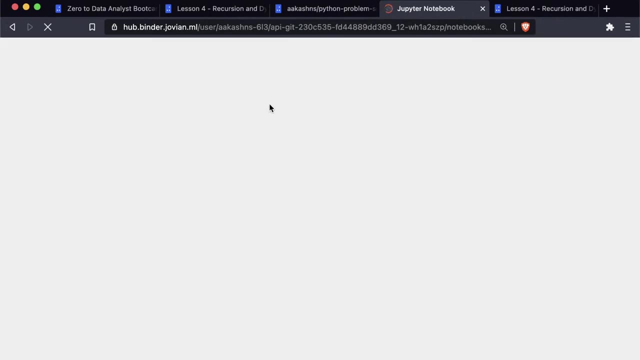 And with just one click this will set up a machine on the cloud for you, Start a Jupiter notebook server, and you will be able to then Execute the code and modify the notebook and save a version of it to your own profile so that you can continue. 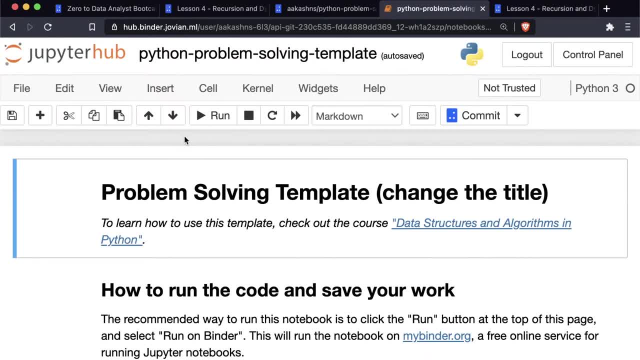 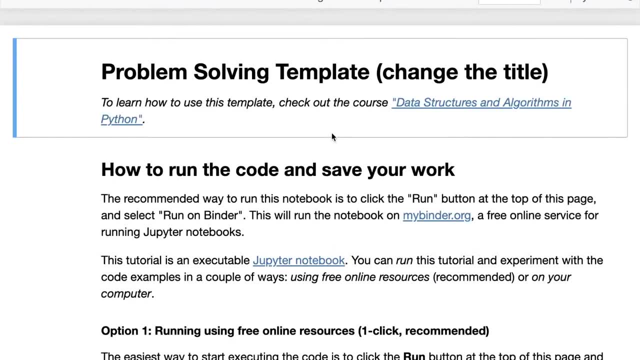 So there we have it. Now we have a running Jupiter hub server. I'm just going to zoom in here a bit so that you can see things clearly. Okay, So this is the problem solving template, And I said we're working on two problems. 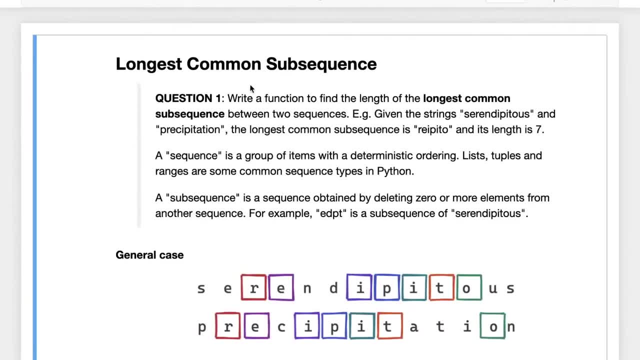 So I have some problem statements listed out here. You can see the first problem longest common sub sequence is listed here And this is a part of the lesson notebook lesson page as well, So you will find link to this problem statement on the lesson page too. 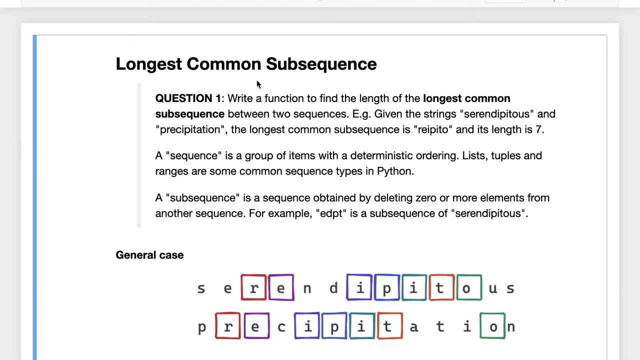 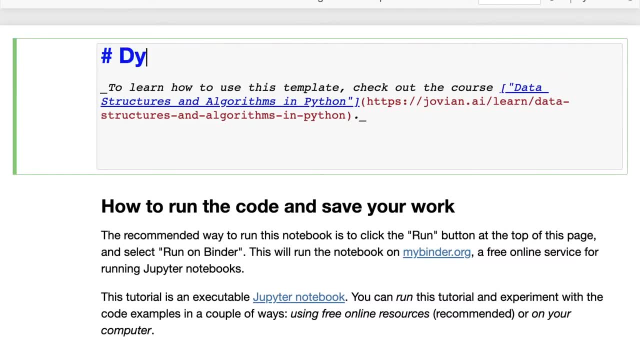 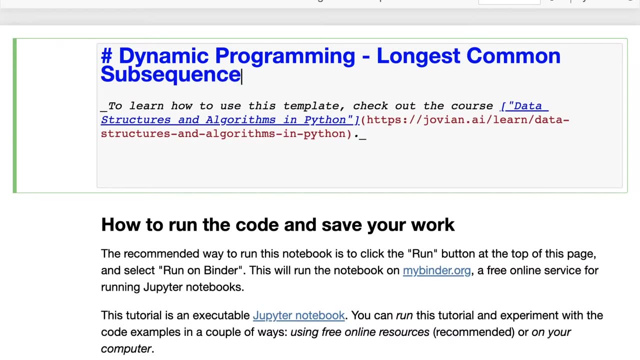 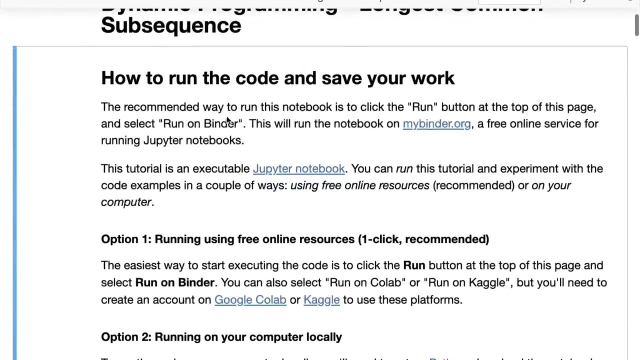 So let's first modify the title of this notebook: problem solving template. Let's change this title to dynamic programming- longest common sub sequence. Let's get rid of this, And then we have the problem. I don't think we need this. Then I'm going to keep the section on how to run your code so that if I share this, 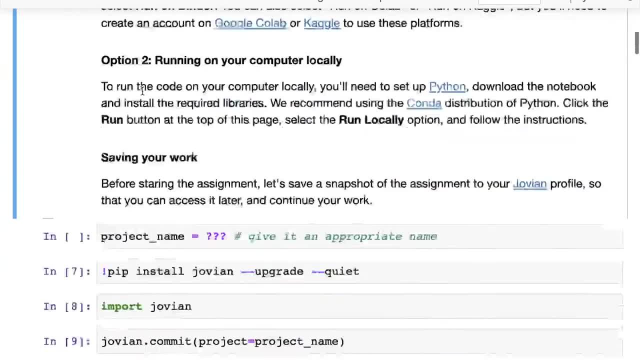 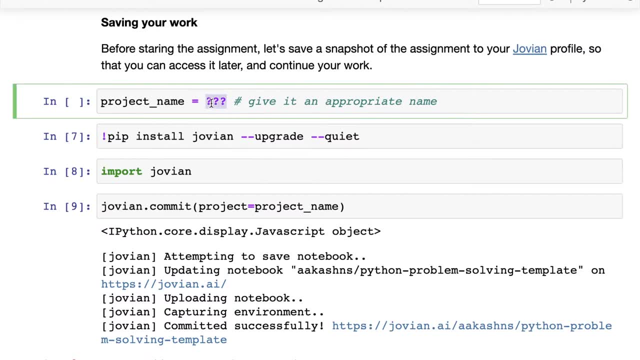 notebook with somebody else, they have a way to run it, and then, before we start the assignment or the problem, let's just save this to our own profile. So I'm just going to give it a name: longest common sub sequence. This is an appropriate name for it. 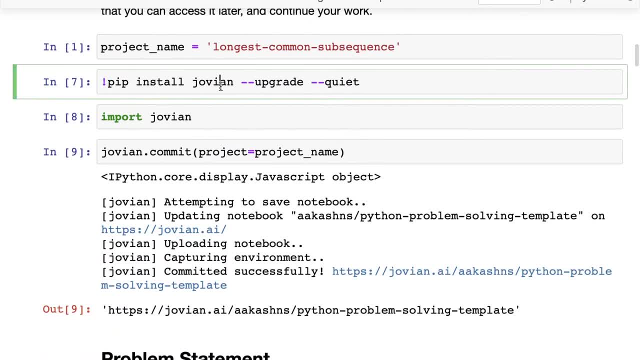 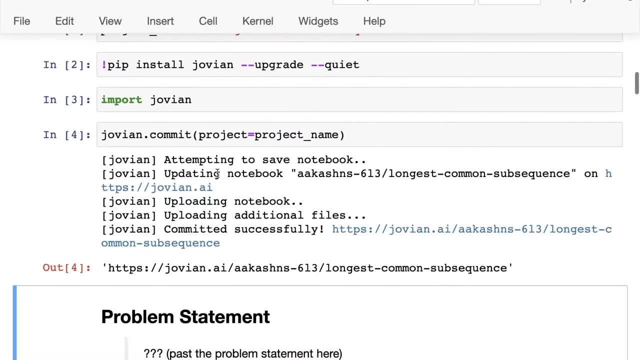 I'm going to give it this a project name: install the Jovian Python library and just run Joviancom it. Now, what this will do is we started out with a template and now we're editing the template by running Joviancom it. 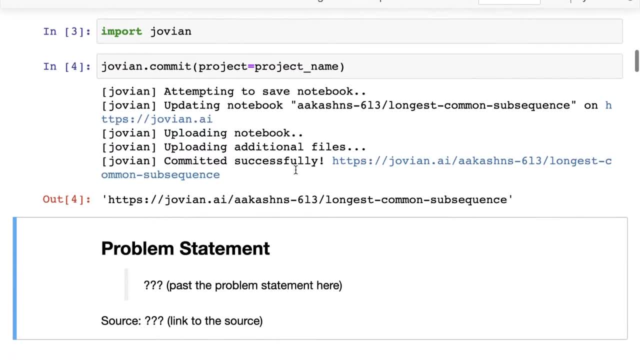 We've saved a copy of the template to our own profile. You can see, this is the link where you will be able to access this notebook and you can run it and continue your work If this Jupiter notebook shuts down. If you want to run it. 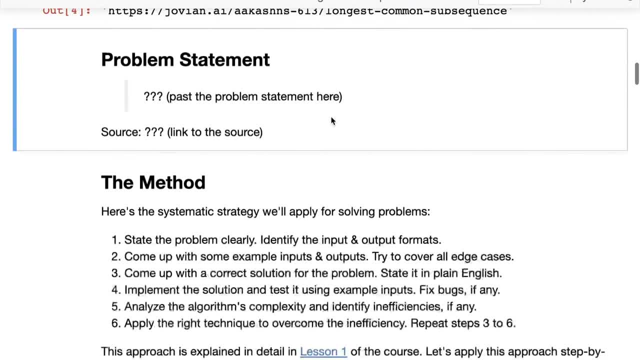 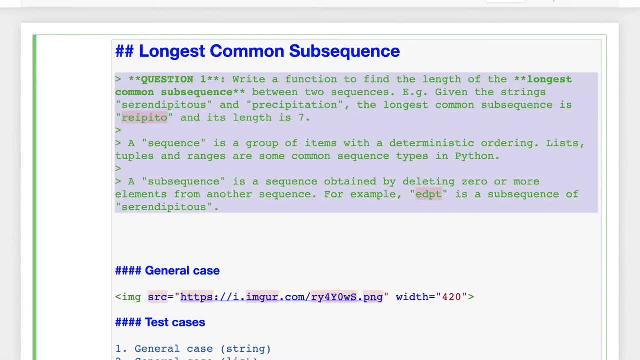 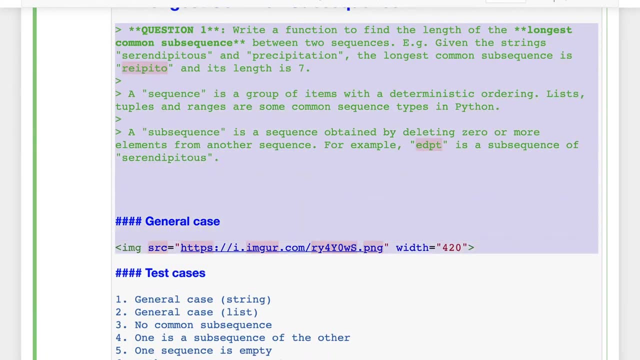 If you want to continue tomorrow, for instance. okay, so now let's look at the problem statement. Now I'll just copy over the problem statement here as well, so that we can see it directly within the notebook. There we have it. 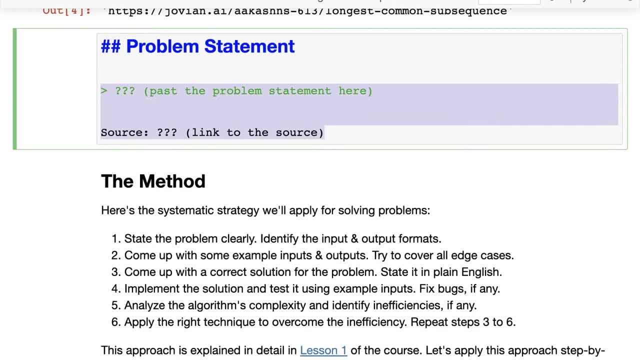 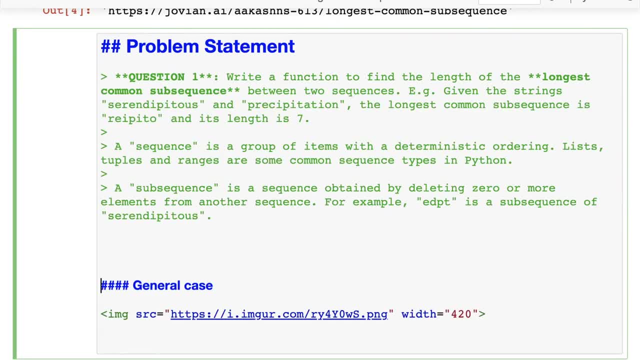 Now you can paste the problem statement, And if you are getting this from statement from some other source, then it's always a good idea to include the link to the original source as well. Okay, now we have a problem statement in front of us. 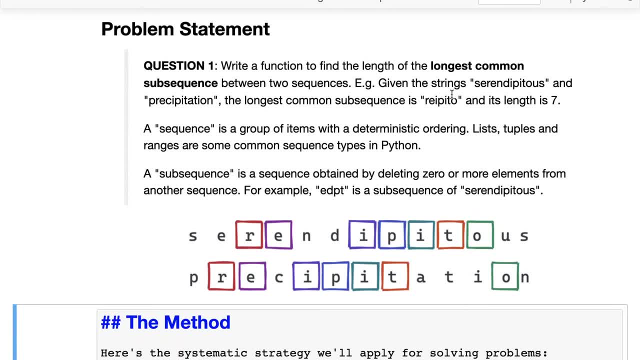 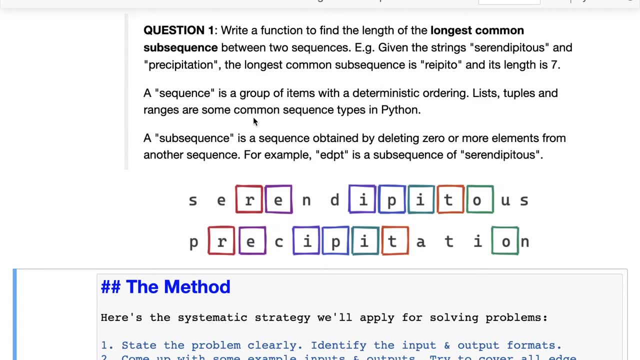 So the question is right: A function to find the length of the longest common sub sequence. So that's a new term. We'll unpack that between two sequences. Now let's first learn what we mean by a sequence. Our sequence is a group of items with a deterministic ordering, for instance a list, a tuple, a range or even a string. 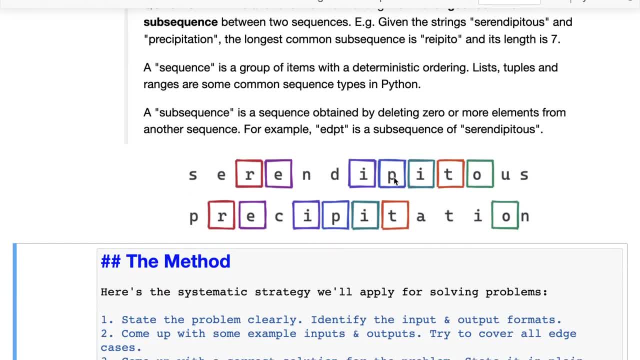 These are some Common sequence types in Python, So here I have the string serendipitous. This is a group of items And this also contains an order. You can see that E comes after S and R comes after E, and so on. 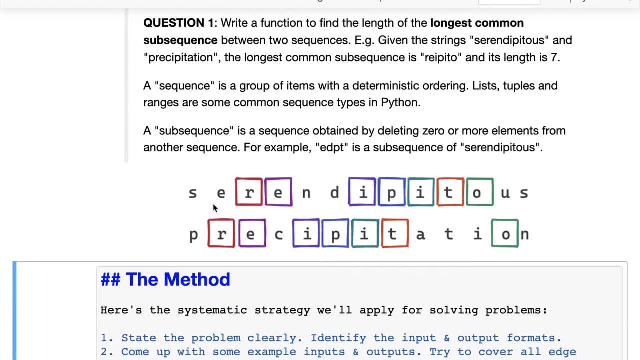 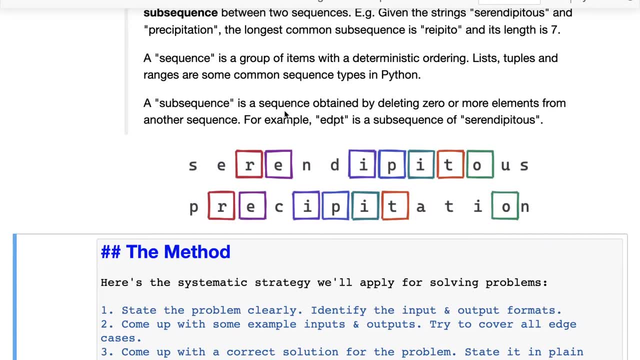 So this is a sequence. A list would also be a sequence. So that would be a list of numbers. So that's a sequence. Then we're looking at sub sequence. What is the sub sequence? Now, a sub sequence is a sequence that is obtained by deleting or removing zero or more elements from another sequence. 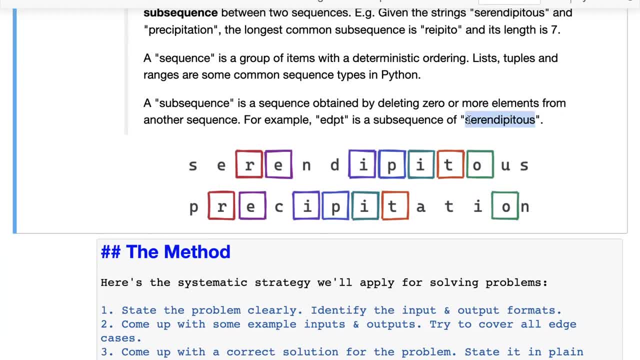 For instance, if you look at Okay, Serendipitous, and if we remove the characters S, R, E, N, I, I O U S, then you will be left with E D P T. So E D P T is a sub sequence of serendipitous. 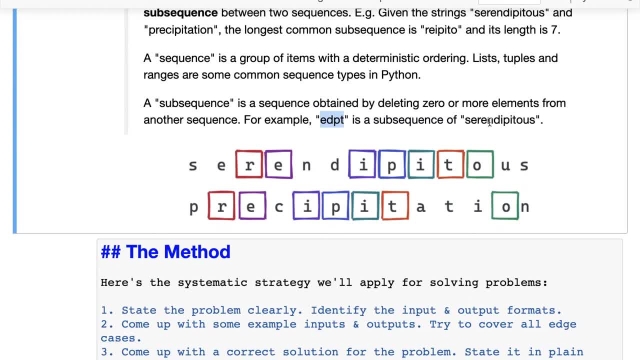 Now two things to note here. E D P T does not have to occur continuously, So these elements can occur anywhere within sequence, but the order should be the same. So E D P T occur in this particular order here And E D P T should occur in the same order here. 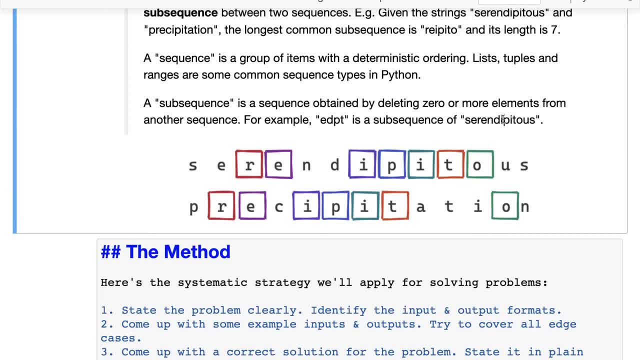 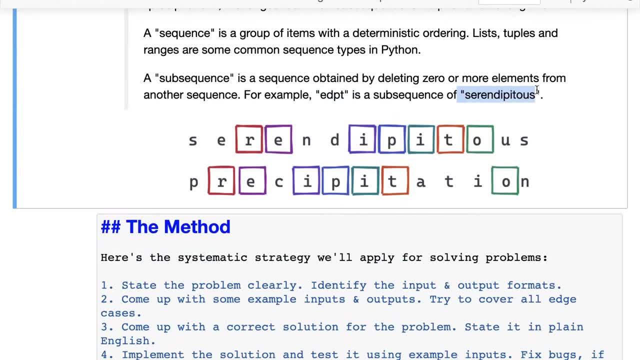 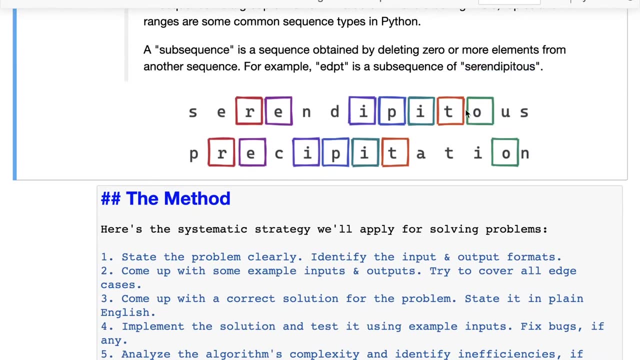 So D should occur after E and P should occur after D and T should occur after P. So those are the two requirements for E, D, P, T to be a sub sequence of serendipitous. And visually speaking, what we can see is if you take a sequence and then you draw boxes around some of these characters or some of these elements of the sequence, 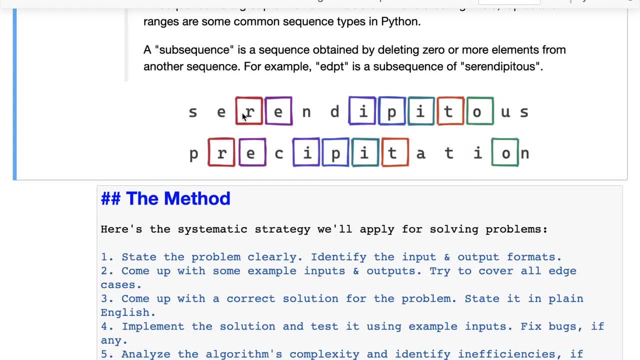 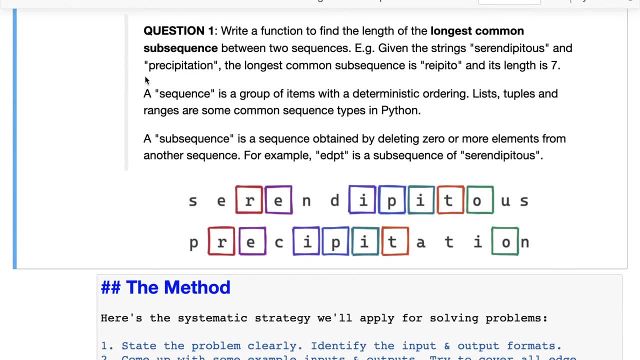 And if you just take the elements in the boxes, then in the same order, then you end up with a sub sequence. So now we understand what a sequence is and what a sub sequence is. And once again, if this is this question is asked in an interview and you're not sure what you mean by longest common sub sequence then, or even what a sequence is, then you should ask the interviewer: what do you mean by a sub sequence? 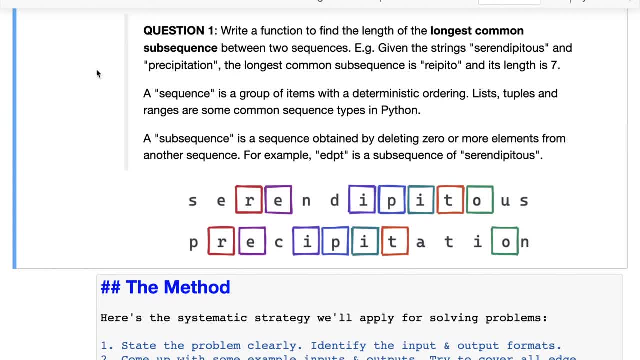 Or what do you mean by sequence, And they'll be more than happy to tell you. It's very important to communicate, whatever you're thinking, whatever questions you have. contrary to what you might think, asking questions is actually a good thing, The more 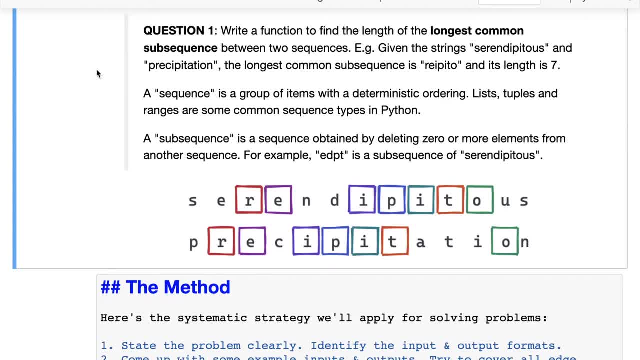 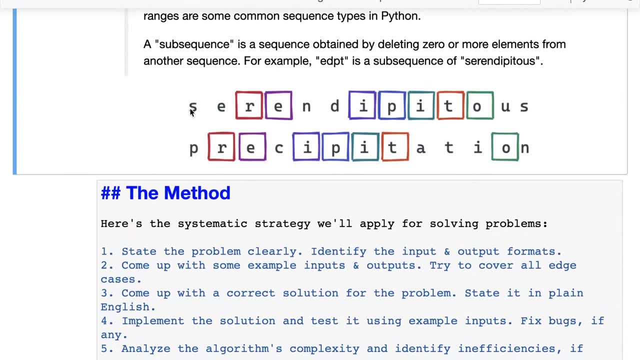 The more questions you ask, the more it is appreciated. Okay, So now we've talked about a sequence and a sub sequence. Now what's a common sub sequence? So let's look at these two strings: serendipitous and a precipitation. 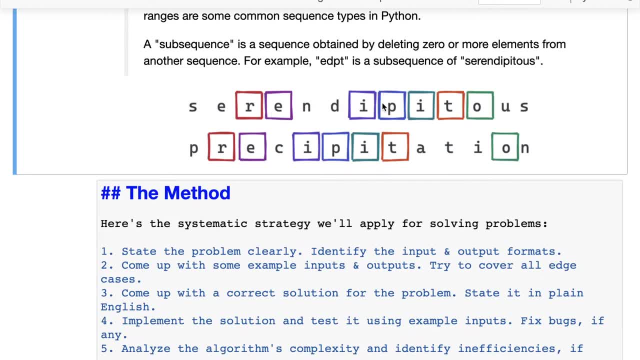 Now, if you pick just these elements that are in the boxes R E I P I T? O, now, you can see that R E I P I T? O is a sub sequence of serendipitous and R E I P I T O. 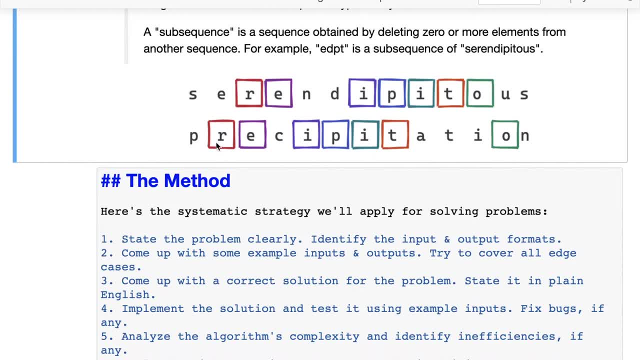 Also a sub sequence of precipitation. So a sub sequence which is common, which is a sub sequence of both sequences, is called a common sub sequence. So R E I P I T O is a common sub sequence between serendipitous and precipitation. 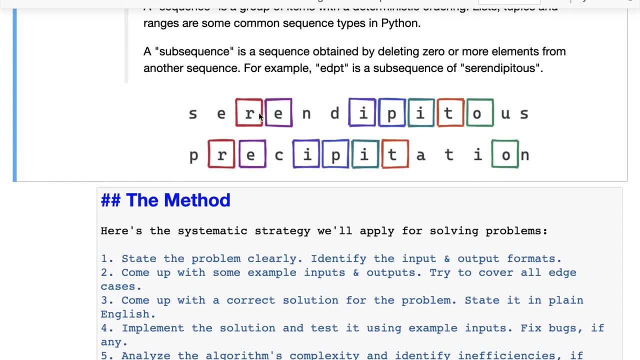 Now you can have many common sub sequences. For instance, we could just look at R E and R E here, and R E would be a common sub sequence too. Or you could just look at: Okay, I T and I T, and that would be a common sub sequence as well. or we've not picked N here, but you could also pick R E N and R E N. 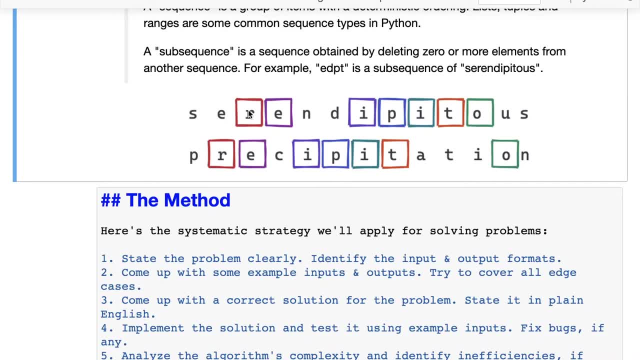 And that would also be a common sub sequence between the two. Now, the longest common sub sequence, as the name suggests, is the sub sequence which, between the common sub sequence between the two sequences which has the maximum possible length, And you can verify this. 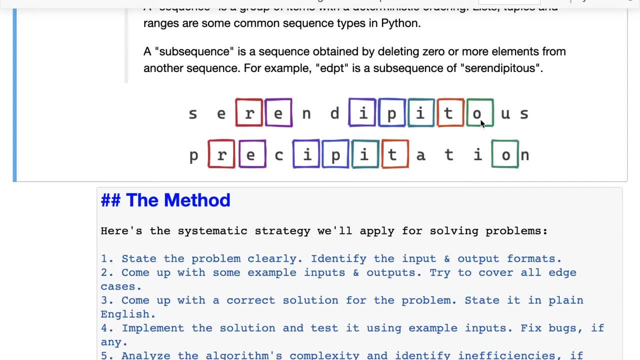 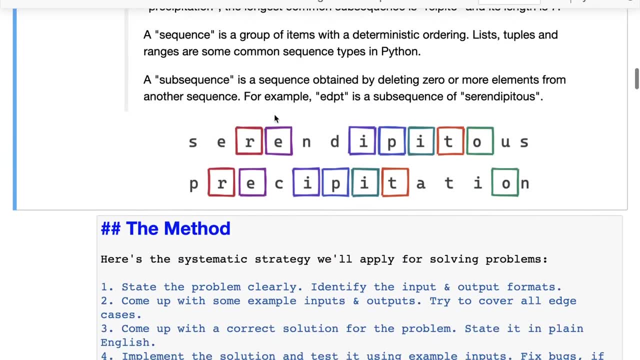 You can try different sub sequences and see that R E I P I T O Is the longest common sub sequence between these two strings, these two sequences, and its length is seven. one, two, three, four, five, six, seven. 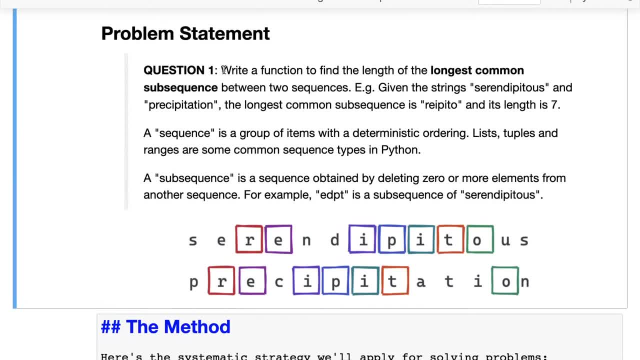 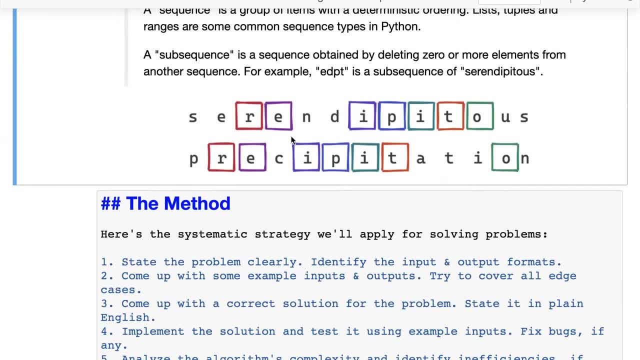 So you have to write a function to find the length of the longest common sub sequence between two sequences. So that's a question And this is an visual example that tells you the answer. Okay, Now that we have the question, we've understood the question. 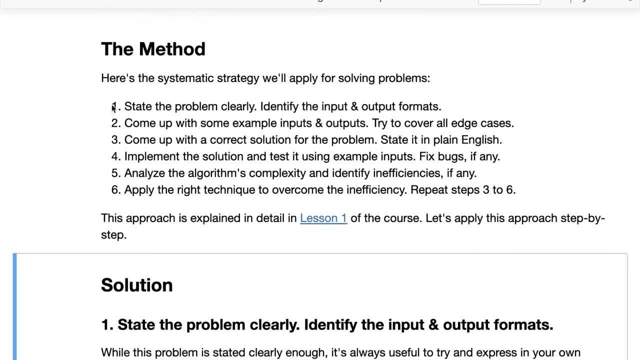 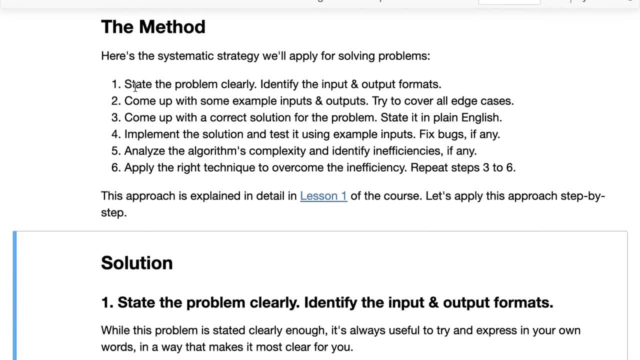 We can start applying the method that we have been learning throughout. So this is a systematic strategy that we will apply, And nothing about this method has changed since the first lesson, even though we've covered a whole variety of topics like binary search and binary search trees and then sorting algorithms and divide and conquer. 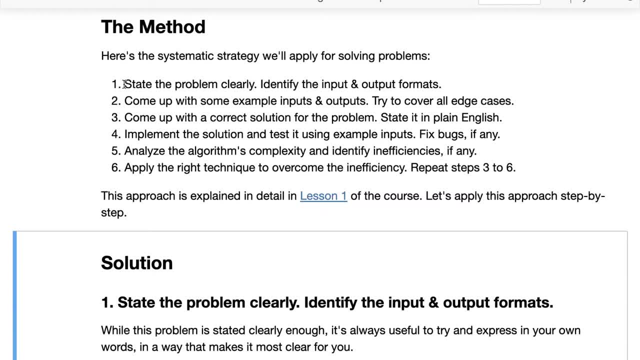 This method has remained the same. The first step is to state the problem clearly and identify the input and output formats. Then the second step is to come up with some example inputs and outputs, And these will be used to test our solution. So we should try and cover all the edge cases, and that will help us write code that is correct. 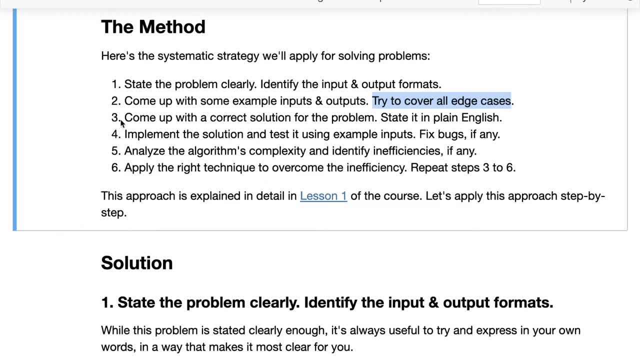 Anticipating all the errors that we might face. Then we come up with the correct solution to the problem and stated in plain English. very important for you to state the problem in plain English before you start coding, so that you communicate your ideas and you also make it clear once you express yourself, then you implement the 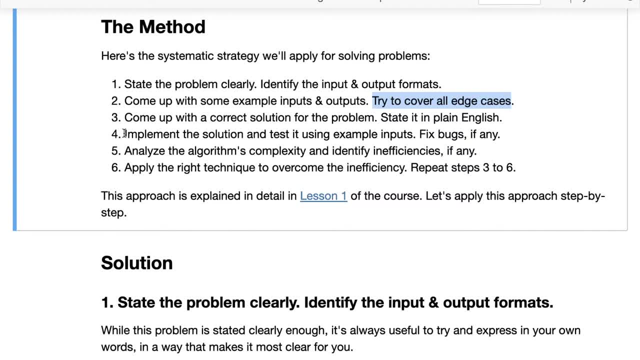 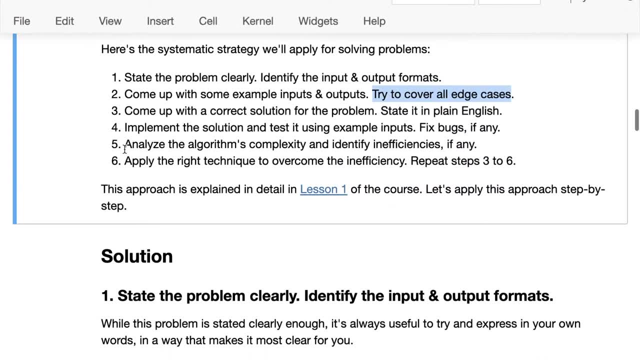 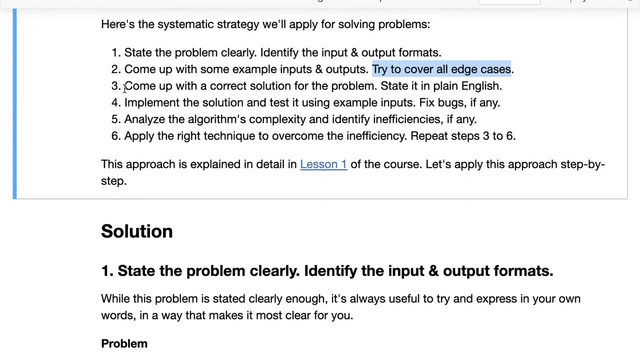 solution And test it using example inputs and you fix bugs if you find any of them- and you will be able to find bugs if you have written good test cases. then you analyze the algorithms, complexity and identify inefficiencies if you have any, and most likely the first solution that you come up with. it doesn't have to be optimal. 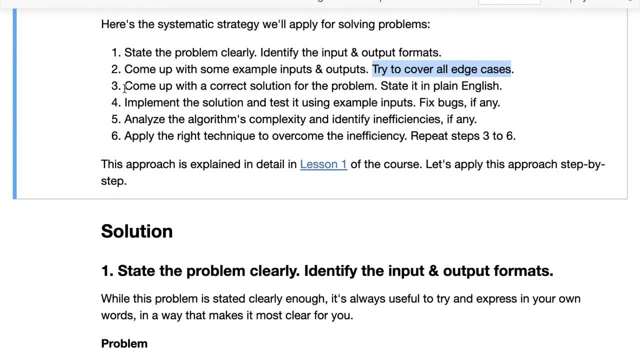 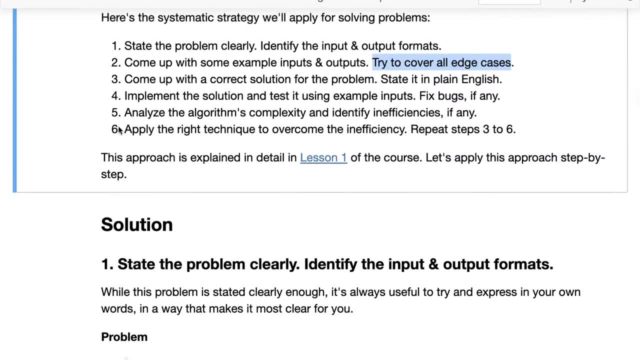 It just has to be correct. So there will be some inefficiency. but it's important to go through that process of first finding a brute force solution and then finding the inefficiency and then apply the right technique to overcome it. You overcome the inefficiency and repeat steps to three to six. 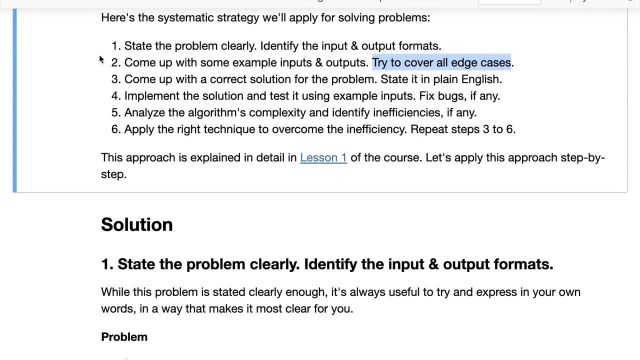 So you identify what's the right technique- And in this case we will learn a couple of techniques called memorization and dynamic programming, And then we go back and state the correct solution again. Then we implement the solution and test it, and then we analyze it again. 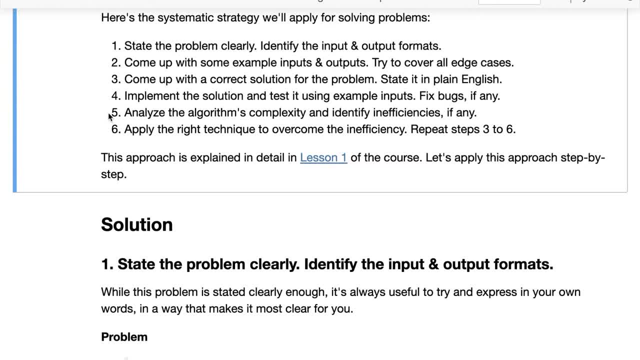 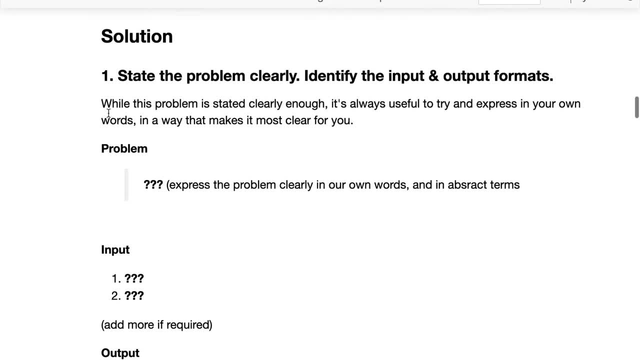 And if there's further scope for improvement, we do that. Otherwise, we say that we've arrived at a optimal or good enough, optimal enough solution. Okay, I hope by this point this you've started to memorize this process, And that's why we keep repeating it over and over, that it should become second nature every time you see a problem. 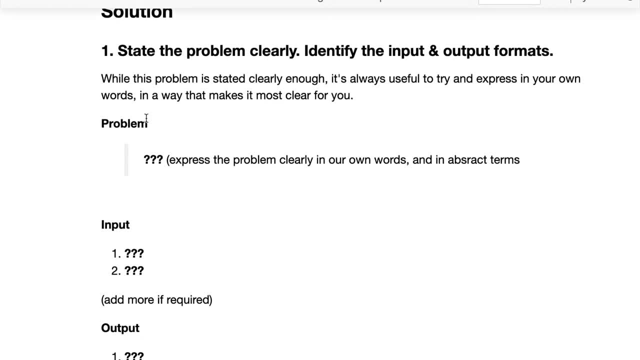 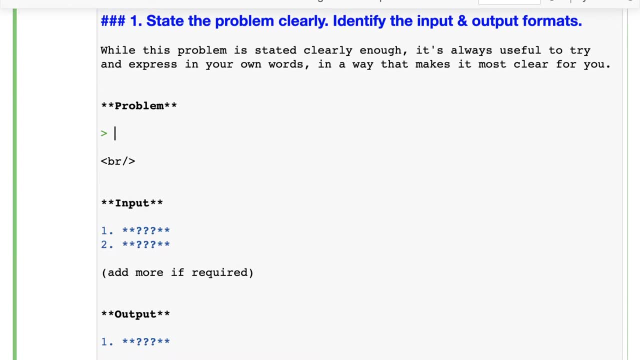 So the first thing is to state the problem clearly and to identify the input and output formats. Now the problem is already stated clearly enough, but let's just state it slightly more clearly. So let's say we are given, and just write it in your own words. 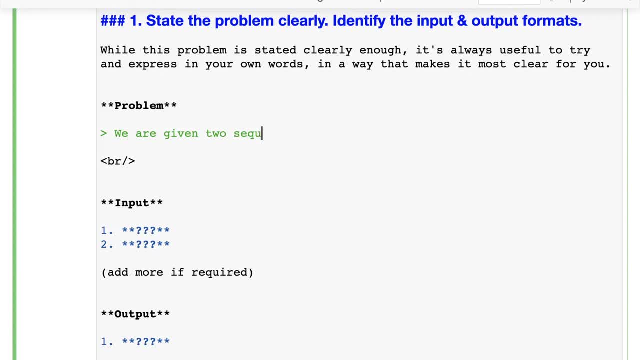 That's more important. What, whatever is clear to you. So we are given two sequences And we need to To find that length of the longest common sub sequence between them simple enough. then we have two inputs. Now we decide the input and output formats. 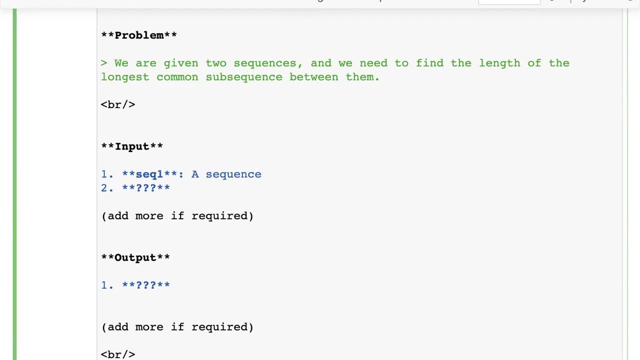 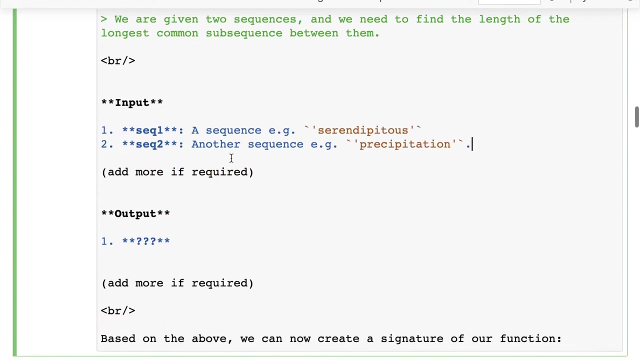 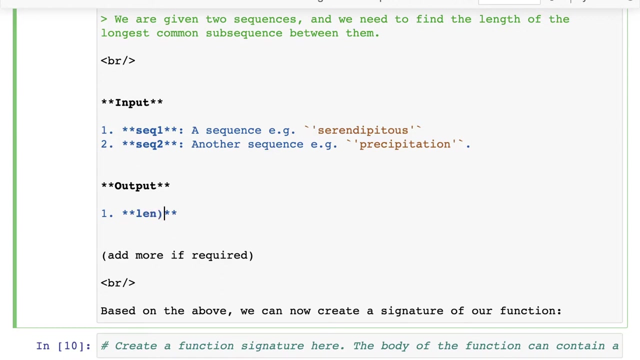 We have sequence one- a sequence example- serendipitous sequence. We have sequence two- another sequence example: precipitation and this. these are the only two inputs that we require, and the output would be the length of the longest common sub sequence. 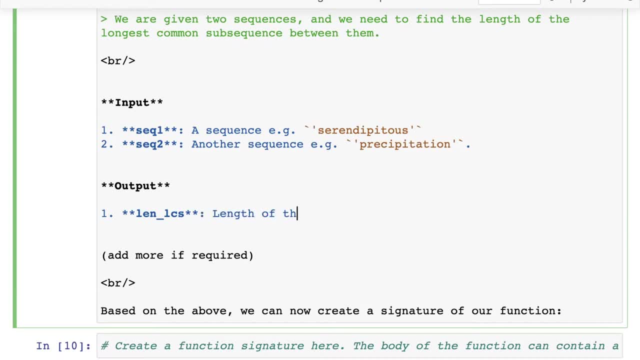 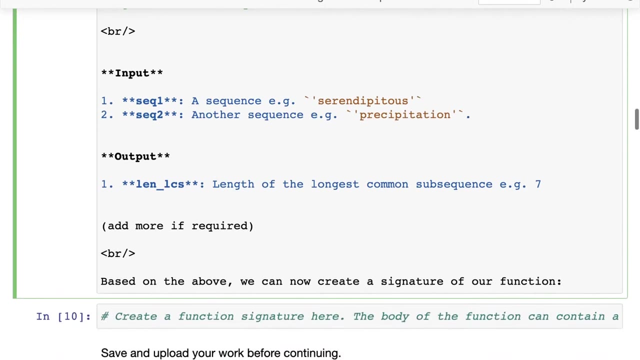 Let's just abbreviate it. Let's just abbreviate it. Let's just abbreviate it. Let's just abbreviate that as LCS, which in this case is seven, and we know what that sub sequence looks like. We've just seen it above. 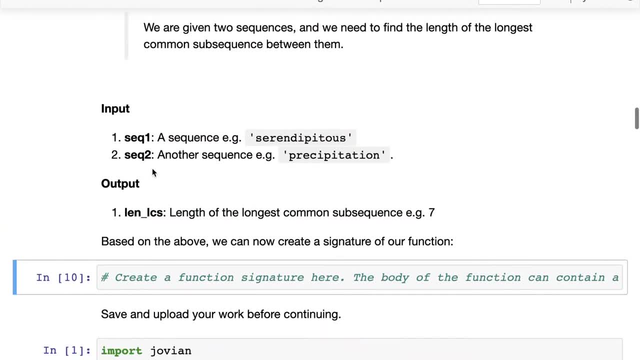 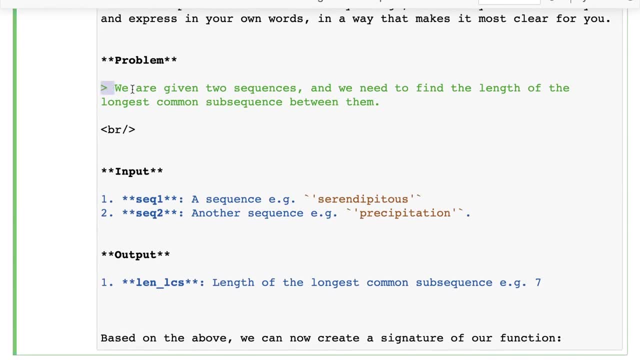 So now, based on this, we can now create, and you can see the problem is now created. And before I talk about the next thing, if you double click on a textile, you can start, And here we are using a language called Markdown. 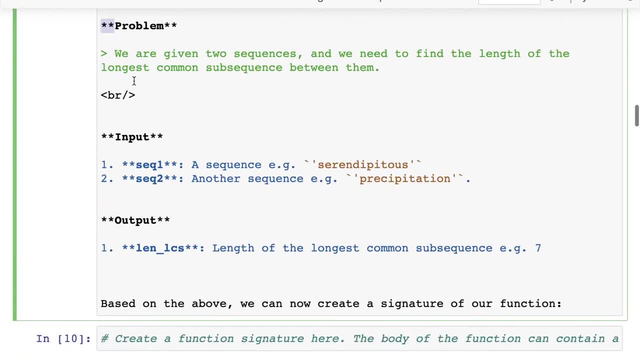 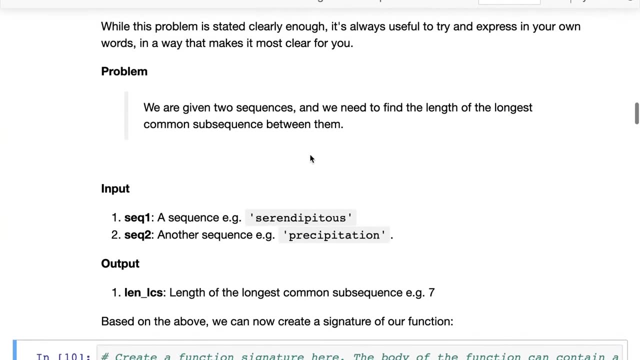 So you can see, this creates a block code, This creates a bold font and this creates a code like font. So let's see here: And the way to go back into the display mode is to press shift plus enter. Now you can see here that now we have the problem. 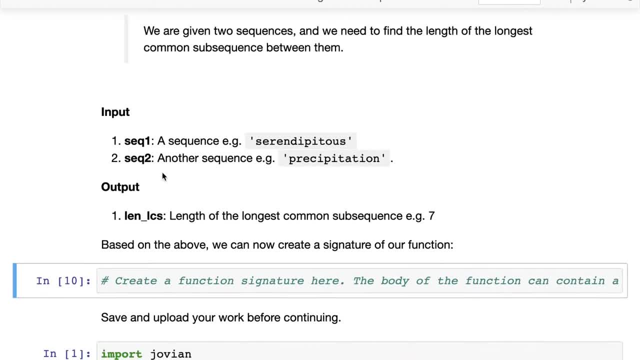 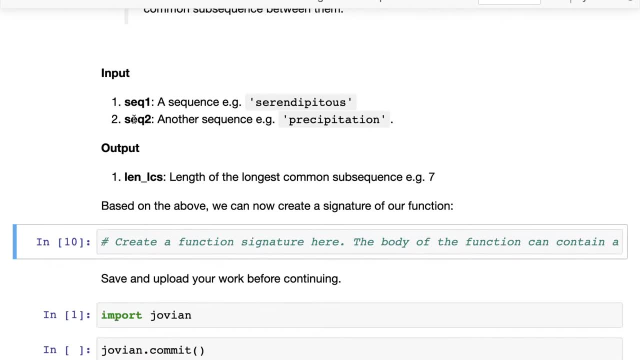 We have the block code and then we have all the styling. So Markdown is a really useful and easy to learn language for formatting your text, especially in Jupiter notebooks. So do learn it. But now, based on this, we can now create a signature of our function. 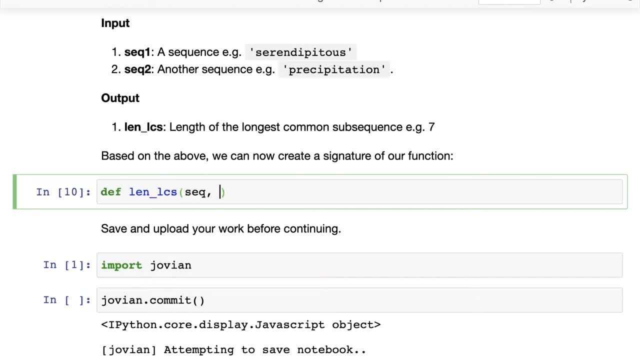 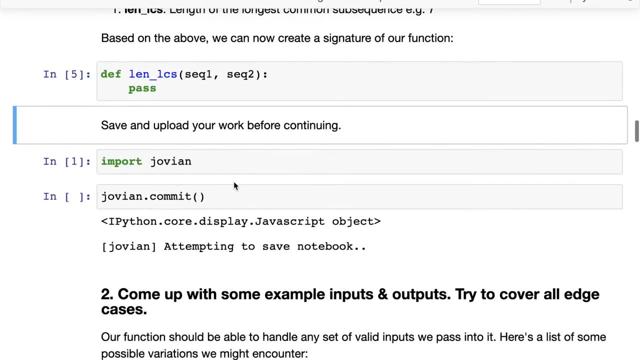 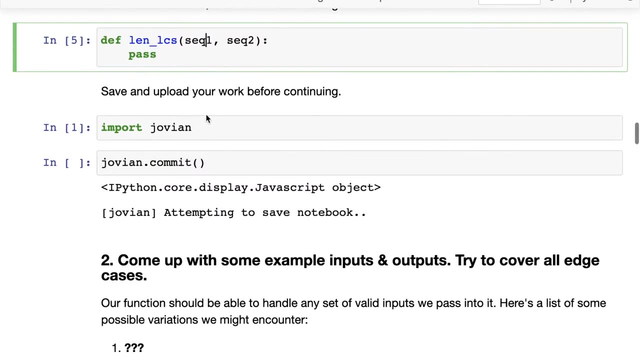 So our function, Len LCS, will accept a sequence, sequence one and sequence two, and it will return something. So that's the basic signature of our function And, even though it's not doing much, just establishing what the arguments are is the first step towards solving a problem. 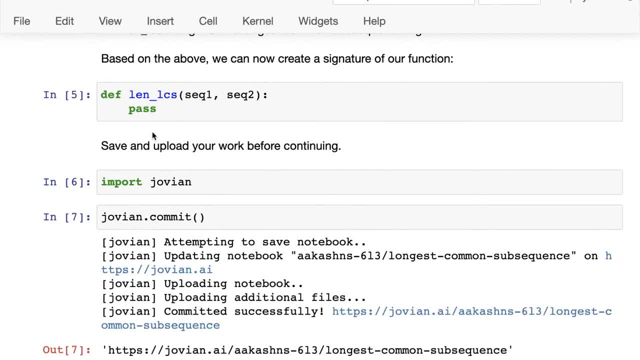 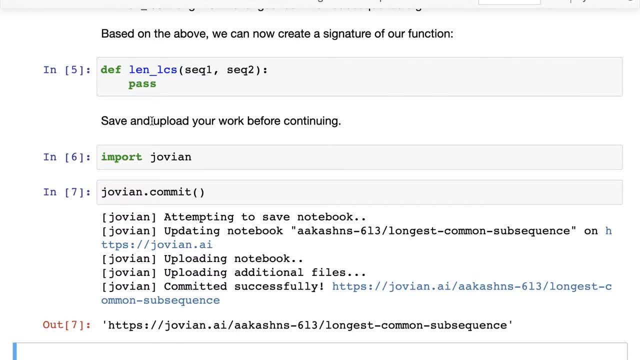 And let's just save our work from time to time. It's very important to keep saving your work on Jovian Because this is running on a free online service, So this will shut down after some minutes of inactivity. So just run Joviancom it and that will save the notebook to your profile and you can read on it. 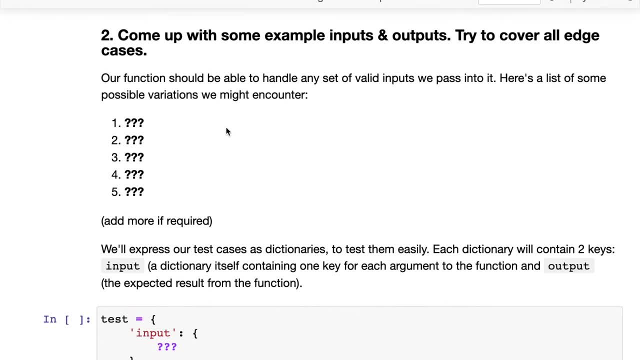 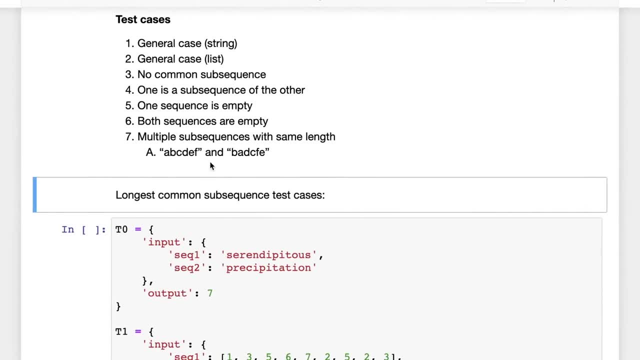 Okay. So then now the next step is to come up with some example inputs and outputs, and here we need to try and cover all the edge cases. So I have written out a few test cases here already. Now the most common case is a general case of a string. 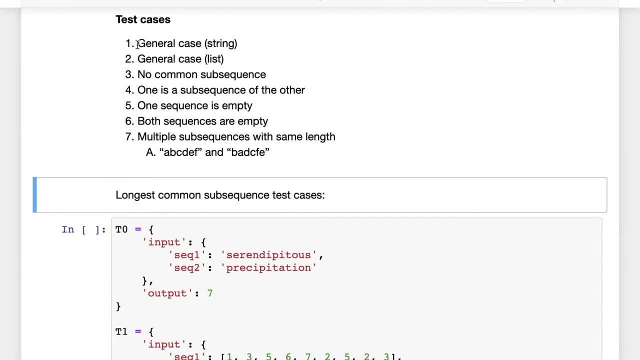 Like we had seven, And if it is in precipitation, that's a common case, there is one of them. Both of them have some common elements and there's a subsequent common subsequence of length seven. But we may also want to test out another type of data. 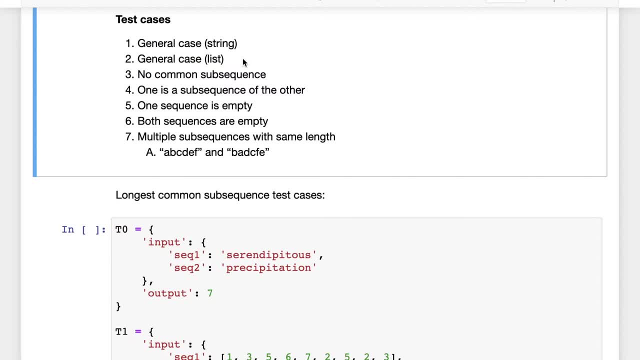 And this is one of the nice things about Python, where you can write functions that operate not just on a particular class and its subclasses, but on any kind of data, as long as it satisfies certain criteria. for instance, strings and lists both allow indexing into them. 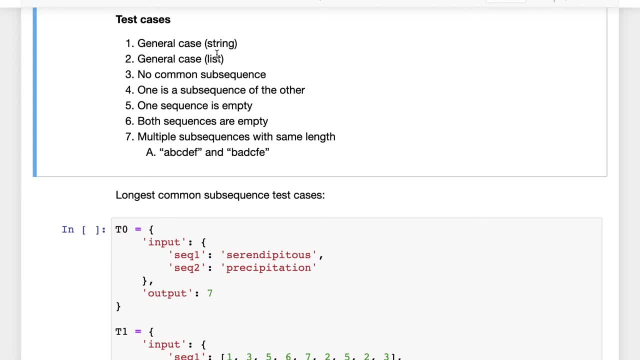 And picking out the ith element or the nth element from the sequence. So they're both sequences, So our function should be able to walk with both strings and with lists. Then here is another case where we have two sequences and they have no common sub sequence. 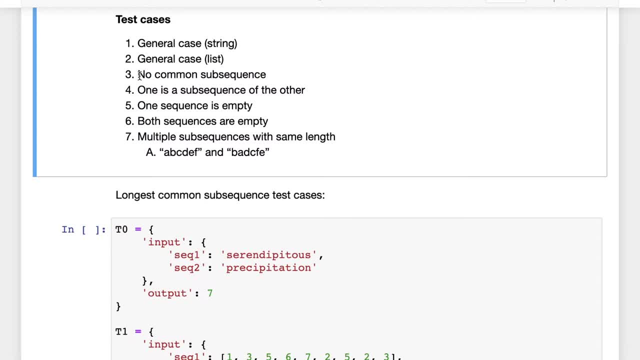 A function should not throw an error here. It should gracefully return the number zero, because the empty sequence is a sub sequence of every other sequence. Does that make sense? Think about it. So in that case, if you, if there's no common sub sequence, then the empty sequence is the common sub sequence. 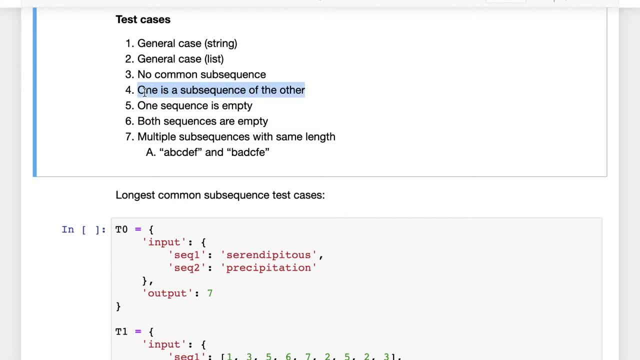 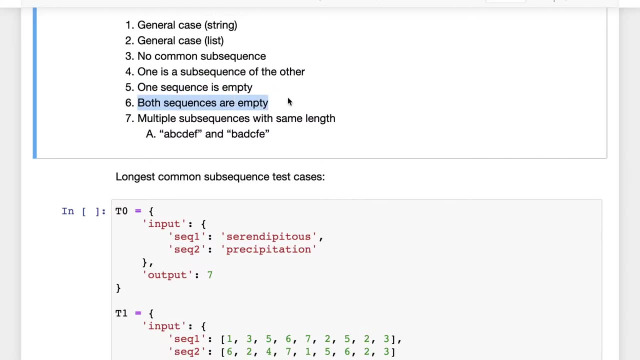 So the answer is zero. And here's one other extreme case where one is a sub sequence of the other. Here's another case where one sequence is empty. Here's another case where both sequences are empty. All of these are important, Otherwise you might miss out certain special cases and you will face an error when you code your solution. 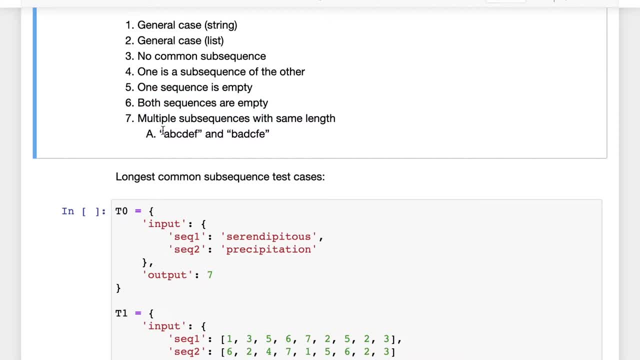 Finally, you can also have this case where you have multiple sub sequences with the same length, For instance, if you have ABCDEF and BADCFE and ACE. ACE is one long sub sequence, of length three, and that's the longest you can verify. 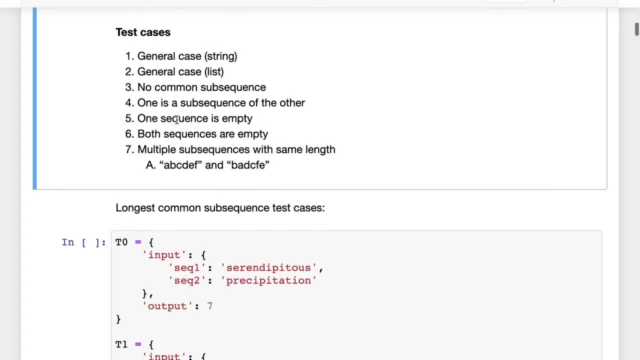 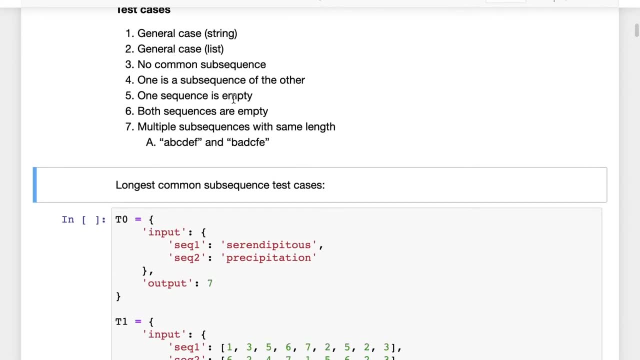 And BDF is another sub sequence which is common to the two and also has the same length. Those are some test cases. Now let's copy over these test cases here in an interview or a coding assessment. What you might want to do is just write these as comments. 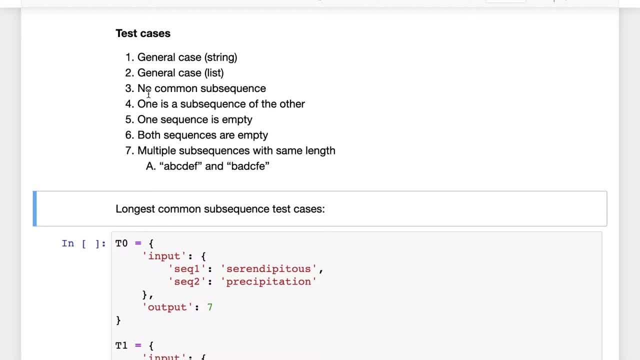 If you have just a single coding screen and try to list at least four or five, but go as far as you can, because this will also help you streamline your own solution And it's always something that is appreciated by interviewers. 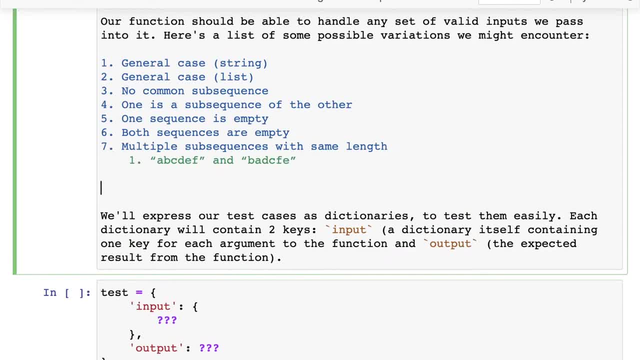 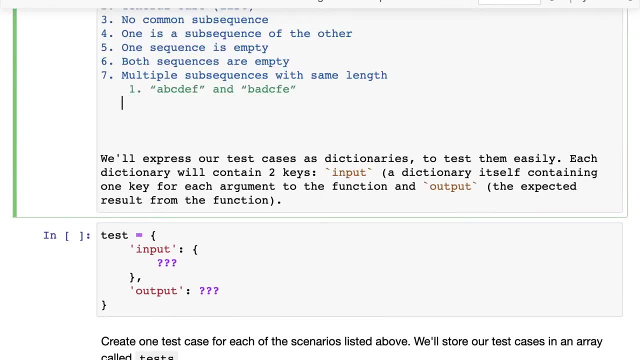 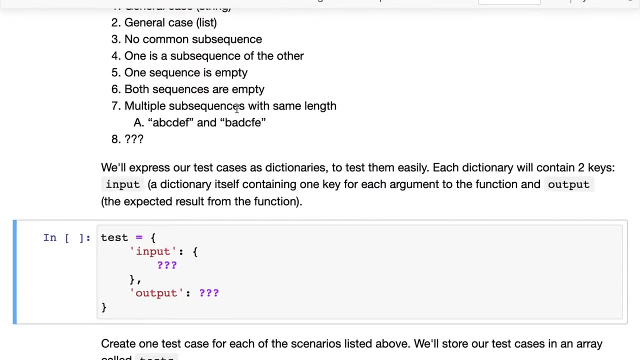 Let's do that, Let's get, let's copy over these test cases here and you can think of more. So if you have some more ideas of things you should test, come up with them. There's no right number of tests. Whatever it takes for you to feel confident is what you need to do. 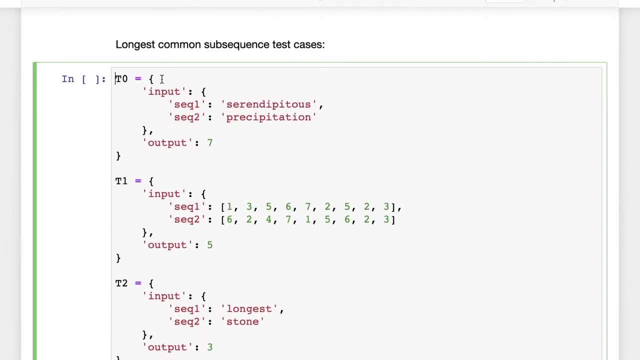 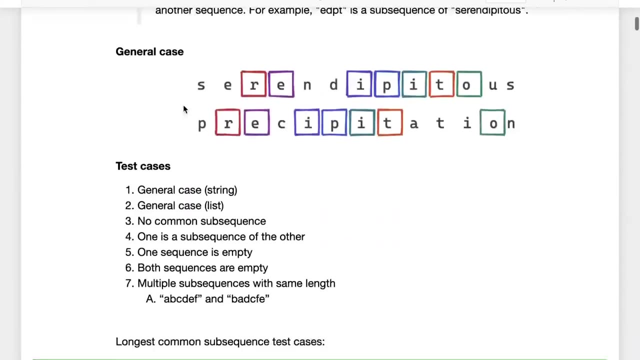 Okay, So now what we've done is we've taken these test cases and converted them into dictionaries, So you can see, here we have this first sequence, sequence one, and remember, that's why we've written out, Oh, that's why we've written out here- the names of the inputs and the signature of the function. 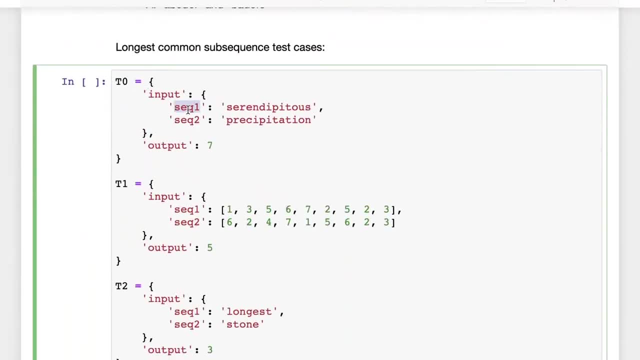 Now we can create test cases as dictionary so that we can test them all easily all at once. So we have the sequence one and sequence two in the input sub dictionary, inside the main test case dictionary, And then we have the output, which is the output of the function, which should be seven, and this you can verify. 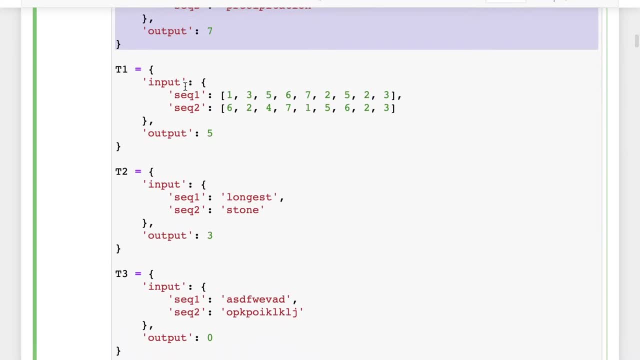 So this is a general case, but then we have another case. in this case we have two sequences. These are both lists of numbers, And in this case the output that we expect is five. And we have another general case: longest and stone. 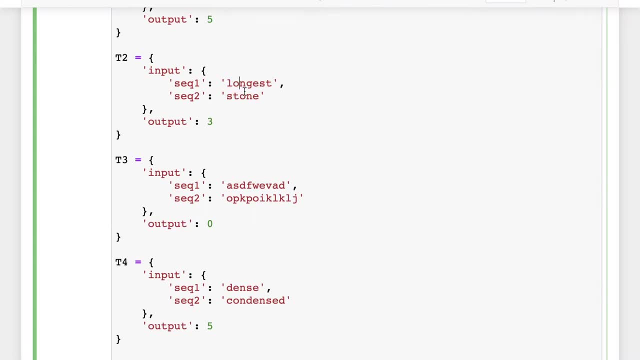 In this case you can verify that O and E is the common suffix. Okay, So this is the common sub sequence. It has the output three. then here we have two sequences which do not have any common elements. All of these come from the left half of the keyboard. 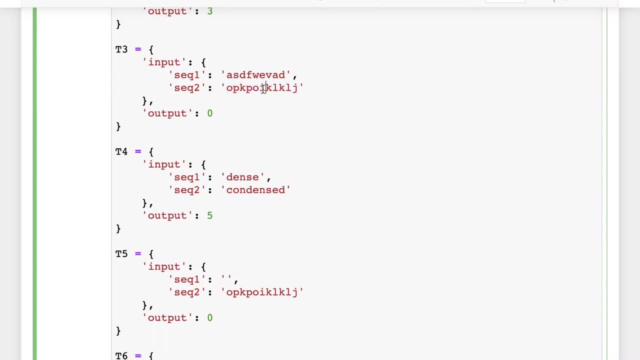 All of these come from the right half of the keyboard, So that was a quick way to generate these two sequences. Then here we have dense and condensed, and you can see that dense is actually a piece inside condensed. So this is a special case where dense is a continuous 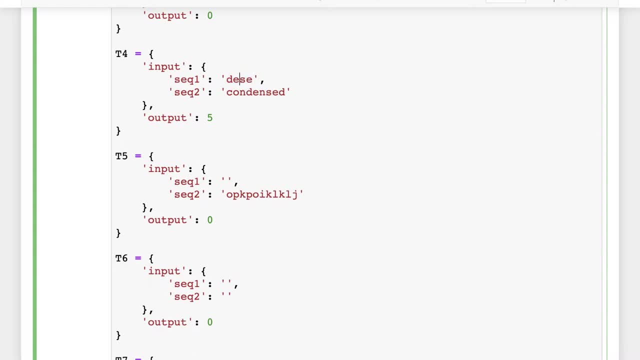 So this is a string of the string, but it, even if we had D E S E, that would still be a sub sequence because D E S E occur in this order. So that's one example, And in this case the sequence one is itself the longest common sub sequence and it has length five. 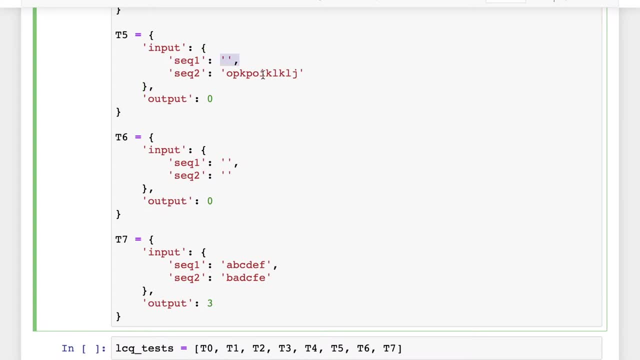 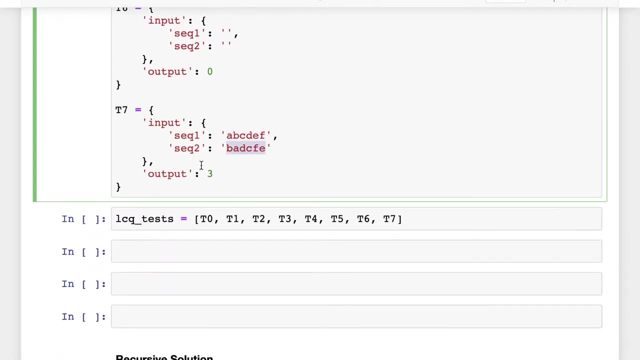 Then we have this case where one of the sequences is empty And you can see, in that case the output should be zero and both sequences are empty. And here is the case where you can have multiple longest common Sequences And even in this case your function should be able to figure out the answer correctly. 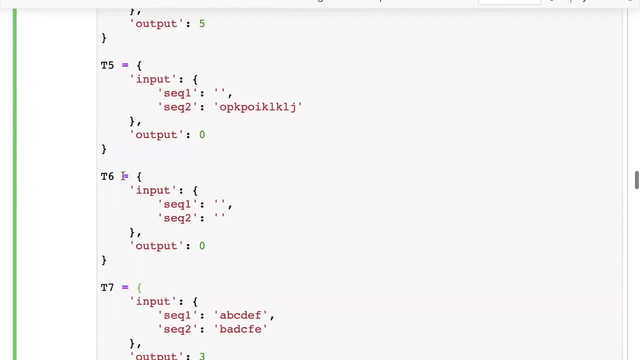 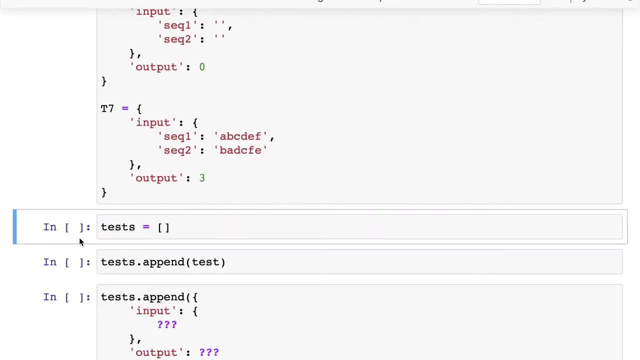 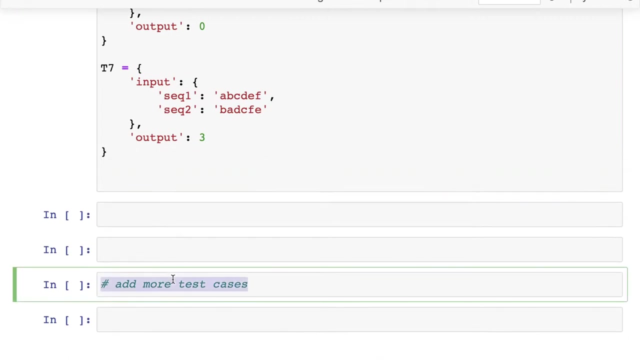 So let's take this and let us copy over these test cases here. So we have T zero to P seven, So that's eight test cases, And you can add more test cases here. Please feel free. coming up with good test cases is a skill that you should develop. 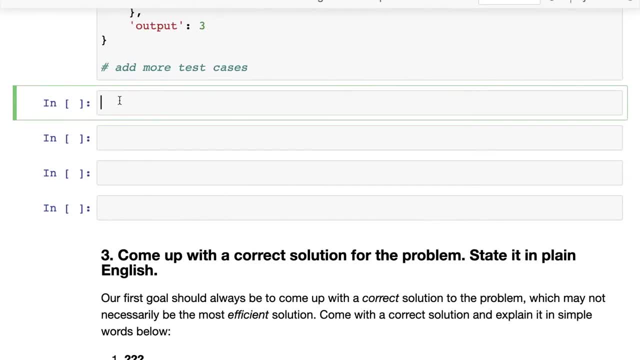 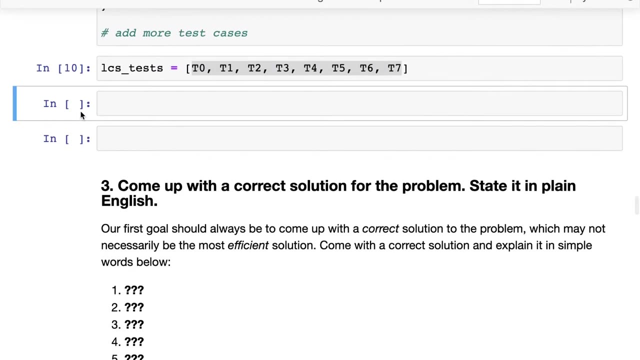 And what we'll do is we'll also Put all these test cases into this function called LCS or longest common subsequent tests, So that we have all of them easily available for testing at once. Okay, Okay. Now next step is to come up with a correct solution for the problem. 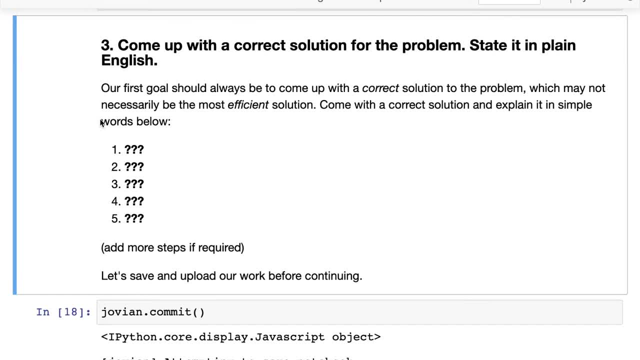 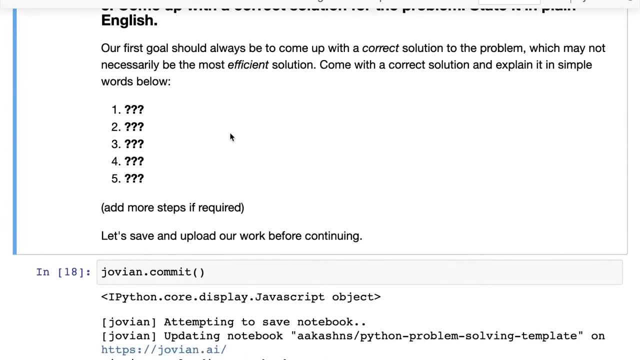 Now we've seen the problem, We have identified some scenarios. Now we need to come up with a simple, correct solution and stated in plain English. It doesn't have to be efficient, It just has to be correct. So here's one idea. 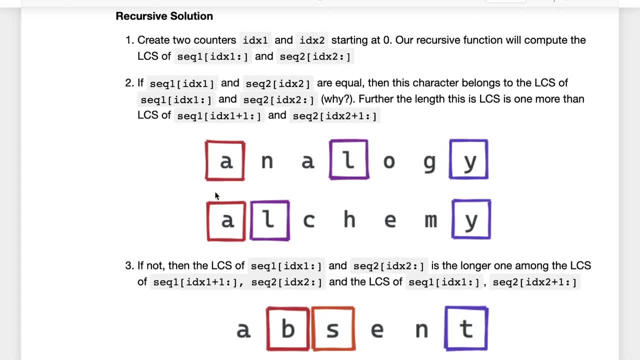 Here's one idea. Here you can see we have a couple of sequences. Let's create two counters, IDX one and IDX two, both starting at zero. So IDX will be a pointer which will start tracking elements, or in the first sequence. 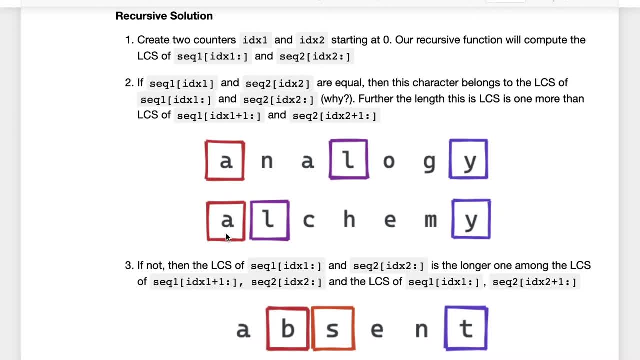 and IDX two will be a pointer: IDX. IDX will start tracking elements in the second sequence And what we do is we will write a recursive function. So we'll write a recursive function which will compute the LCS of sequence one from IDX to the IDX, one to the end and sequence two from IDX, two to the end. 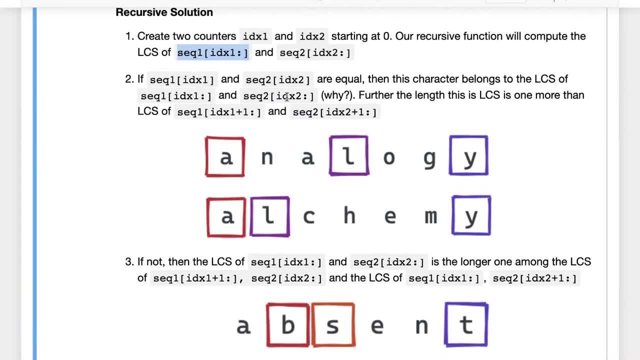 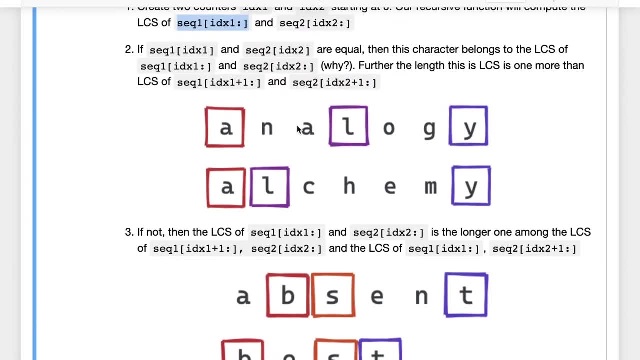 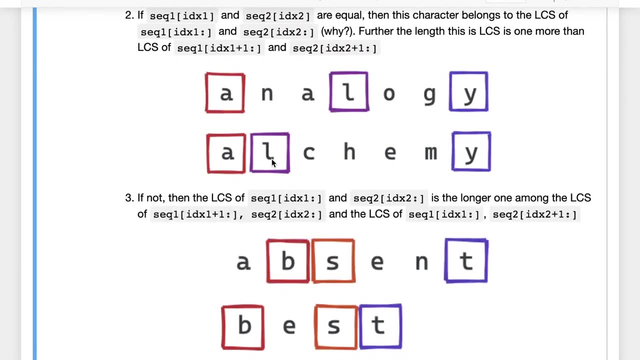 So what does that mean? Uh, let's say IDX one has the value three and IDX two has the value one. So you can see zero, one, two, three. So sequence one, IDX one onwards is L, O, G, Y and sequence two, IDX, uh, IDX. 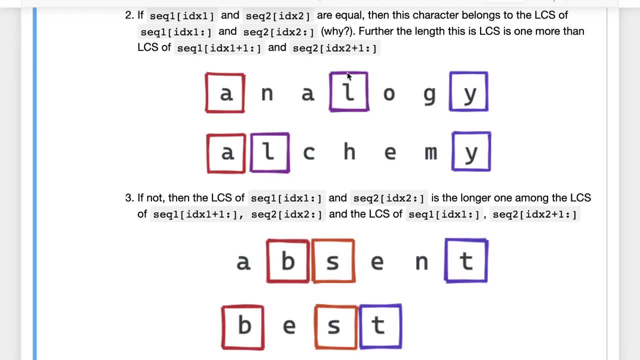 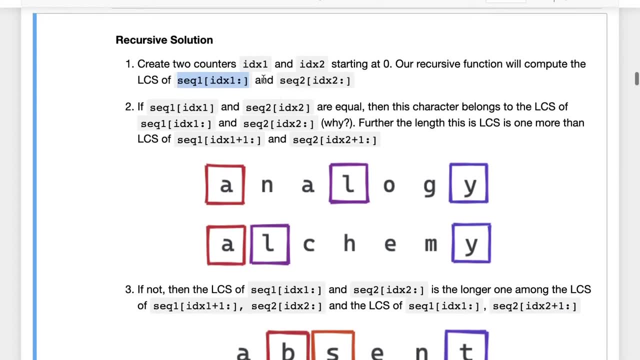 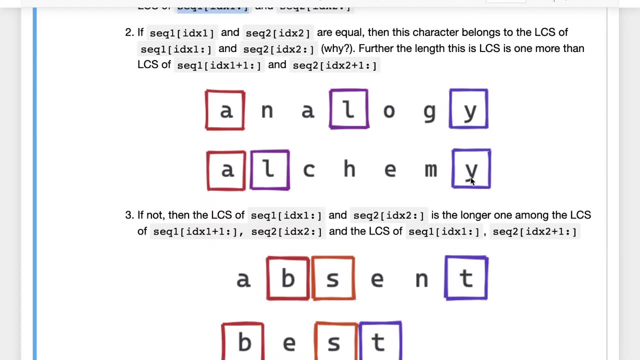 two onwards is L, C, H, M, E, M Y. So we're looking at this portion of the problem and this portion of the problem and a recursive function, when invoked with IDX one and IDX two, should return the length of the longest common subsequence Between. 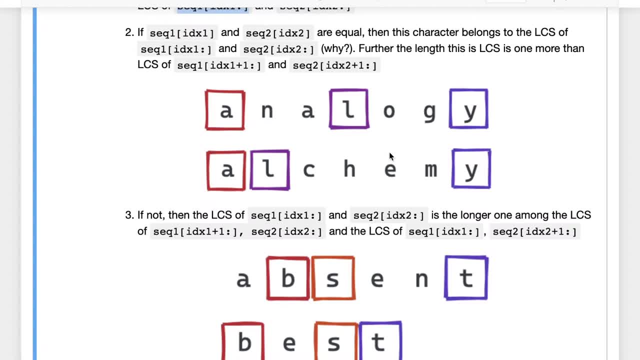 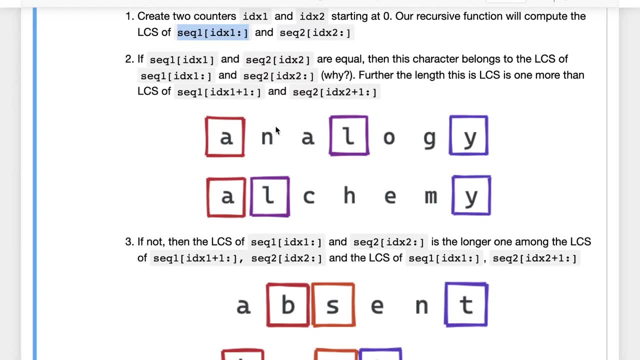 These two portions, So L O G Y and L C H E M Y. Now, why are we doing this? We need this longest common subsequence for the entire string, Don't we? Now here's the logic Why: why we're writing this recursive function, which can theoretically compute: 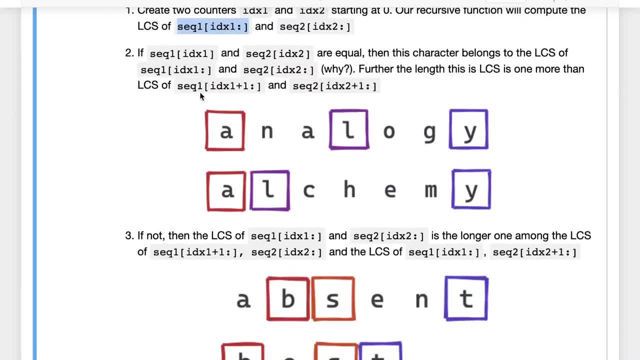 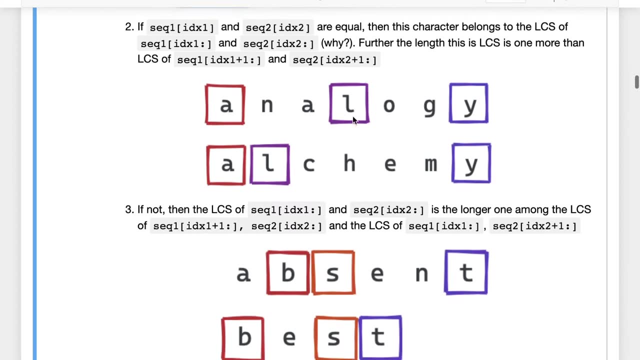 this subsequence for from any position onwards. So here's how we do this: If sequence one of IDX one, So if IDX one was pointing to L And IDX two was pointing to L- here as well, If sequence one of IDX one and sequence two of IDX two are equal, then this: 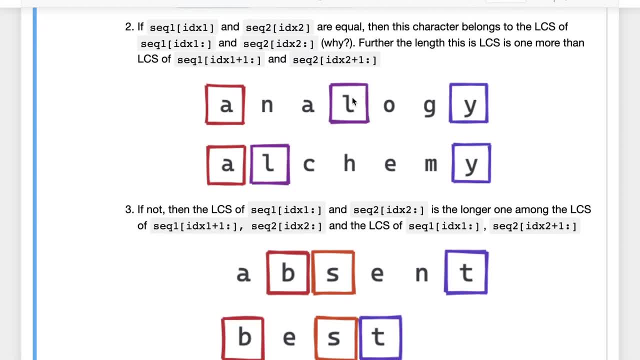 character L belongs to the LCS of this portion and this portion. Okay, Why think about it? It makes sense because these, these elements are equal. So if you pick the longest common subsequence of this and you pick the longest common subsequence of the remaining, 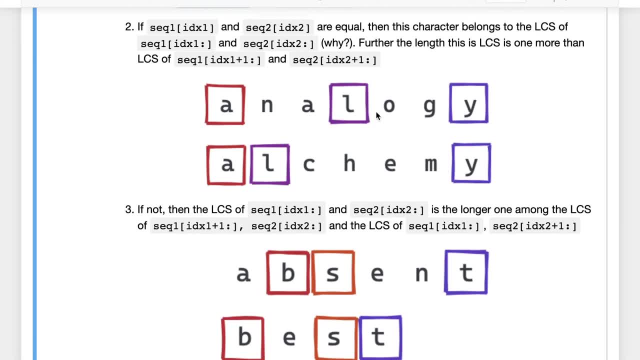 Then you can always add L to board to that subsequence and that will make the subsequence longer, right? And that way it follows that L will always occur in the longest common subsequence between L, O, G, Y and L C, H, E, M, Y. 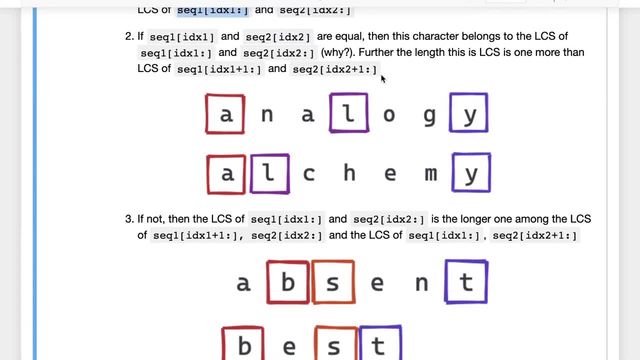 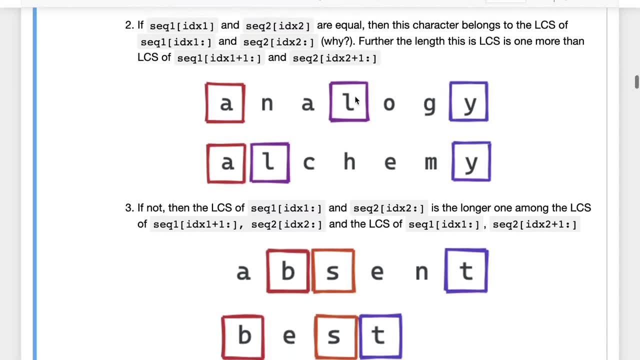 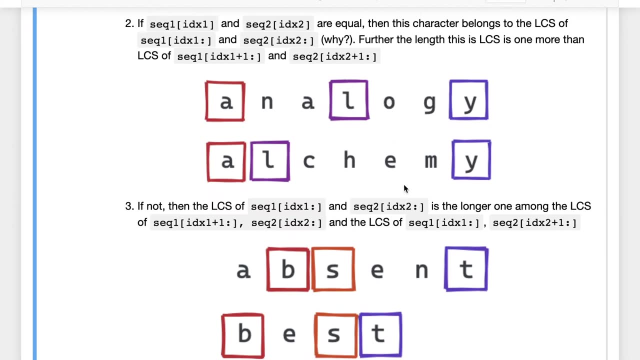 Okay, So we know now that this will occur. L will occur in the longest common subsequence. Further, the length of this longest, the length of this longest common subsequence will be the length of the longest common subsequence Subsequence between O, G, Y and C, H, E, M, Y plus one. 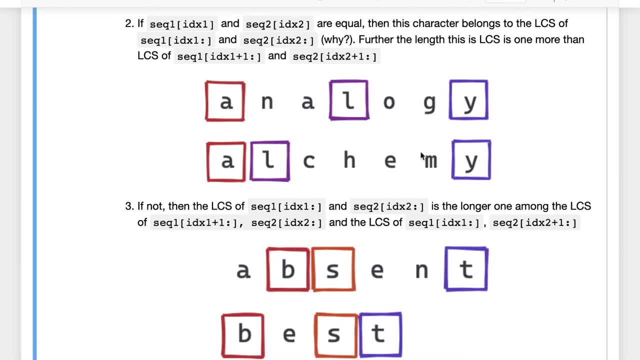 Okay, And now you can see why a recursion is required. because what we can now do is we can say that if sequence one of IDX one and sequence two of IDX two are equal, then we simply call the recursive function on sequence one of IDX one plus one. 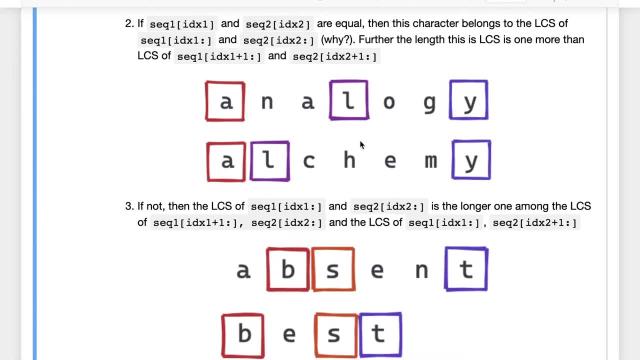 So O, G, Y and sequence two of IDX two plus one C, H, E, M, Y, and assume that recursion will give us the solution there And simply add one to it because this is equal. Okay, So that's one case If sequence one of IDX one and sequence one of IDX two are equal. 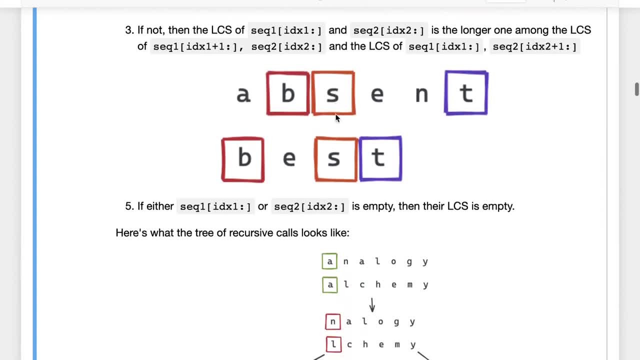 Great, But if they're not equal, right. So for in this case, for instance, you can see that if IDX one and IDX two are both zero, So IDX one points to E and IDX two points to B. So if they're not equal, then one of the two things should hold. either a does not. 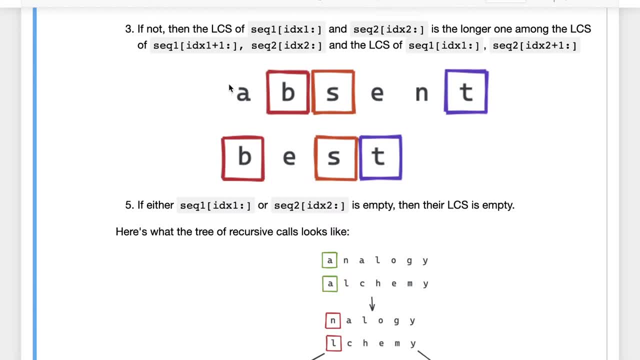 occur in the longest common sub subsequence between the two strings, or B does not occur in the longest common subsequence between two strings. Now we don't know which one, but that's the power of recursion, that we can just try both. So we can simply ignore A and we can get the longest common subsequence between B, S, E, N, T. 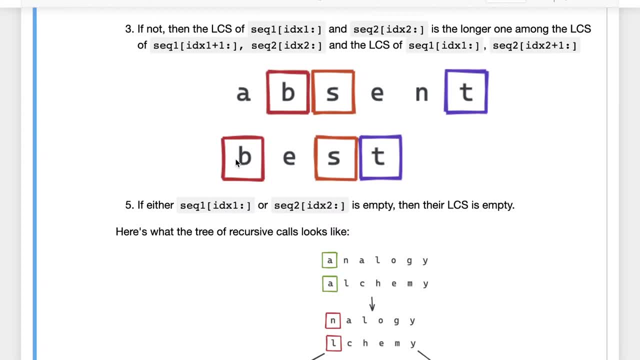 and B, E S T and check its length. And then we or we can simply ignore B and we can get the longest common subsequence between A, B, S, E, N T and E S T And check the length. Now, whichever is longer in length, that becomes the solution for the two strings. 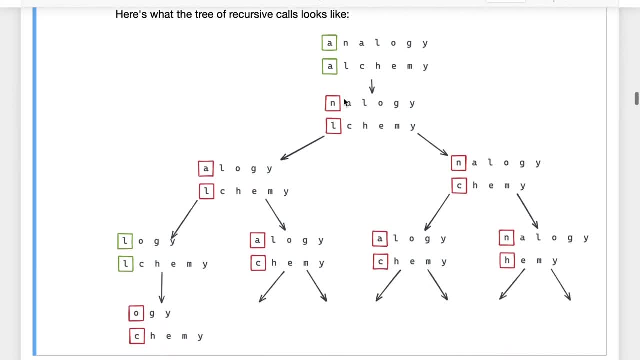 Okay, So this is what it looks like. We start out with analogy and alchemy. We compare A and A. these two are equal, So we know that the longest common subsequence is one. The length is one plus LC, LCS of analogy and alchemy. 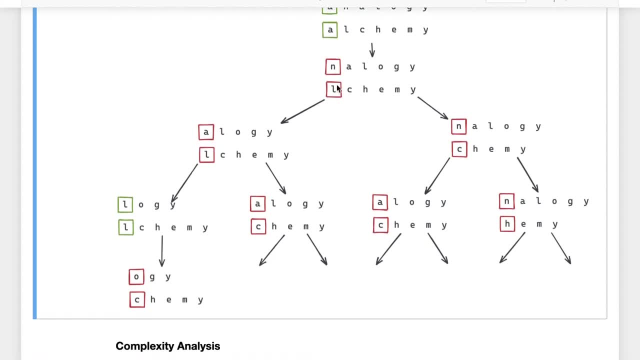 Okay, Now we compare N and L, and now we see that they're not equal. So either N does not come in the longest common subsequence or L does not come in the longest common subsequence. So we try both. We remove N here. 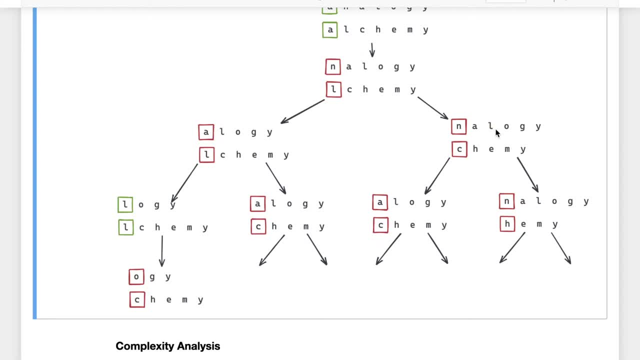 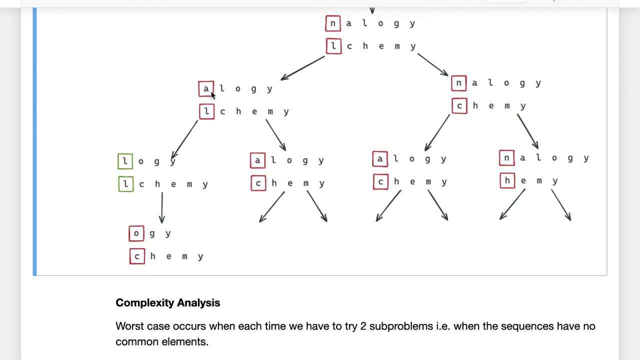 You see a L O G Y and we remove L here. We see C H E M Y. Now, once again, A and L are unequal. So either A does not occur in the LCS of these two strings or L does not occur in the LCS of these two strings. 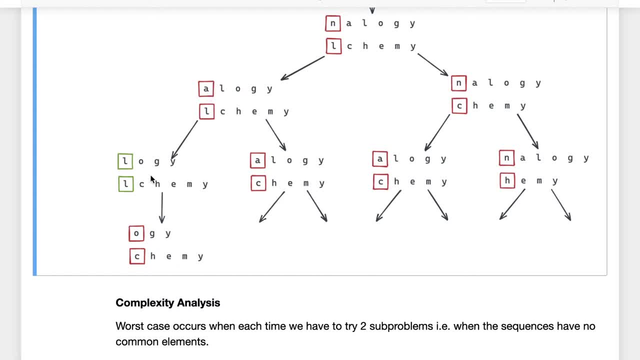 So if it doesn't occur in the LCS, we can remove A and try again. If L does not occur in the LCS, we can remove L and try again, And here once again we get a match. So in this case we know that L occurs in the longest common subsequence of these two elements. 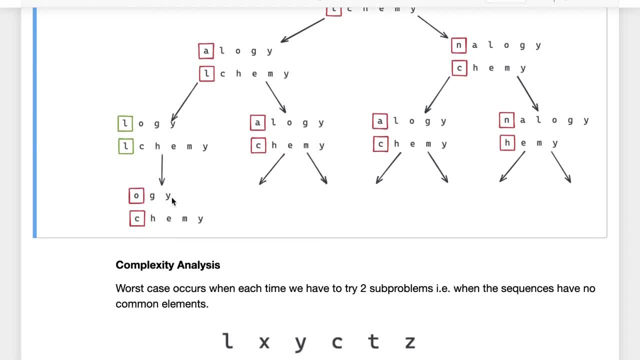 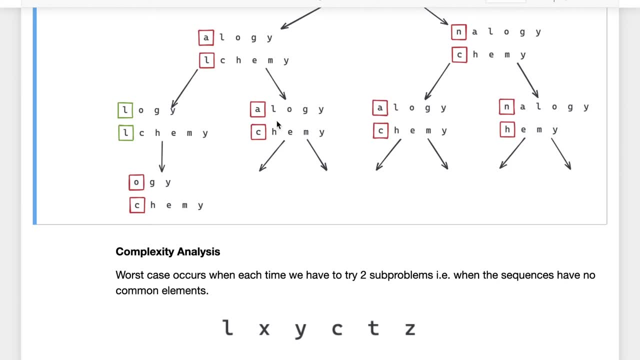 So now we can get the LCS of O, G, Y and C, H, E, M, Y, Okay. And then, as these recursive calls complete, you can see that this entire tree pans out. You can see that each time you either get one child or you get two children. and if you go all the way down, and then you 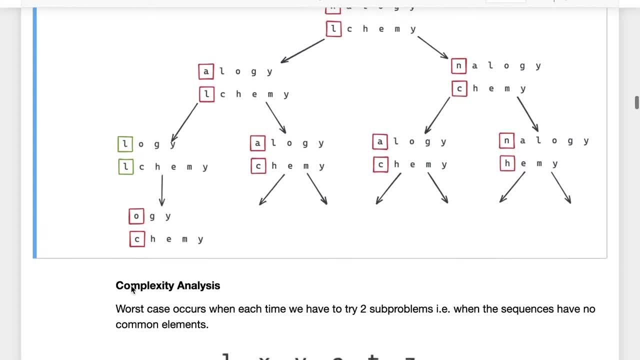 go back up and simply count the number of matches for each path you will key and you take, keep taking the maximum. So here you get back an answer. Let's say you get back an answer of size two. Here you get back an answer of size one. 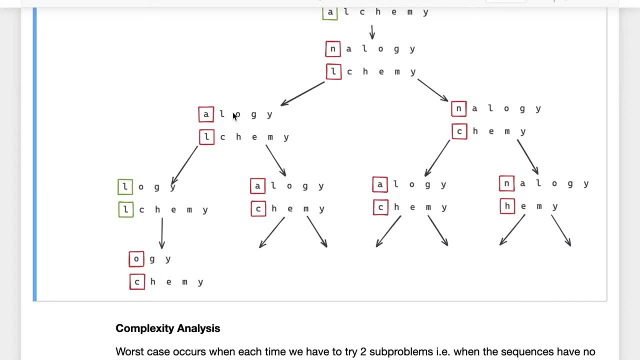 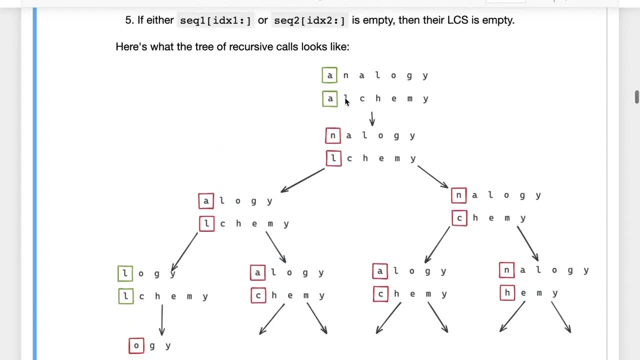 So the answer for this is simply the maximum of two and one which is two, And then the answer for this is simply the maximum of two, And let's say this is three, then three, And the answer for this is simply one plus three, four. 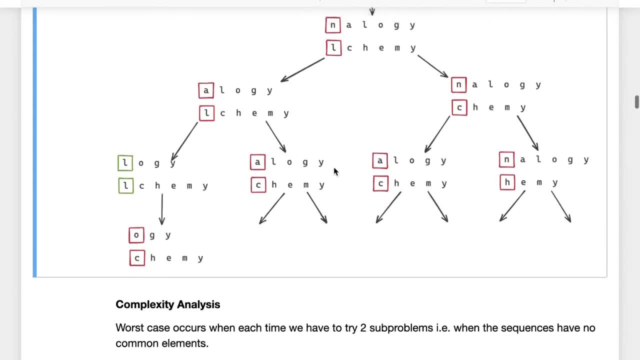 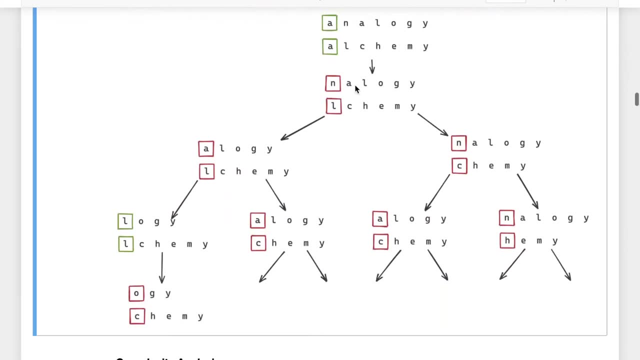 Okay, So this is the way that we will build up the solution. So we've Now looked at the recursive solution expressed in text And we've looked at the recursive solution expressed as a tree. Now it's possible that it still may not make sense to you how exactly this is working. 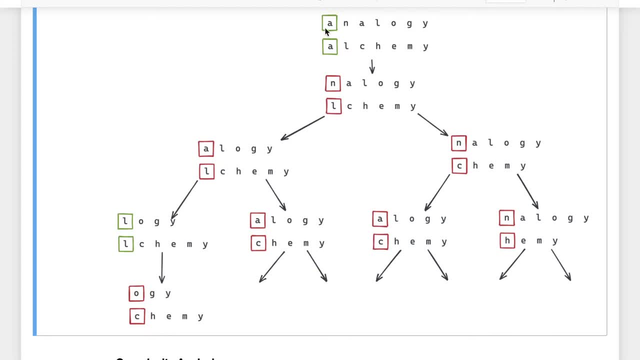 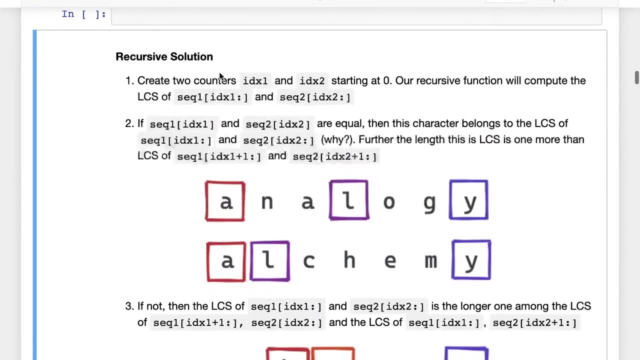 And that is where you should start trying to create this tree yourself. So pick up a pen and paper and then start drawing on pen and paper. Take an example and try to read each step here and try to work it out like a computer. Okay. 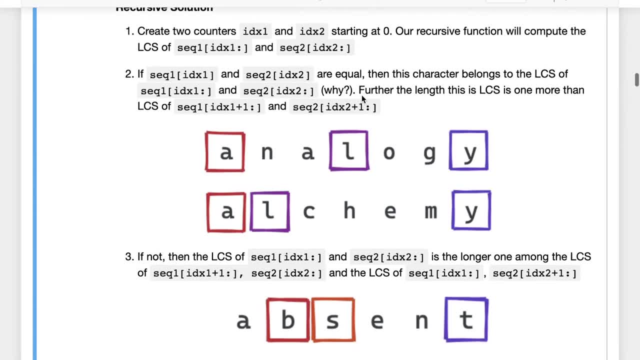 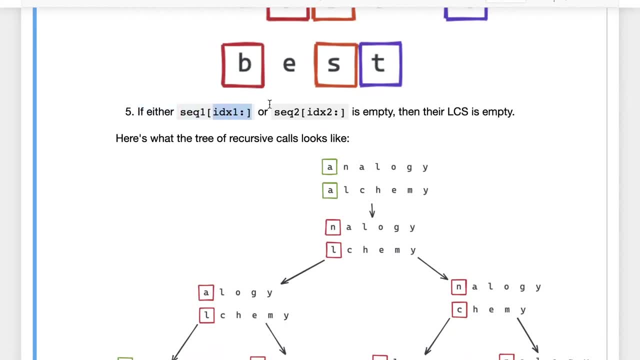 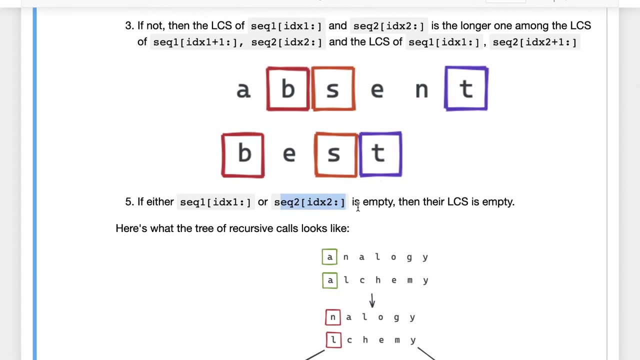 And just thinking about it. that way It will help you understand this algorithm. Now, one last thing is that if either of the sequence one from IDX onwards or sequence two from IDX onwards is empty, which means the index has reached the end point in after doing some recursion, then their LCS is empty. 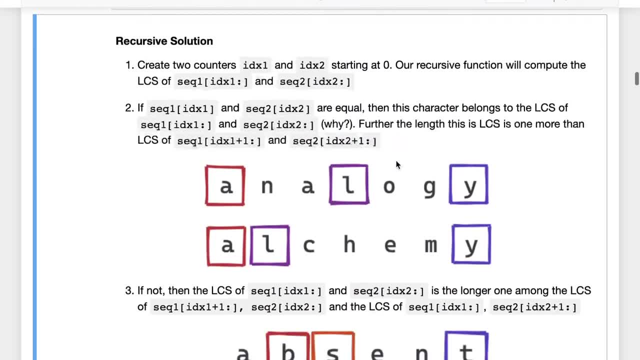 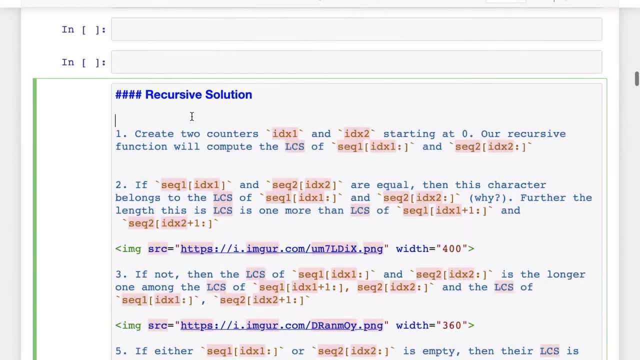 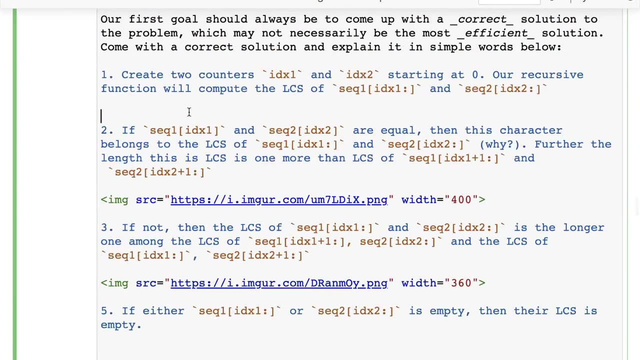 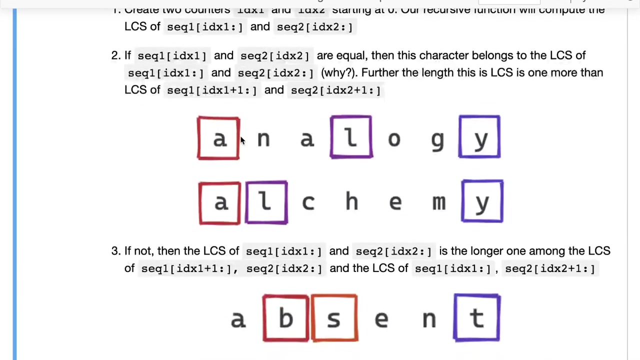 So the length is zero. Okay, So that is the recursive solution here. I will just copy over this recursive solution to, along with the entire tree. Now, obviously, in an interview you do not need to write all of this in in a lot of detail, or you do not need to. 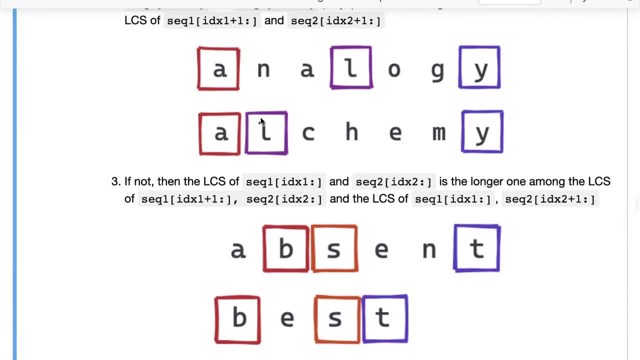 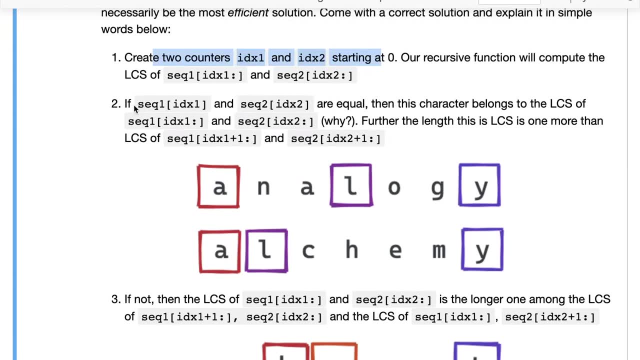 So it's helps to show diagrams sometimes, but you don't really need to do all of this. All you need to do is express yourself clearly that we will create two counters and the condition to check is whether these two elements had those counter positions are equal. 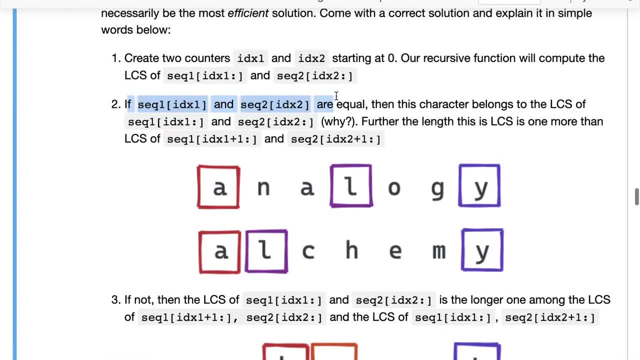 What do we do If they are equal? What do we do if they're in equal, and why are we using recursion here? So we are using recursion We can because we can use reuse some of the sub problems to compute the final problem. 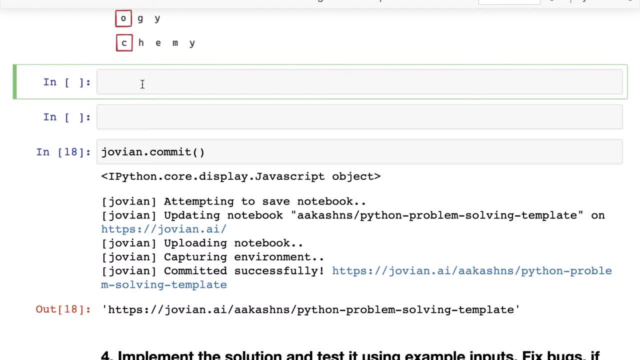 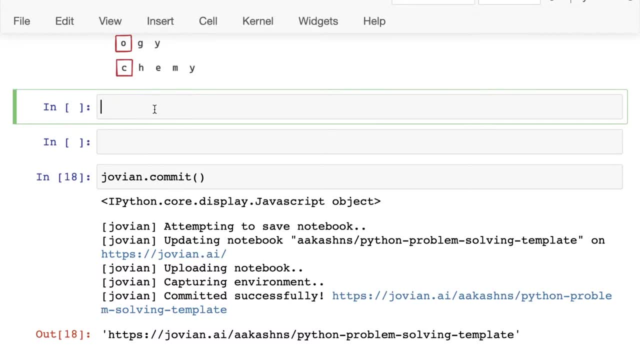 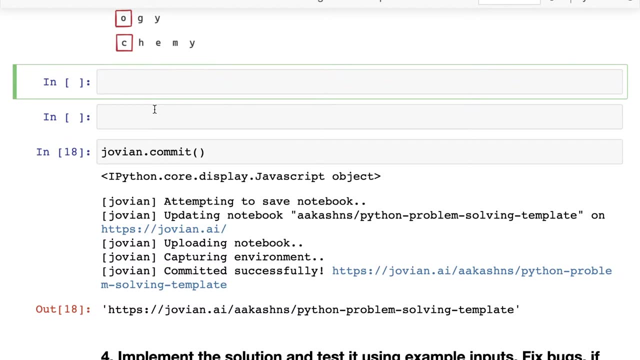 Okay, And understanding recursion is really important for solving data structures and algorithms from this, because it's like a superpower pretty much. pretty much every problem that you see one way or another can does boil down to recursion in one way. okay, so now let's save our work once again, and now. 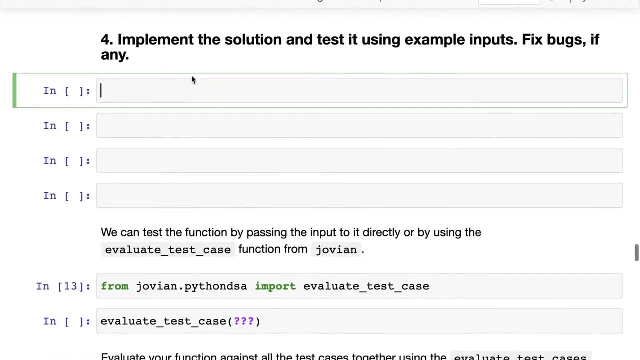 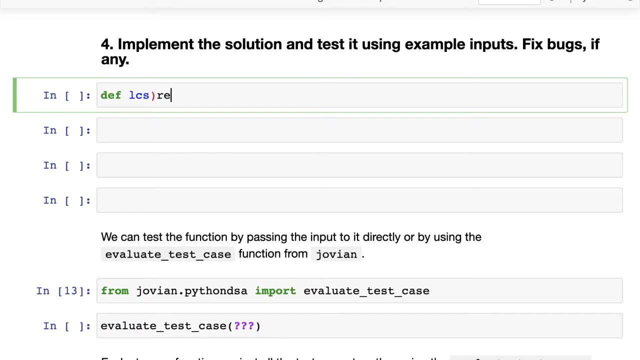 we're ready to implement the solution. So we have the recursive solution in front of us And if you remember the four steps, let's go. let's go ahead and implement it. So we see, let's just call it LCS- recursive, and this will accept a. 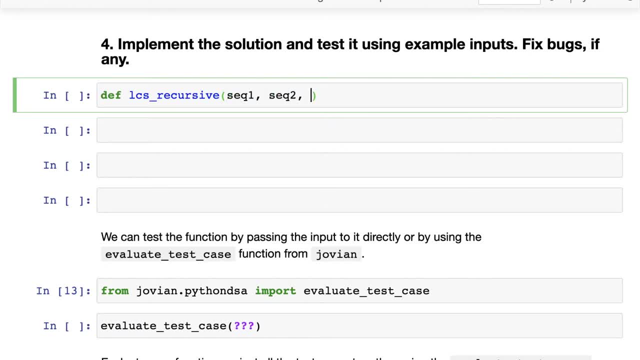 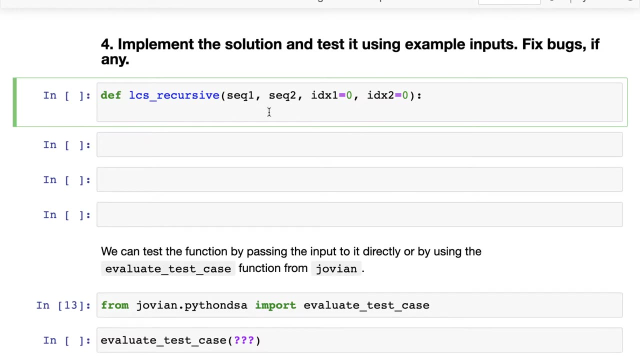 sequence one and a sequence two, And let's also initialize IDX one and IDX two, because we will be calling this function recursively. So we'll simply use these two counters, IDX one and IDX two, and set them to zero. Now the first thing we need is if IDX one is equal to the length of sequence. 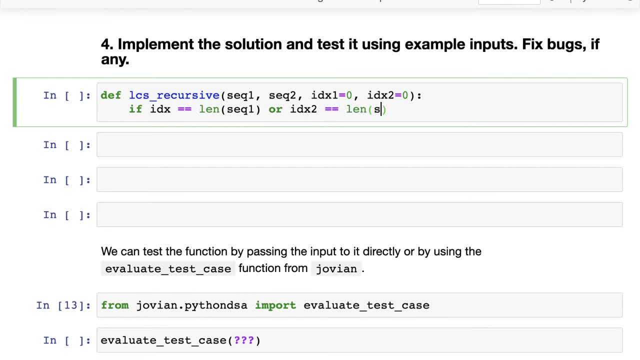 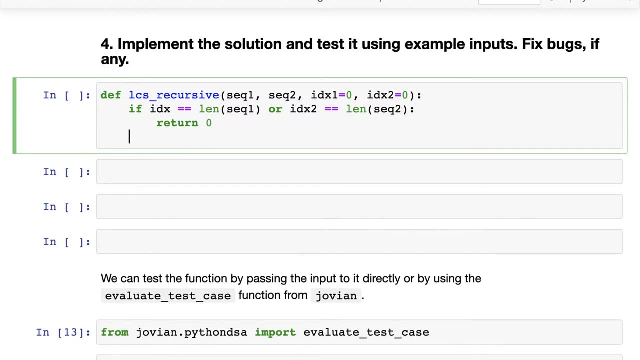 one or IDX two is equal to the length of sequence two. then we return zero Again. this is a common thing. that happens, that the base case or the end scenario is something when you're describing the algorithm, you will describe at the very end. as you're drawing the tree, you will notice. 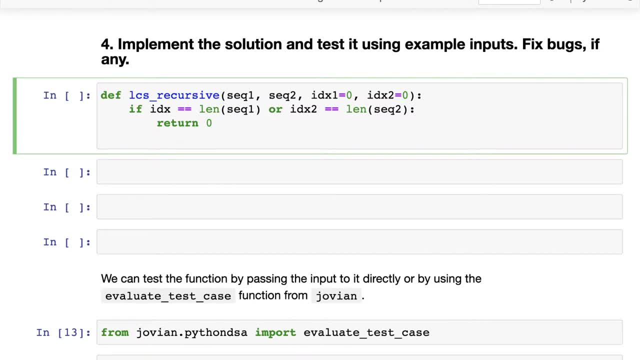 what the end case and scenario is. But when you're coding the algorithm, the end scenario or the base case comes at the very top, because otherwise we'll try and access IDX one from sequence one And that will throw an error. So that's why you need to handle the base case at the very beginning. 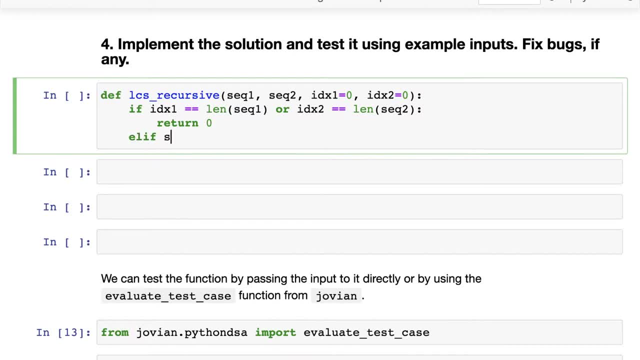 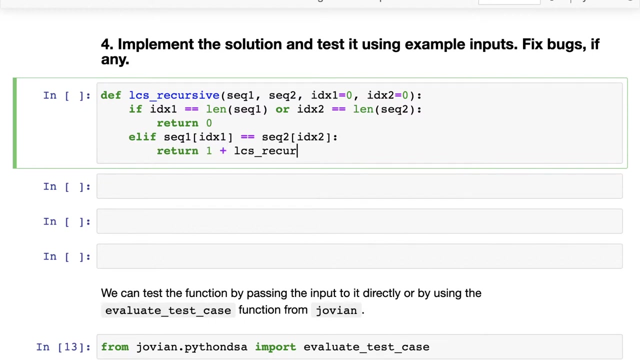 Okay, Next, moving ahead, if sequence one of IDX one equals Sequence two of IDX two, great, we found a match. but we simply return one plus. now we can call LCS recursive on sequence one, sequence two and we increment IDX one by one. 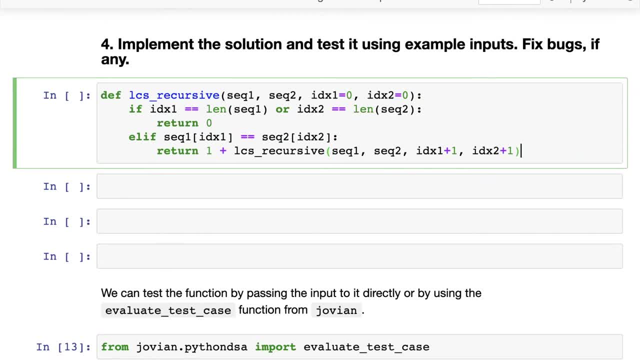 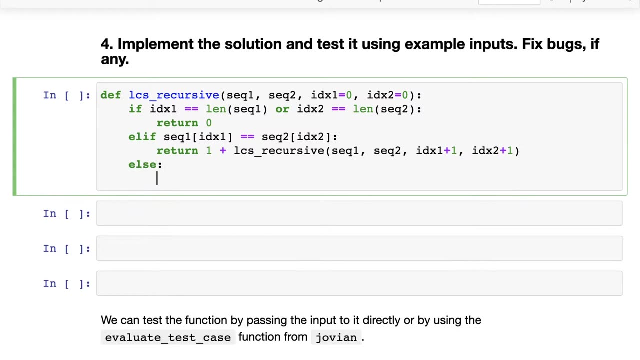 And we also increment IDX two by one. Both of these need to be incremented, Okay, Because we are going to use this element, this common element, as an element in the sub sequence. Okay, So there's just one recursive call here. That was nice. 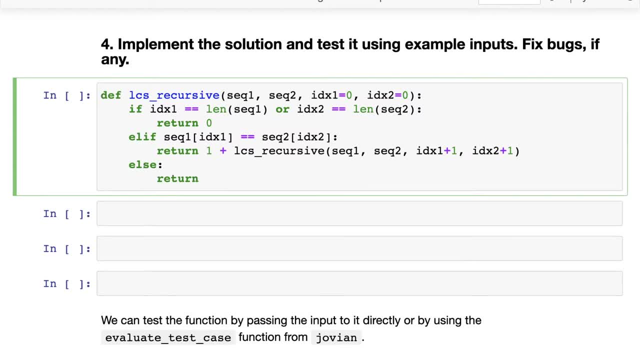 Otherwise we have to either ignore the first element of, or the current element from sequence one, or the colored current element from sequence two. So we have two options. So we have option one, which is we ignore the current element of sequence one. So this becomes LCS recursive sequence one, sequence to IDX one plus one and IDX two. 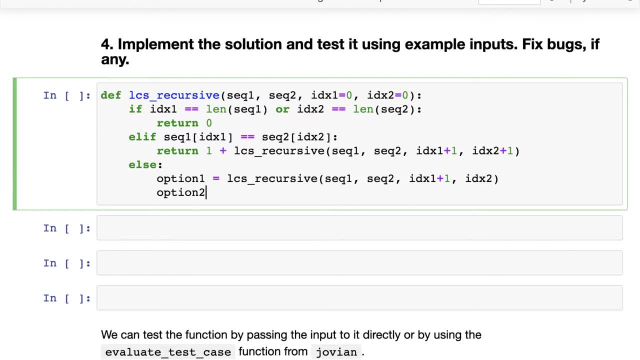 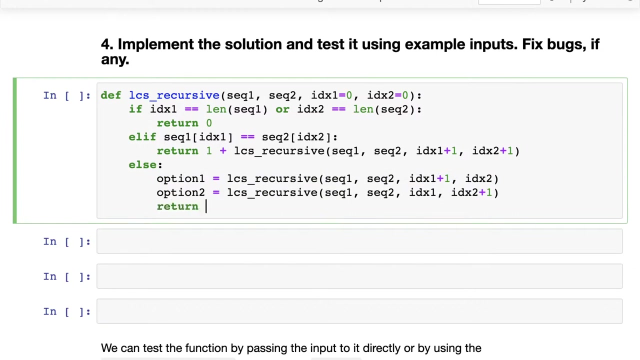 And then we have option two. this is LCS recursive. Once again, we sequence one and sequence two, and this time we increment IDX two. Okay, So make sure you understand this piece, because this is really the key here. And then the length of the longest common subsequence is simply the maximum of option one and option two. 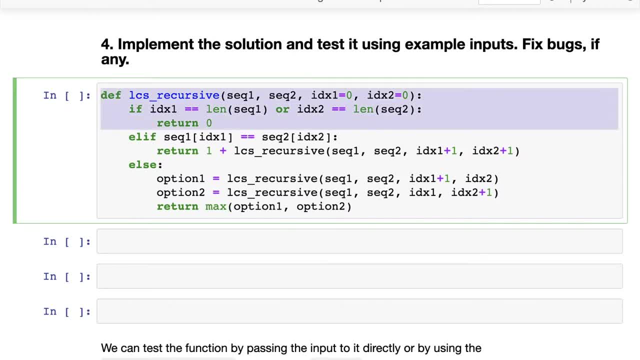 Okay, And that's it, What may have seemed like a fairly tricky problem Once you start thinking about it recursively. Okay, What happens if we simply compare the first two and they are equal and they're unequal. Okay, Now we need to solve the problem for the remaining um. either we add one or we take two. 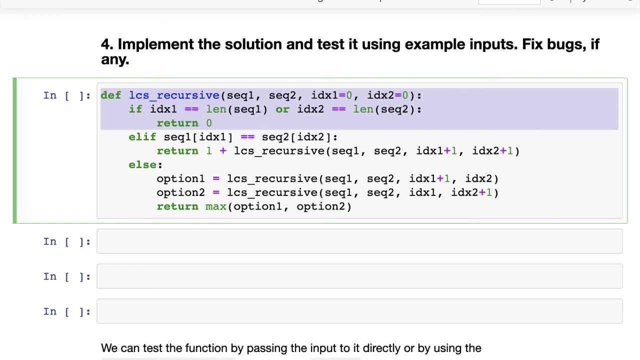 Or we ignore one of the elements right. Once you get that thought, the recursive thought, then the solution and the code simply presents itself to you. It's just about seven lines of code. Okay, That's our LCS recursive solution. Now let's test it out. 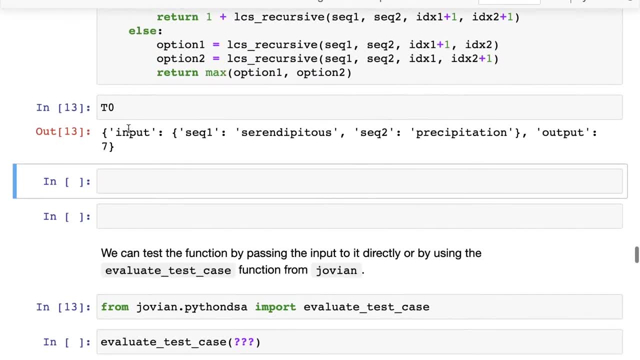 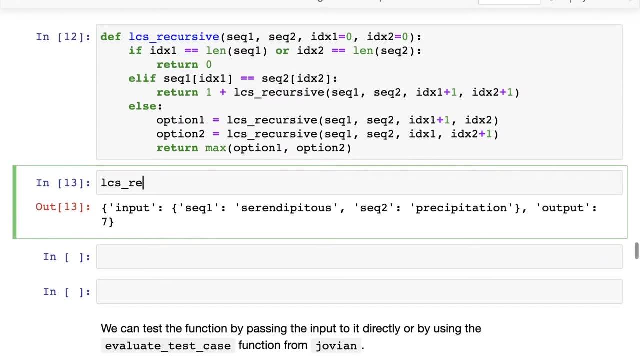 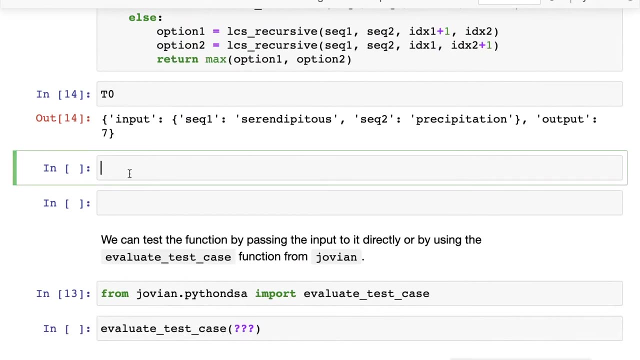 Let's look at a test case: D zero- Okay, So here we have serendipitous and precipitation as the inputs. Let's call LCS. Okay, So let's keep that around so that we can view it later. Let's cause: call LCS recursive on zero. but of course we need to fetch from T zero the input and uh, get sequence one out of the input. 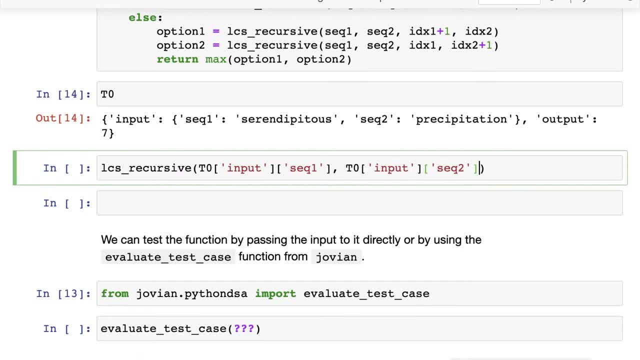 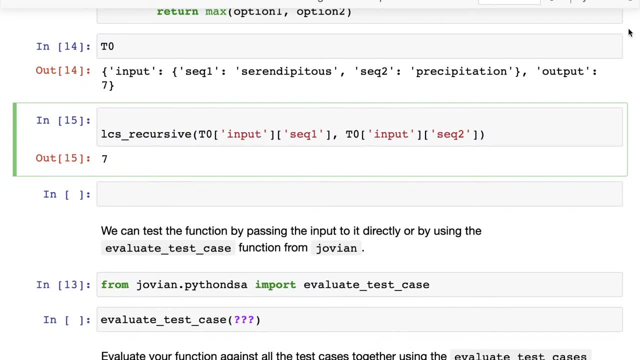 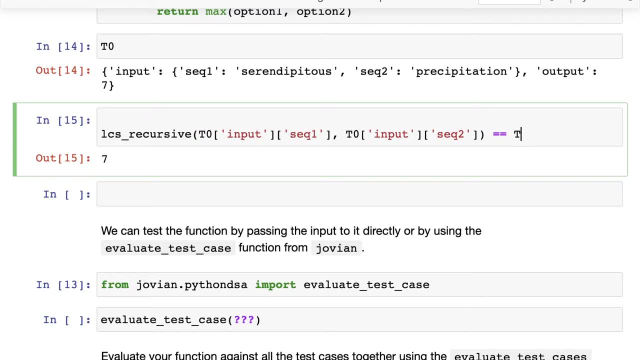 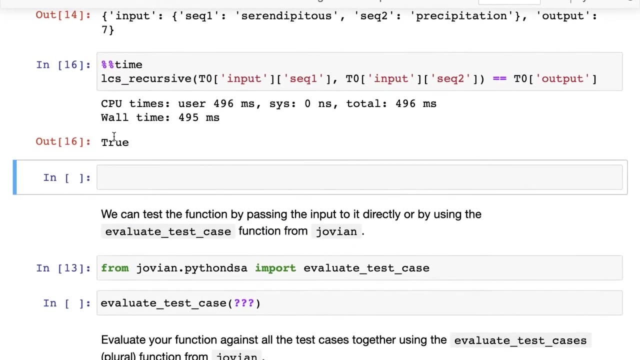 So if we simply put in here D, zero output- and I'm also going to put in this special command called percentage, percentage time- this is going to tell us how long the cell takes to execute. Yeah, So now you can see here that we get back through and sell. it takes 490.. 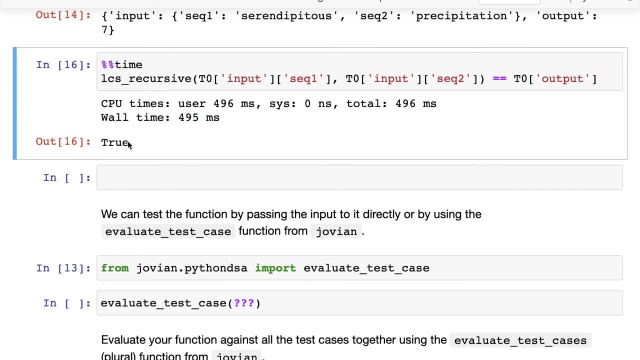 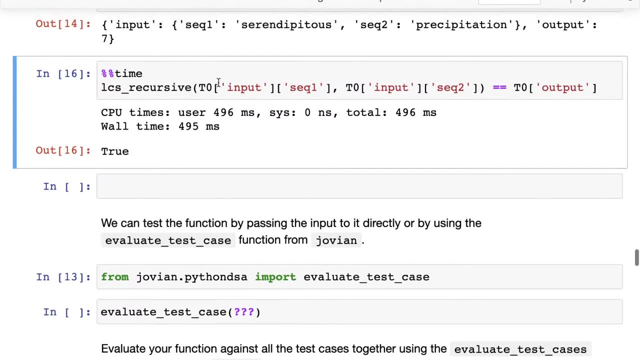 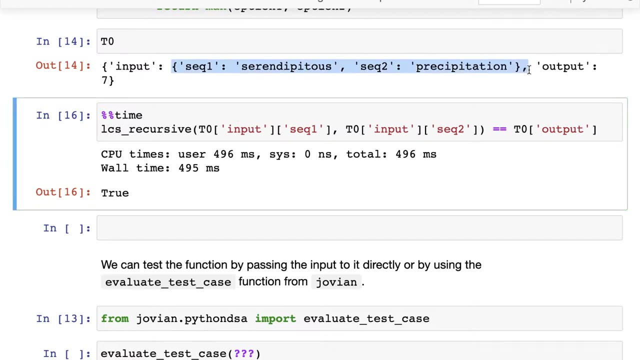 95 seconds or half a second to execute, And that's it. So now we have tested this test case. One small thing I can tell you how to improve this slightly is because in E zero of input as a dictionary and because the names of the elements of the dictionary are sequence one and sequence two, which also match the argument names of LCS recursive. 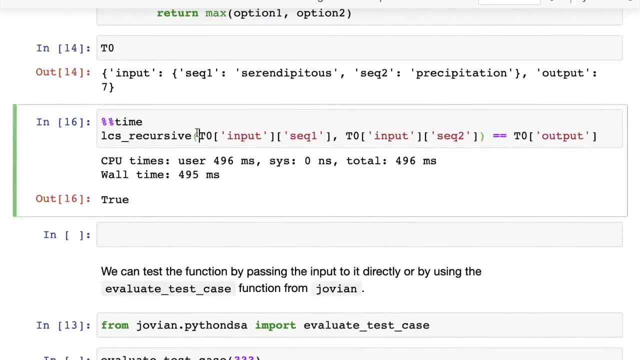 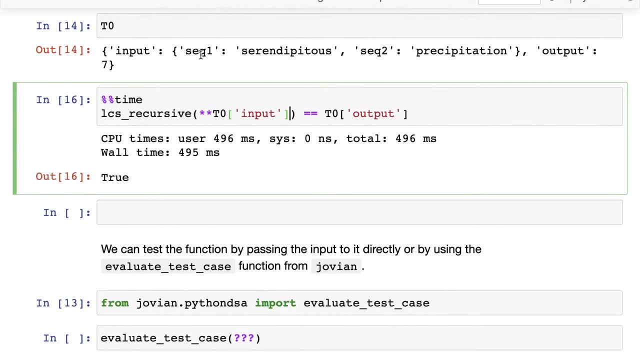 You can see, here we have sequence one and sequence two. What you can do is you can simply Say star, star, T, zero input, and Python will automatically grab each key. So sequence one will be passed as the argument. sequence one- and sequence two will be passed as the argument. sequence two. 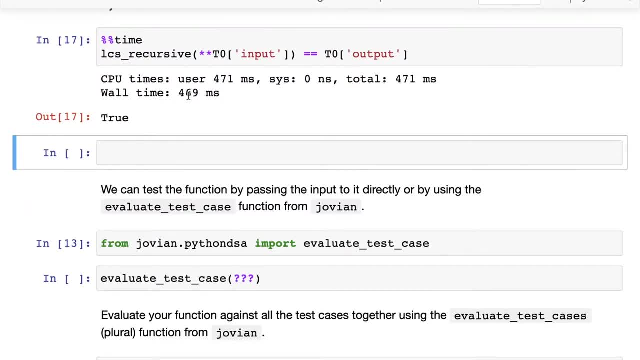 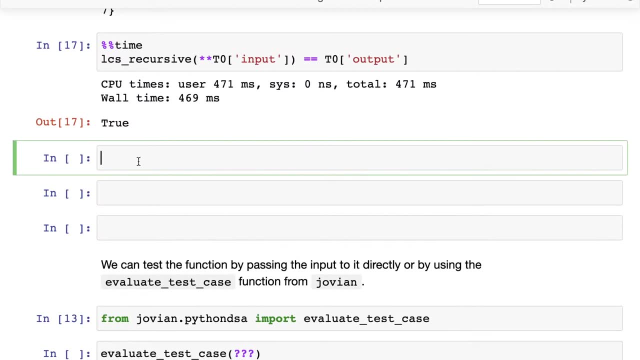 That's. this is a small trick here that helps us speed up the reduce the amount of code we need to write. Okay, Now we've tested one test case, but that's not enough. We should be testing all the test cases. to test all the cases we can write a for loop for. 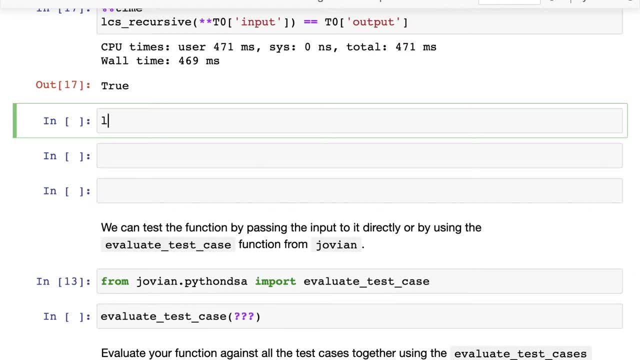 T in tests et cetera. but we can do something else too. We can use the evaluate test cases function from Jovian, So from Jovian, not Python DSA, the module. we will import: evaluate test cases. 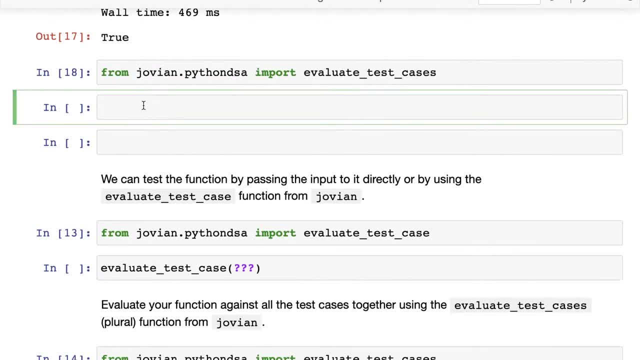 It's a helper function that we've created for you, but it's really simple to write. You can just use a for loop as well And we call evaluate best cases on the function that we want to test. Okay, So we have the test, which is LCS recursive, and the tests that we have, which is LCS tests. 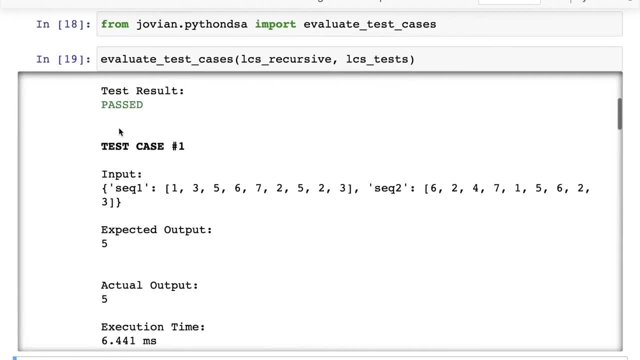 And when we do this, it is going to try out each test case. You can see it's tried test case zero, That was a pass. it tried test case one and it's also printing out the input, the expected output, in the actual output. 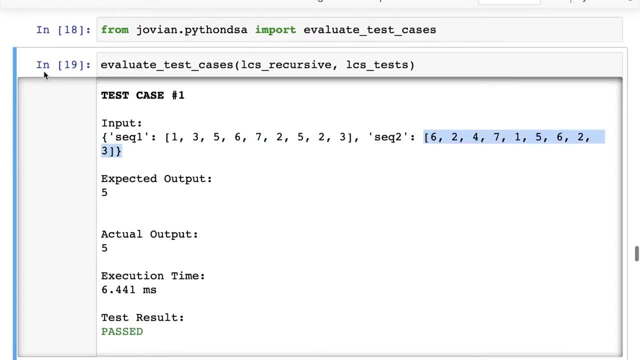 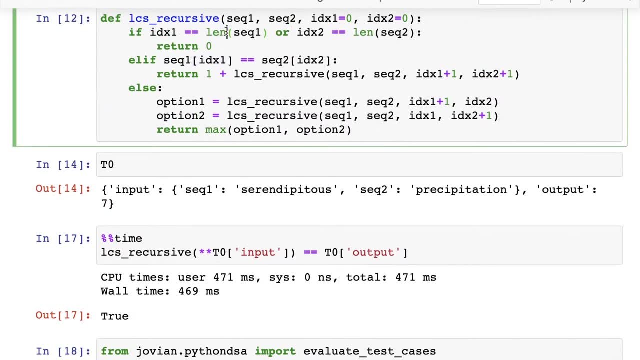 The test case one was lists, and lists work too, because all we've used here is indexing and length, And these are both things that are available. These are both things and lists, and this is something that's very nice about Python: the dynamic nature of the functions. 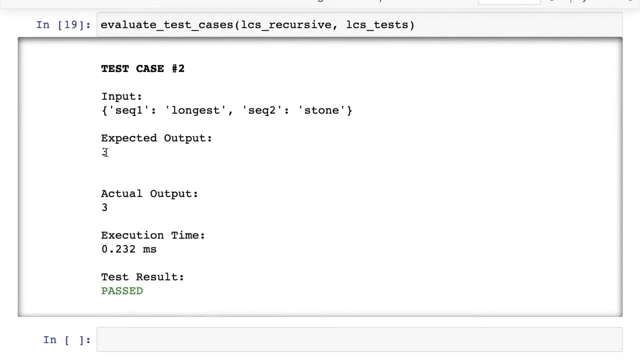 Oh, once again, this worked perfectly fine. And then here we have another one, longest in stone. The expected output was three and the actual output was three as well. Here we have ADS F, E, W, 80 and another string. They have nothing in common. 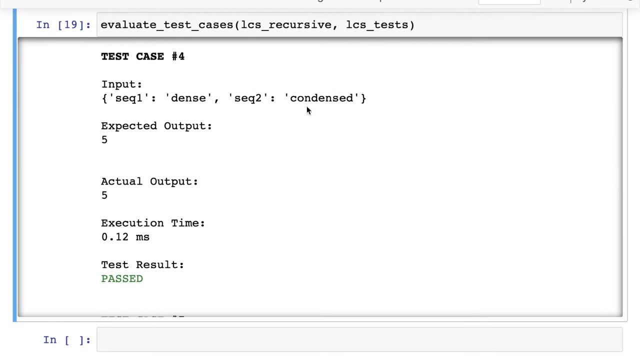 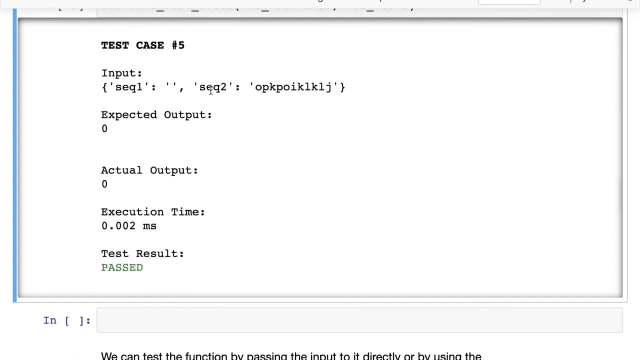 So the expected and actual output are both zero. Here's one where one is the is already a subsequent of another, So the smaller one becomes the longest common sub sequence, And then we have an empty string, and then we have two empty strings. 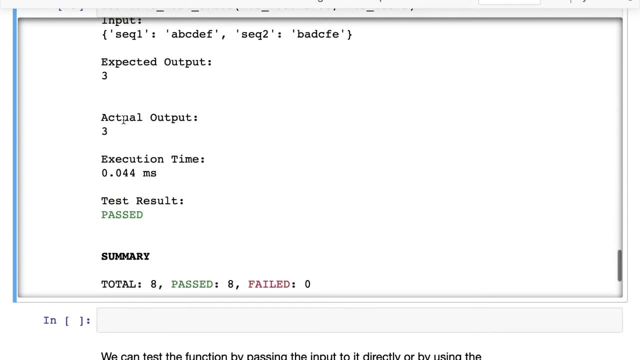 And, finally, we have multiple, longest common sub sequences. We still get back the right output. Now, if any of these field, you would know exactly what went wrong. For instance, if you had an issue in this case, where the two of these were empty, and that would tell you that you've. 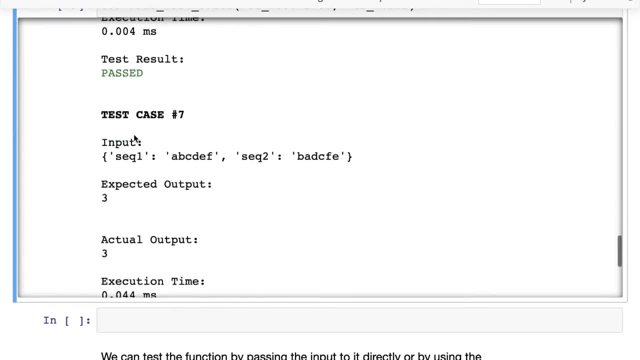 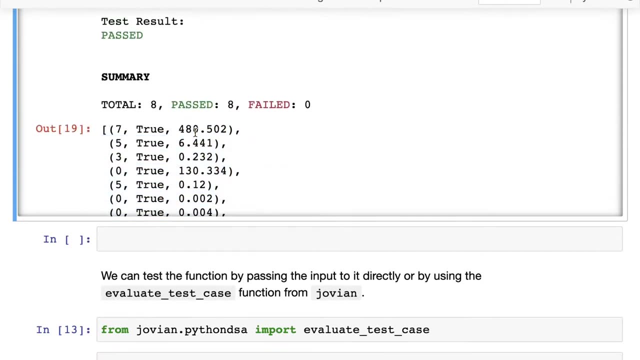 probably not handled that empty case properly, And that is why having great test cases is very important. Okay, And we can see the timing, So these as well. each of these took about, uh well, four 80 milliseconds was the highest. 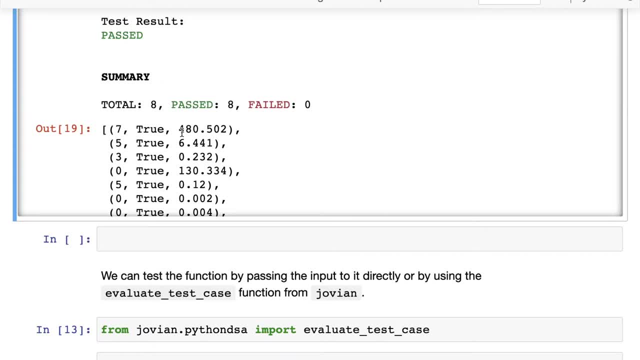 Now that's still a bit high. I would say the 480 milliseconds- because we are just looking at a sequence of serendipitous and precipitation, which are of very short length If you're looking at a really long sequence. for instance, this technique is used for DNA sequencing. 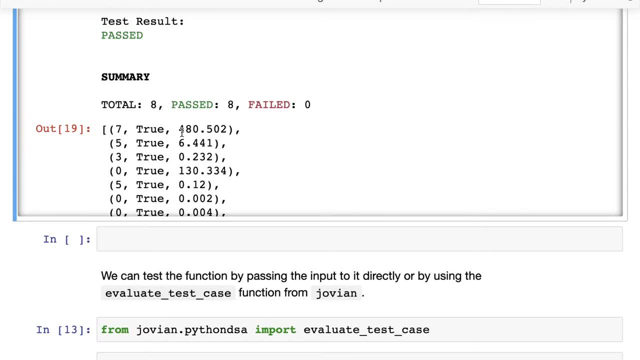 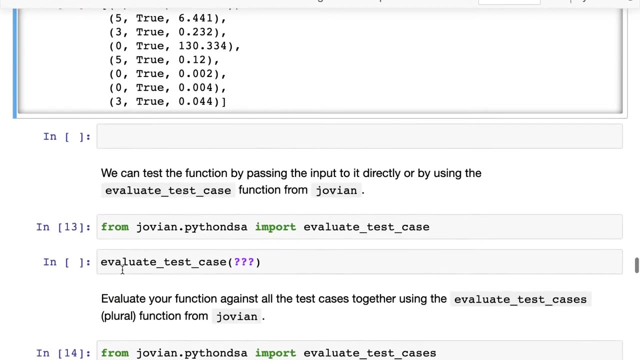 And we were looking at two DNA strands or two, doing two DNA strings and trying to get the common sub sequence out of them, And these can go into thousands, or sometimes millions of elements. That would Make it rather slow. Okay, So we do want to improve this algorithm further, but let's do that. 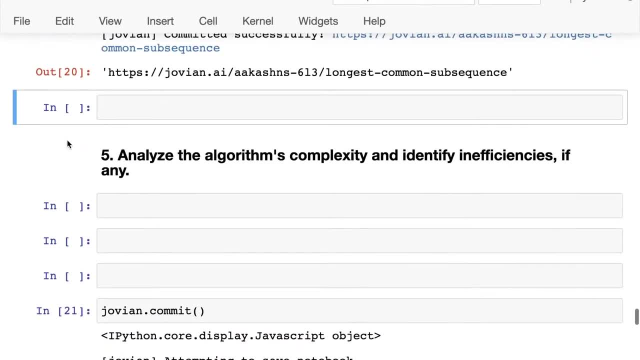 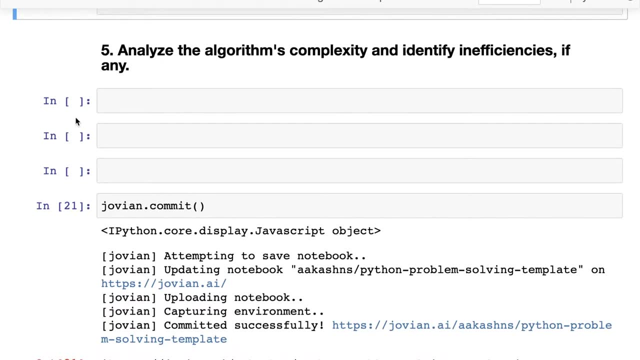 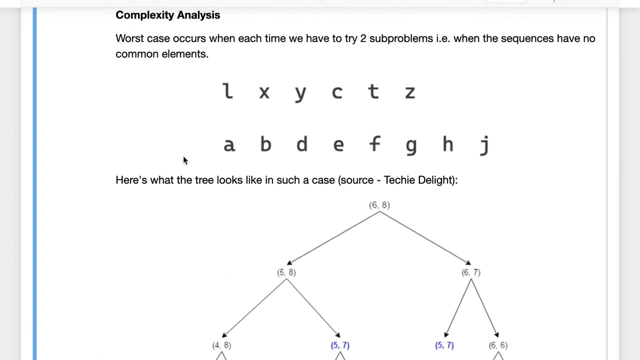 And before that we can just commit our work once again. Uh, but the first thing before we improve the algorithm is to analyze its complexity. How long does it really take? Okay And identify any inefficiencies? now to analyze the complexity, Let's look at an example and let's consider the worst case. 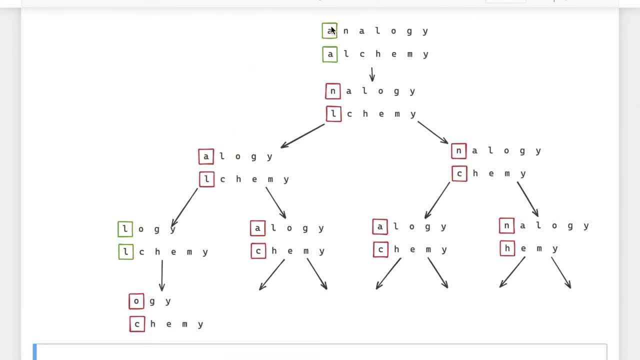 Now, when does the worst case occur Here? we've seen that if two elements match, then we simply have one sub problem or one recursive call. But if the two elements or two elements off the sequences don't match, then we have two recursive calls. 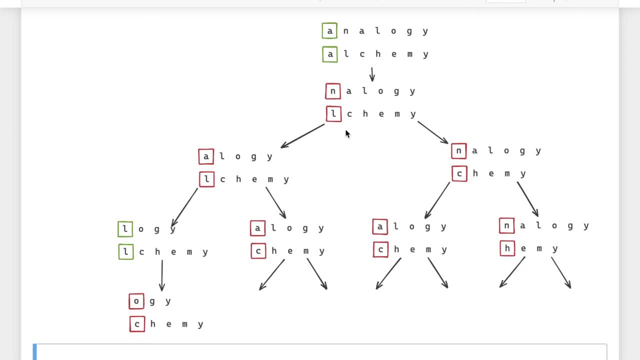 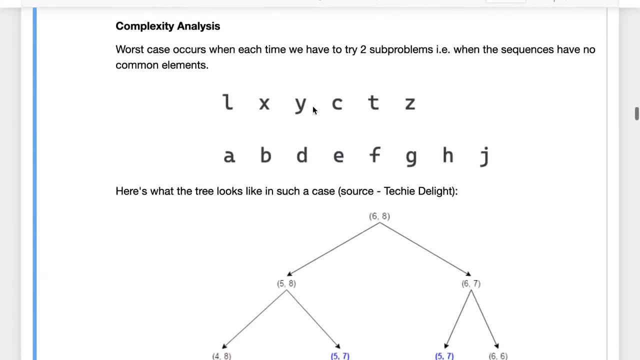 So if you have two completely distinct sequences where none of the sequences, none of the elements match, then each time we will end up with two sub problems, So that becomes the worst case. So the worst case occurs each time we have two sub problems where the sequences have no common elements. 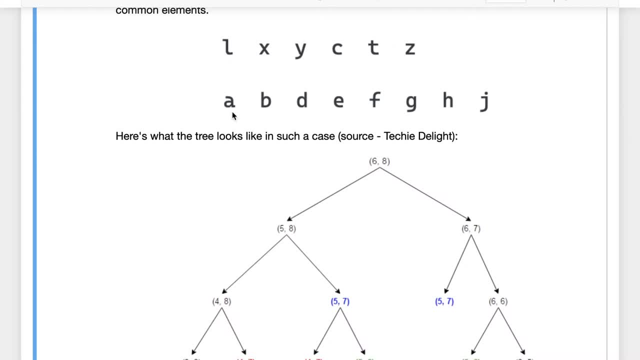 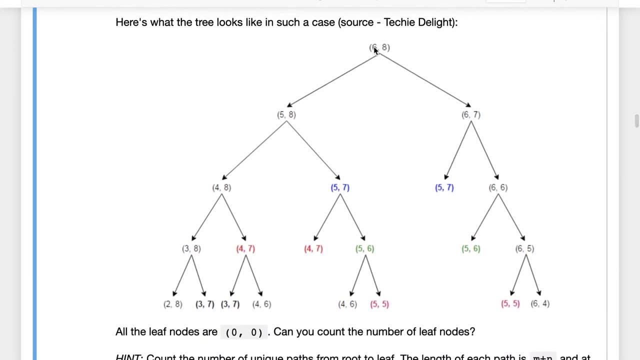 And here's an example. This is a sequence of length six. here's a sequence of length eight, and this is what the tree will look like. So now we have no longer put the actual sequences, We've simply put what is the length of the string that we started with. 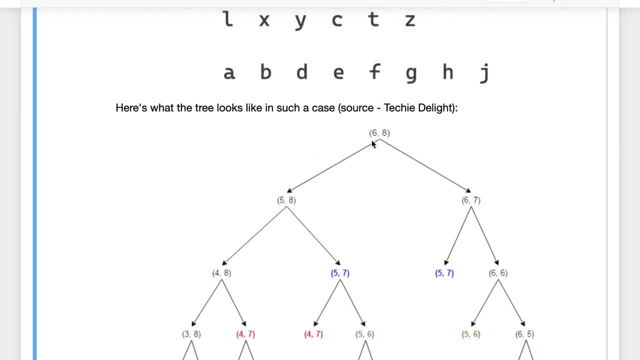 So here we started with strings of length six and eight, And then we say that we either ignore the first character of the first string or the first sequence, or we ignore the first element of the second sequence, And that gives us two sub problems. 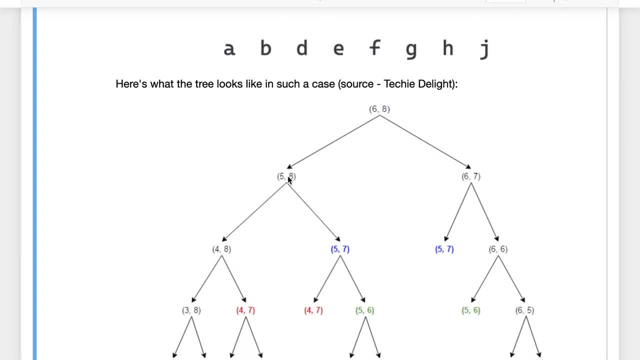 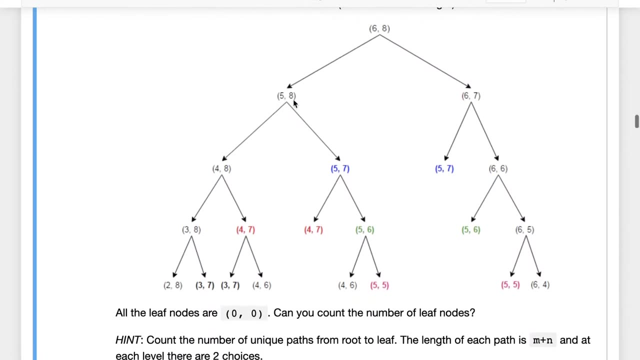 And this time the sequences have length: five and eight in this case, and six and seven In this case. okay, so we either reduce one from the left or we reduce one from the right. And once again here, we either reduce one from the left or we reduce one from the right. 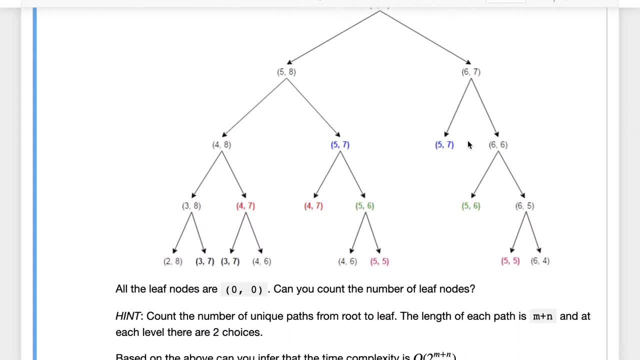 So this way we create a tree, and you can also see that a lot of common trees get created, and that really is what is the inefficiency, And we'll talk about that. but what will happen here is five- seven. we'll then call four, seven and five, six and five, seven here. 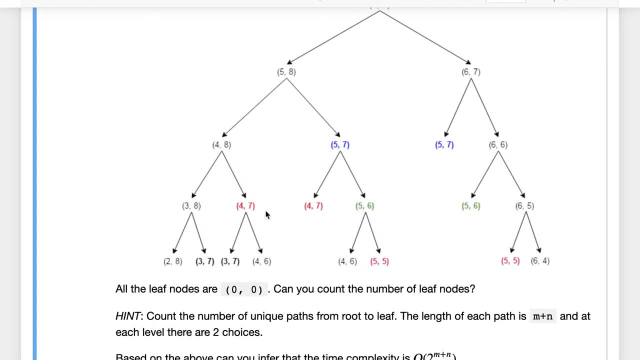 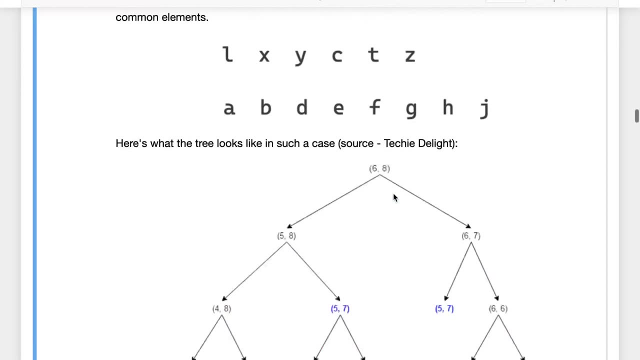 We'll once again call four- seven and five six, and four- seven and four- seven will get repeated here in five- six and five- six will get repeated here Three times here. So there's a lot of repeated calls that are going to occur. 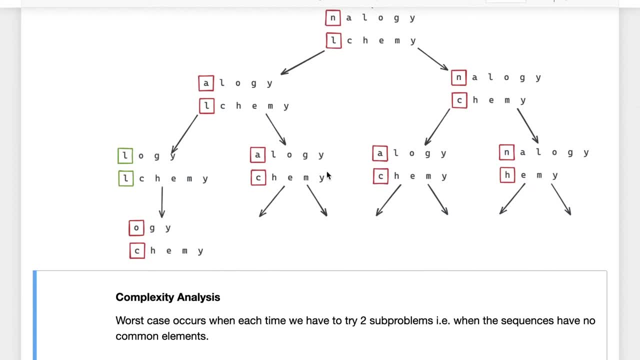 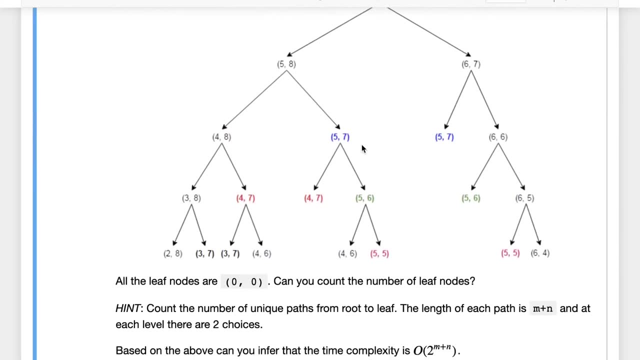 And you can even see this here at the top. you can see that a L O G Y, the problem was called repeatedly: Um. so that's really a source of inefficiency. but now the question becomes that we know that all the leaf nodes will end at zero, zero. 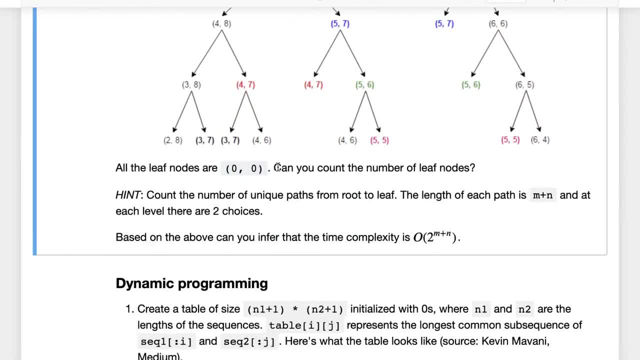 That's when the entire three ends. So can you count the number of leaf nodes? Okay, Can you count the number? If you keep expanding the street, completely, expand each of these, Okay, So we won't skip any of them. Can you count the number of leaf nodes? 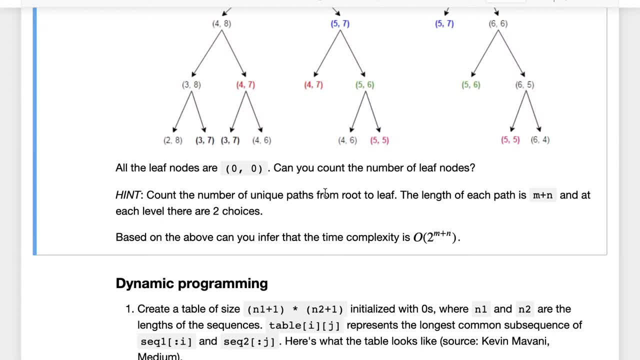 Now, if you count the number of leaf nodes, we know that in a binary tree the number of leaf nodes, if the number of leaf nodes is L? um, then the height of the tree is uh. if the number of leaf nodes is end, then height of three is log N. 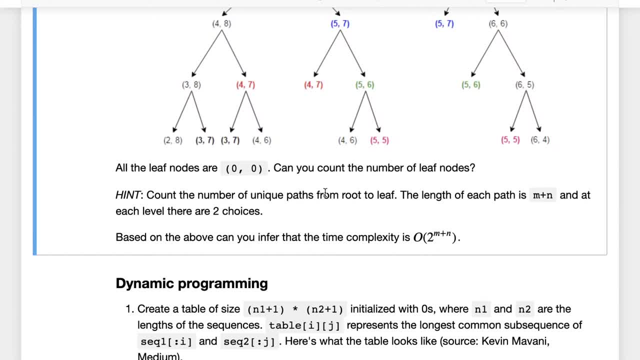 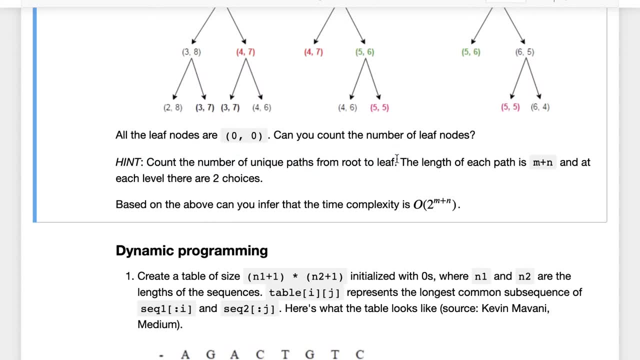 And based on that we can actually determine the actual size of the tree as well. So we know that to count the number of unique parts from root to leaf will give us the number of leaves. So each time we have two choices: we either reduce from the left or we reduce from the right. 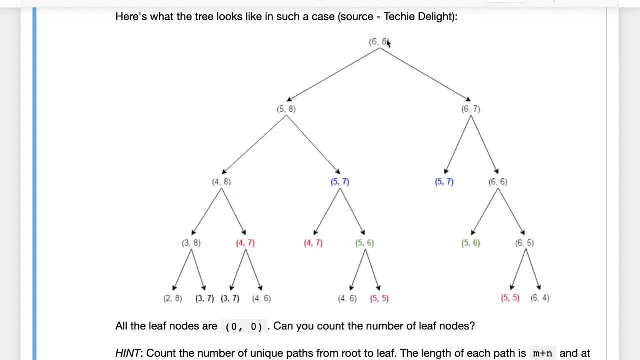 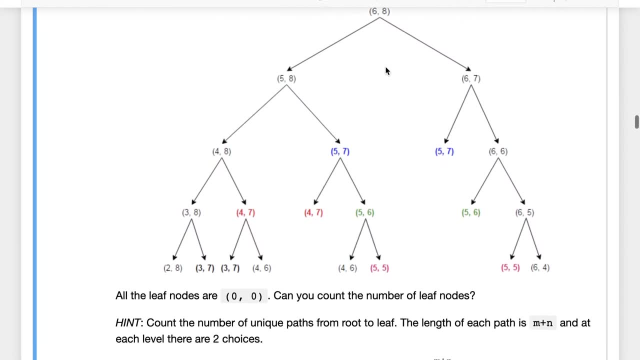 So to get to zero, zero, we would have to reduce all the elements from the left and we would have to reduce all the elements from the right. That means if you have strings, or if you have strings of length or sequences of length, M and N, then you would have to make M plus N choices in total. 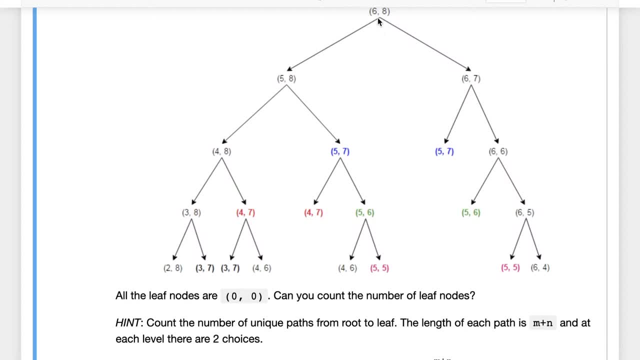 And you. so each time you have M, you have to make M plus N choices. in each time, you have to choose whether you want to To reduce from the left or from the right. we have two choices and you have to make those two choices: M plus N times. 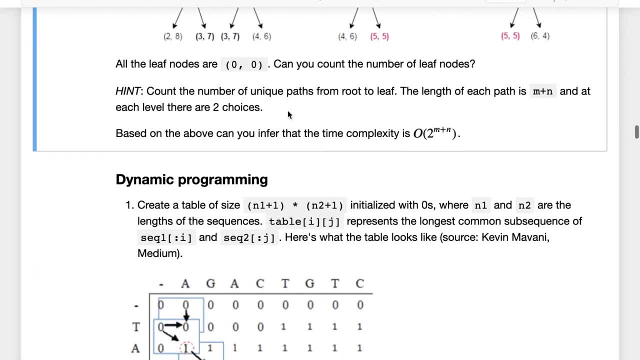 That's the right way to put it really. So that means each time you come you do two choices. So you have to multiply it by two, multiplied by two, multiplied by two, and you keep multiplying that and you will end up with two, to the power of M plus N leaf nodes. 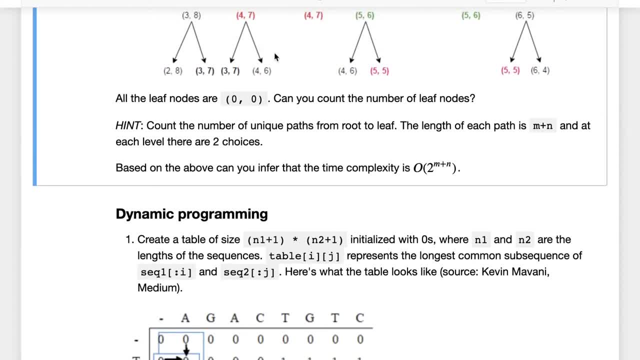 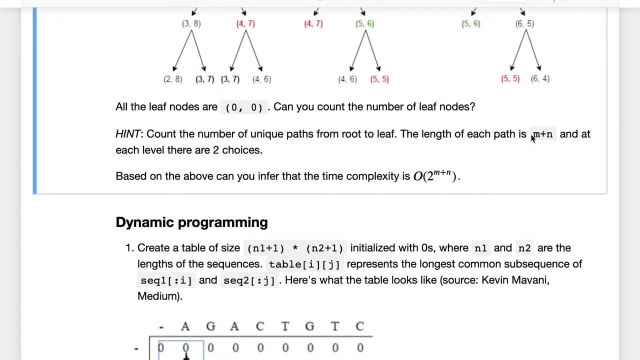 Okay, So here is an exercise for you. Draw this tree on a piece of paper, mark out how the number of leaf Nodes, how the length of each part is M plus N. figure that out And based on that can you conclude that it takes two to the power of M plus N leaves to complete this tree. 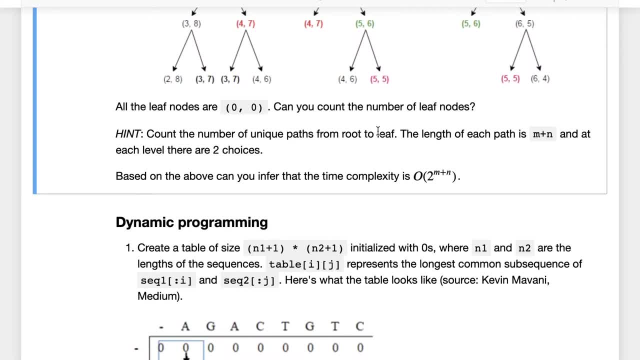 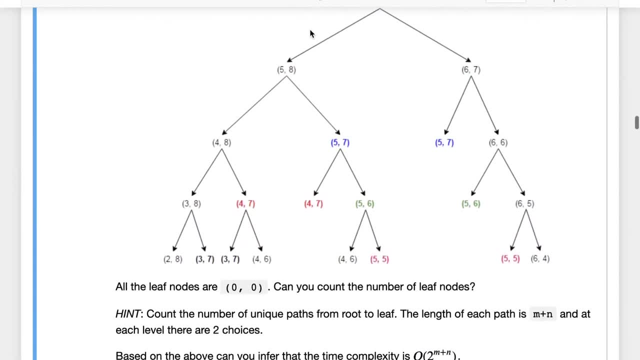 And if two to the power of M plus N is the number of leaves, then the total number of elements is in the tree- Simply double of that. Once again, this is something that is very easy to verify. You can check it here. 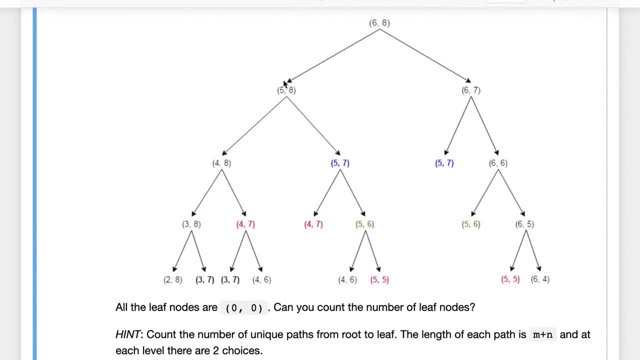 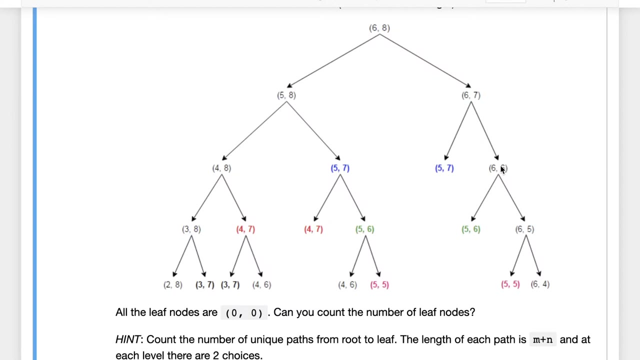 For instance, if you just consider these two levels, the, if you have two leaves, then the total number of leaves is two. The total number of elements in the tree is two plus one three. actually it's double minus one. So two into two, four minus one three. if you have three levels, you can see here that if you have four leaves and the total number of elements in the tree is four into two, eight minus one seven, and you can see that here. 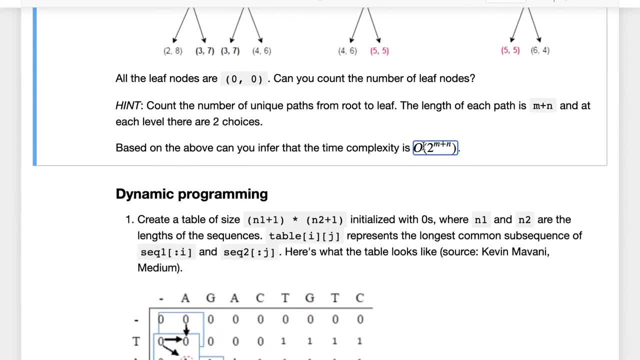 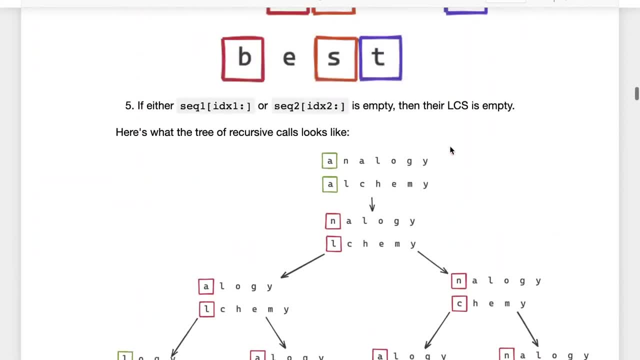 So it follows essentially that we have an exponential number of sub-problems we have, we are calling the recursive function and exponential number of times and inside the recursive function we are doing Okay. So inside the recursive function we are doing a constant time work. 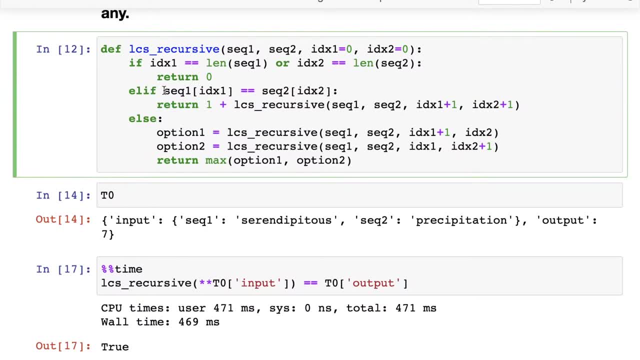 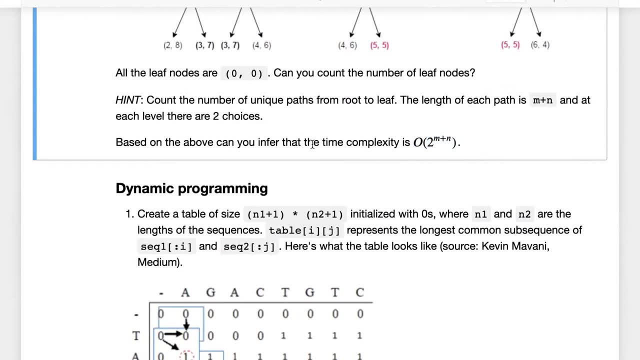 So you can see here that there's no, there's no special work that we're doing. All we're doing is some comparison and we're doing an addition. Both of them are constant time. So we make two to the power of M plus N recursive calls inside each. we do constant work. 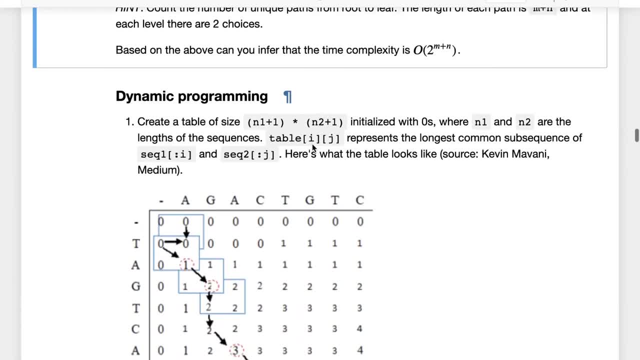 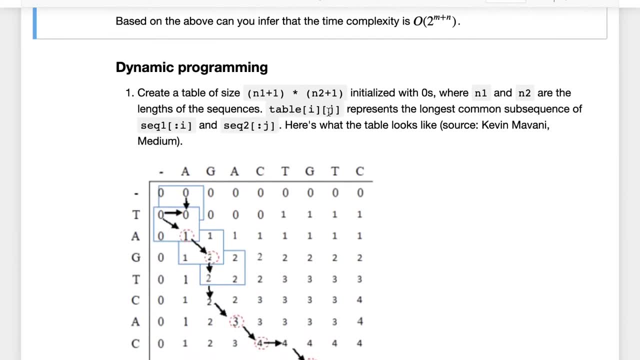 So the time complexity is order of two to the power of M plus N. Okay, That's a rough explanation. We've not gone into a lot of depth because we've covered this over and over in three lessons, but the exercise for you to is to verify how exactly it is. 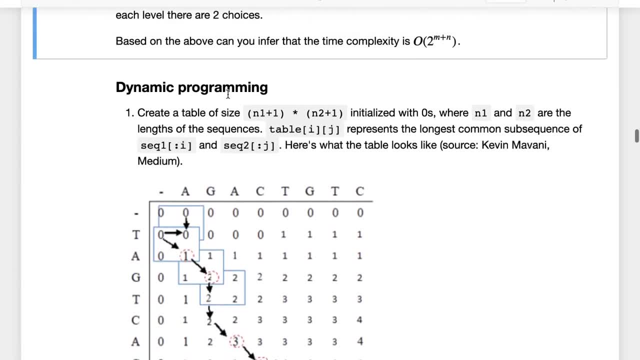 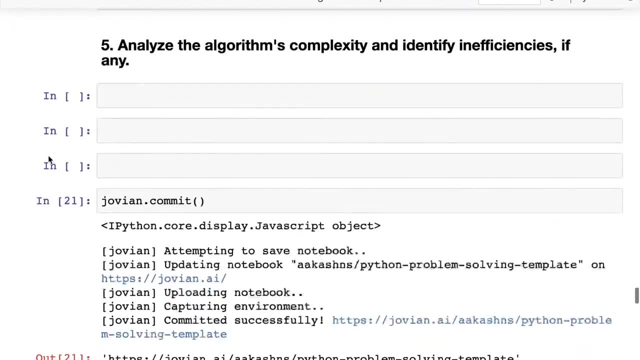 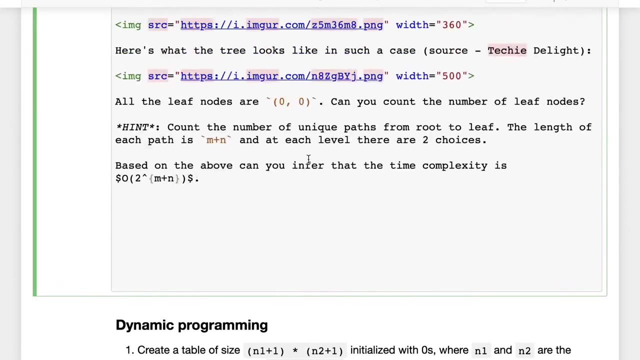 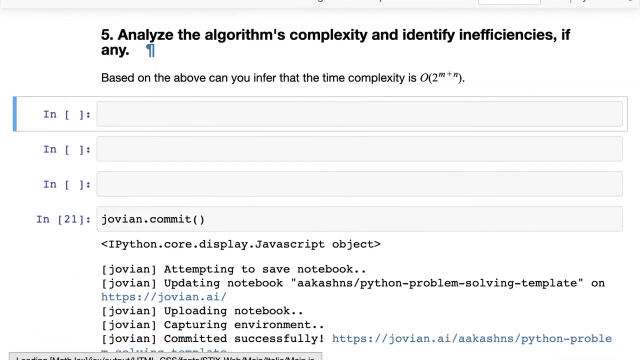 Two to the power of M plus N. Okay, So that's our recursive solution. And we know, we now know that the time complexity is two to the power of M plus N. Let's just copy that over here. And the inefficiency, as we said, in this algorithm is that we are calling the same problem. 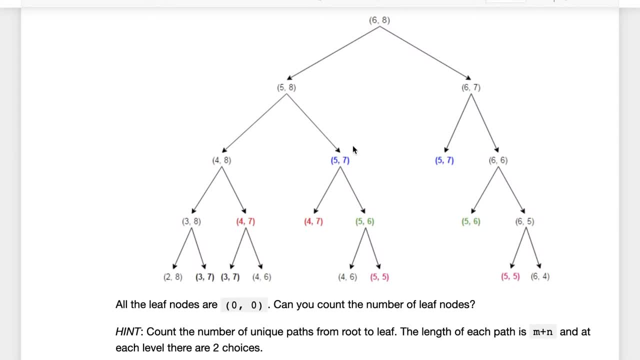 We're calling the exact same problem, though LCS recursive function is called with IDX equal, IDX one equal to five and IDX two equal to seven and IDX one equal to five and IDX two equal to seven. the same time twice. So each of these sub problems will be called twice. 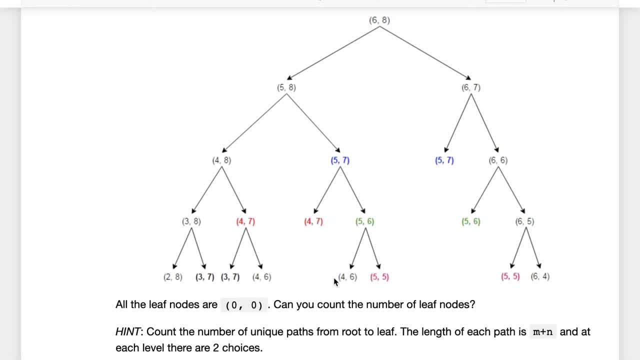 And then each of the sub problems within them will be called twice And, of course, some of these sub problems will once again get shared. So there's a lot of repetition. Now there's a simple solution here, which is simply to remember some of these results. 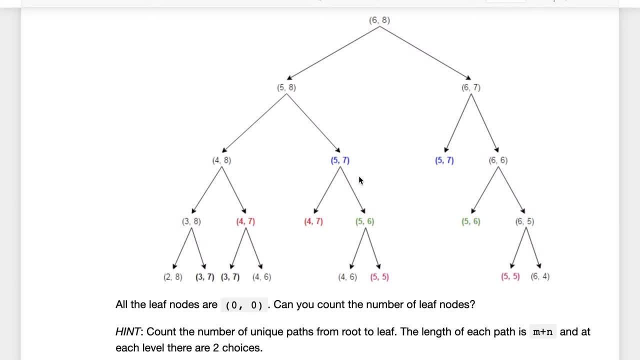 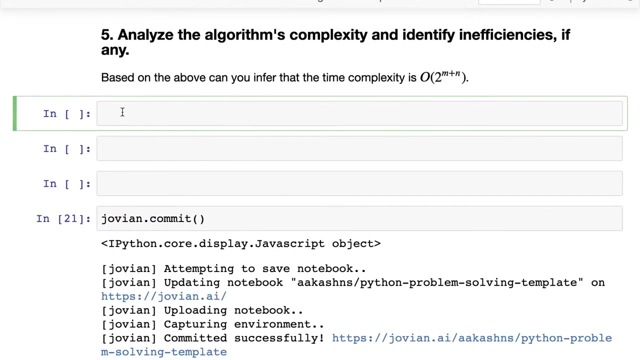 Okay, And this technique is called memoization- And you may also just call it memorization, because you're just remembering some of these things, but memoization is a technical term for it And we remember these solutions in our dictionary called memo. So what we're going to do is we're going to follow the same recursive strategy, but this time we are going to maintain a dictionary called memo and we're going to track intermediate results within the dictionary. 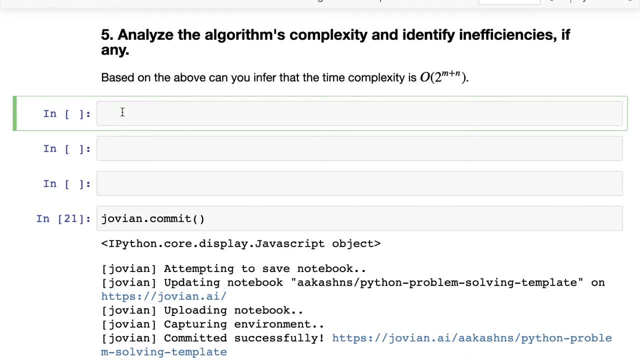 And if we find an intermediate result already exists in the dictionary, Then we will not compute it again. Okay, So let's see. So now we write LCS memoized, or let's just say LCS memo for short. it takes a sequence one and it takes a sequence two. 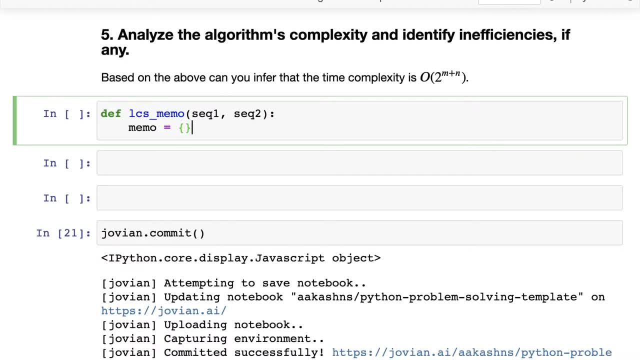 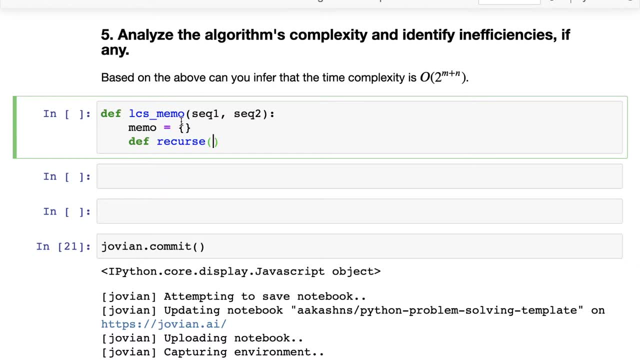 And this time we create this dictionary called memo and then we write a function inside it. So we will write a helper function, a recursive helper function, inside the LCS memo function, so that it has access to sequence one and sequence two, And we will simply start it out with IDX one. 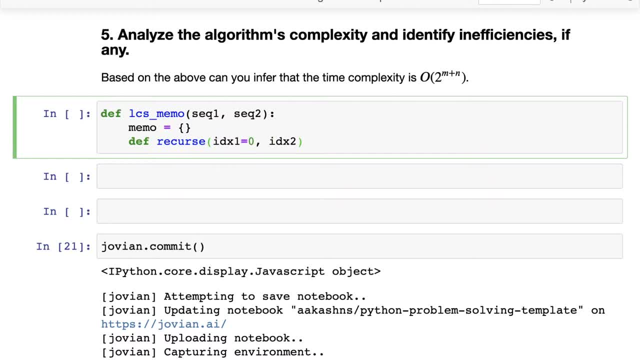 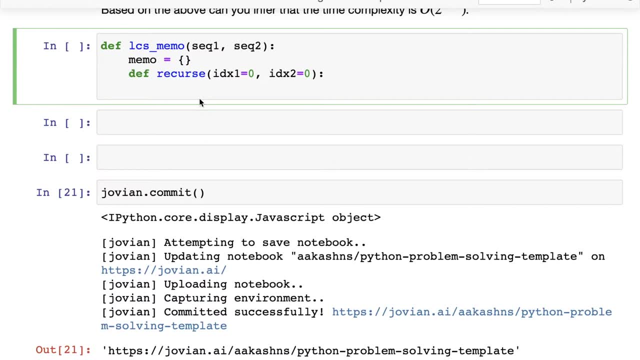 As zero and IDX two as zero as well. IDX one will track the position in sequence one. IDX two will track the position in sequence two. Now the first thing we do is create, using the two indices, create a key. So we are going to create the key IDX one comma. IDX two. 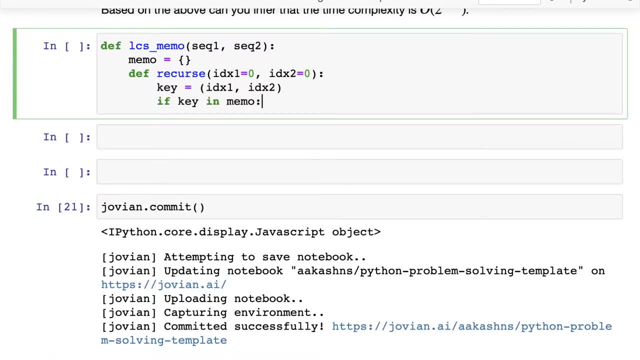 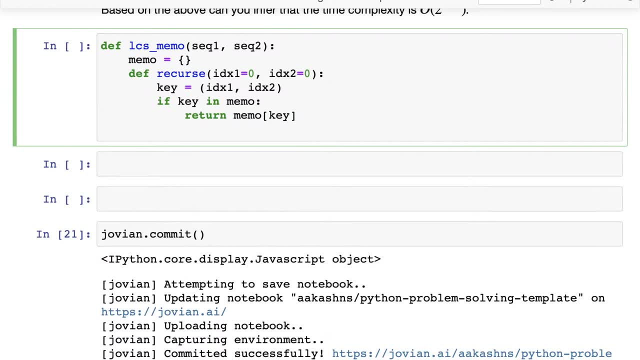 And if the key is present in the memo. so this is the way to check: If a key exists in a dictionary, then we simply return memo of key. simple, The problem is solved. We don't have to solve this problem because it's already. it's already something that we've solved. 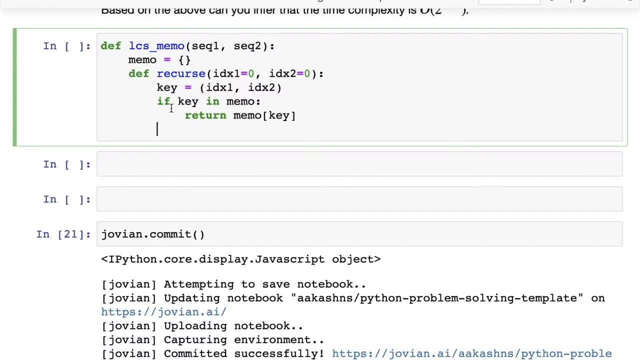 If it isn't, then we need to solve the problem and save it in the memo. Now here we know that we can now write our same three recursive cases. Now, if the base case, if IDX one is equal to the length of sequence one, or IDX two is equal to the length of sequence two, then we simply set memo of four. 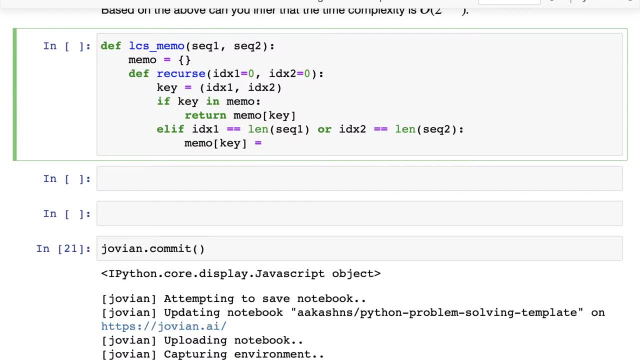 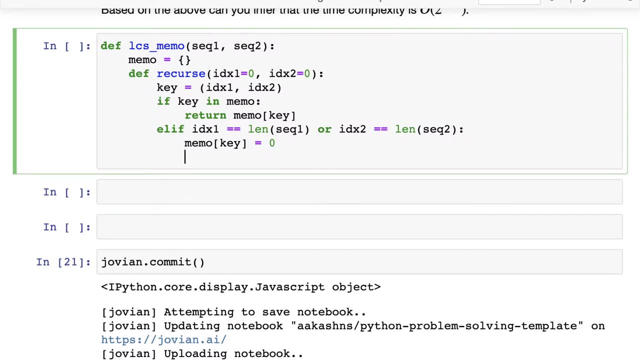 Okay, So we have key as zero, because by this point we have reached the end of the strings. There's nothing left for us to compare LF IDX. sequence one of IDX one equals sequence two of IDX two. So in this case, this is the case where the current characters are equal. 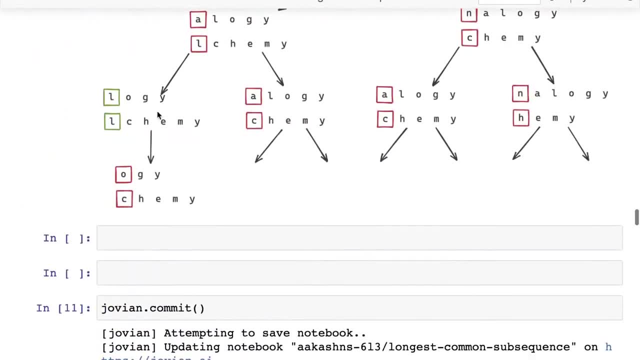 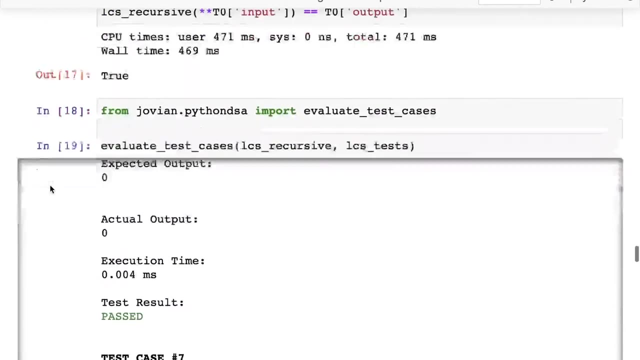 This is if we go up here and look at the tree once again. this is a case like this, where the current characters that we are pointing at are equal, So in that case we simply return. we simply get the result as one plus the result for the remaining, with the first character removed. 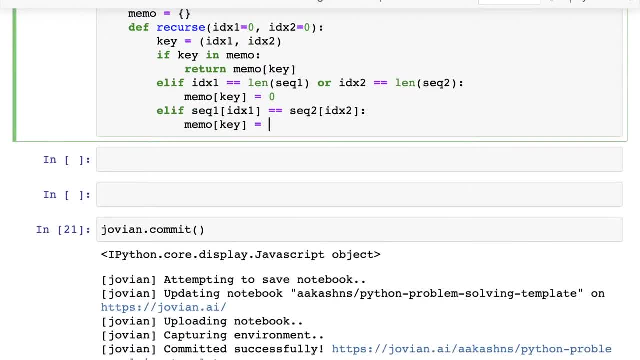 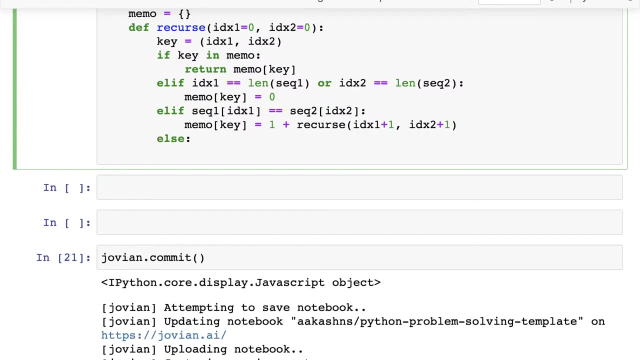 So in this case we simply set memo of key to one plus, We call the recursion, So the recursive function. again it occurs IDX one plus one and IDX two plus one great else. but there's a case where the two elements are not equal. 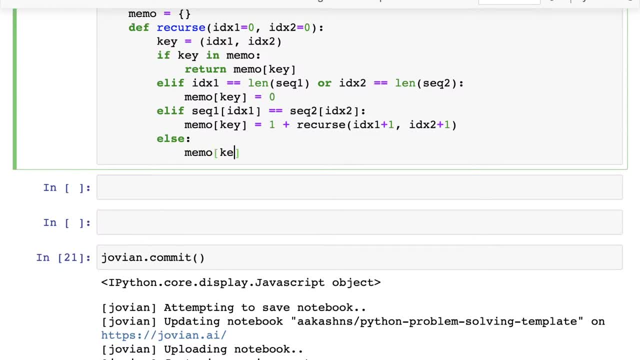 And this is where we have two options. I'm not going to write the two options separately, Let's just do a max directly here. max, and we say: rickles with IDX one plus one comma, IDX two and rickles with IDX. 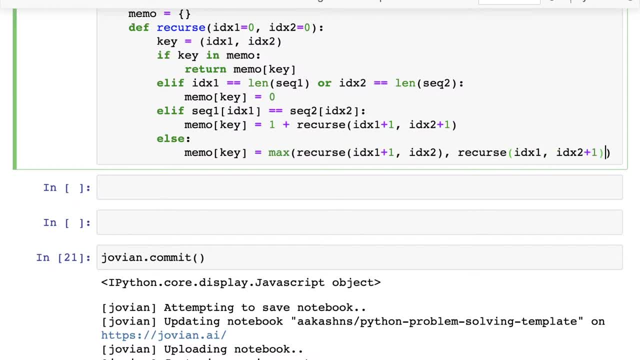 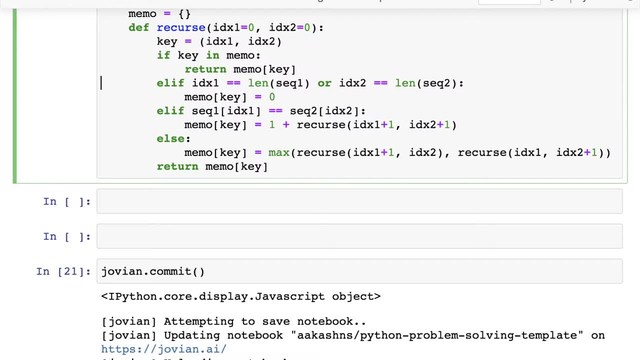 One IDX, two plus one. Okay, And finally, from the recursive function we return memo of key. So we have, whichever case it is, we have computed the result and saved it in the memo. So this time these computations will not get repeated again and again. 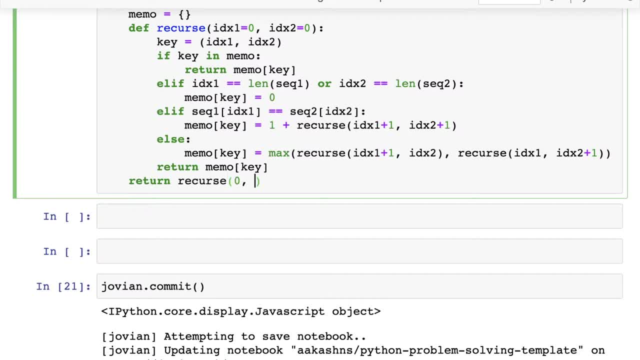 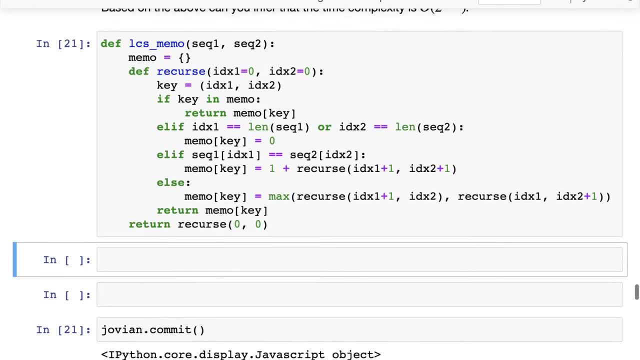 And let us know it'll done because of zero comma zero, because zero comma zero is the entire Yeah ring and that's it. And this is the common strategy that you should apply Whenever you come up with a recursive solution and you see the inefficiency. 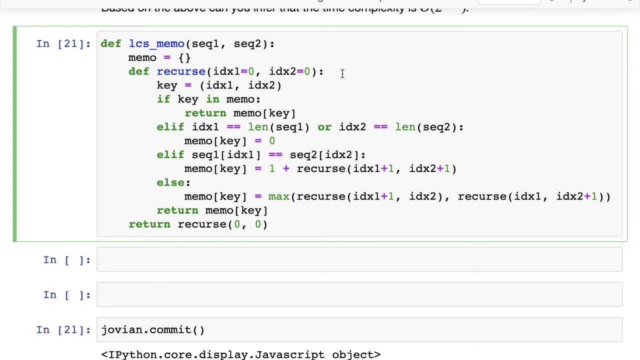 coming because of the same problem being called again and again and again. this is where you need to apply this technique called memorization right, And in this technique, you will then be able to simply store intermediate results. So it's really simple. 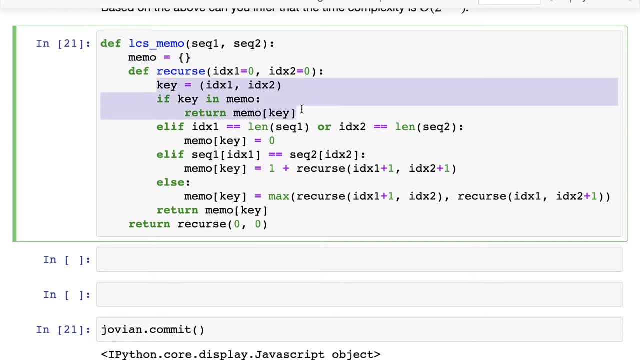 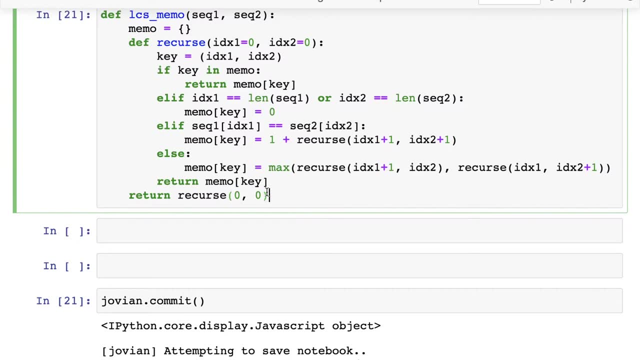 You just create a dictionary and then you add one or two lines of code here and you make sure to save the result in that dictionary Whenever you compute a result. the next time you don't have to compute it. Okay, And we can test it out. 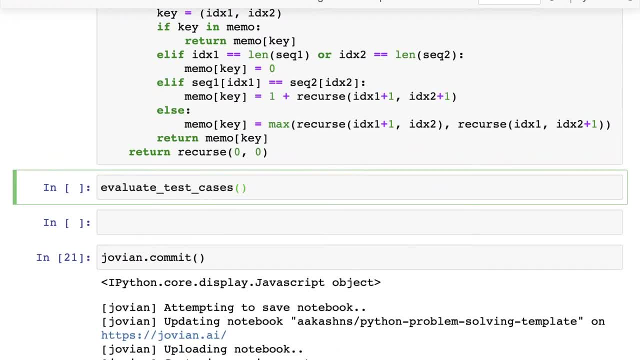 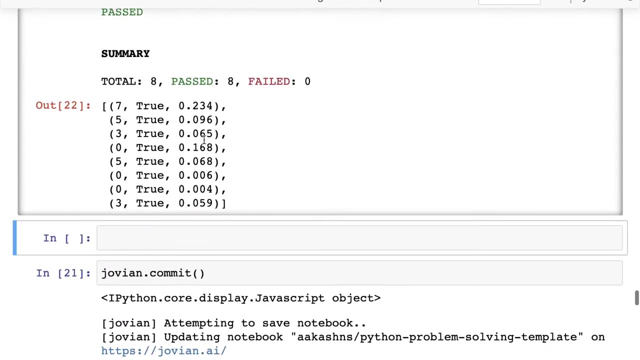 We can test it out with all the test cases. evaluate the test cases, So LCS, memo and LCS tests, and you can see that all the test cases pass. Now, not only do all the Test cases pass, You can see that the time taken is now lower. 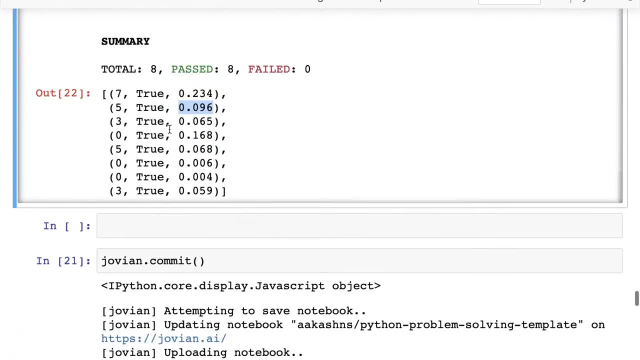 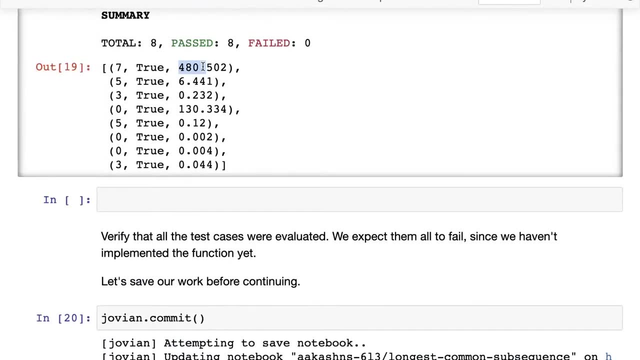 Okay, So that's nice. The time taken is now lower. Now we went from 450 milliseconds. If you just go up here, you can see that it took 480 milliseconds for the for finding the longest common subsequence between precipitation. 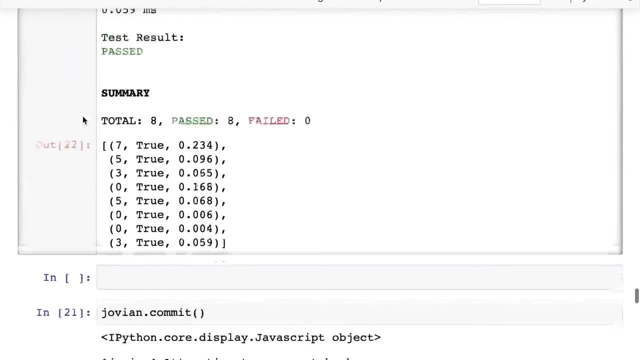 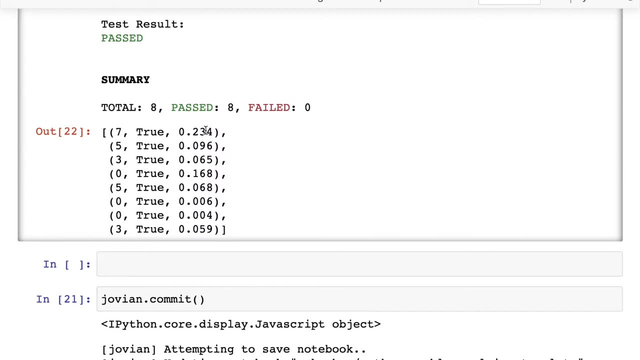 And serendipitous. but in this case it only took about 0.234, which is 0.2 milliseconds. So it is 2000 times faster, even for strings of length, seven or eight, And that's a huge boost. 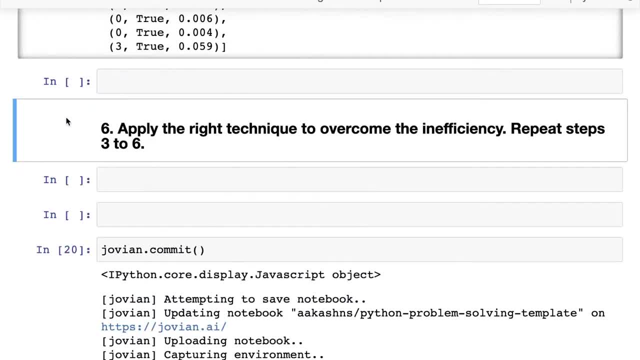 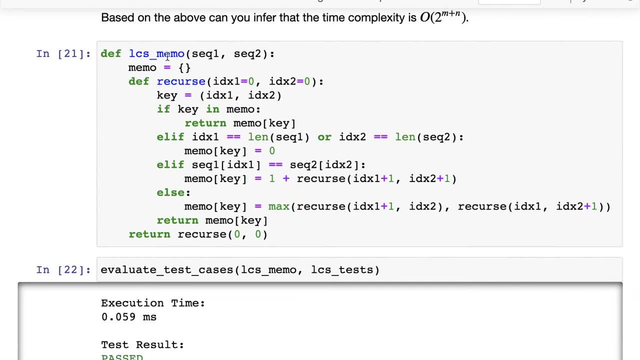 Um, let's analyze the complexity here. Let's look at the complexity Now. a quick way, an easy way to find the complexity of the solution is to see where the computation, how many times the computation can occur. Now this is. 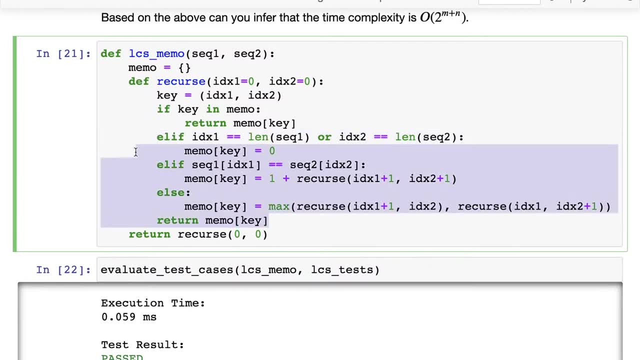 Where the bulk of the computation is occurring in a recursive call and this computation is avoided if we already have something in the memo. Okay, So that means that the only number of computations that we need to do is equal to the maximum number of elements that can end up in the memo. 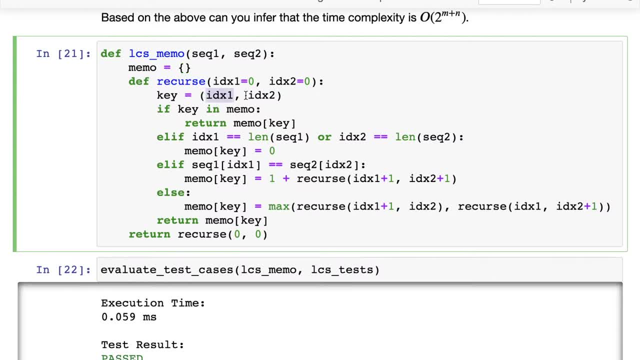 Now, what are the keys in the memo? Look like the keys in the memo. look like IDX one and IDX two. Great, And what values can these take? IDX one can take zero to M values, If M is the length of sequence one, let's say. and IDX two can take zero to N values. 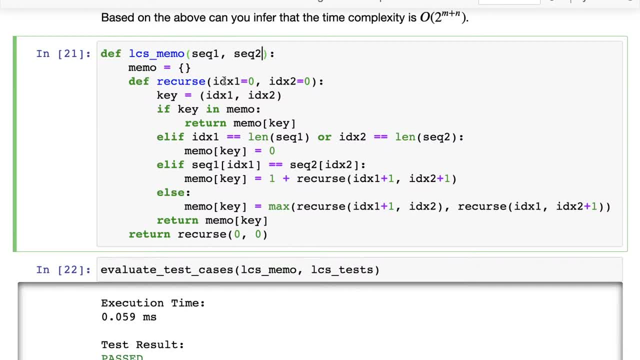 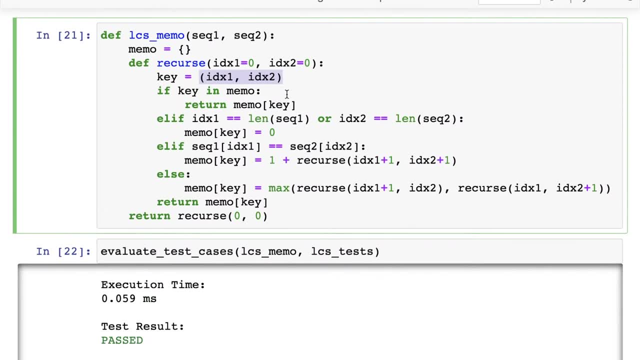 If N is a sequence, a length of sequence two. So in total, the possible number of keys is M times N. The possible number of keys is M times N. The possible number of things that you need to store in the memo is M times N. 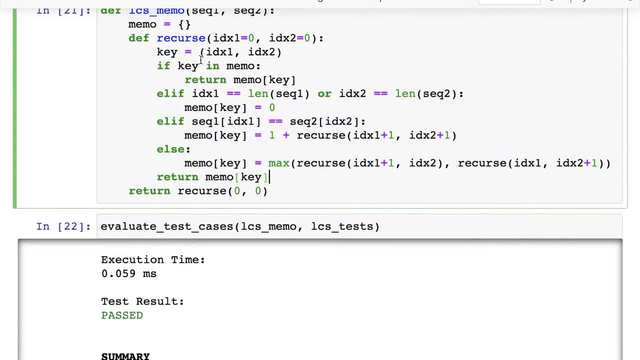 And for each of them you do constant work. And then the next time you try to access this, you do not need to do the rework, You do not need to call any recursion, You can simply access the memoization right. 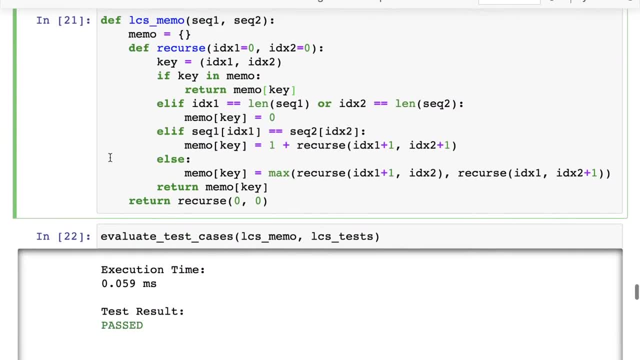 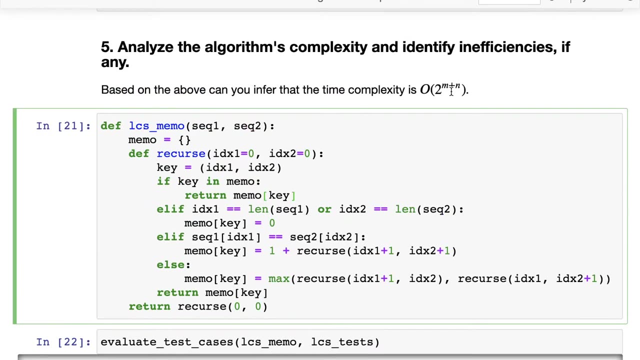 So what that tells us is the complexity of this case, and in any memoization case in general, is equal to the number of keys, which in this case is M times N. So the time complexity here is order of M times N. So we've gone from two to the power of M plus N, which, if you, if M plus N was, 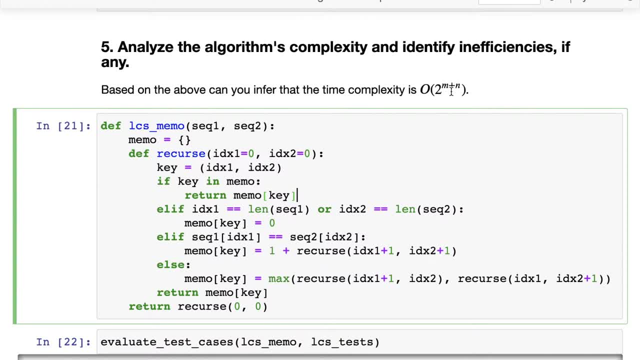 equal to 30 would be 1 billion to M time. order of M times N. So let's say both strings were 15 and 15, but that would just be 225 operations. So we've gone from 1 billion operations to 225 operations simply by storing. 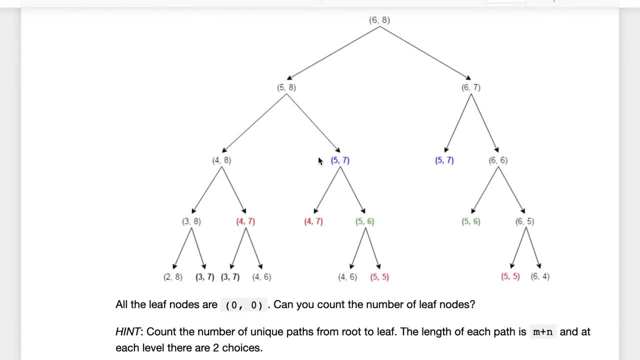 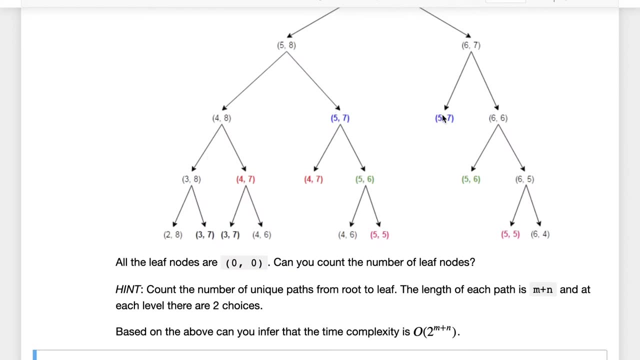 intermediate results and so very powerful technique that we apply all the time. So now you can see here that the first time five seven is computed, The next time five seven does not need to be computed again, And that's why this tree here is actually marked out. 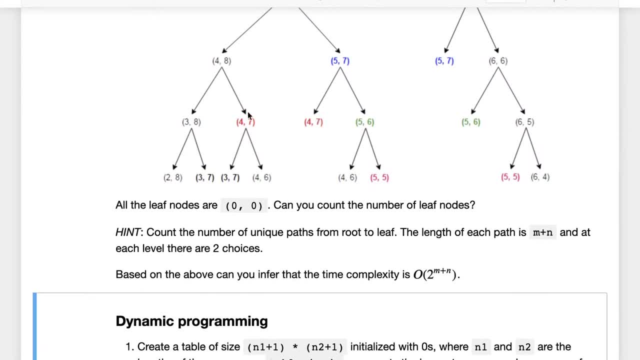 So this is the tree for memoization. This is the first time four seven was computed. It never needs to be computed again. So this entire tree of computation gets eliminated And similarly this entire tree of competition gets eliminated. We are eliminating from 1 billion computations almost all except 225 computations. 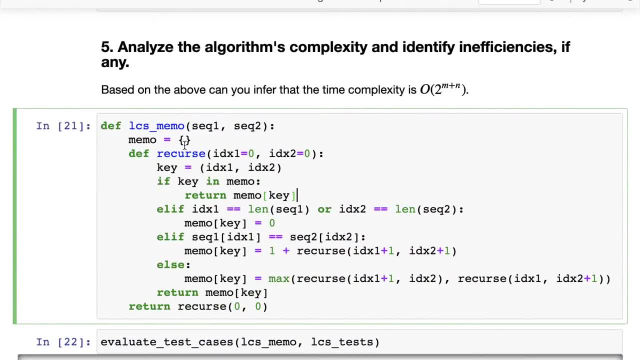 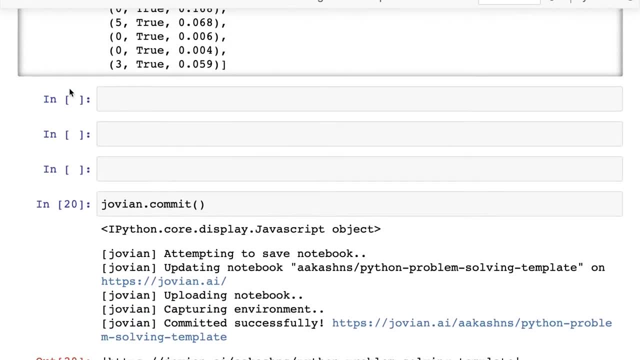 So we are left with practically nothing And that speeds up your algorithm by a huge, huge factor. So that's memoization And, as he said, it's really easy to compute the time complexity of memoization: Just simply count the number of keys and then just track. how much work do you need to compute each key? 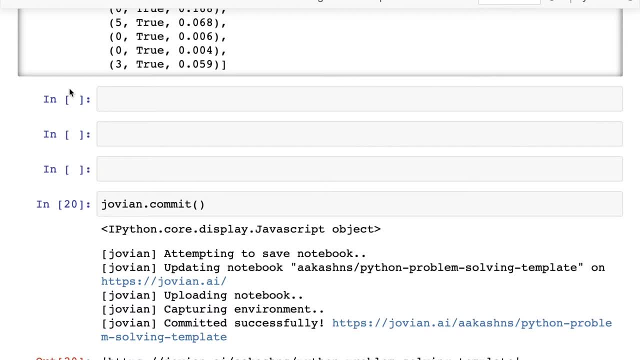 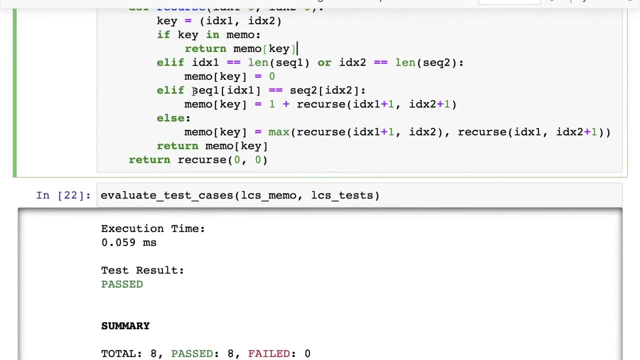 Assuming that you already have the recursive solutions for the remaining. Okay, So how much work do you need to compute each key using some other existing solutions? Now, in this case, that was constant, because all we needed to do was compare and add. 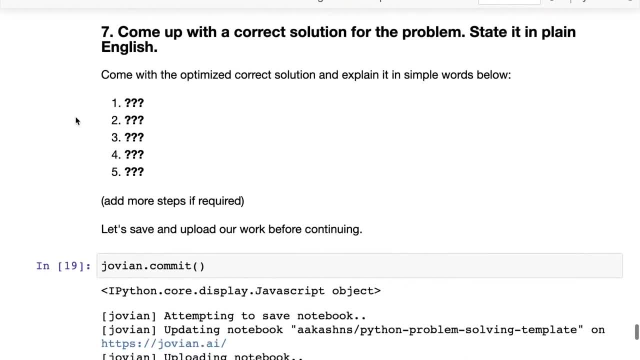 So we know what we want to do with. how much work do we need to compute each key And from that we define the term. And if I start by saying move the key, move the key. and then we're going to look at the virtualization process. 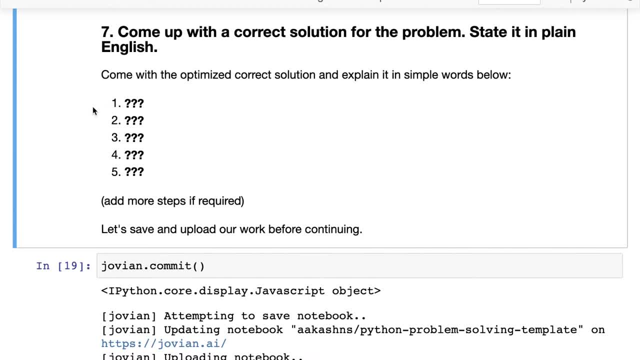 So the first step is to add the recursive commands to the machine. The second step is to add the recursive to each key to the machine, And the third step is to add the recurve commands to each key, And then we'll look at the rest of the code. 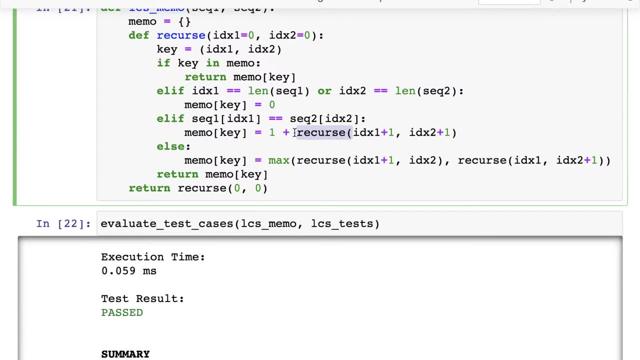 Now we just have to take two steps and go through it each time. One is to define the code, which is going to give you a nice idea. The other is to define the code itself, and then we'll go through it one by one. 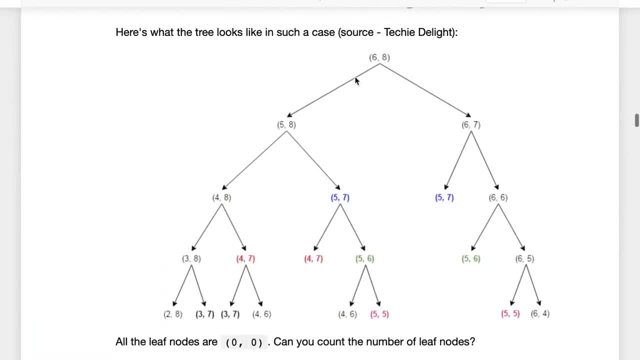 Okay, has an overhead and the overhead for the question. if you see it this way, is that for this function execution to complete, you need this function execution to complete and this to complete, And for this to complete, you need this to complete and this to complete. 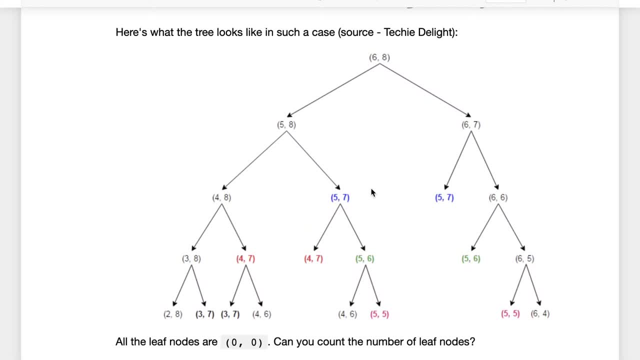 Right. So the idea here is that for each new recursive call takes more space in the memory and it also takes longer because now we have to allocate some memory and then set up that function stack, the function stack for the execution of that function. 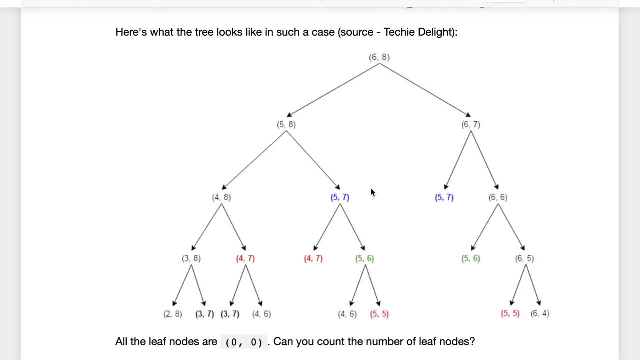 So if you have a large tree, then you're creating hundreds, thousands or possibly millions of open functions, all of which have their own memory, And that can eat up a lot of memory And sometimes that can also take up a take longer time. 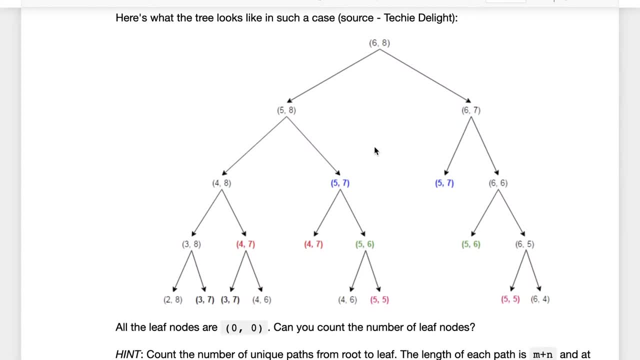 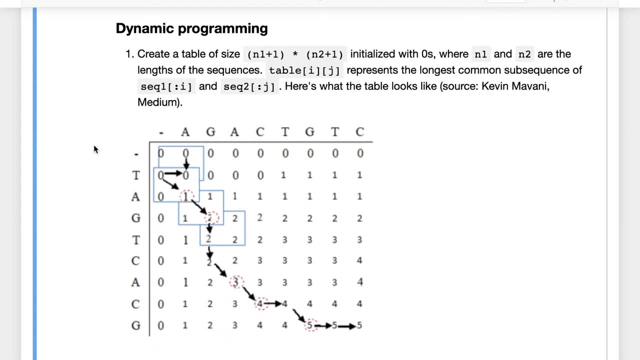 So the solution to replace recursion is iteration. And how do we do that? We do that using a technique called dynamic programming, So we'll do almost the same thing. There are a few changes here. Instead of using a Dictionary to track intermediate results, we will create a matrix, because we know. 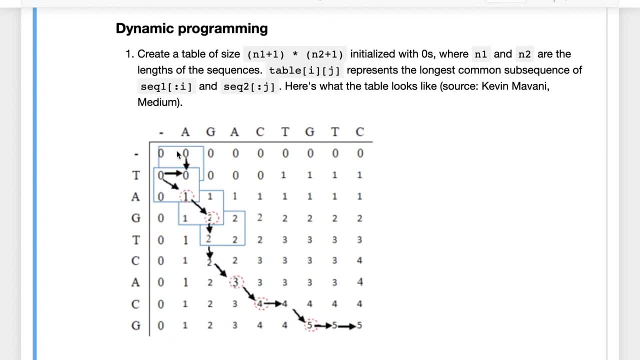 that sequence one, the IDX one, can go from zero to N or zero to N one, let's say, where N one is the length of sequence one and sequel IDX two can go from zero to N two where N two is the length of sequence two. 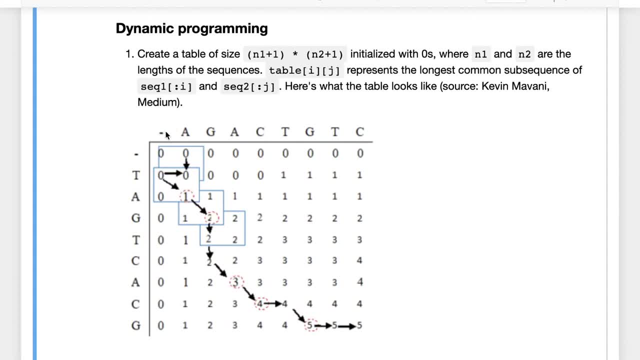 And what we can do is we can use a for loop or a couple of for loops to fill out all these sub problems without having to require a recursion. Okay, And this is how we'll do it. So let's say, these are the two strings that we're working with. 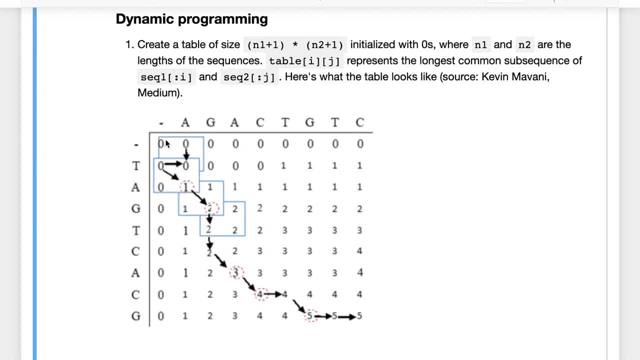 This is string one: E a CGT, and this is string two. And these, this is what the DNA sequences look like. So what we'll do is we will create a table of size and plus one plus one, and N one plus one and N two plus one. 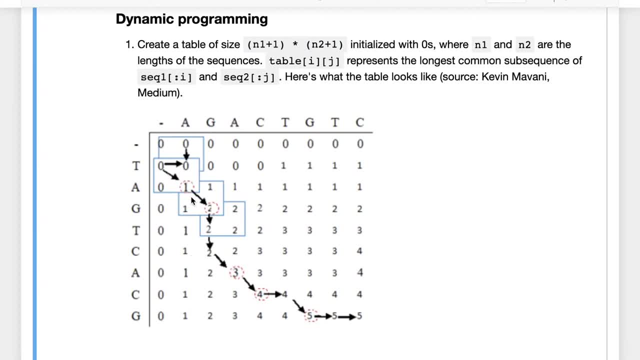 So you can see that there are N one plus one rows. So if this is of length N one, these are N one rows. and then there's an additional row And similarly there is there are N two plus one rows Here. 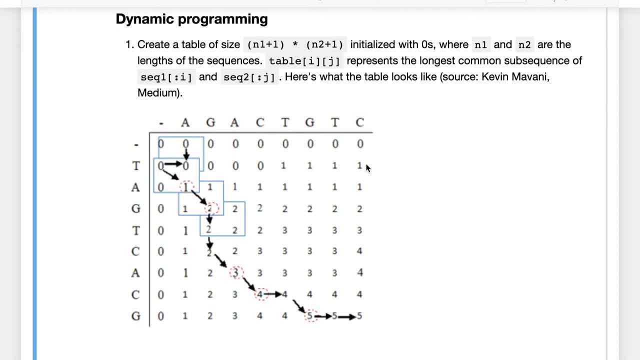 So if this is of length, N two, there are. there are N two plus one columns. So you can see these are N two columns and there is an additional column here and table of I N G. So let's say table of, uh, if I N G are zero. 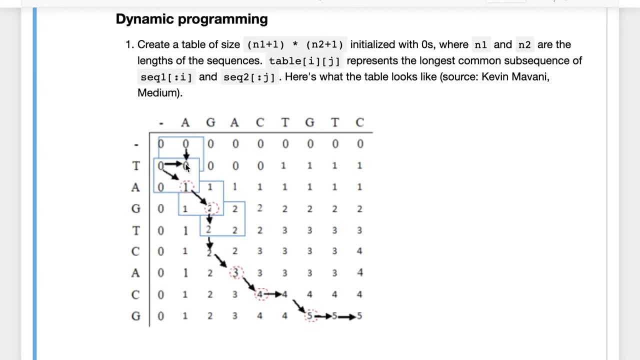 So I is a pointer for the first sequence and J is a pointer for the second sequence. So I selects a row and J selects a column. So table of I N J represents the longest common sub sequence Off sequence One up to I, which means sequence one. 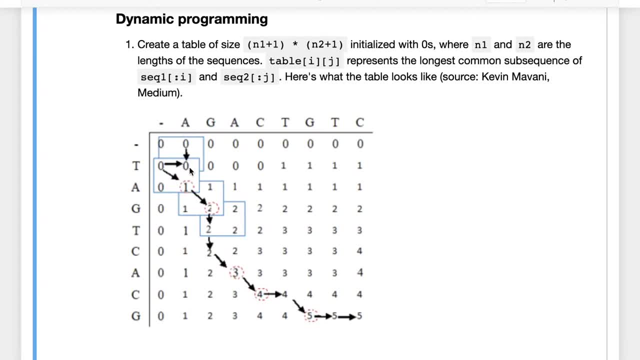 So here, if let's say I was one and a J was one, So this represents the longest sub sequence of sequence one up to I, So all the positions before one, which means only the zero position, just T, and sequence two up to J, which means all the positions up to the first position of up to up to one. 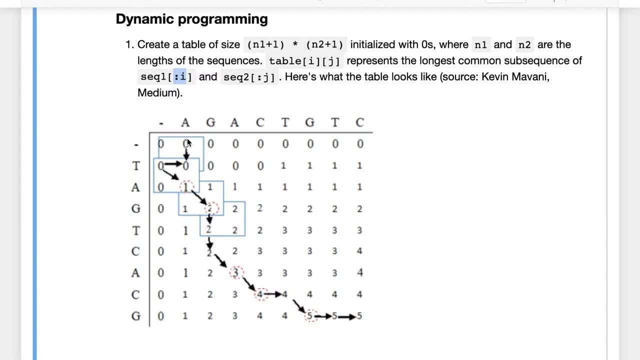 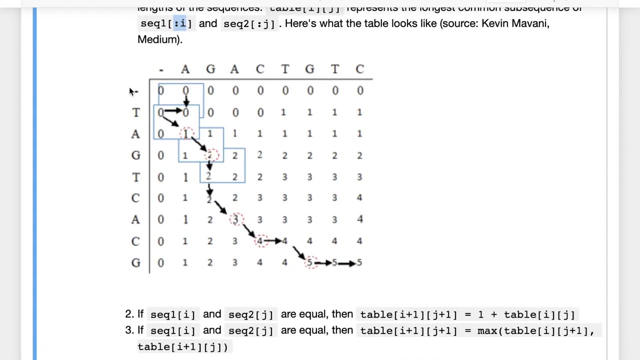 So which means only the zero position, So which means a okay. So table one in a table I J represents the longest common sub sequence of these two, of just a NT which is zero. on the other hand, if we skip ahead a little bit, if we skip ahead to, let's say, this position, you can count here. 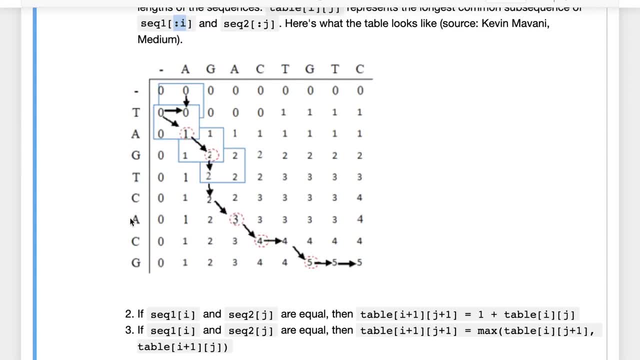 I go: zero one, two, three, four, five, six. So this is six here, And here we have zero one. zero one, two, three. So this is so. this is table of six, comma three. the table of six, comma three takes the first six elements, which is T, a, G, T, C, a, and the first three elements a, G, a of sequence two. 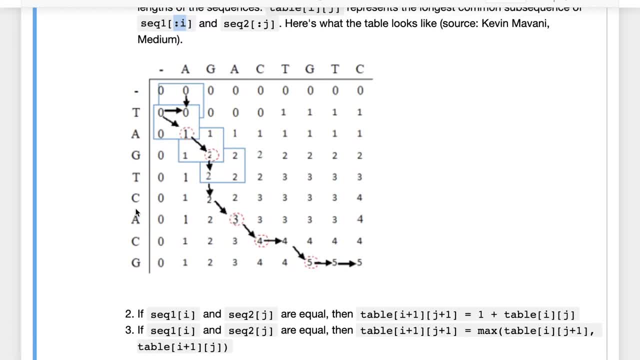 And it stores the result of the longest common sub sequence between these two. Okay, So I'll just let you look at the table and maybe even draw the table on a piece of paper and verify that the length three You can see here: a, G a, a G a occurs here. 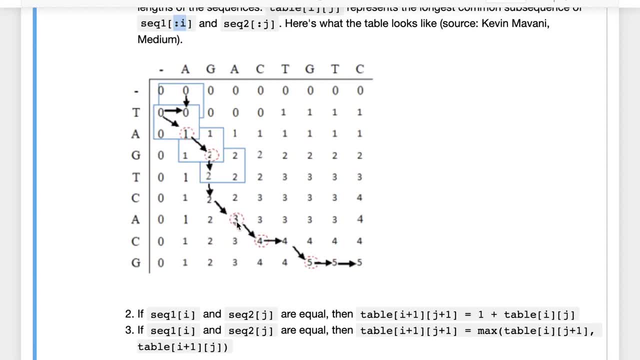 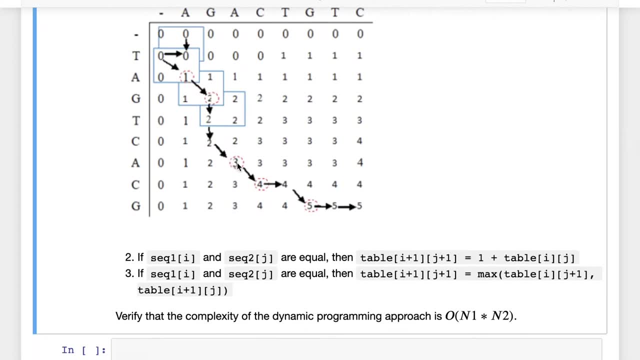 So a G a is a sub sequence of T a, G, T, C, a, So the longest common sub sequence between them is three. Now what we do is we will now compare the next elements of. we will now compare sequence one of I and sequence two of G. 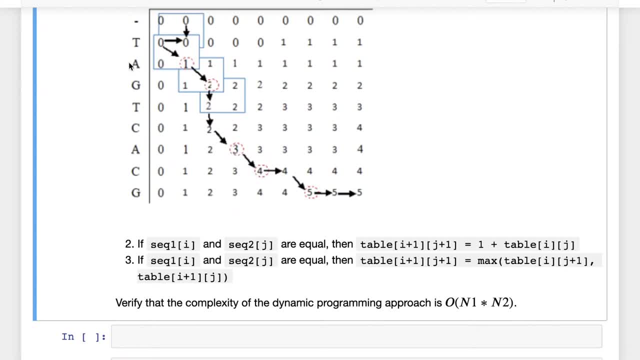 So let's say we are looking at, let's pick an example, Let's say sequence. or let's say I has the value. I has a value zero, one, two, three, four. I has a value of four. Oh sorry. 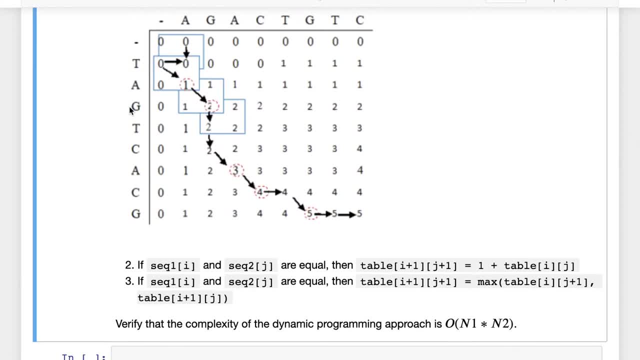 Let's say I has the value zero one, two, I has a value of two, and let's say G has the value one, So zero one. So if we compare sequence one of I, so which is G, and sequence two of a sequence two of G, which is also G, and if they're equal, so if they're equal, then 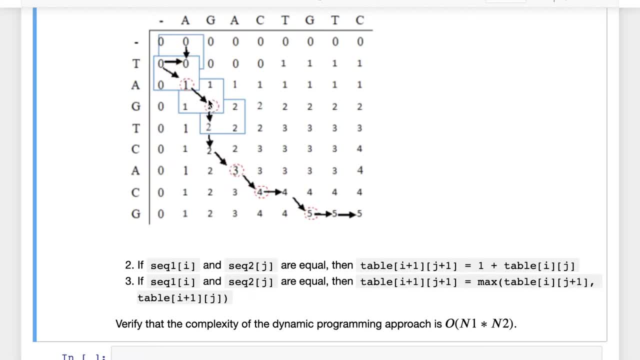 Able, Able of I plus one on J plus one, which is this value, right? So remember, I is two and J is one, So table one of I plus one, So table one of three is zero. one, two, three and table and they will own of I plus one, G plus one is able, one of three and a table, a table of I plus one and G plus one. 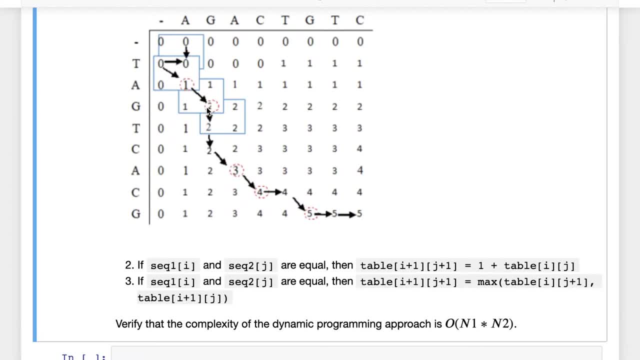 I being two and J being one is table one of three and two, and table one of three and two is the value two. So this value is obtained by adding one to table one of I comma G, So because these two elements are equal. when we can then say that if we take the longest common subsequence of T and E and add one to it, that will give us a longest common subsequence. 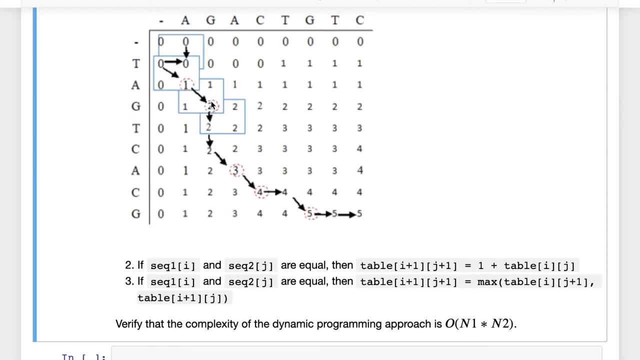 So the longest common subsequence of TAG and AG. so the exact same logic as recursion. we have simply now reversed it. So we now- now we're looking at the last element, so that we can keep filling out the last value using some previous values. 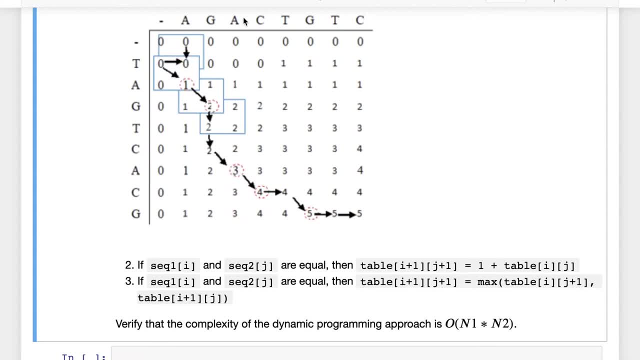 Okay, So this is one case. Similarly, here's one other case where a and a are equal. So the longest common subsequence between TAG TCA and the longest common subsequence between AGA is one, plus the longest common subsequence between TAG TC. 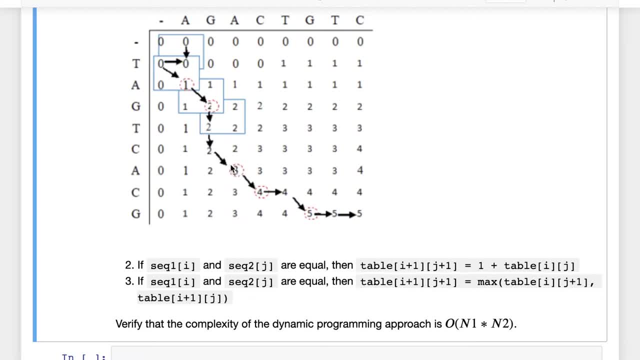 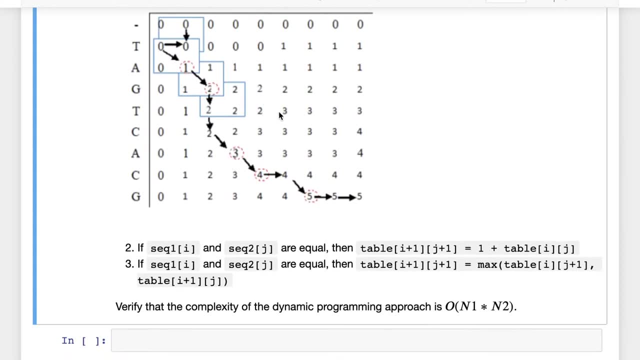 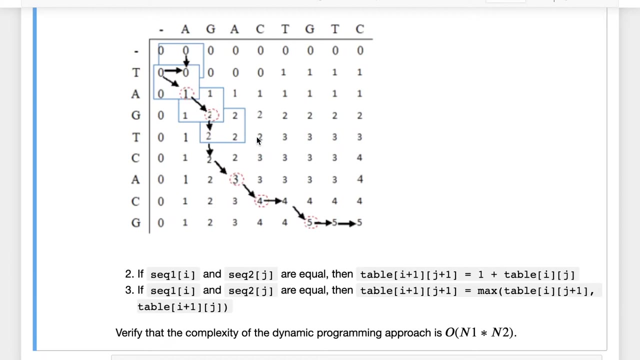 And EG. okay, One plus this value. So that's one case. The other case is if they're not equal. So let's look at this value, for example, over here. So we have TAGT on the side and then we have: okay, let's, let's look at this one. 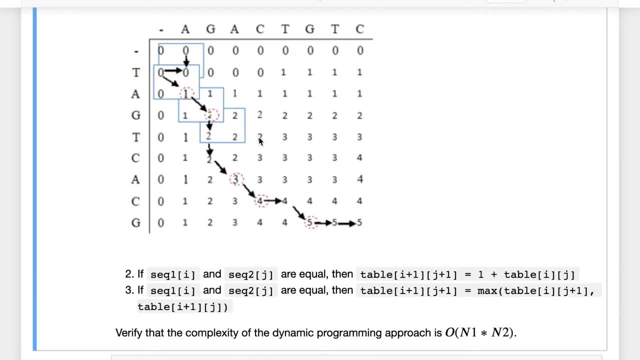 Uh, we have TAGT on the side and we have AGAC on the side. Now T is the element here and C is the element here. They are not equal. So that means the Longest common subsequence between these two either does not contain T or it does not contain C. 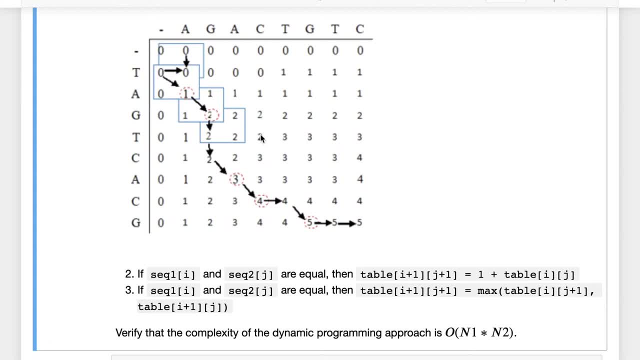 It cannot contain both, obviously, because one of the strings has to end. So if it does not contain T, then it is this result, And if it does not contain T, if it does not contain C, then it is this result. So we simply take the maximum of these two, maximum of these two to get the result for this. 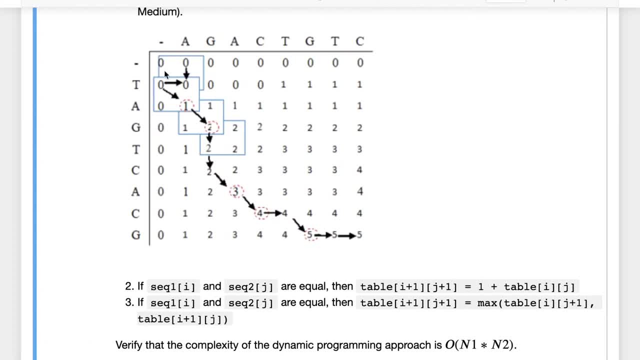 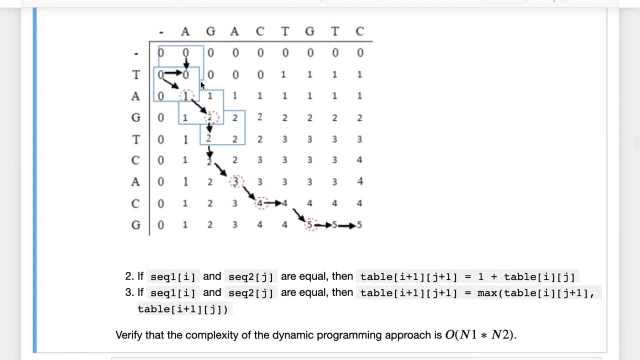 If these two elements are not equal- and that is how you fill out the table- You start from the top. The first row is zeros because we are, we have empty strings, And the first column is also zeros because we have empty strings to fill out an element. 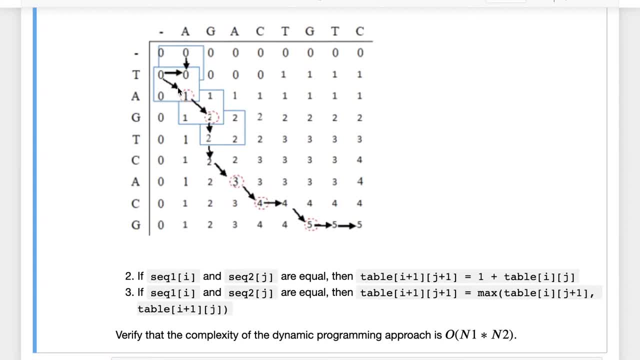 You compare if the two elements are equal. and if they're equal, we simply add one to the diagonally left top left element. If they're unequal, then we take the maximum of the element above it and the element to the left of it. 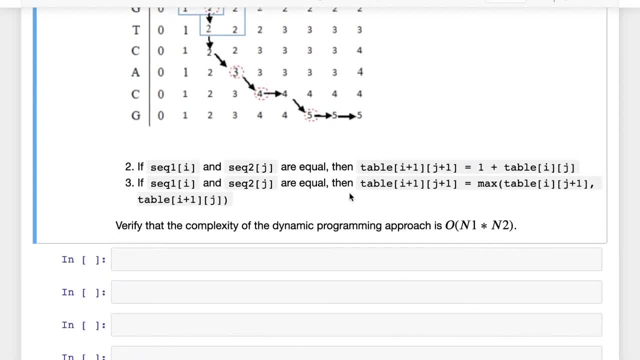 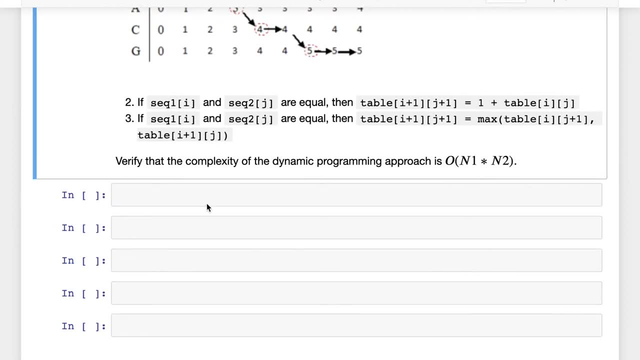 And that way we fill out the entire table. Okay, So that's the dynamic programming solution, And I know this can seem a little bit complicated. Uh, honestly, I still get confused with dynamic programming a lot of times, And that's why I like to just draw tables and write things out carefully. 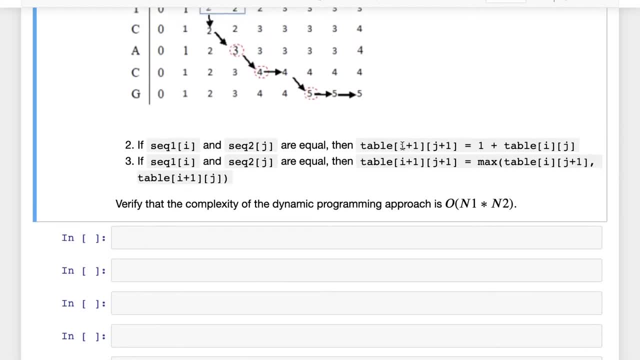 Okay, And and especially, you have to be specially careful with indices, because here we are saying that if sequence I, one, I and sequence to J are equal, then table one of I plus one and J plus one is one plus table IG. 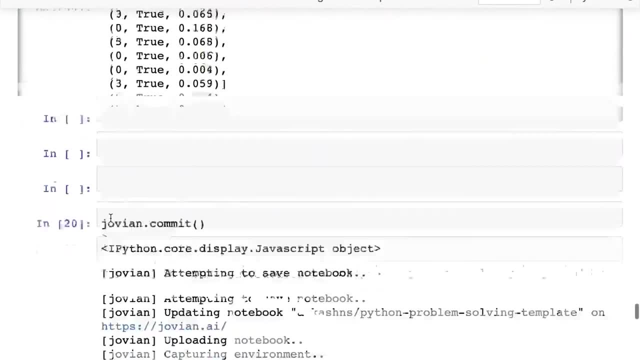 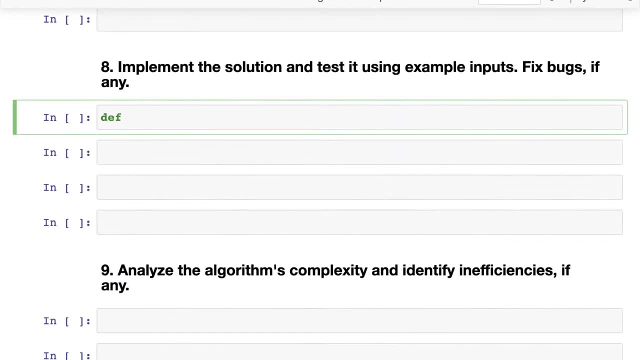 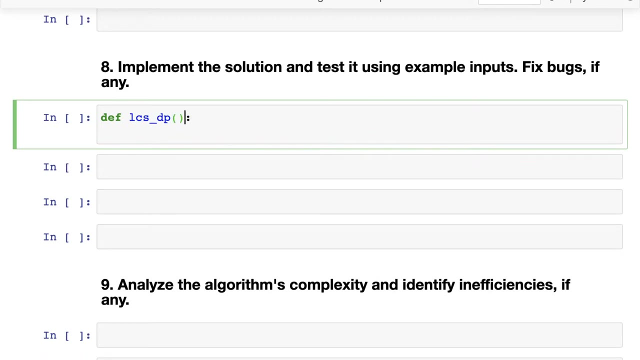 So be? just watch the indices carefully here. but let's implement the solution, Let's implement the dynamic programming solution. So let's say LCS, dynamic programming. So we'll just say DP here, And we have sequence one, And we have sequence two. 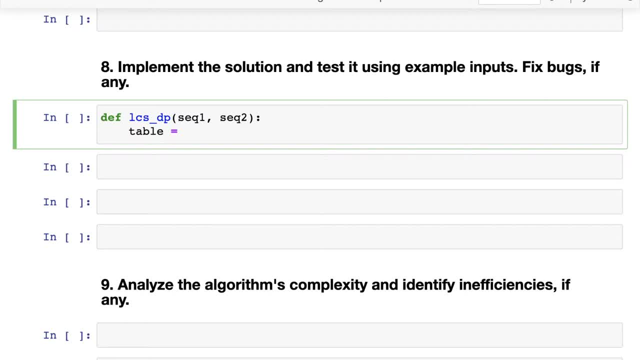 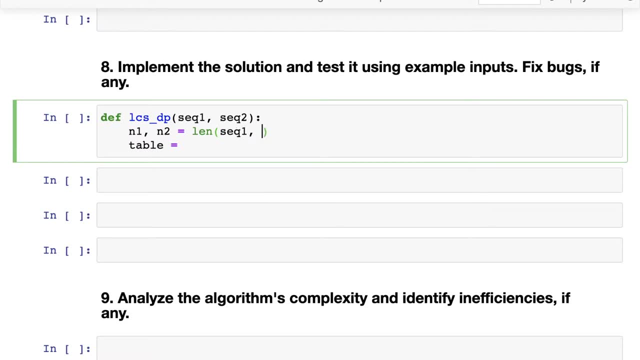 And the first thing we need is we need a table of results. Now, this table for it. let's just grab N one and N two. So length of sequence one And Okay, Okay, Okay, Okay, Okay. Length of sequence two. 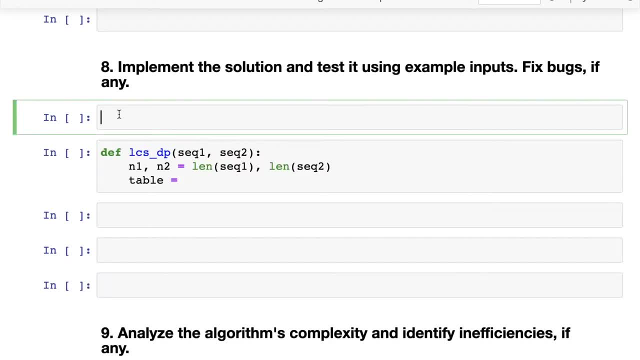 And now we need to create a table with all zeros. How do you create a table with all zeros? A way to do it, a way to create a list of zeros, is this: zero four, underscore in, let's say, and let's give anyone an end to some values. 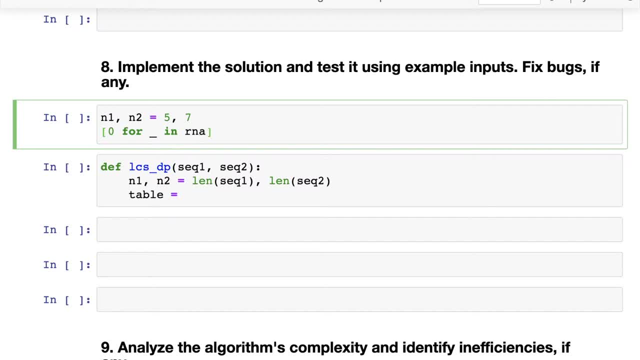 Now, if you want to create a list of zeros of length and one use, you simply say zero, four underscore, or you can even say zero for X. You're simply ignoring whatever value you're getting from a range. a range and one, and that's going to give you a list of zeros. but we don't want a list of N one zeros. 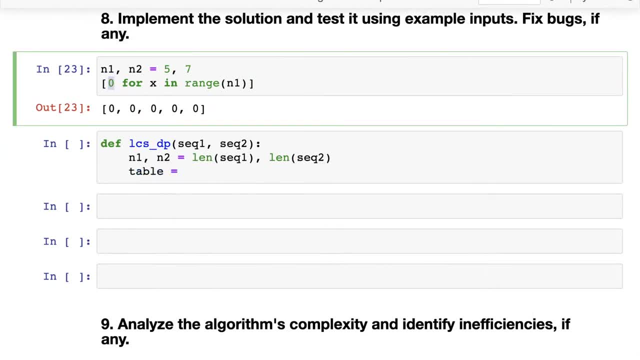 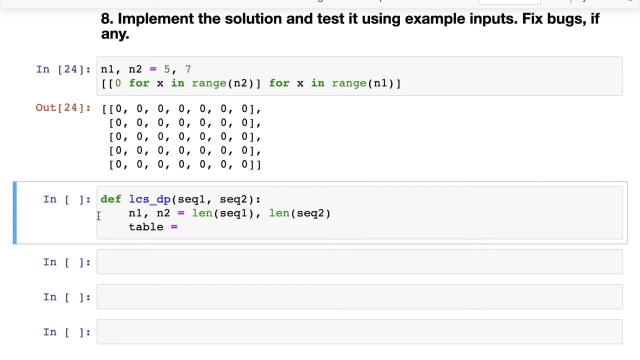 We want these more. these want to be rules, So we want each of these to itself be a list of zeros of length and two. so zero, four, X in range and two, And now we have. you can see that we have five rows: one, two, three, four, five. then we have seven columns. 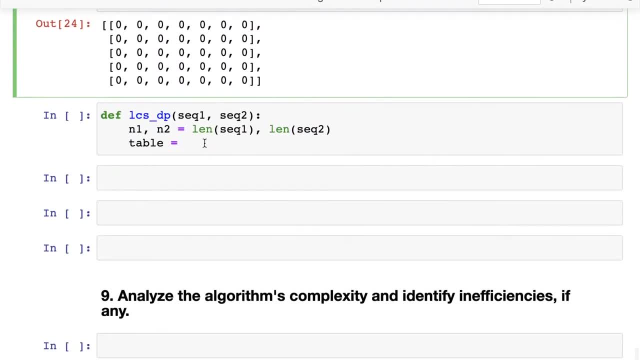 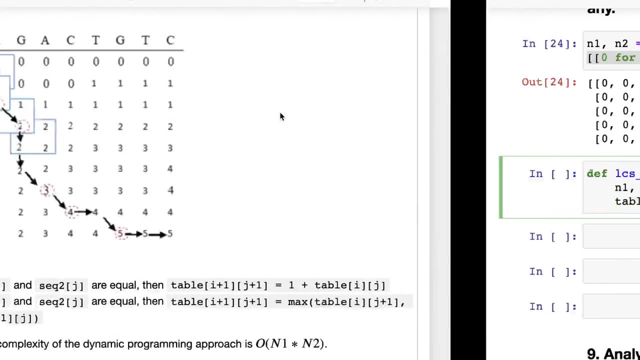 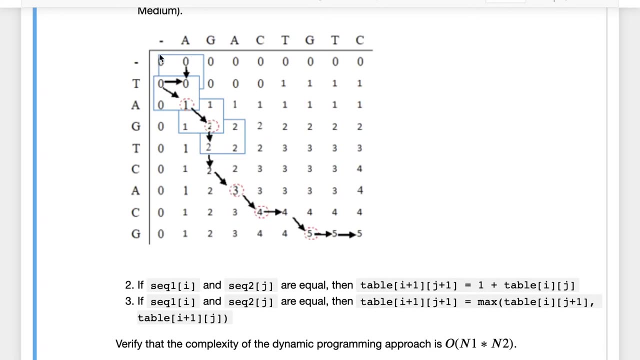 One, two, three, four, five, Six, seven. So this is the table that we want to create initially. Okay, Now there's a table that we've created. This is going to be this exact same table, And we're simply going to start each string from position one, this time, not from position zero, because we want to have this additional row where we don't consider either of these. that just makes computations a little easier. 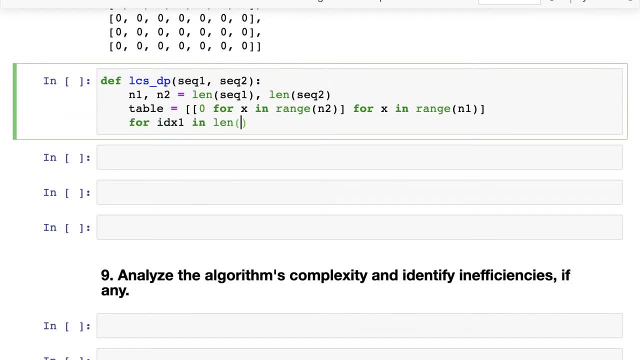 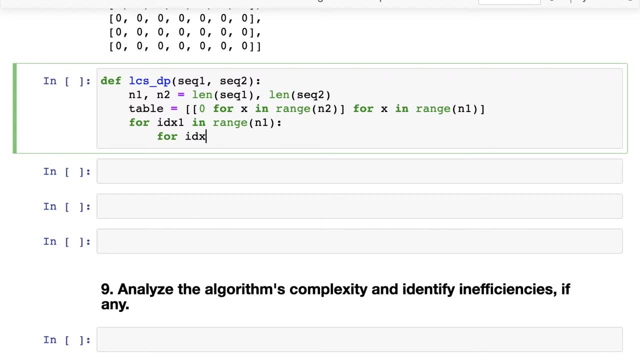 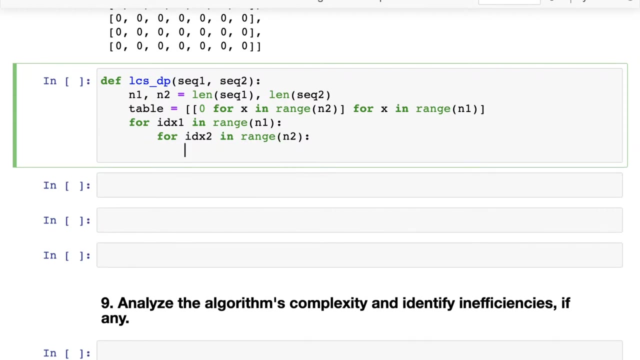 Now we say for IDX, one in Len addicts, one in range and one. So that's, that's going to iterate over the rules. and then for IDX true, in range and two, and that's going to iterate over the columns. And first we compare if sequence one of IDX one is equal to sequence two of IDX two. if they're equal, then we can fill out table of. 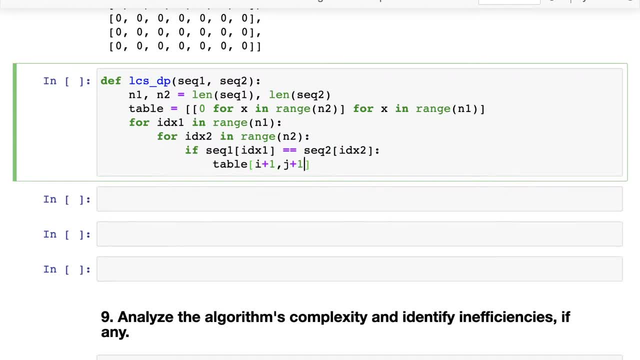 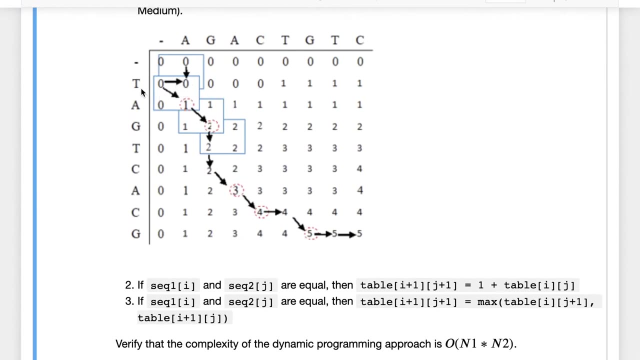 I plus one and J plus one, as one plus able of IJ. Okay, And we can see this. we can see this here. Suppose the first elements were equal. So suppose this will suppose IDX one was zero and IDX two was also zero. 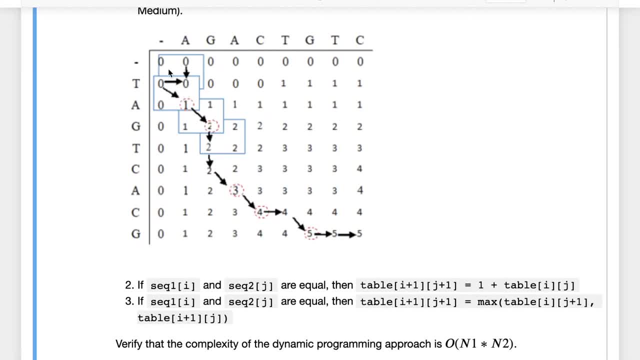 Suppose they were equal, then this value should be one. So this value should be one plus the diagonally top element, and that holds true Anywhere Within The list. So wherever you have two elements equal, like G and G are equal here. 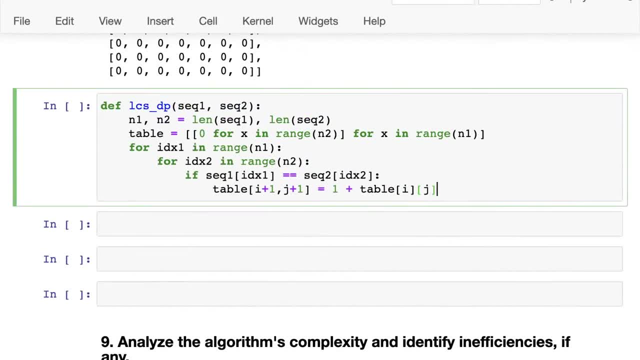 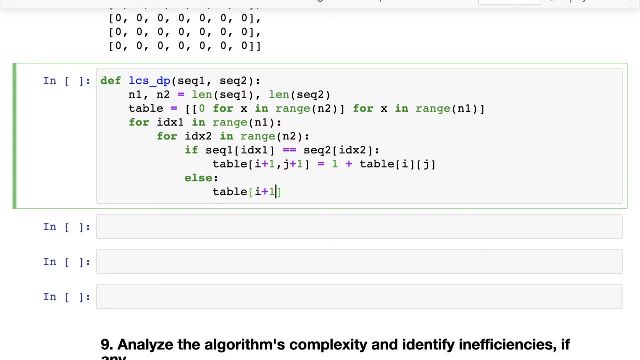 So this value is one plus this value, Else we have table I plus one and J plus one is max of able I come a J plus one. So you stay in the same row or you you go to the previous row or you go to the previous column which is table of I plus one. come on G. 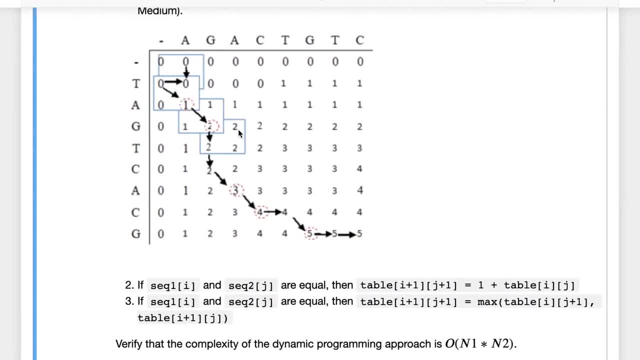 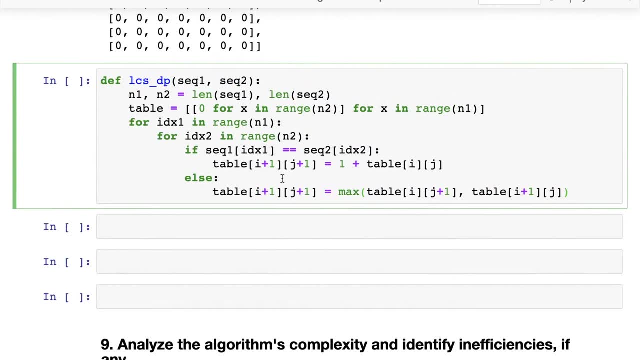 And this is the previous column. Okay, So this is this case where G and air not equal to GNA are not equal, Then we take the maximum of these two values and that's it. That is going to fill up the table for us. 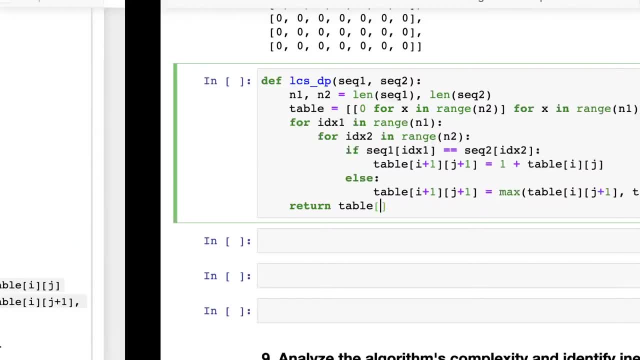 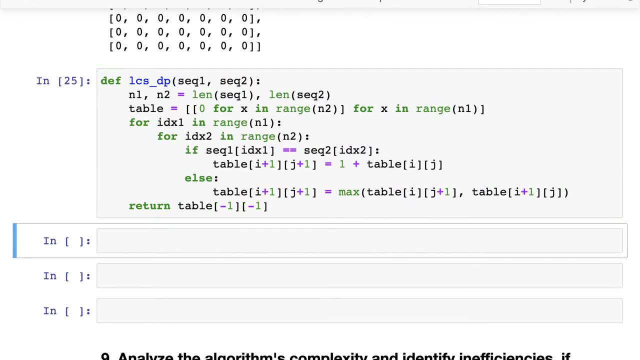 And then we simply say: return able. We simply want the bottom right element, So we can simply say: return table: minus one, minus one. So this is going to get that last row, last column, And that's our dynamic programming solution. Let's do evaluate test cases here. 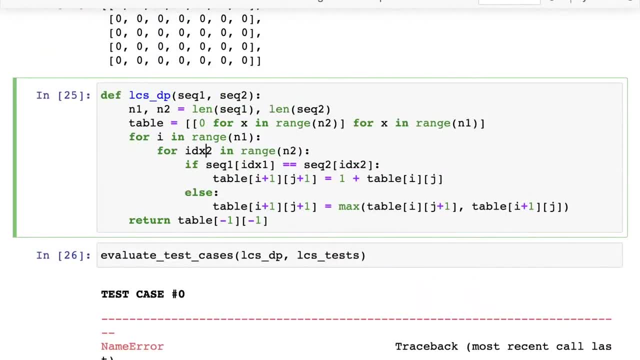 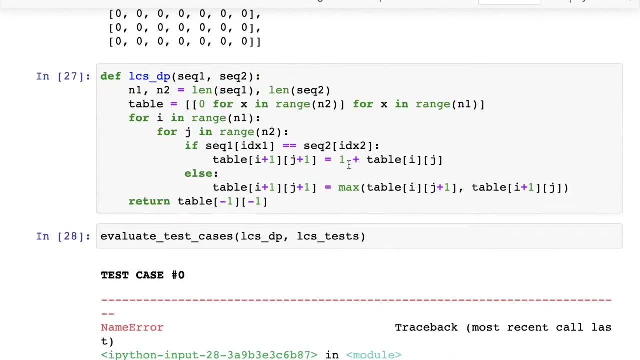 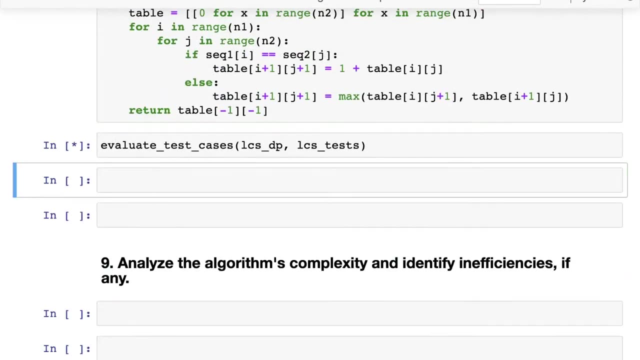 Okay, It turns on. So there's no I. okay, let's just call this I and J IDX. one is not defined. Let's just make these INJ. now that we're doing this coding live, You can see that even after a decade of coding, I still make all of these issues. 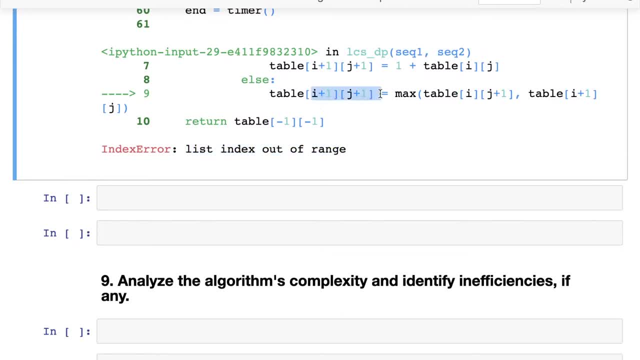 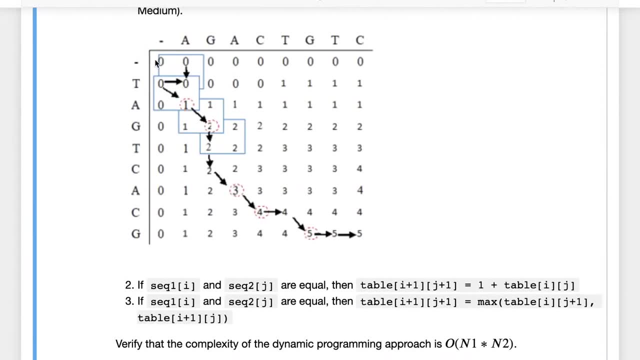 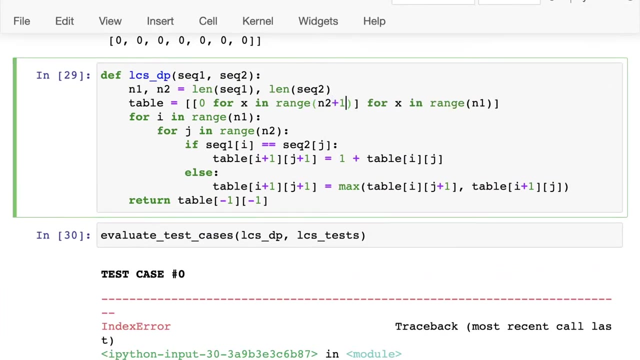 It says the list index is out of range. It seems like I plus one and J plus one. Oh, that's because, So remember, we need an additional row and an additional column to track the case where either of the strings is empty. So we need to get range N two plus one here, and we need to get range N one plus one here. 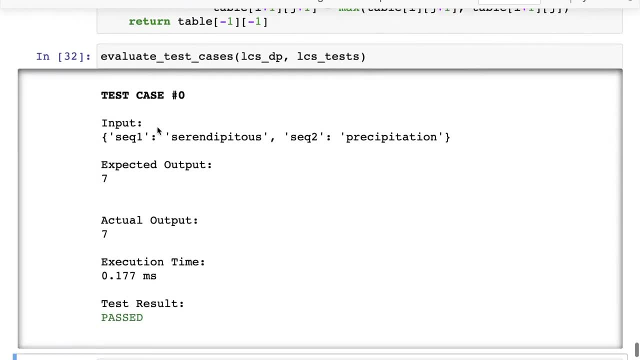 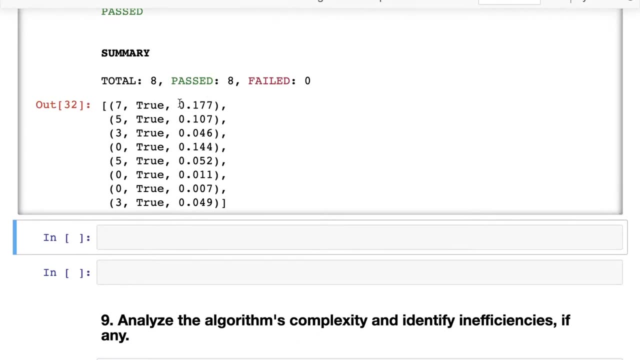 Okay, And that's why it helps to have test cases, so that you can fix all of these issues. Now you have test case zero- it passes- and test case one, two, three- all of them pass. You can see that all test cases have passed and you can also verify that the amount of time it took is now lower than the amount of time. 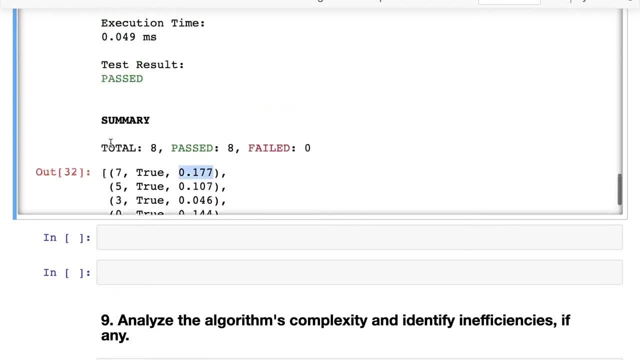 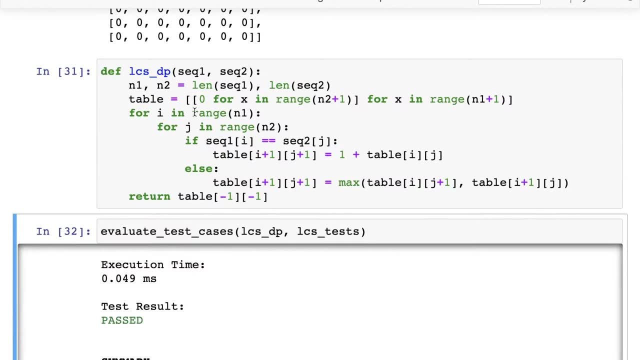 You can also verify that the amount of time it took is now lower than the amount of time it took for memoization, and so that's the dynamic programming approach: You simply create a table and you fill out the table, but sometimes just working with indices within the table can get confusing. 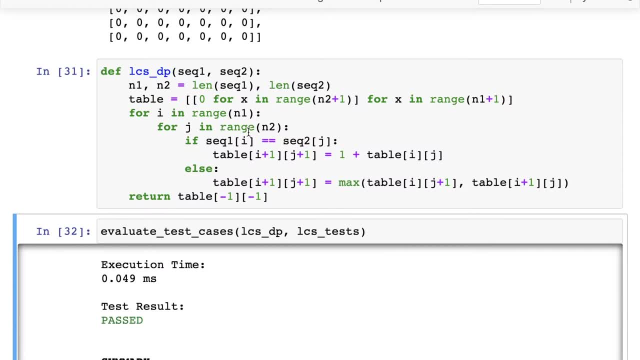 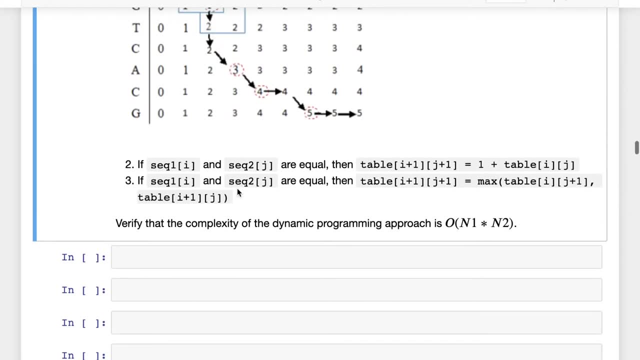 So it helps to work with it on paper and make it clear to yourself and then write it in English. That's why we've written it in plain English here And now. an exercise for you is to verify that the complexity of this dynamic programming approach is. order of N one times N two. 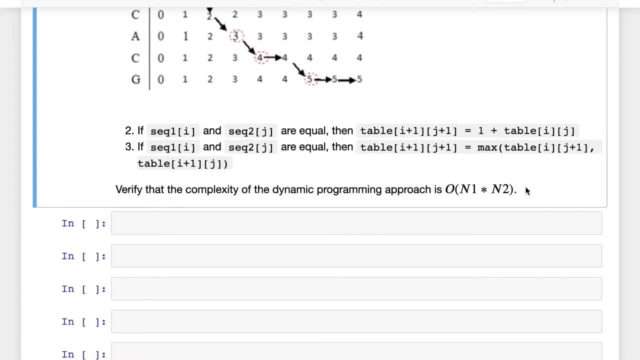 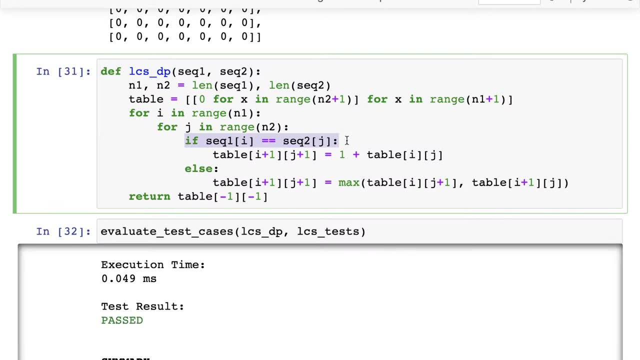 So, which is the same as memoization, And it's actually more straightforward to see here, because you have two for loops and then each of these for loops. you are simply doing a comparison and an addition And there's not even any recursion to very, very there's not even any recursion for you to vary or worry about. 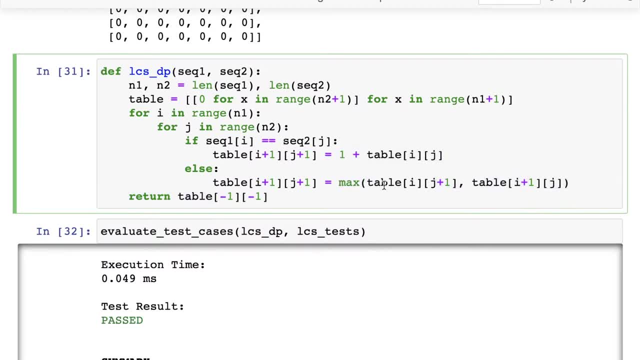 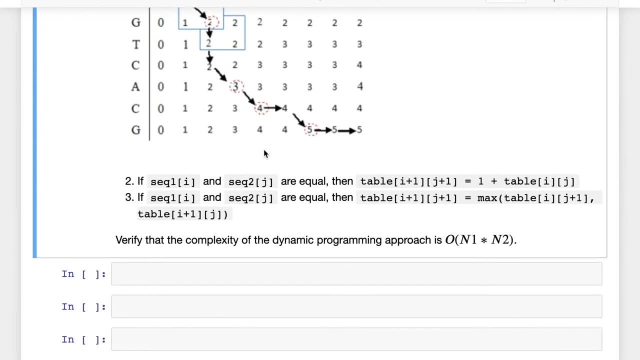 So you just do a comparison and you do an additional, you take a maximum pretty straight forward to order, of N one times N two, and it does not even invoke an another function. So it does not take up too much memory, It does not take up too much time. 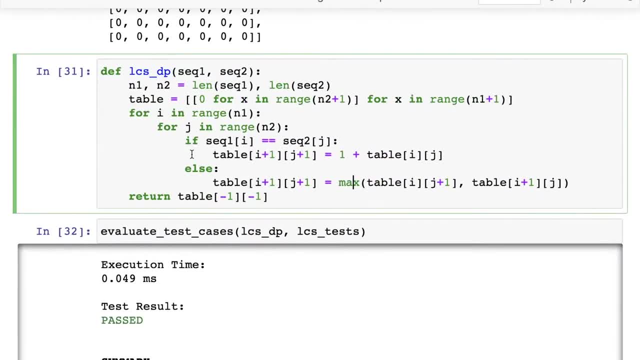 It's very, very efficient, And this is how you solve pretty much every dynamic pro dynamic programming problem. You write a recursive solution, You come up with the brute force solution, and keep in mind that recursion is Almost always the way to go about creating a brute force solution. 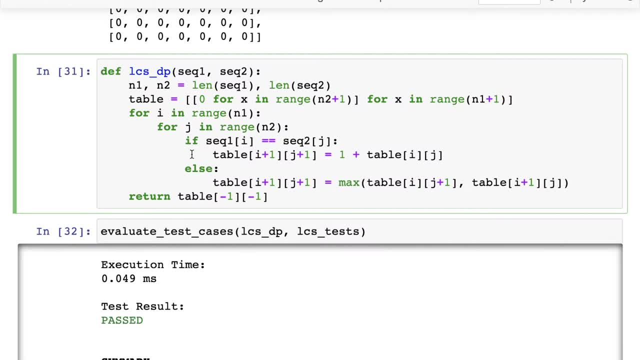 So you come up with a recursive solution and then you identify, you draw the recursion tree And if you see that the same sub problem is being called again and again, that is a point where you can introduce memoization. So you introduce memoization and sometimes you can just write the memoized solution. 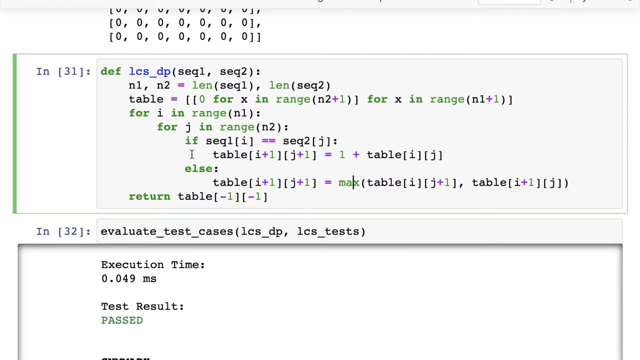 And that's enough, because it's easy to reason about. You just put in a memo and you're done with it. Um, even the interviewer or the coder Or the coding assessment will accept that solution. but in some cases you will be asked to then remove the recursion and write it as a in an iterative fashion. 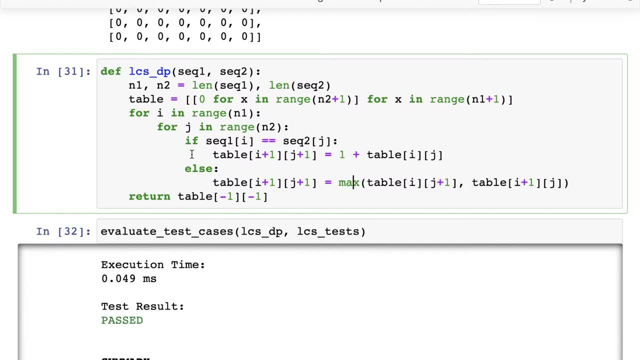 And that is when, then, you have to start drawing a table and think about what are the rows and columns in that table need to represent. So here, the IJ element of the table represented the first, the first I elements of sequence one and the first IJ elements of sequence two. what is the longest subsequence between them? 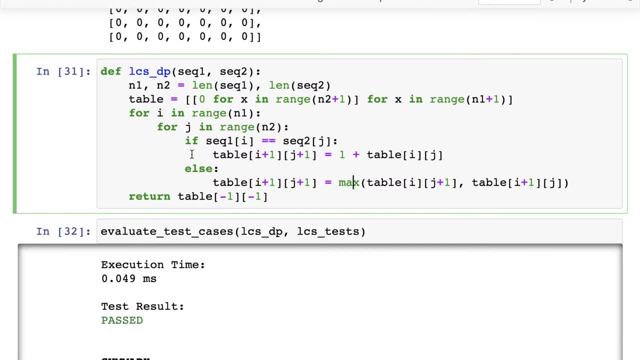 And we use that to build the next, Next column, And we then filled out the entire table and we simply use the last value. Now, again, this is not very straightforward. uh, how to come up with this, And the way you do that is by solving problems. 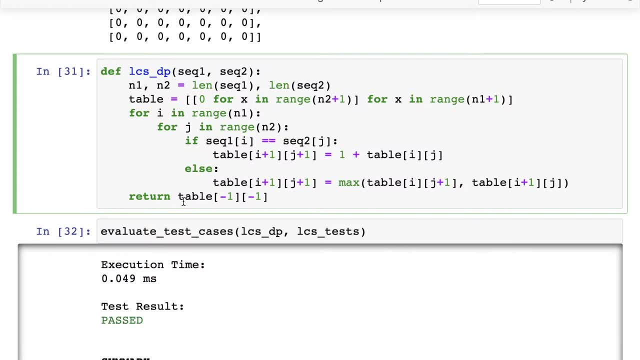 If you solve five to 10 dynamic programming problems, you will get some intuition about how to build the tables, And it's always always very helpful to solve it on pen and paper first, especially with dynamic programming, so that it's clear to you. 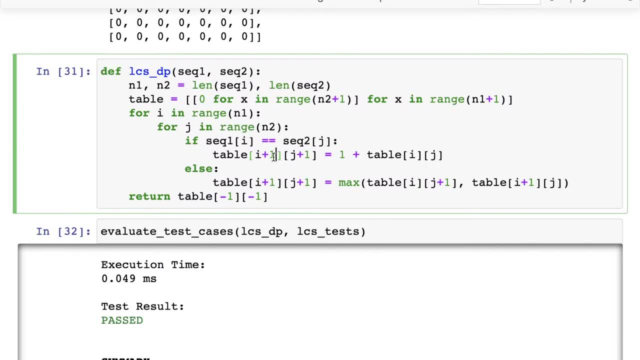 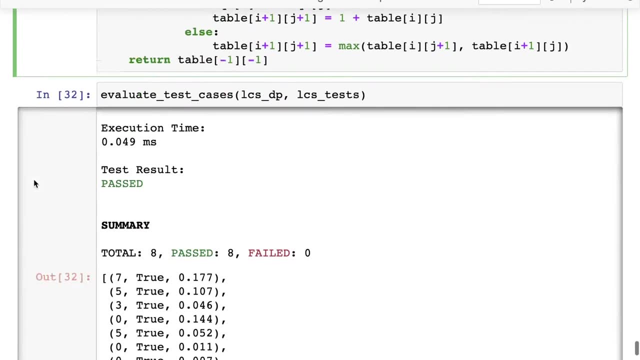 What each element Of the table represents. Otherwise, you may make a lot of off by one errors like missing the plus one here or missing the plus one here, and get confused, just like I did pretty much. And that's the time The time. complexity is pretty straightforward. 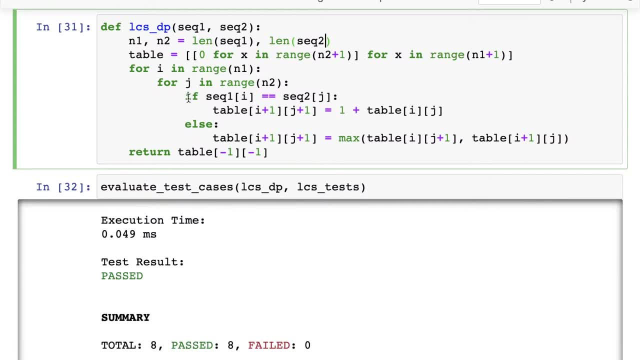 In most cases it is simply the size of the table, but sometimes you may have to do more than constant work here to keep that in mind. see what it is that you're doing inside your loop, inside of inside your loop, If you have to go back and check the entire length of the string. 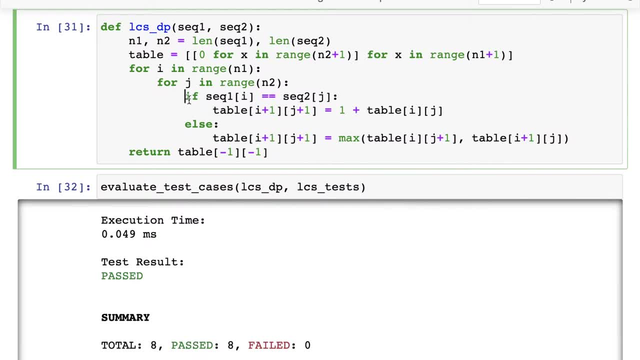 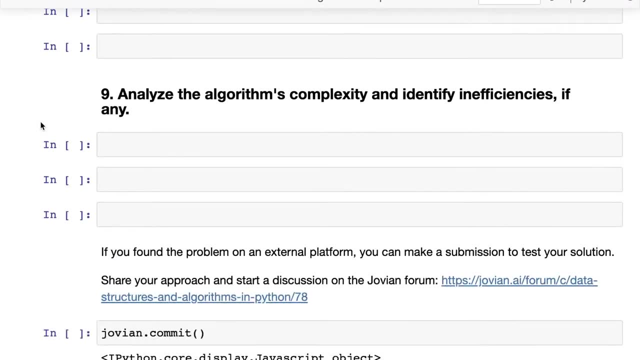 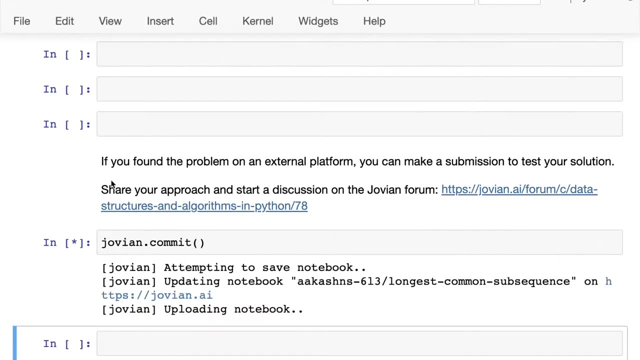 So that will introduce Another factor into the equation. So keep that in mind. but in most cases, counting the iteration should be good enough to give you an idea of the time complexity. Okay, So that's the first problem, And let us just commit this- and now it's saved- to my profile. 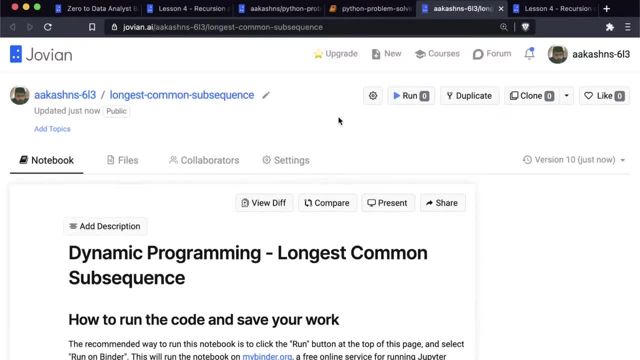 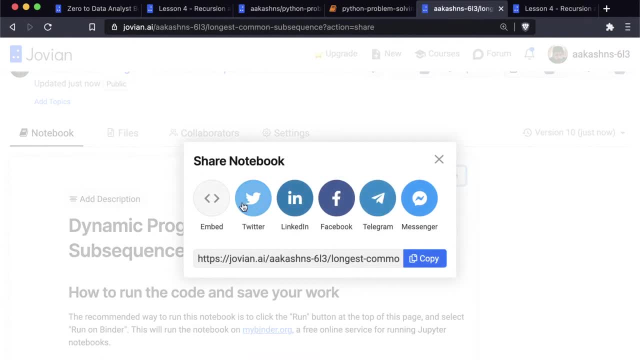 If I just open this up here, you can see that now I have this notebook, or longest common subsequences, And I can share it online. Whenever you work on a notebook, it's always a good idea to make it public. put it up on Jovian. 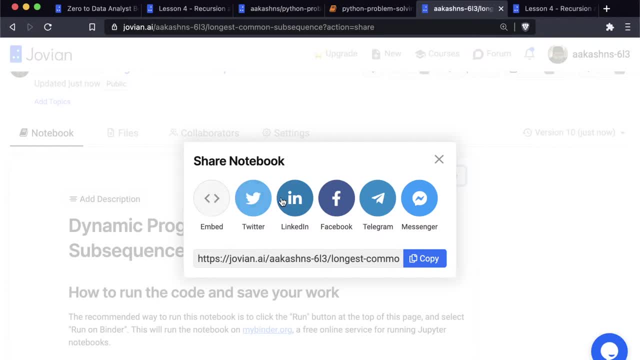 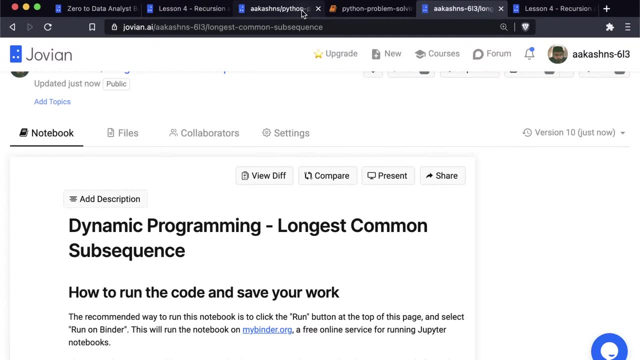 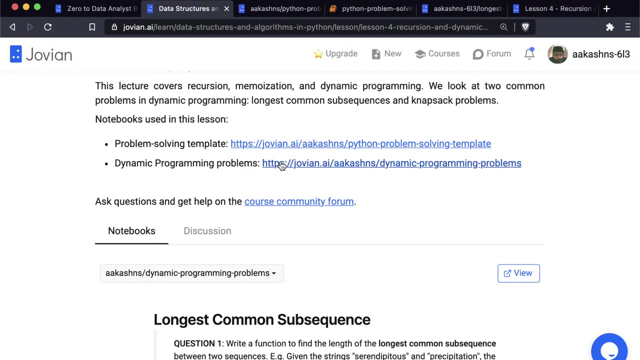 All you need to do is run Joviancom and share it online. Just press the share button and then you can share it on Twitter, LinkedIn, Facebook or whatever you like. So that's the first problem that we looked at. Now let's come back to listen for- and, by the way, the problems that we're talking about, all the problem statements, the graphs, the images. 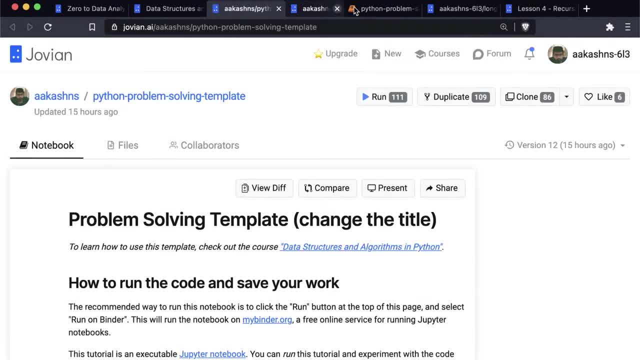 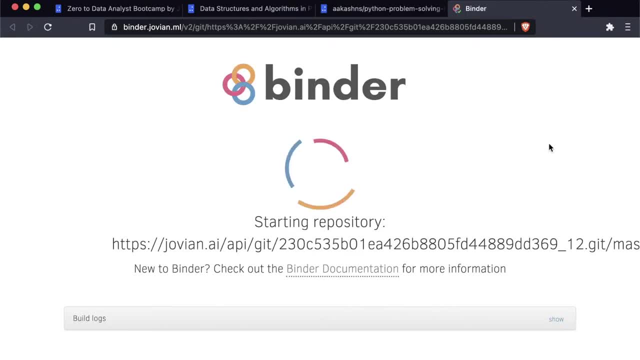 You can see them in the second link here, but we will. We can open up the problem solving template and now we'll use it for the second problem. Let me run this once again. we're going to look at the second problem, which is the knapsack problem. 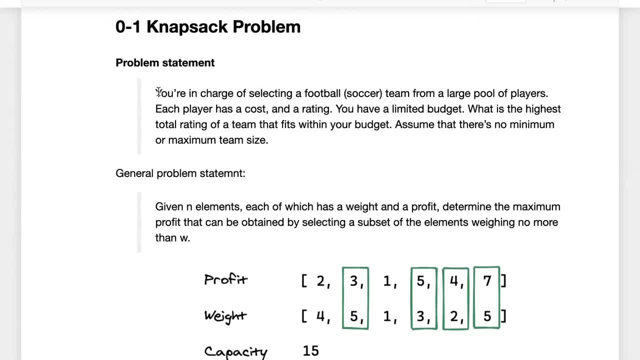 So let's read the knapsack problem. It's also called a zero one knapsack problem. Here's there are many variations of this problem, but here's one way to state it that you might come across, or something similar. So you are in charge of selecting a football or a soccer team from a large pool of players, and each player has a cost and a rating. 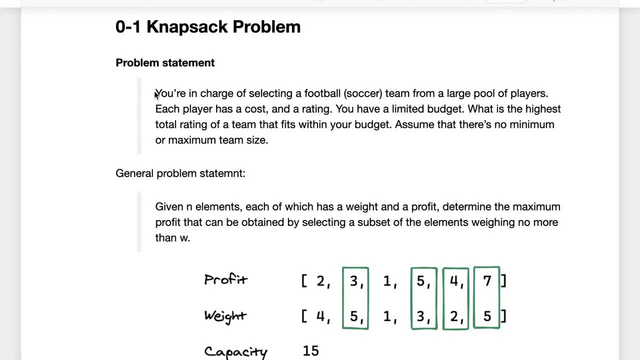 So there's a selection going on. You have to come up with a team for this year and you have a large pool of players. Each player has a cost and each player has a rating. Now you have a limited budget, so you need to build a team within the budget. 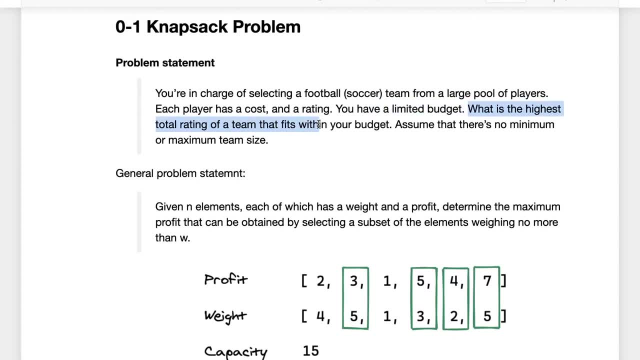 So what is the highest total rating of a team that you can create which fits within your budget? So this is the question: here You have to maximize the total rating but fit it fit the total cost within your budget. We have two variables here: rating and variables. 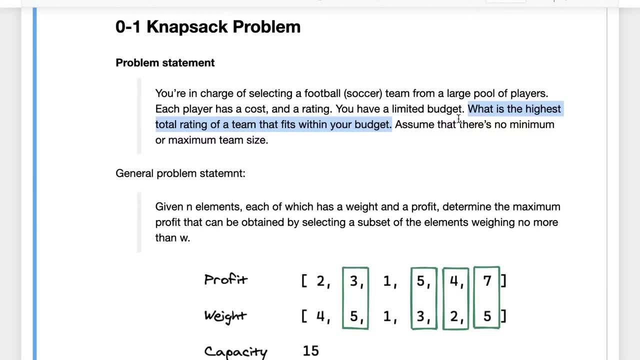 Rating needs to be maximized. Cost needs to be simply optimized to the extent that it fits in the budget, And this is simplifying. assumption here is that you can assume that there is no minimum or maximum team size. This is simplification, And later you can introduce a criteria there as well, that you want to build a team of exactly 10 people and see if. 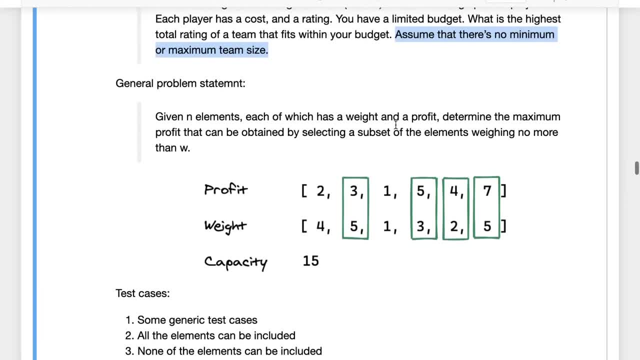 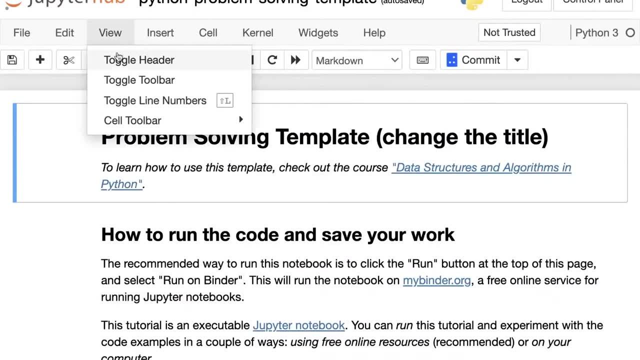 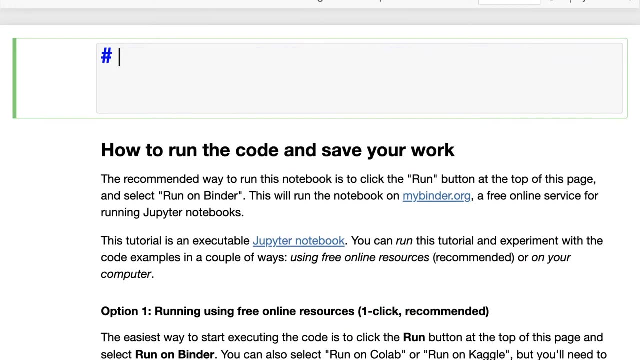 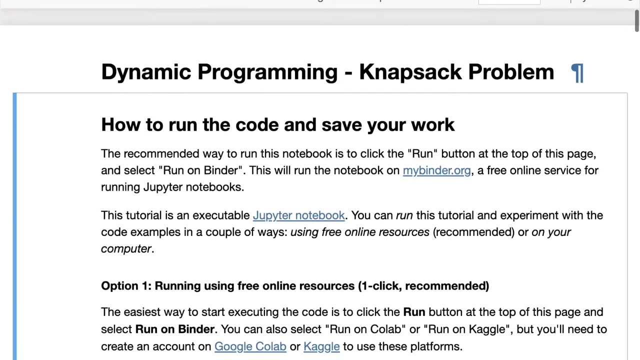 you can also solve that problem in a way. So that's the knapsack problem. Let's copy it over. And here's a Jupiter notebook, a fresh problem solving template. Let's simply change the title. here It is also called the zero one knapsack problem, because each item can either be chosen 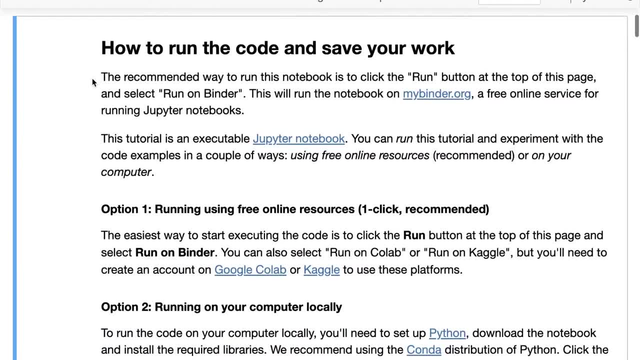 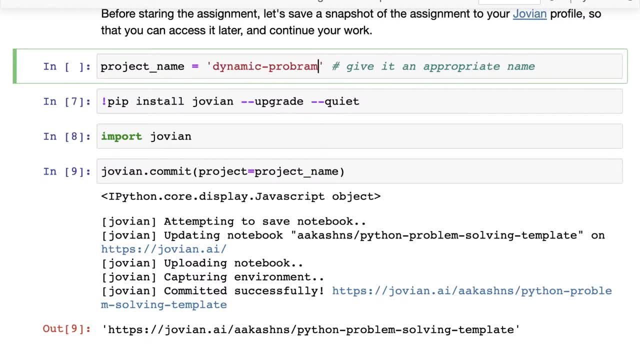 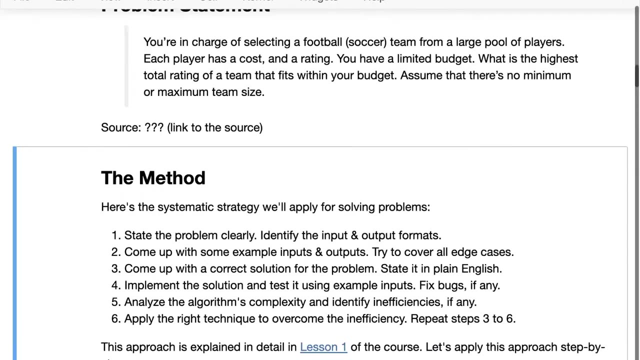 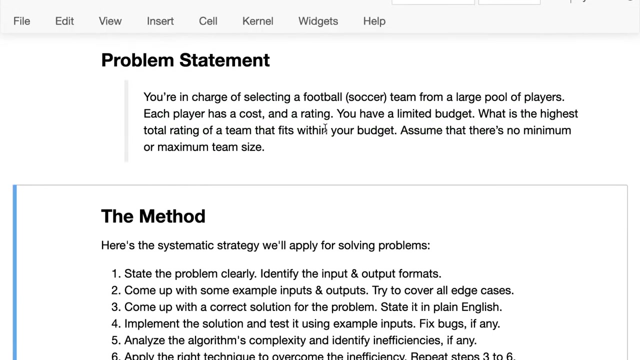 Or not chosen, and let's give it a project name here to let's commit it and let's paste the problem statement here, Okay. So that's a problem statement, Okay, And this is a specific or a special form of a more general problem statement. 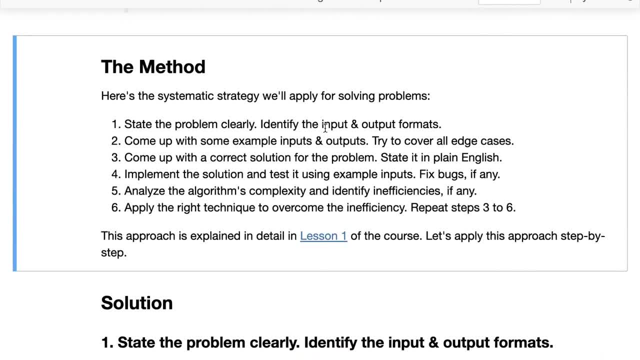 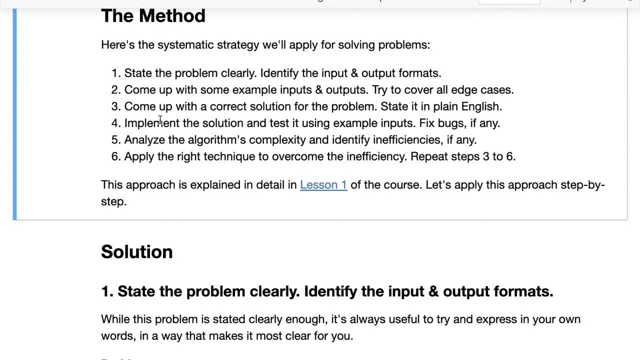 And we look at the general problem statement in a second when we try to state the problem clearly. but here's once again the systematic strategy we'll apply: we will state the problem clearly, identify the input and output formats, come up with some example inputs and outputs and try to cover all the edge cases. 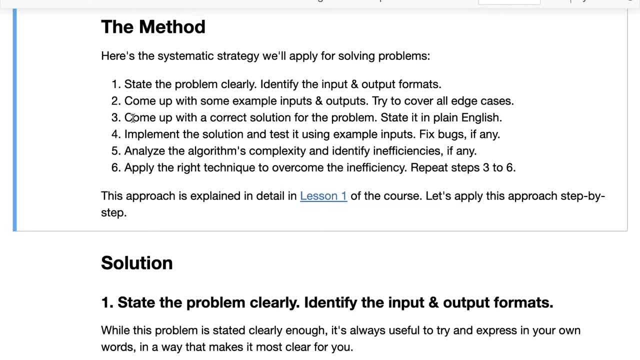 Then we will come up with a correct solution for the problem and state the solution in plain English. It just has to be simple, correct solution, Not too complex. Then we apply the right technique to overcome the inefficiency And then we so we analyze the algorithm and identify any inefficiencies after implementing the solution. 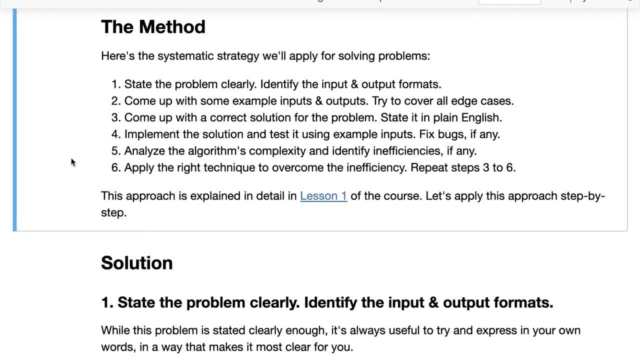 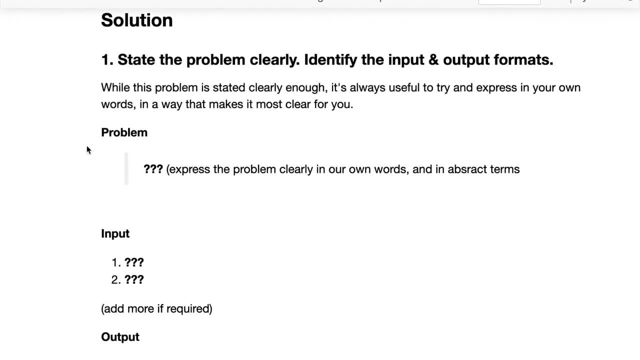 And, finally, we apply the right technique to overcome the inefficiency and then repeat the process of stating the solution, implementing it and analyzing it. So, to state the problem clearly, what we can do is we can abstract on the problem in more general terms, 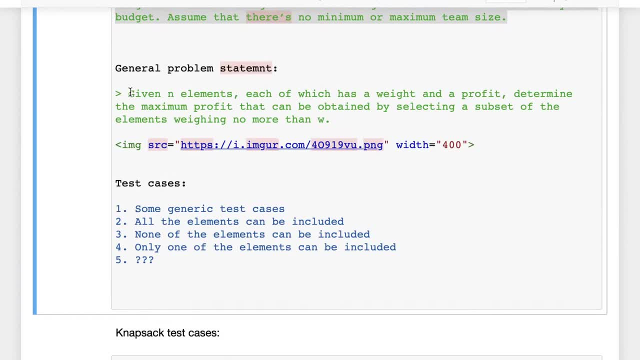 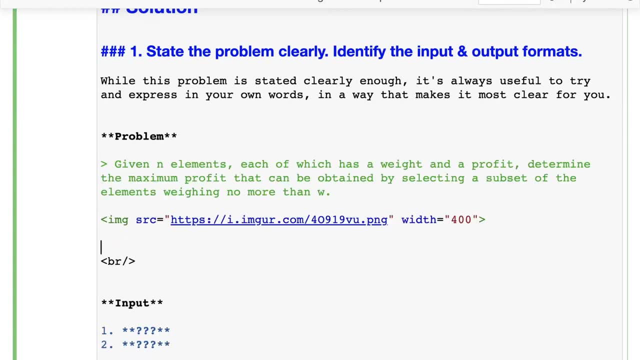 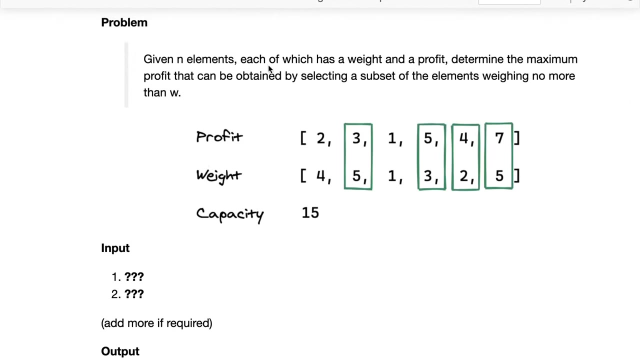 And that is what is stated here. So let's take a look at the problem and state the solution in plain English, and let's just grab that and we'll take a look. So here we have. we are given N elements, and each of which has a weight and a profit. 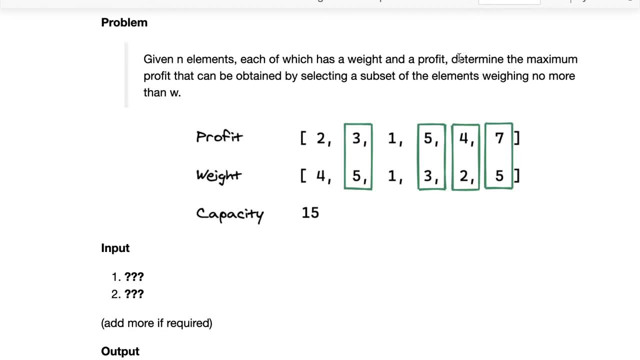 So you have N elements and here's the profit of each element and here's the weight you can of each element. So you need to determine the maximum profit that can be obtained By selecting A subset And a given weight: W. So you have a capacity, a maximum capacity. 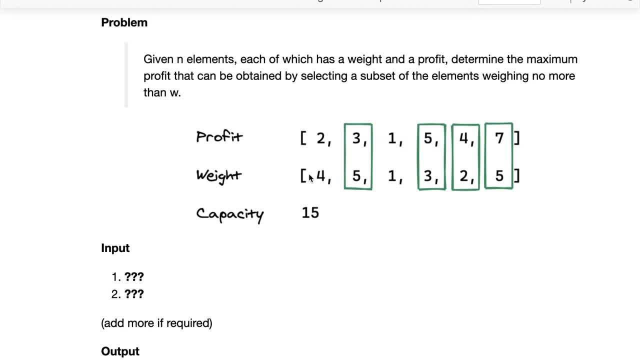 Let's say the maximum capacity is 15. And you have to select certain elements so that you fill out. the total rate is no more than the capacity and the total profit is maximized. That's, and this is why it's called the knapsack problem. 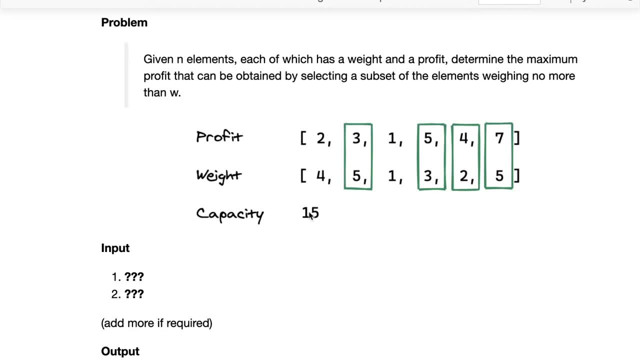 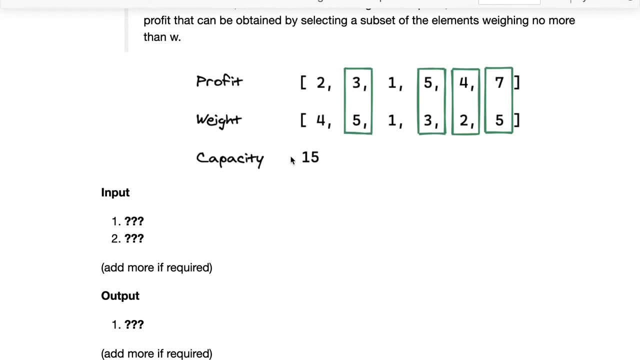 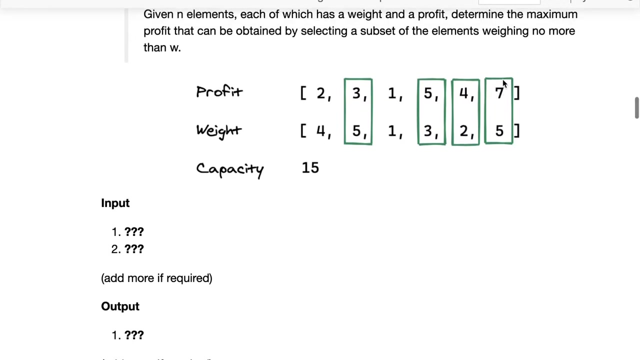 It's assuming, here you have a bag or a knapsack with a capacity of 15 kilograms and these are the weights of the items And these are the profits. Now, in this case- you can see in this example- The optimal selection is these four elements, which are the weights: five, three, two and five, so that you fill out the total capacity of 16 or 15 and the. the solution on the maximum profit that you can obtain is seven plus four, 11 plus five, 16 plus three, 19.. 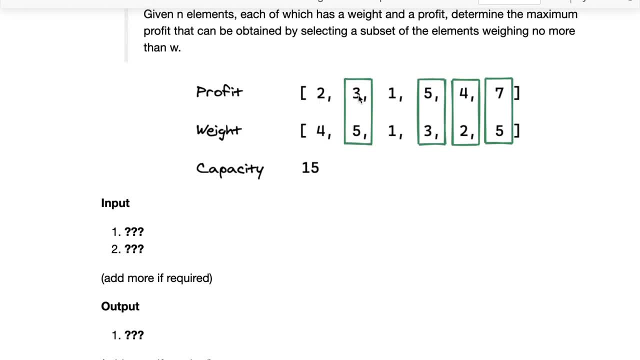 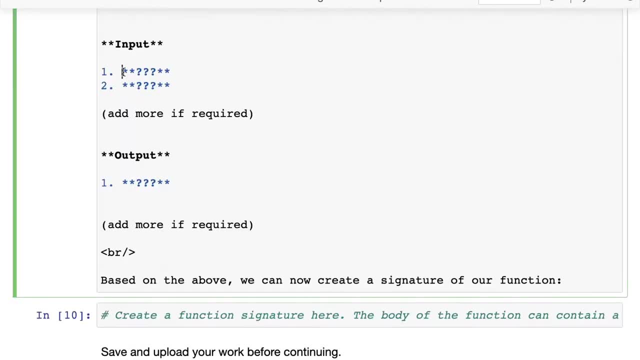 Now you can try other combinations and verify that this is actually the best solution. Do give it a shot. So what are the inputs here? So we have- it's pretty clear We have- an input: weights. So these are the weights of the. this is a list of numbers containing weights. and then you have profits- a list of numbers containing profits, and this should have the same length as weights. 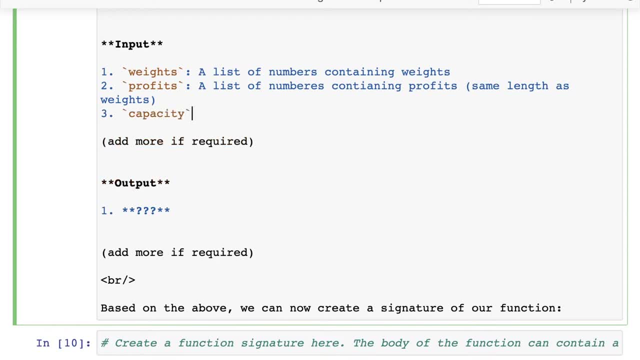 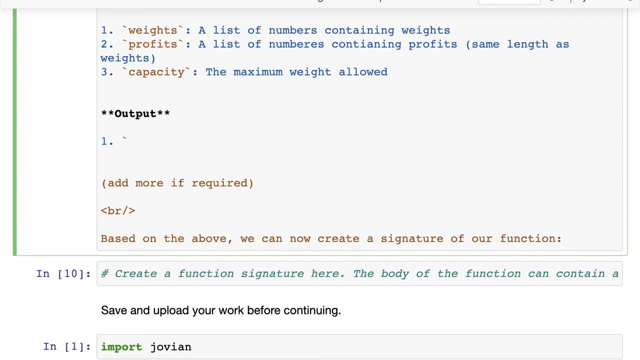 And then, finally, you have a capacity. So this is the maximum weight allowed. And there you go, And now we have outputs. So now the output would simply be the max profit. This is the maximum profit that can be obtained By selecting elements. 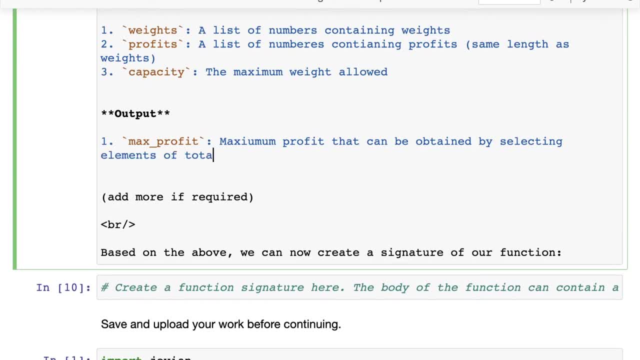 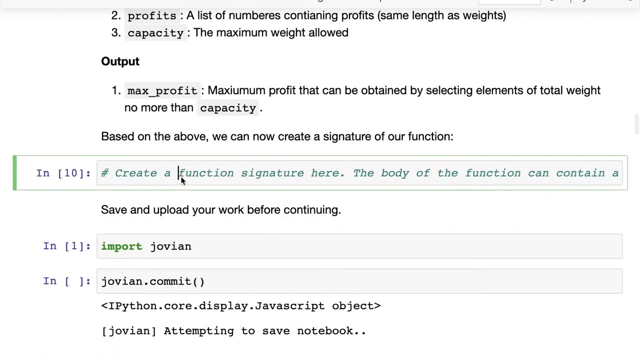 Of total weight, No more than W or no more than capacity. Okay, Great. So that gives us a pretty good starting point. Now we can write a function signature here. So we write max, Let's say def, max profit. Okay, 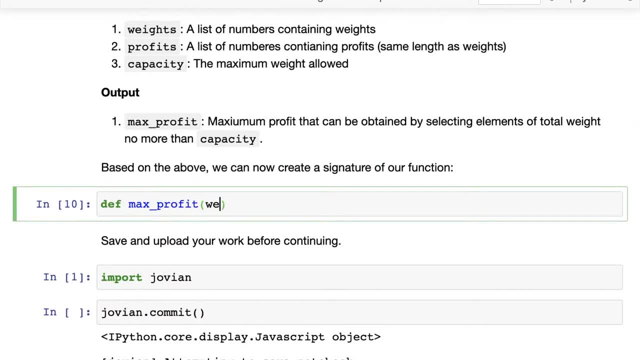 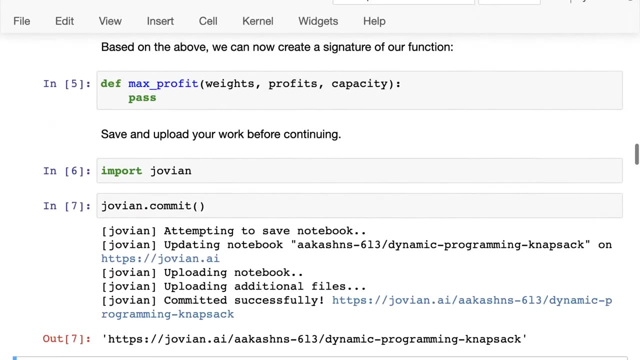 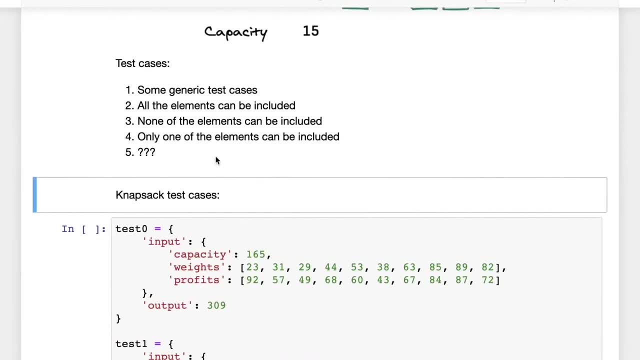 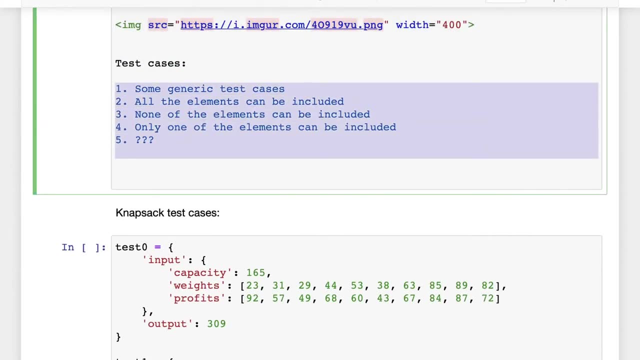 Now we need to come up with some example, inputs and test cases. Once again, we have listed out a few test cases here, but we will have a few generic test cases where you just a random set of weights and profits and you identify the knapsack, the optimal solution. 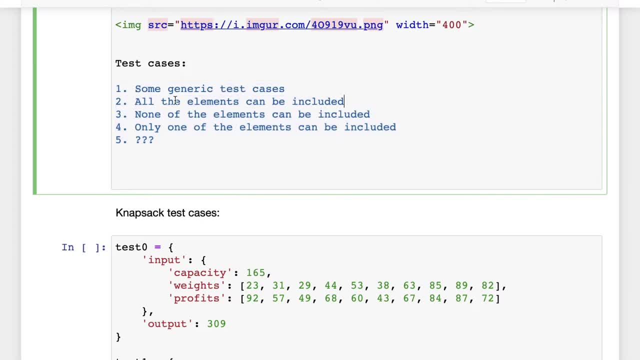 Then here's one option where all of the elements can be included. You can take everything. Here's another option where none of the elements can be included. You have to think about all these scenarios. Here's one where only one of the elements can be included. 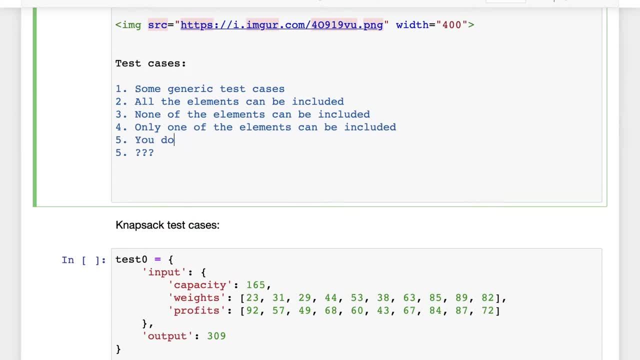 Then you may also think about areas where you do not use the complete capacity. Okay, You do not use the complete capacity because the optimal solution is actually taking a lower capacity. So there may be a way to fill out to capacity, but that may have a lower profit than another option which? 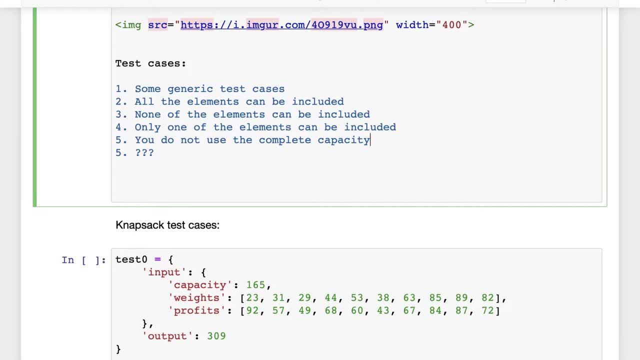 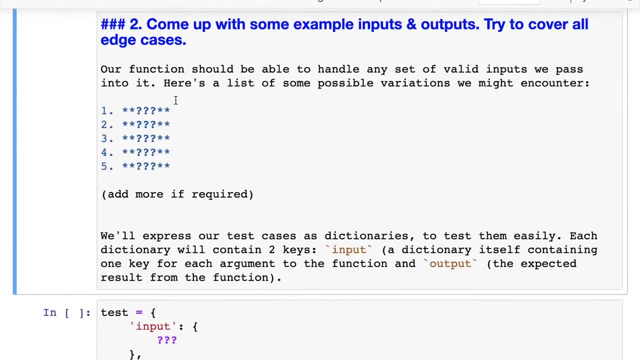 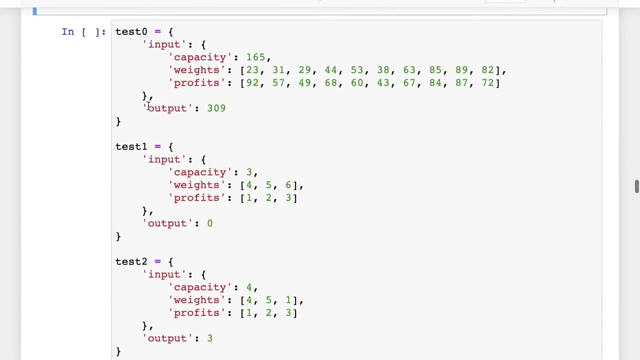 takes less than the complete capacity but has a higher profit. So think about some cases here, think about some good test cases here, and I will just copy over these for now, And then what we'll do is we will express these test cases once again as 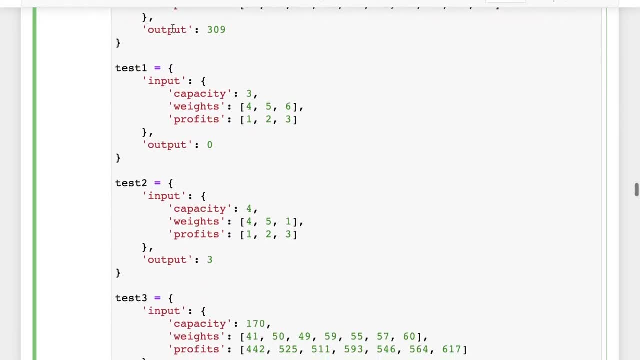 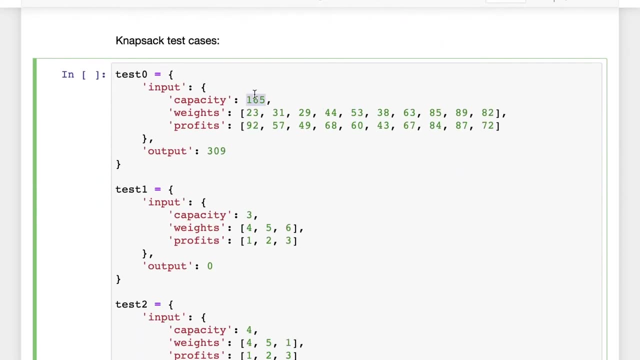 I mentioned dictionaries. we have test zero, test one, test two, all of these express and dictionaries And these are covering all the test cases that I mentioned here. You can see here are some weights and some profits and the capacity is one, 65.. 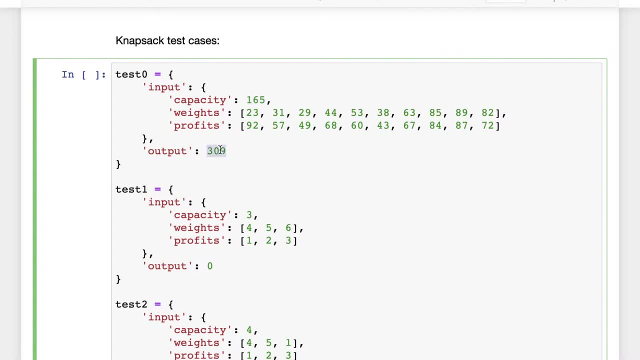 And then the optimal solution is three zero nine. Now we are simply asking here for the optimal solution, the maximum profit that can be obtained, But an extension of this problem is to identify which are the elements that should be chosen, And it's a simple extension. 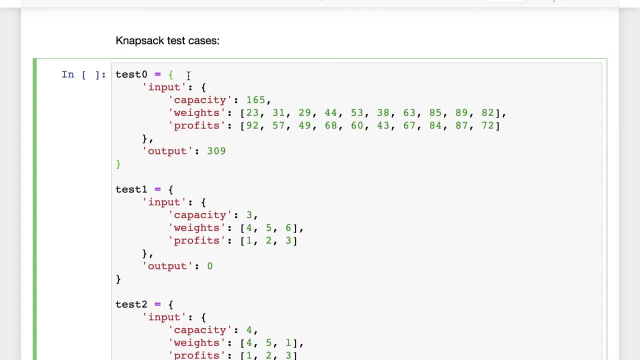 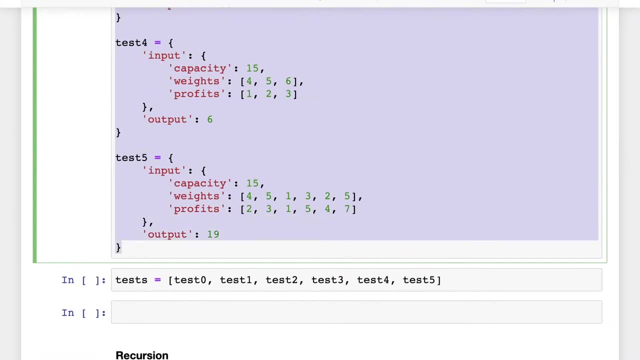 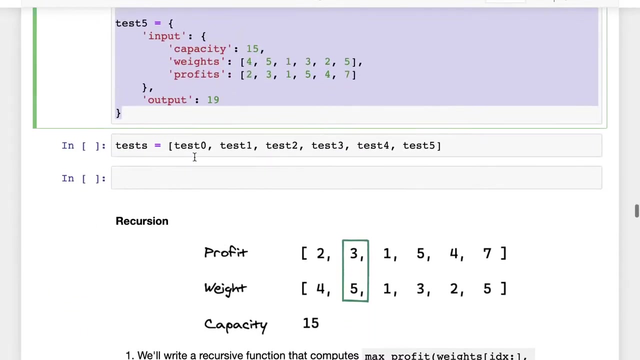 It's a good exercise for you to try out And you can discuss it in the forums. We have test zero, test one, test two, test three and four and five. So we have a total of six, six test cases. Let's copy over these test cases here and let's put them here into a single string. 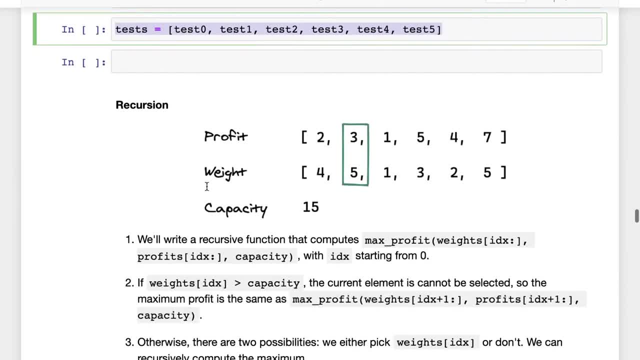 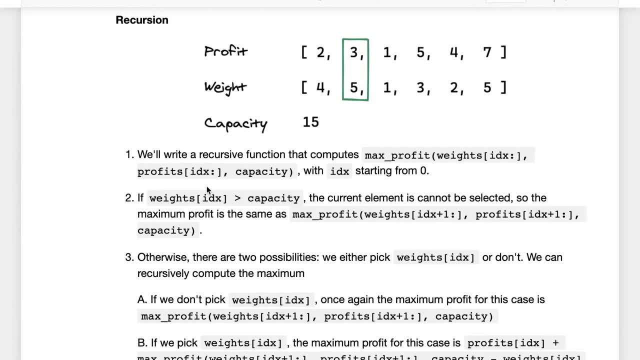 And that gives us the test cases. Okay, Now coming up with a solution. So, once again, the first step is to try and come up with a recursive solution, And a recursive solution is, again, quite straightforward. We'll write a recursive function: max profit that given an index. 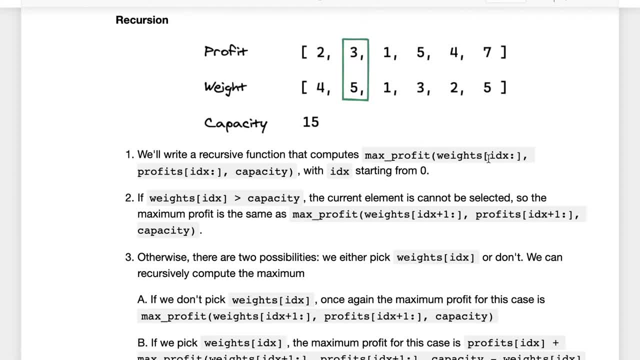 So this time we have just one sequence. So given an index within the sequence, so let's say you have an index IDX, it computes the maximum profit that can be obtained using the elements from IDX onwards. So three, one, five, four, seven using all of these elements, IDX onwards. 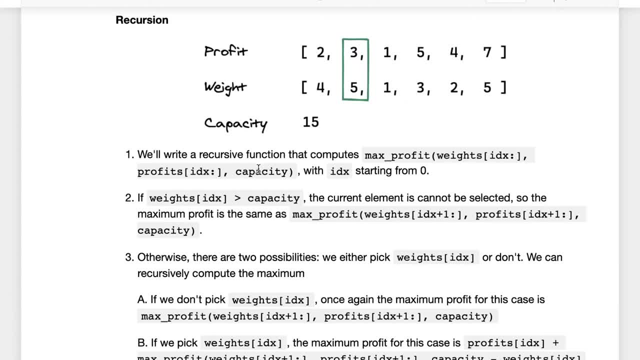 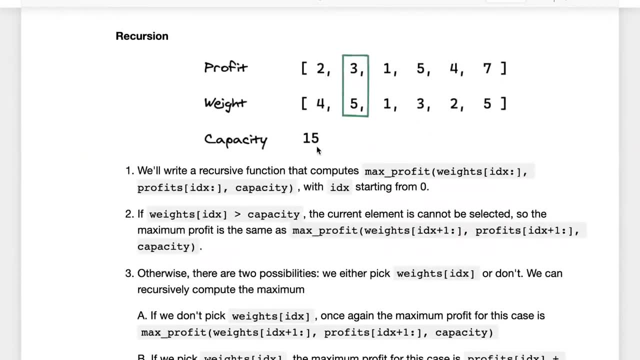 The maximum profit that can be obtained right And using a given capacity. So it will take an index, So it will take an index and a capacity. So if let's say the IDX is one, so it will then look at just these elements and have the capacity is 10.. 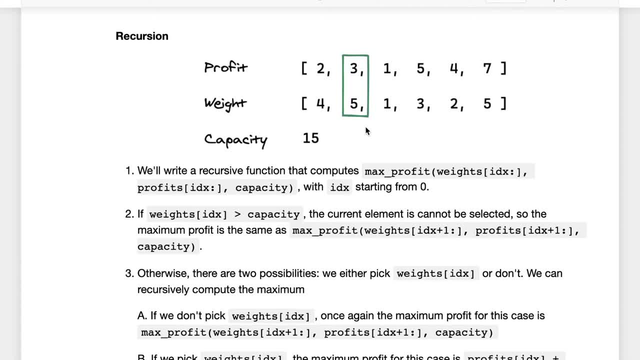 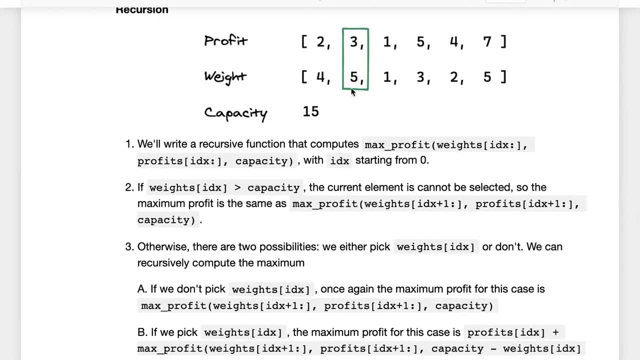 So it will try to fill the capacity of 10, and that's the recursive function. And why are we creating a recursive function like this? There's a simple reason. Now suppose IDX Has the value one and the capacity is 10, or let's say, the capacity is three. 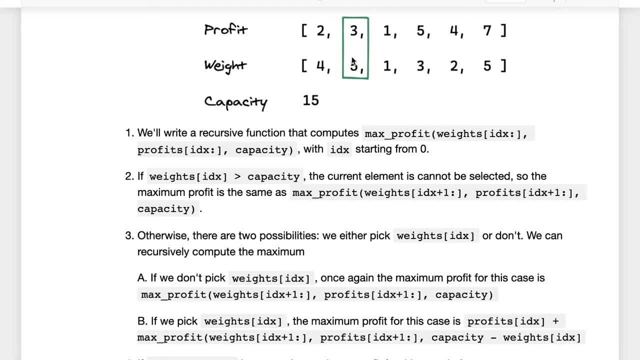 Then the weight of this element is greater than the capacity, So that means it cannot show up, It cannot be selected because it cannot fit inside the bag, the knapsack that we have. So then the solution for this sub problem with IDX equal to one and capacity equal to three is same as the solution for this sub problem. 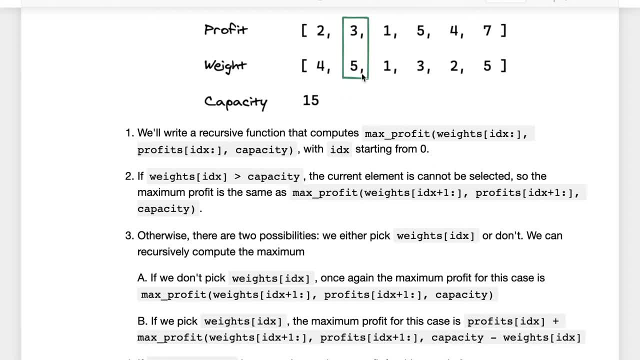 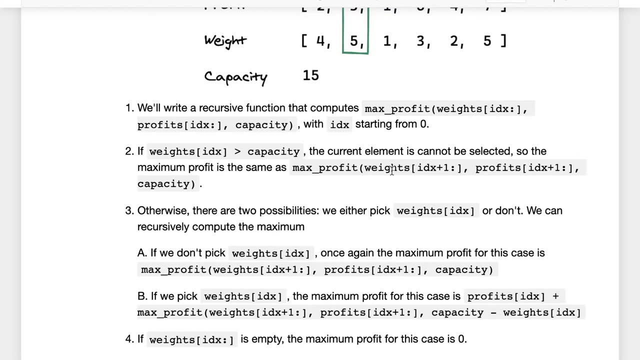 with this element removed because you cannot include this element within the knapsack, right? If you remove this element and simply consider these elements, the remaining elements, which essentially means IDX plus one, So max profit of IDX plus one, profit of weights, IDX plus one, profits, IDX plus one and capacity is the answer. or max profit of weights, IDX, profits, IDX and capacity, because the current weight five is greater than the capacity. 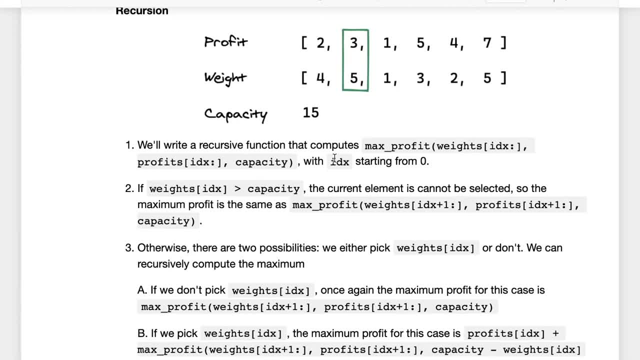 Three, Which is which the recursive function has been invoked with. So that's one option. but the more general case is that you have enough capacity. So let's say you have a capacity of 10, recursion was called with a capacity of 10 and you are at IDX one. 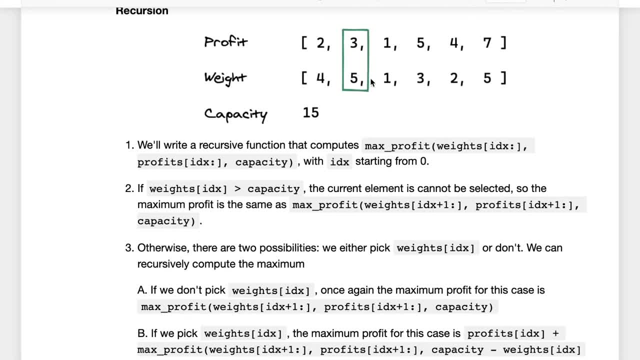 So then you have two choices: Either you include this element in your knapsack, or you do not include this element in the union option, because you don't know whether the optimal solution will have this element or not. So you try both. So there are two possibilities. 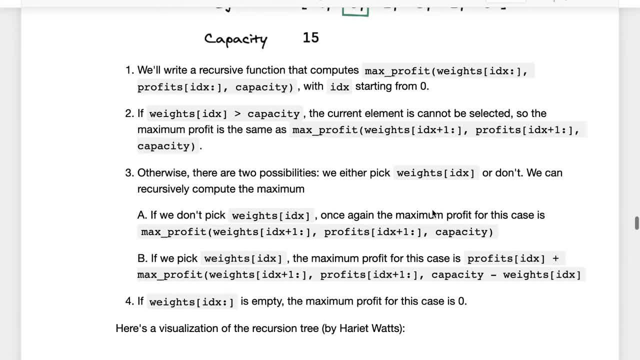 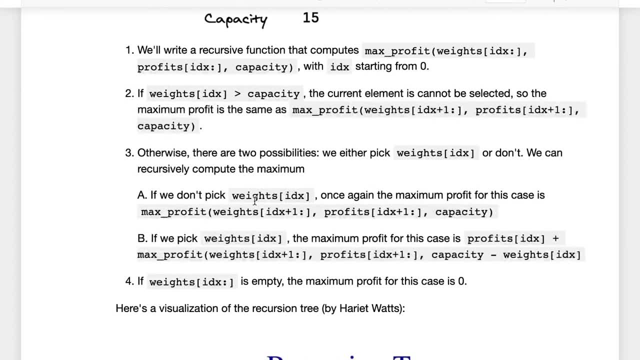 We Either pick weights IDX, this element, or we don't, And what we can do is we can simply compute the result in both cases and pick the maximum. So if we don't pick weights IDX, then once again, if we don't pick this element, so the capacity remains the same. 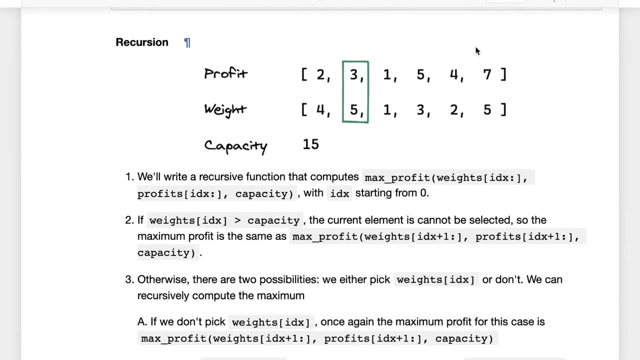 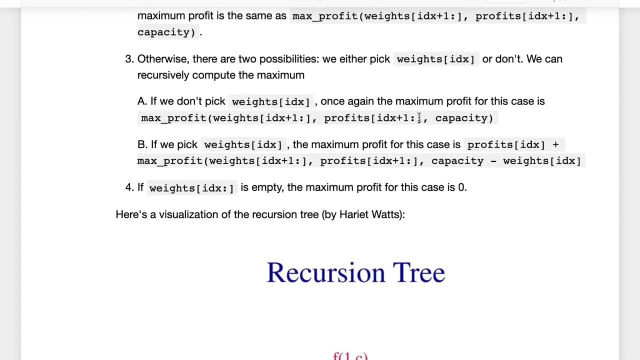 Let's say the capacity was 10.. So we simply try out to fill out the capacity of 10 using the remaining elements. So we simply call max profit with weights: IDX plus one, profits IDX plus one onwards and the remaining capacity, which is 10.. 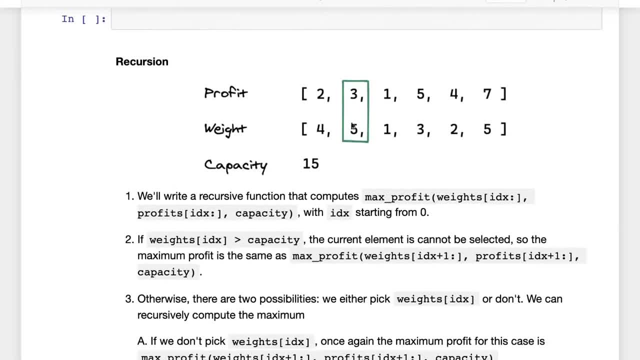 But if we do pick the element, if we pick the element and we had a capacity of 10, then the optimal, then the solution, the best solution in this case will have a profit: three more than the solution for this case And since we've also used of some capacity, so we need to add three in the profit and we need to subtract five from the capacity. right. 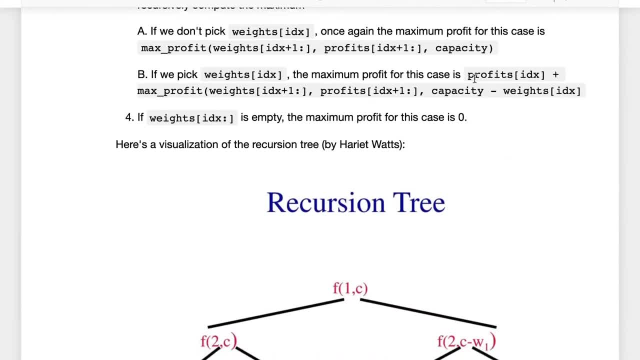 So if we pick weights IDX then the maximum profit for this case is profits of IDX Plus max profit of weights IDX plus one onwards profits IDX plus one onwards. But because we've used up some capacity, we reduce the capacity in the recursive call. 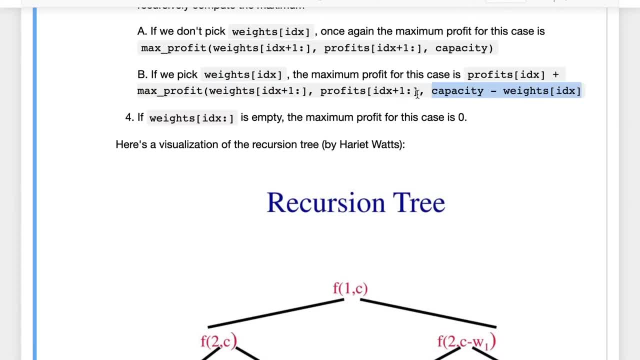 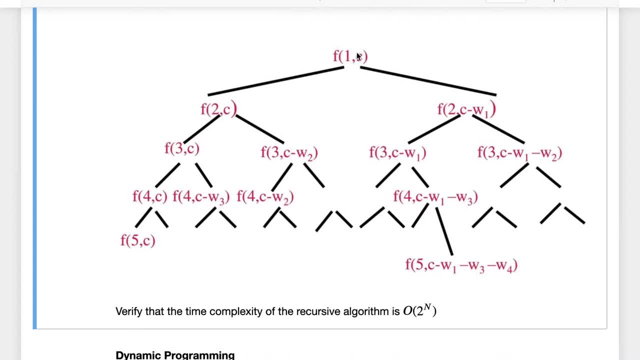 Okay, And that is why a recursive call takes both an index and a capacity. Okay, I hope that makes sense. So here's a recursive tree that tells you the same thing. We started the first index and we, we have the capacity. 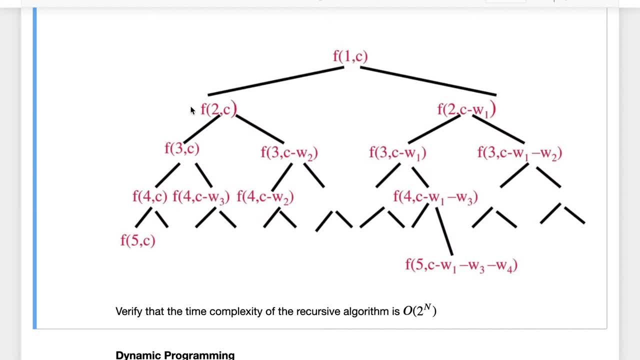 And if we don't pick the first element, then we simply, the answer is simply The the best solution for second index onwards with the same capacity. If we do pick the first element, then the answer is the second solution: onwards with the reduced capacity, with a profit added. 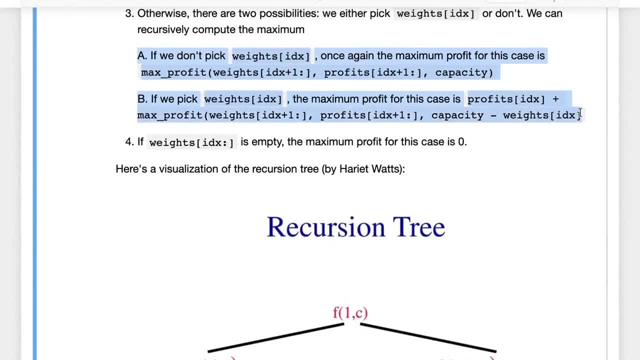 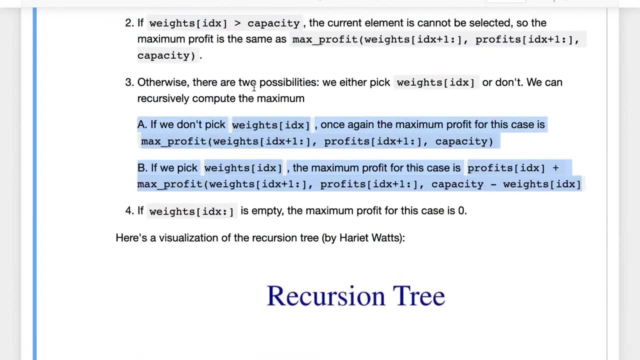 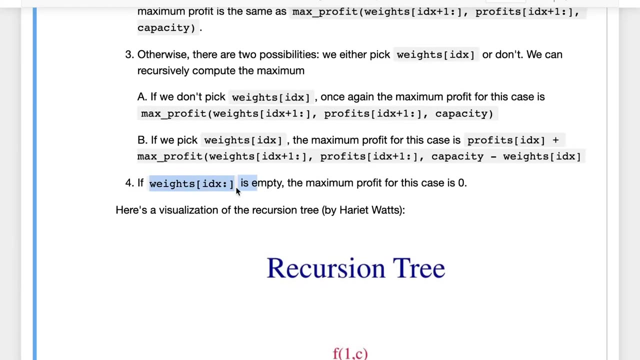 Okay, And then we simply take the maximum of these two cases. So we call these two recursive calls and then we simply take the maximum of these two cases to get back the final result or the final best answer. And the final end case is that if we've reached the end, if weights IDX onwards is empty, 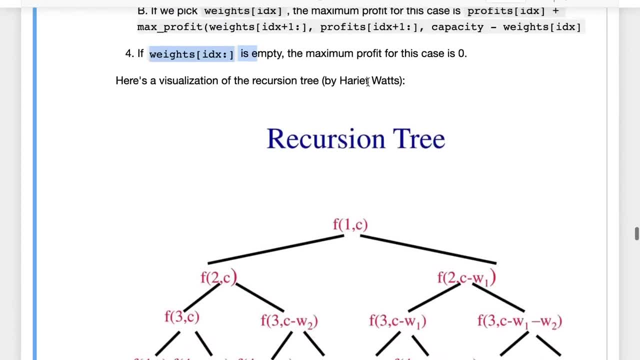 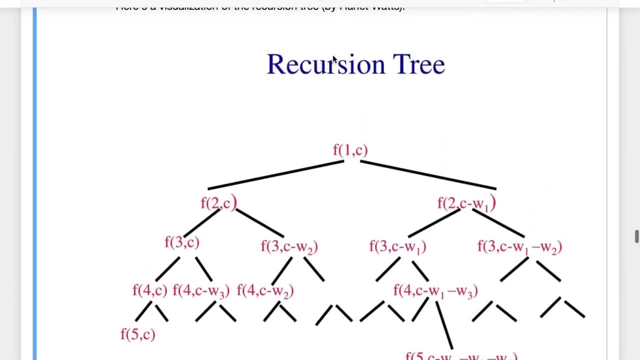 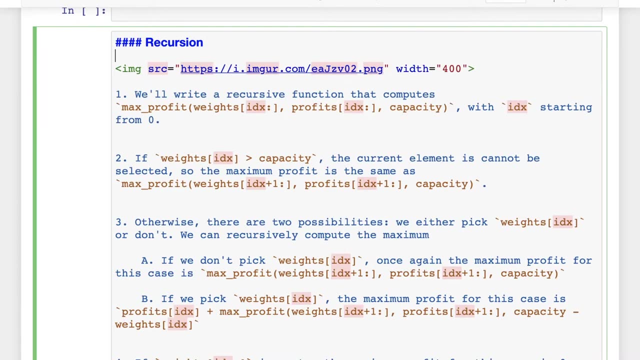 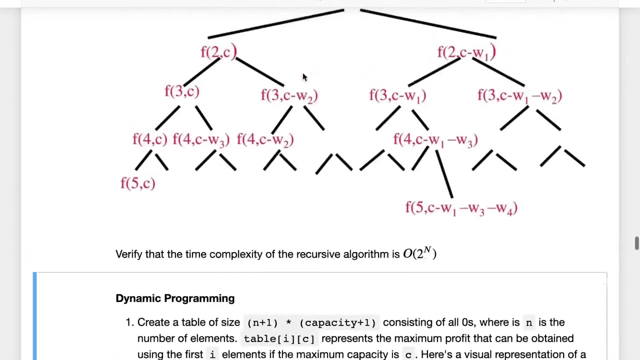 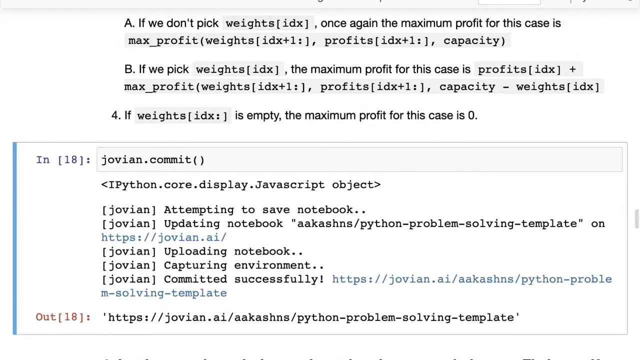 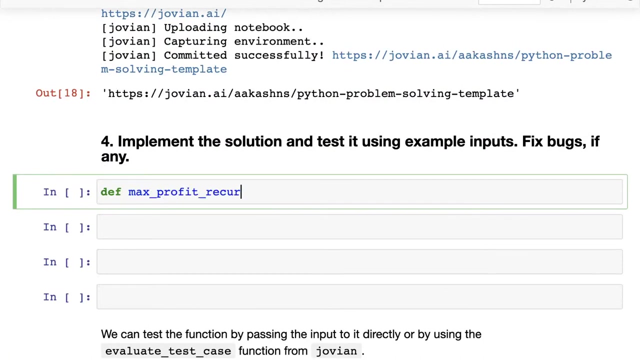 If the index that we're tracking has reached the very end, then, irrespective of what the capacity is, the maximum profit is in that case is zero. So let's try and implement this Now. let's copy this over as the explanation And let's try and implement the solution. let's say, let's call it max profit recursive, and this is going to take a set of weights, it is going to take a set of profits and it is going to take a capacity and is also going to take an index, which the index will start out at zero. 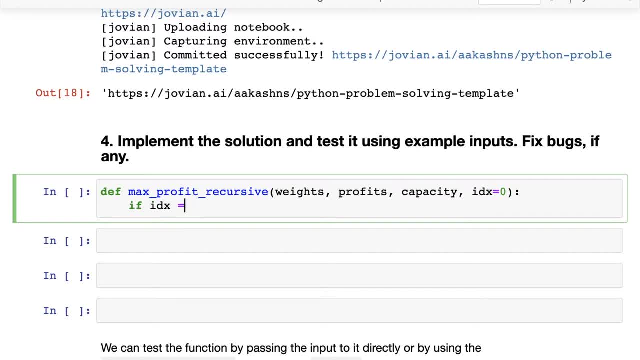 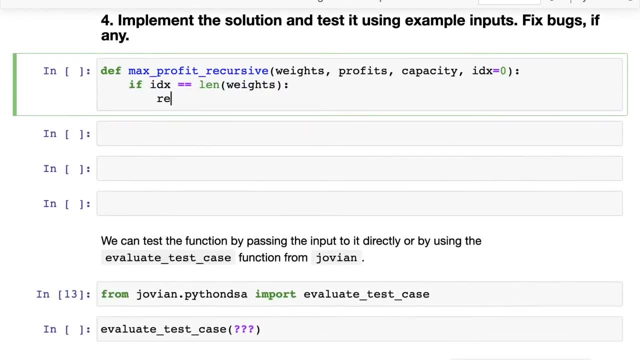 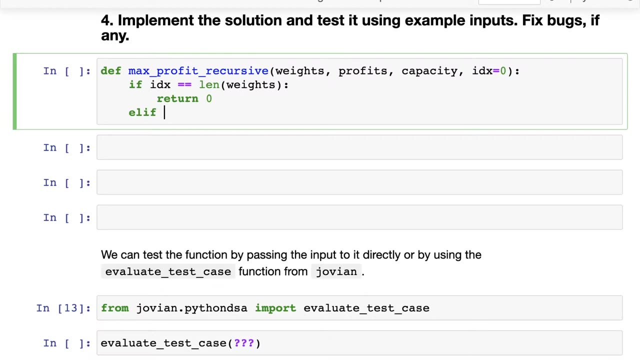 So now, if the index is, we started with the base case. so if IDX equals the length of weights, in this case there's nothing left to do. we simply return zero because we don't have any more elements. then we check if the weights IDX is, so the current element is greater in weight than the capacity. then it's a pretty straightforward solution. 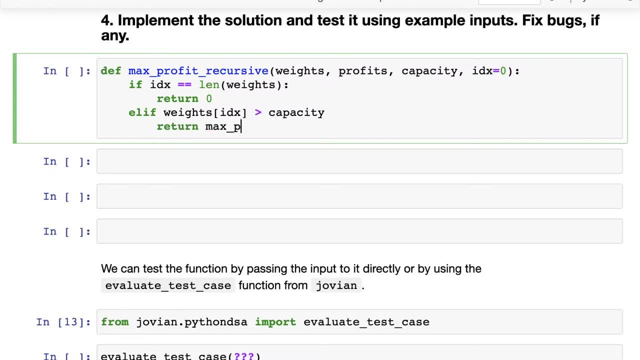 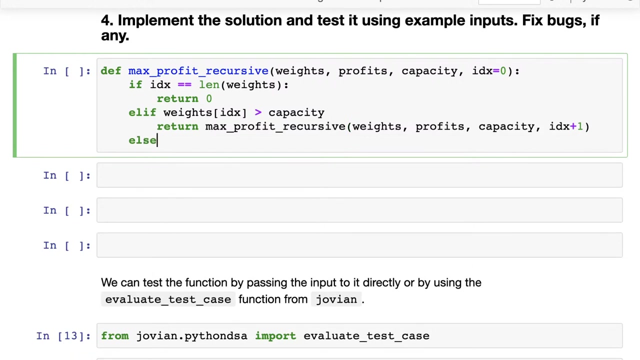 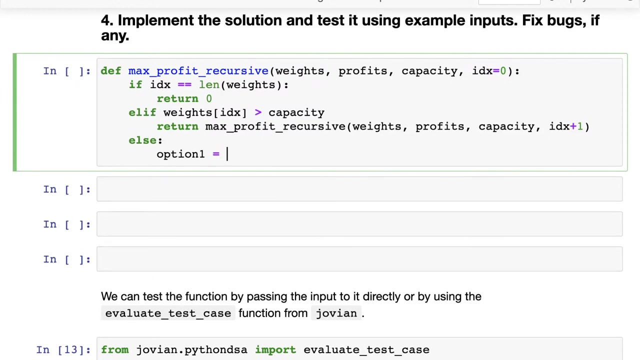 We simply return Max profit, recursive of weights profits, capacity plus one- sorry, capacity- and IDX plus one. So we simply ignore this element because we cannot fit it in the capacity that we have. else we have two options. We have option one. option one is: even though it can fit within the bag, we don't take it. 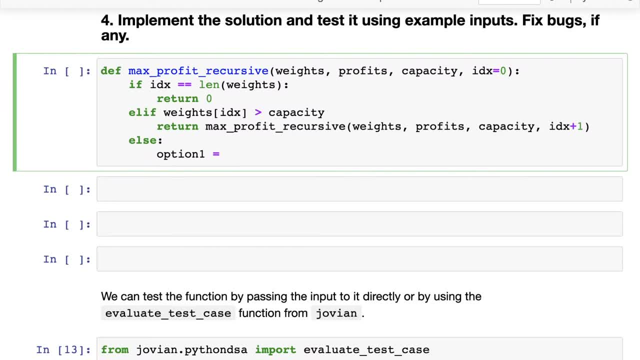 We, we, Because the optimal solution may still not have it. just because it fits does not mean we should take it. So we look at the option one, which is once again the same as this, where we ignore this element. And then we have, we look at option two. in option two, we actually put this element into the bag. 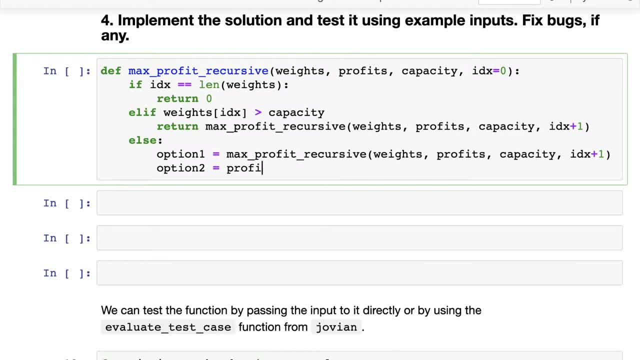 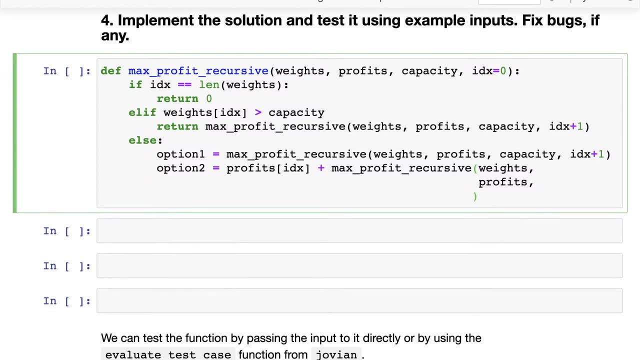 So, since we are putting this element into the bag, then we get, we get profit from it. So we get profits of IDX and then we call max profits recursive And this time we call it with weights. So we take the weights and profits and now the capacity has reduced a little bit because we have taken this element. 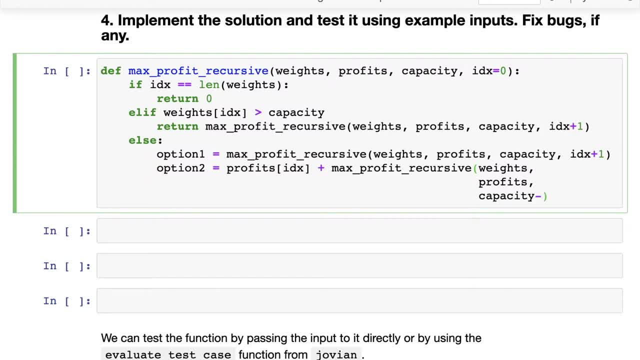 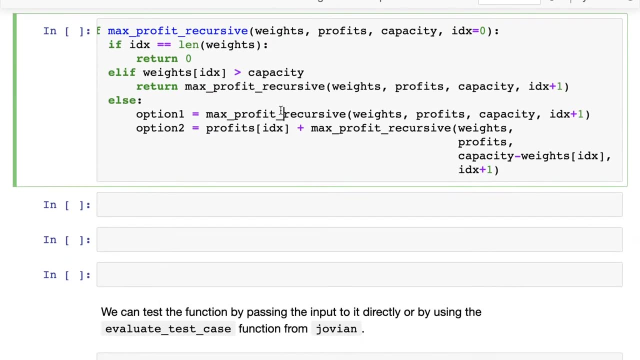 So now we can, now we need to fill the remaining. we fill the need to fill the bag with the remaining elements, from IDX plus one onwards, with a limited capacity of capacity minus weights of IDX, And then, finally, we just put in IDX plus one so that we can start calculating the solution from the next element onwards. 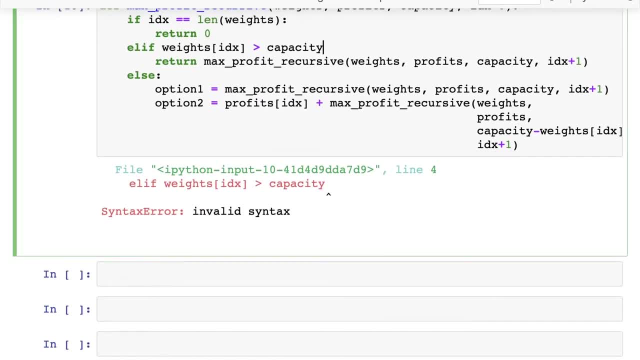 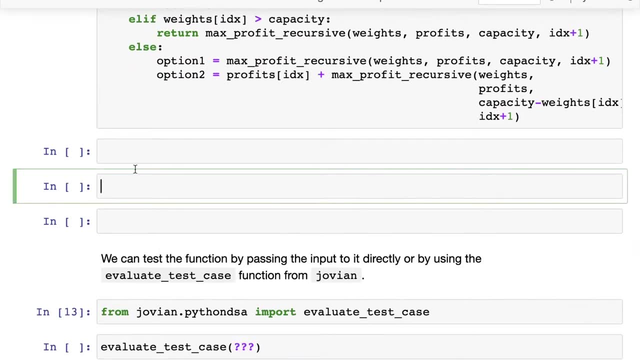 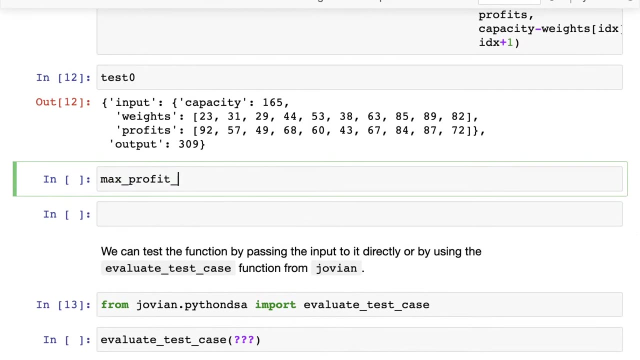 So that's max profit recursive. Again, not very difficult, It is just about six, seven lines of code and let's try it out. Here's test zero. Let's try max profit recursive with test zero input And we need to get weights, capacity and profit, all of these out of it. 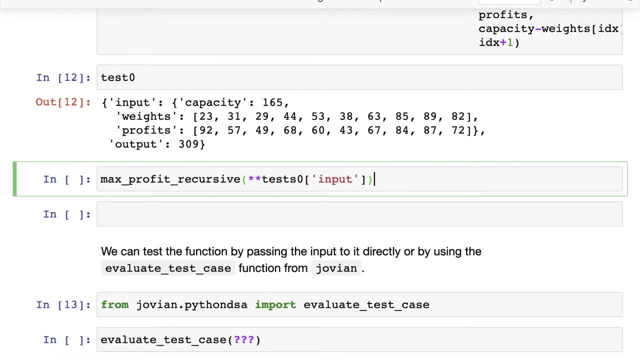 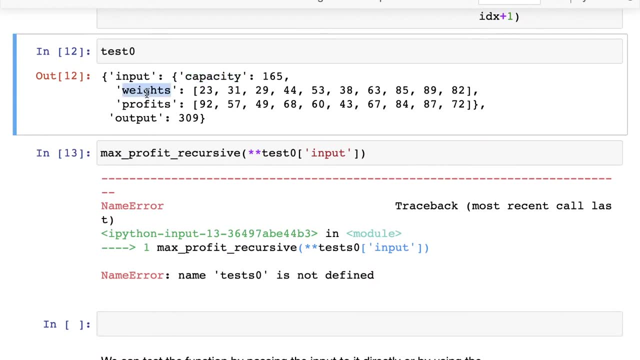 Simple. The simple way to do that is simply to put in star star and we'll get back. all of these will get passed in. capacity will get passed as a capacity parameter in, weights will get passed in as a weights parameter and profits as a profits parameter. 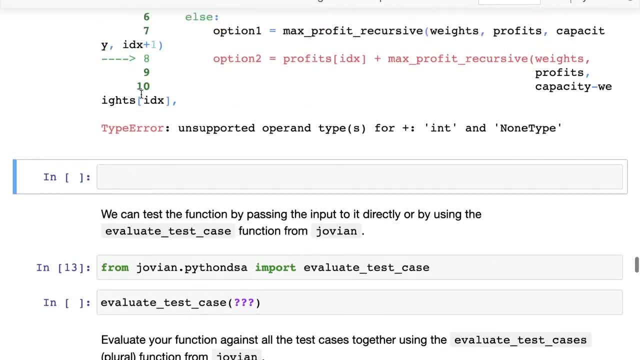 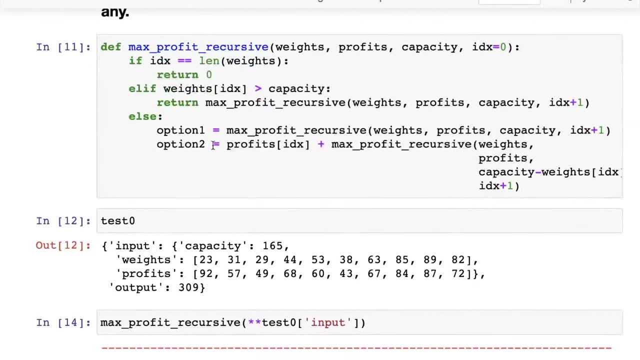 Okay, So we've encountered an error, and that's completely fine. Completely fine to encounter an error, I see. So what we've done here is, uh, we have not really taken the maximum of these two. We just need to find the two options. 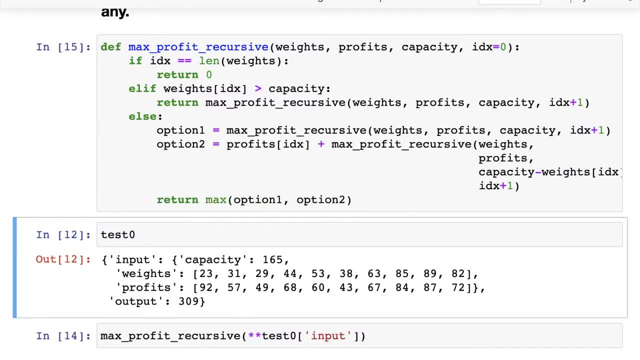 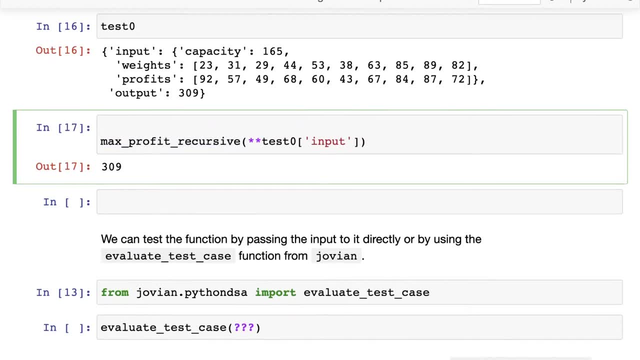 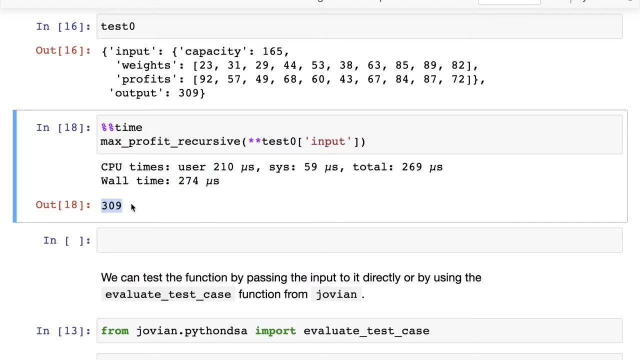 So we do need to take max of option one and option two. Okay, Once again, this is why helping test, having test cases, helps And you can see that now we call max profit and we can also add a timer here. The max profit it takes 210 microseconds but it result. it returns a result three zero nine. 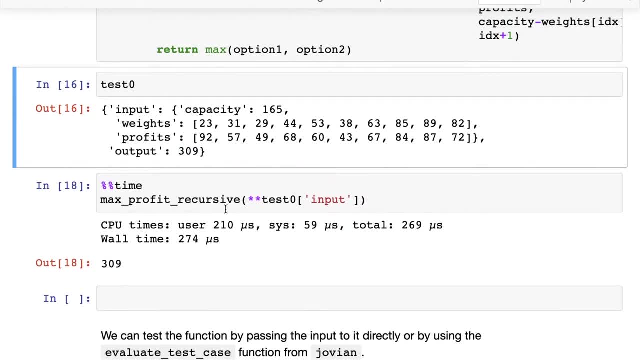 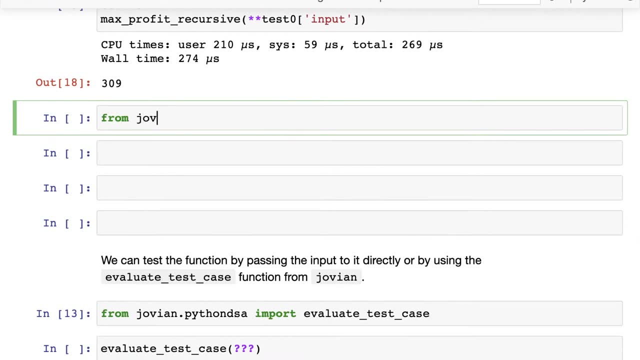 Great, We get back the result three zero nine here, which is what we expected. So our function is working correctly. We can even evaluate it on all the test cases. So from Jovian dot Python, DSA, we import evaluate test cases. 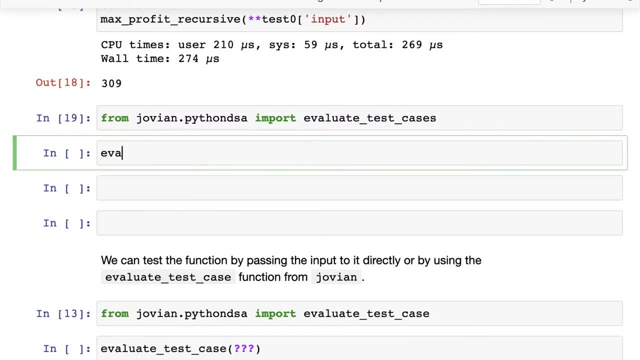 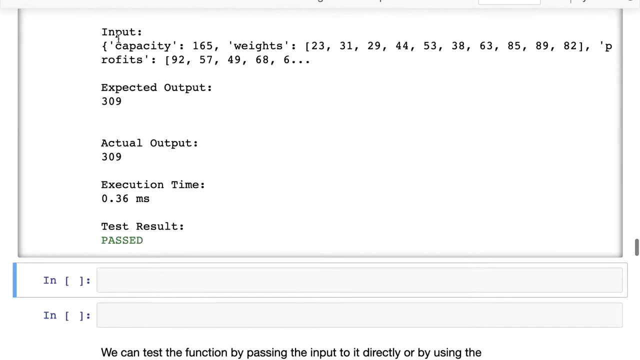 And then we simply call evaluate test cases on all the inputs. So we pass in max profit recursive And then we pass in all the test cases as tests. Now you can see that we have these test cases and each test case seems to be passing just fine. 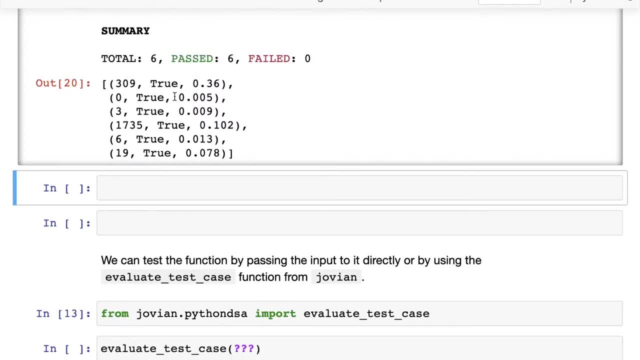 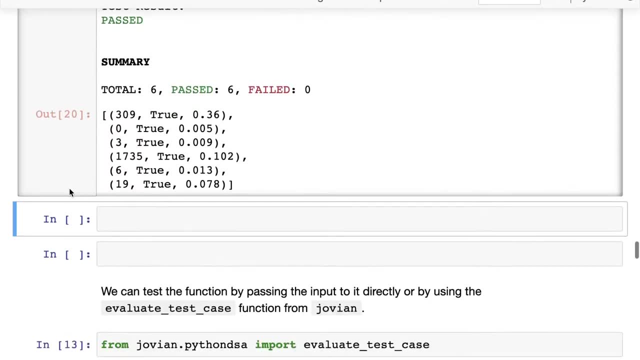 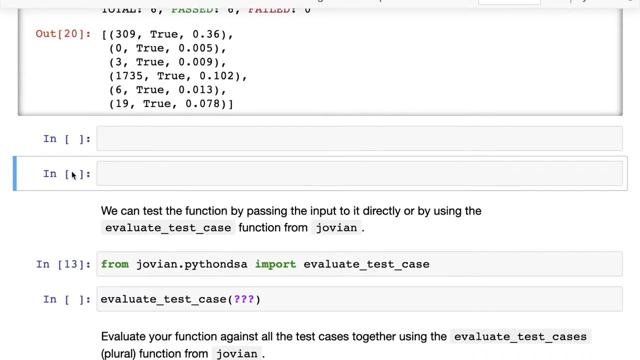 All six X test cases have passed and these are the times they took. So that's your recursive solution, Pretty straightforward Once you reason it out. once you maybe just look at an example, draw a tree of recursion yourself, work it out on paper. 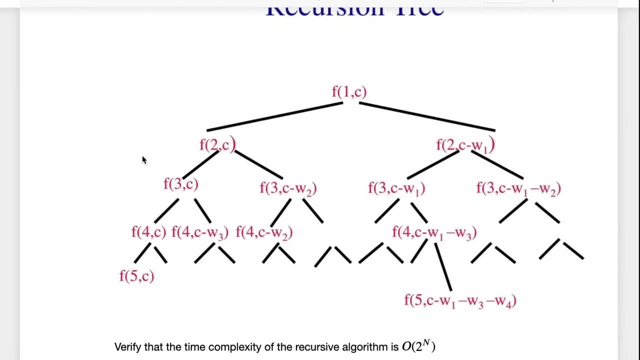 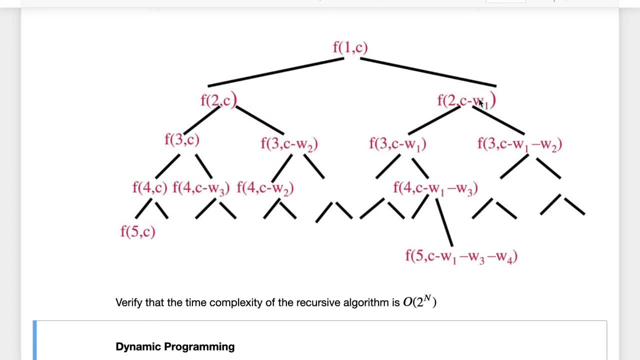 The code is, in fact, in most cases- In most cases- fairly simple, And this is what the recursion tree looks like Each time we make a choice to either include the element or not include the element. And now you can reason the complexity very easily, because now we have N elements for each one. 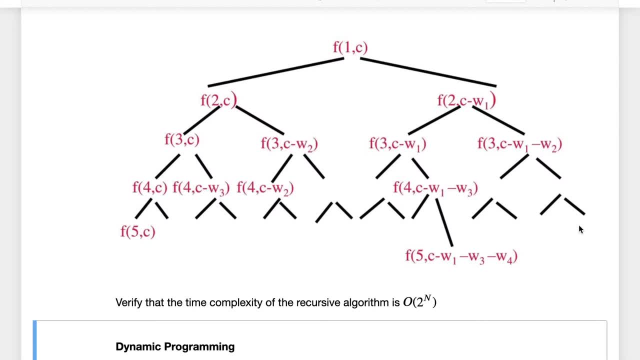 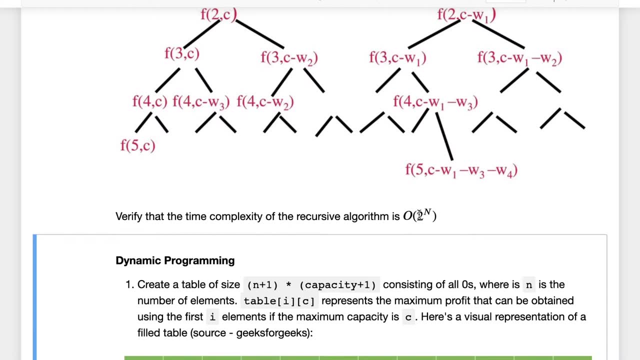 We keep making this choice. So that means we end up with two to the power N leaves, And from there it follows that the complexity of the recursive algorithm is order of two to the bar N, right? So it could be two times or C times two to the bar N, but uh, 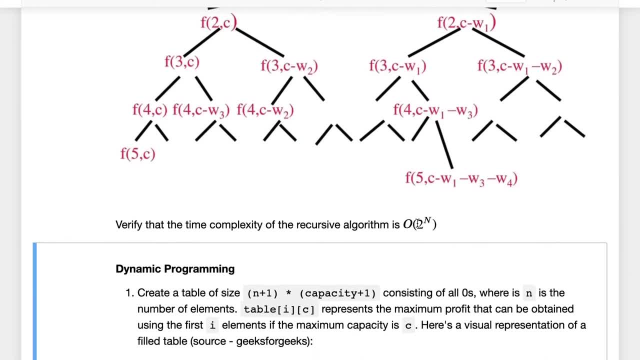 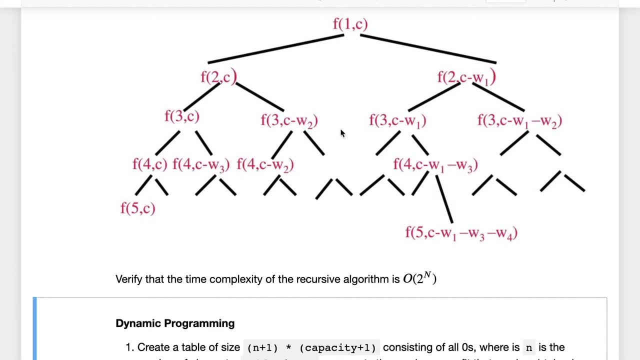 and in the bigger notation it's order of two to the power of N. So it is exponential. and complexity- And why is it exponential complexity, Once again there are. it's a possibility here that we may be computing a lot of things repeatedly because we are 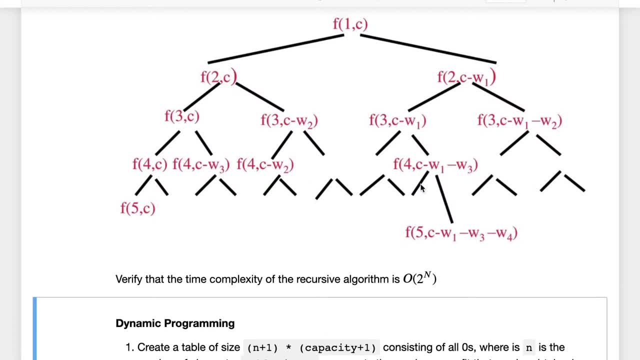 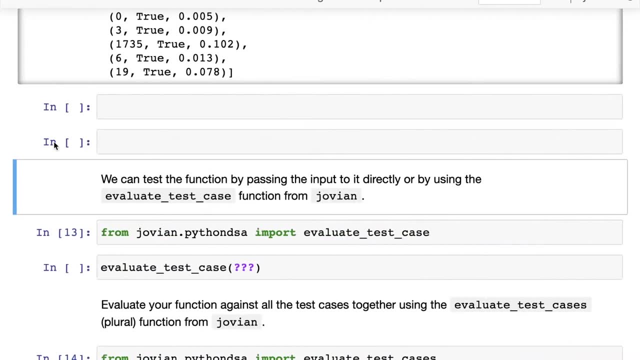 creating so many of these sub problems. So it's possible that we may be creating, we may be re-computing a lot of data here. So now the task for you, or the an exercise for you, is to write the recursive memoized version of this. 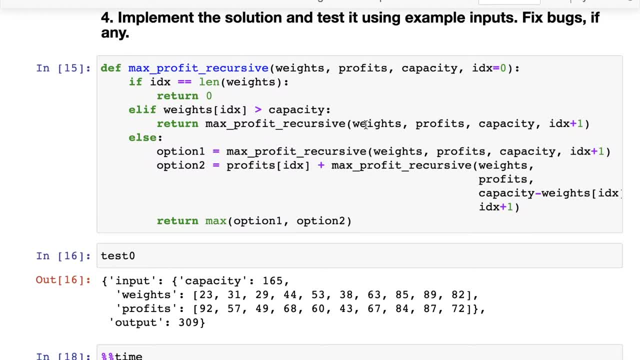 So what is it that you need to memoize Now? the trick here is to look at what is changing within the recursive calls. So now, in max profit recursive you can see that weights and profits remains the same, but it's the capacity and the IDX that change. 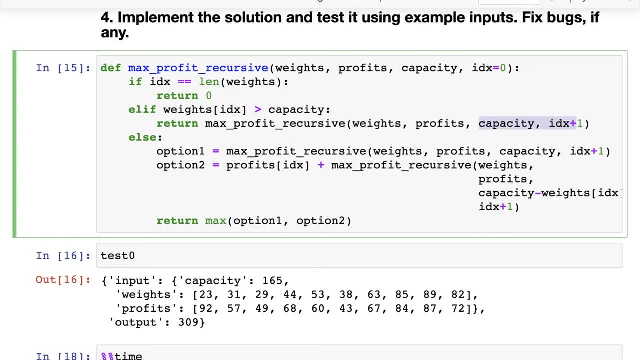 So you can take the capacity comma, the index, the IDX, as the key in your memoization dictionary And each time you compute, So each time let's say you compute this or you compute This, store the result in the dictionary before returning it. 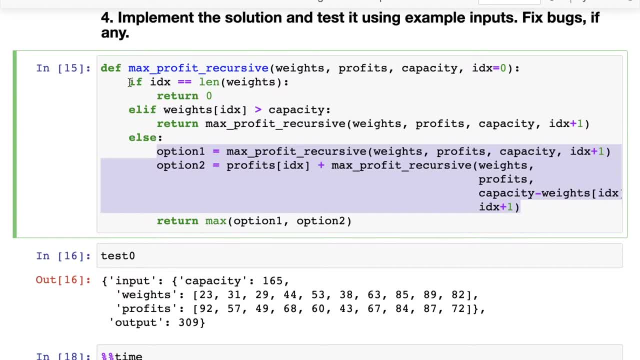 And then, at the beginning of the recursive function, check within the dictionary if this value is already present. Okay, So remember what we did for longest common subsequence: we defined a recursive function internally, We defined a memo, a dictionary, internally and the recursive function kept, either checking the dictionary or filling. 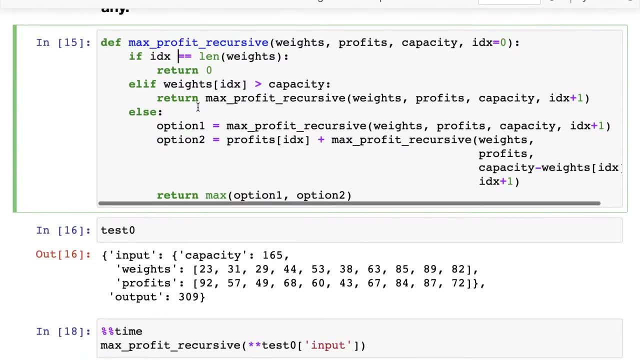 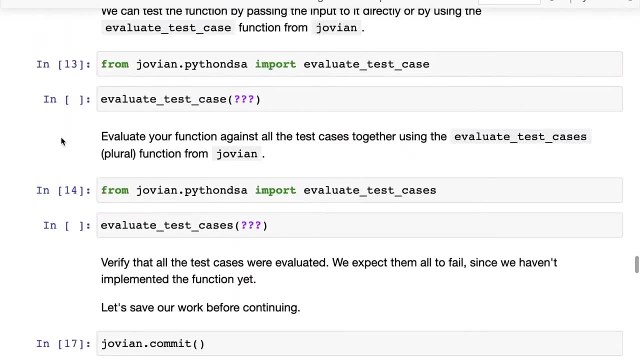 the dictionary if it could not find a value and that could eliminate a loss. Okay, So you can do a lot of the repeated work in your problem. Okay, So that's the challenge for you: to try out implement the memo solution. 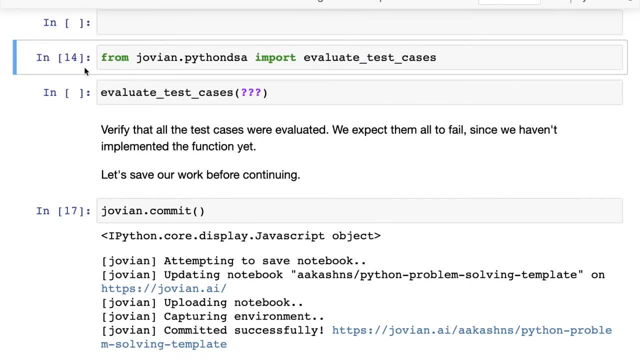 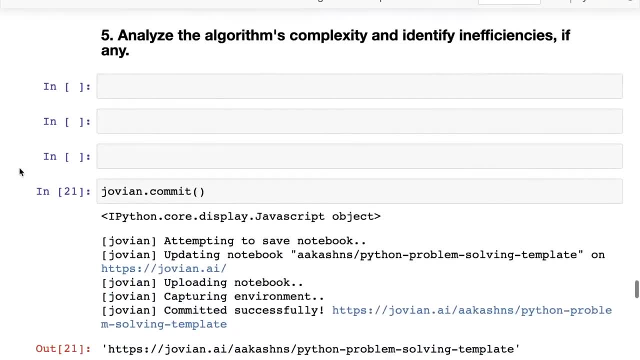 And what we'll do is we will go ahead and we will implement the dynamic programming solution. So let's just come at our work once again, and we've analyzed the algorithms. complexity in recursion: It's order two to the power of N in memoization. 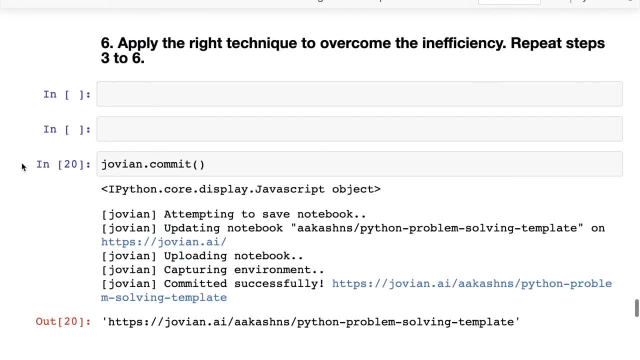 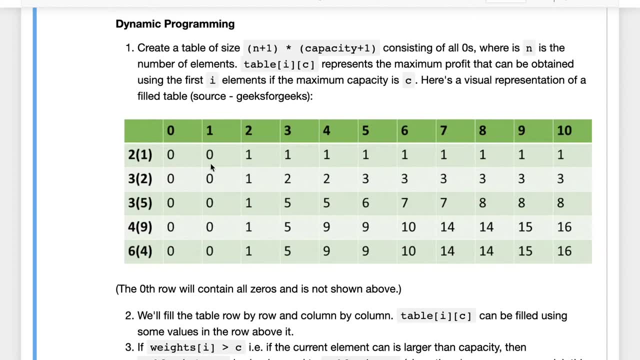 Now, that's an exercise for you. What do you think the complexity will be? but let's apply dynamic programming. So let's look at a dynamic programming solution. Now, once again, for dynamic programming you have to create a table. You always, almost always, have to create a table. for dynamic programming, 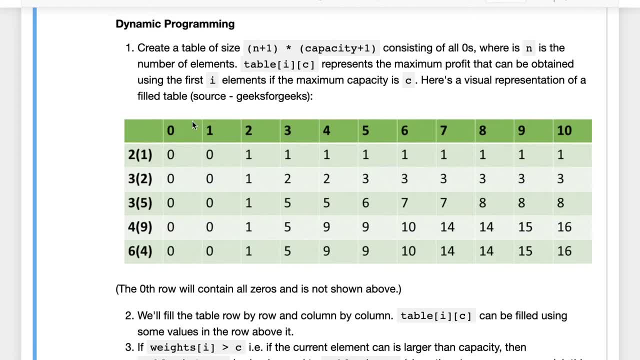 And in this case we can see that there are N elements. So there are N rows within the table because we have N elements to choose from, And we are. we have a number of columns going from zero to capacity, plus one going from. 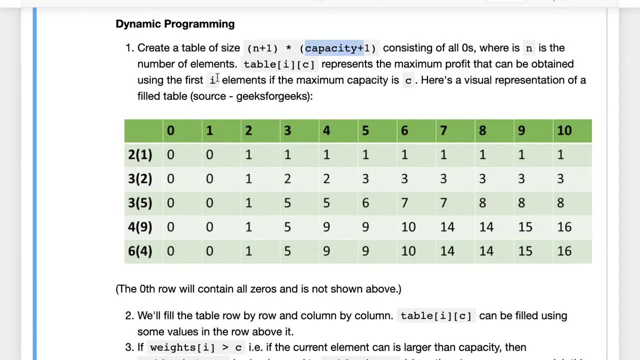 zero to capacity, And that's why there are total of capacity plus one columns And in fact, what we can do is we can also include another column at the top here, another row at the top here, which we have not, which is not shown here, but what N represents? N is the number of elements. 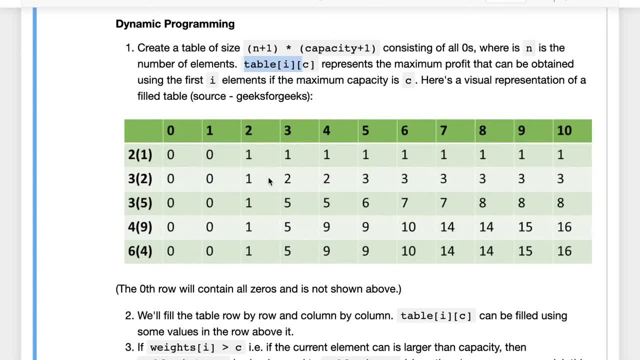 So what N represents or what the a particular element in the table represents. So, table of I, comma C: what it represents is the maximum profit that can be obtained Using the first I elements if the maximum capacity is C. okay, So if your maximum capacity is C, let's say your maximum capacity is three, what is the? 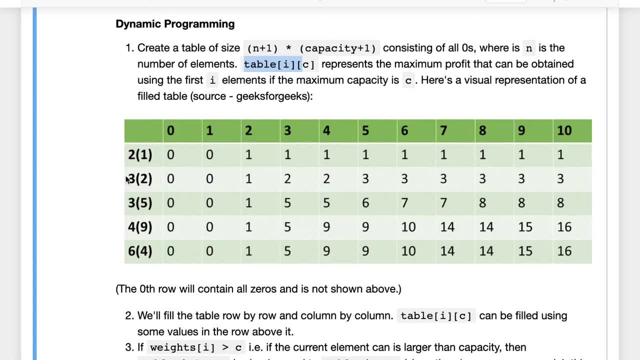 maximum profit that you can obtain using the first two elements. So, um, here let's say we are at this person, So using the first two elements off the list within this capacity, okay, So, So the first two elements have weights one and two and the capacity is three. 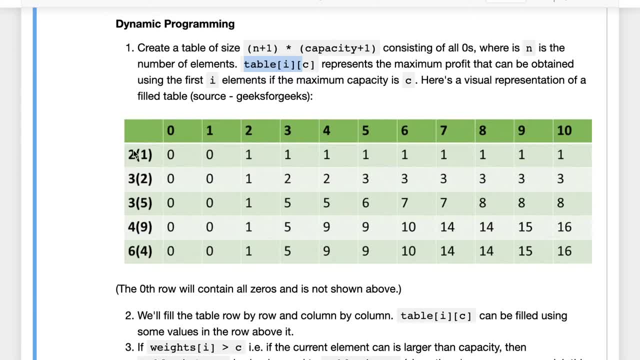 So you can. you can actually pick a. sorry, the first two elements of weights, two and three, and the capacity is three. So you either pick this element or pick this element. Now, if you pick this element, the profit is one. 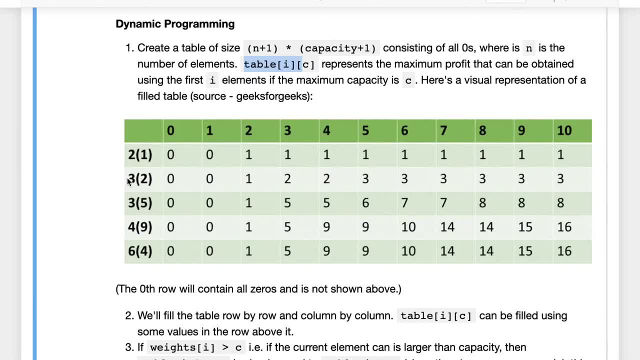 And if you, if you pick this element, the profit is two. So the solution is to pick this element and you get- uh, you fill the capacity three and you get a profit of two. You cannot pick both because your capacity is three. 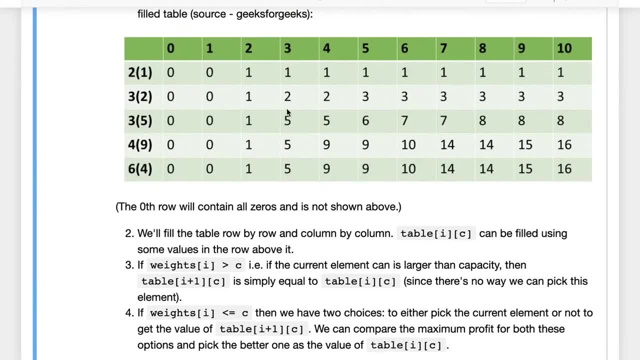 Okay, So that's the logic here. A very simple visual representation. Now, remember that there will also be a zero throw here, which we have not shown, but this is something that should be here. Uh, another zero throw. So the zero throw represents that you've not picked any of the elements. 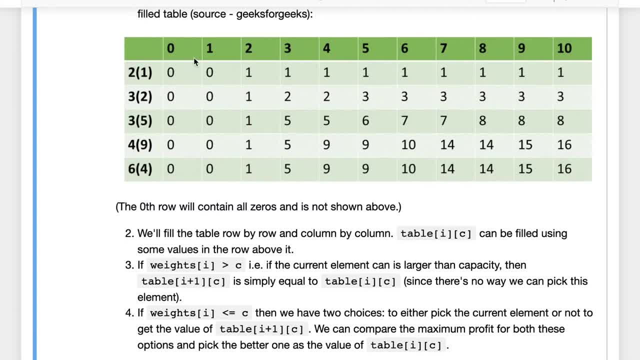 And if you don't pick any of the elements, it is simply going to contain all zeros And that's why it's not shown here. The first row assumes that you have picked. you can pick only the first element, So you can- you- you can't pick the first element- till a capacity of two. 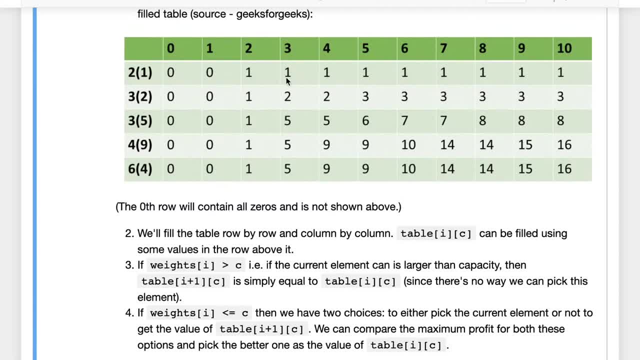 And then, from a capacity of two onwards, you pick the first element and that has the maximum capacity of one, the maximum profit of one. the second row, or the row Number two with row, with index two represents the fact that you can pick both of these elements. 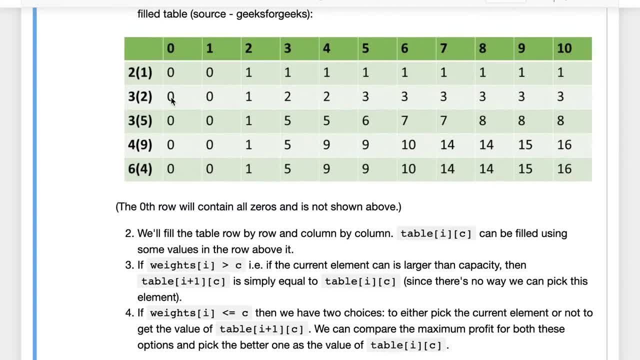 And if you can pick both of these elements once again at capacity zero- none of them can be picked at capacity one- None of them can be picked at capacity to- this element can be picked, which has a way to, and it gives you a maximum profit of one at. 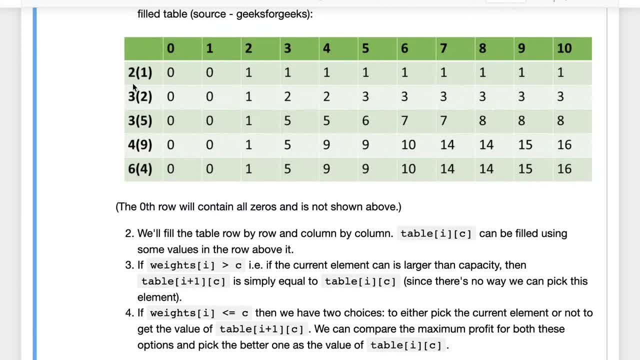 capacity Three. this element can also be picked. So now you have a choice to pick between the two of these. So you might as well better pick this one, because this is going to give you a higher profit, And then, finally, when the capacity becomes five, you can pick both of these elements, and you can pick both of these elements. 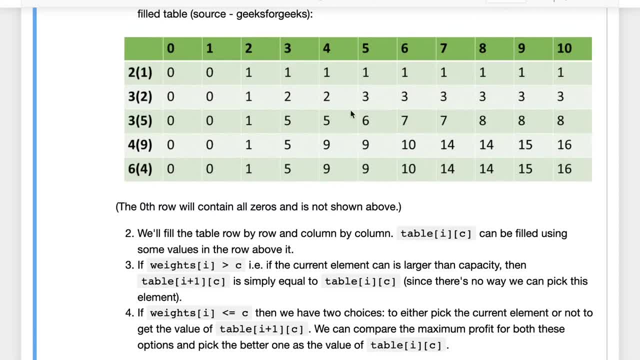 And that is going to give you a profit of two plus one, three and so on. So you keep filling out the stable. for each step here, or for each set of first I elements, you fill out the capacity table And then you use the information to fill out the next row and the next column, and so on. 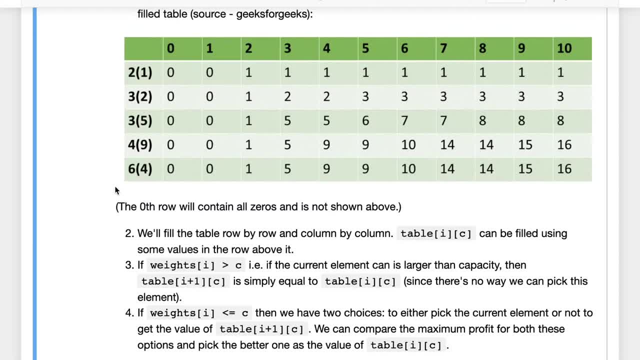 Okay, And finally, what we need is using all the elements and using the maximum capacity that we have. What is the maximum profit that we can obtain? So the last element of the table will give you the result. Okay, So what does the logic look like? 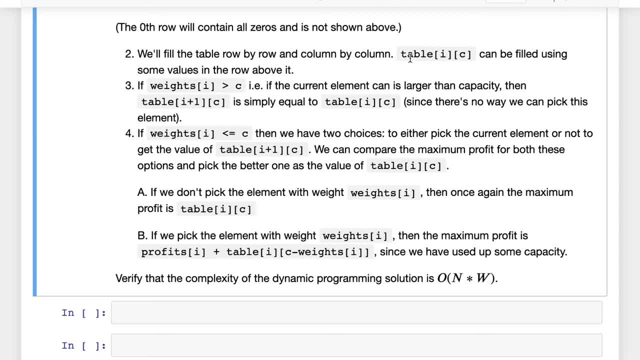 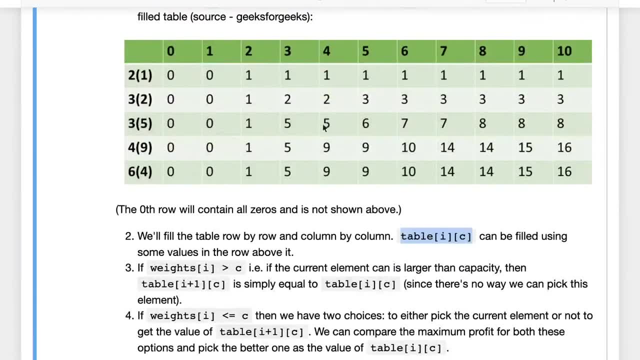 We will fill the table row by row and column by column. Now, if table of I comma C, They will have I comma C. Let's say this is a certain position here. Table of I comma C can be filled using some values in the row above it. 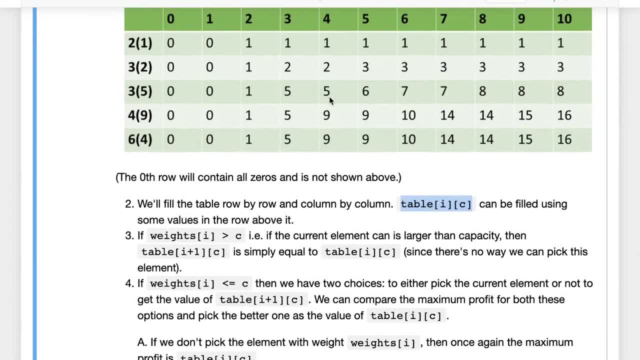 Okay, Now, if you look at the table of I, comma C, you look at, look at this element, for example: Yeah, Let's look at this element here. So in here, C has the value three, and then I has the value zero, which is a row that is not shown. one, two, three, four. 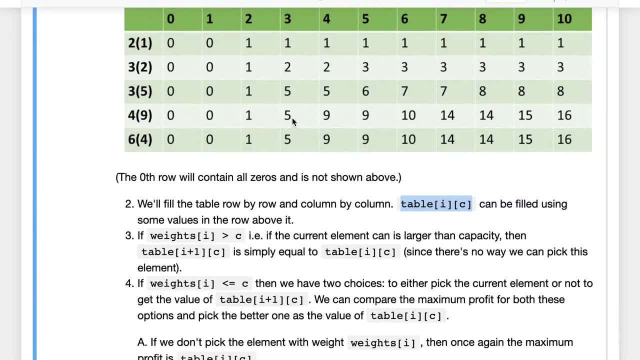 So I has a value of four and C has the value Three. So if yeah, so if weights of I is greater than C, so zero, one, two, three, four, um, if, if the, if this, if this weight, so this. 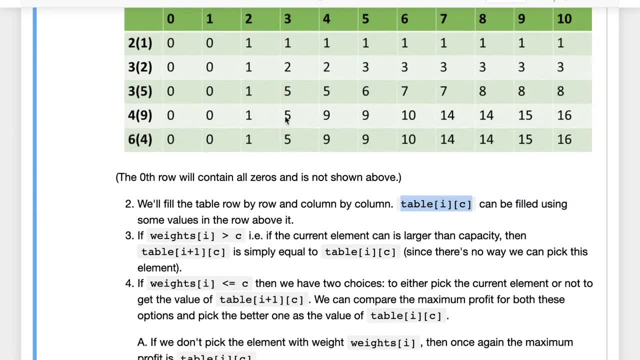 weight. the weight of this element is greater than the capacity. So the weight of this element is four: It is greater than the capacity. Then this element cannot show up in this maximum profit. Why? Because it's weight is greater than the capacity. 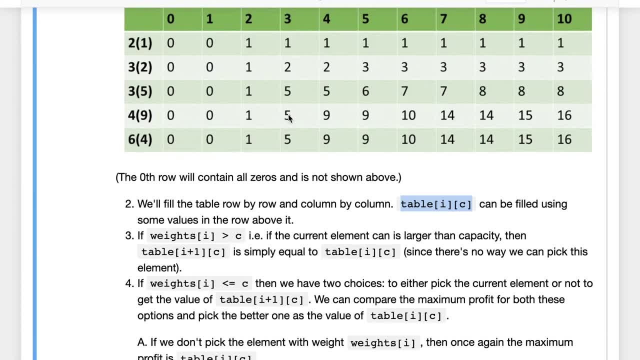 So obviously it cannot show up in the maximum profit. Now, if it cannot show up in the maximum profit, then the so then this cell can be filled using the value above it, because in any case you cannot put in this element. 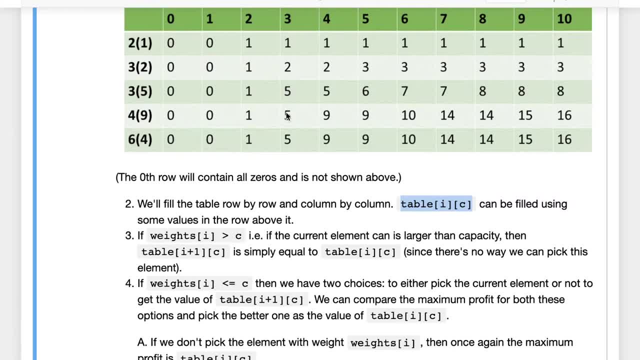 So you might as well get the result by using the first three elements, And in that case the value of the cell is obtained from the value of the cell above it. That's one case. Now, on the other hand, let's come here. 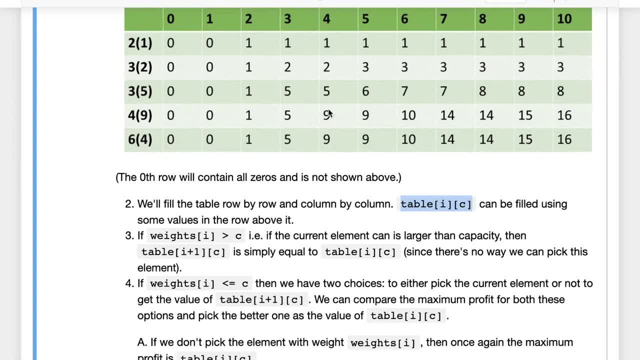 You come to this case, it to this cell in two. In to fill this cell, because you have a capacity of four, you have the option of either choosing this element or of not choosing this element. Now, if you do choose this element- let's say you choose this element with a capacity of four or with a capacity of four, you get back a profit of nine. 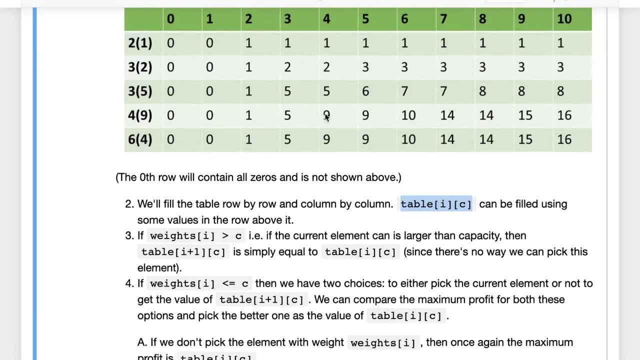 And now you have no more capacity left to create more, to fill more elements. On the other hand, if you do not choose this element, then that's the same as this value, Because if you do not, This is an element, then you have to fill the capacity of four using the value of using the first three elements. 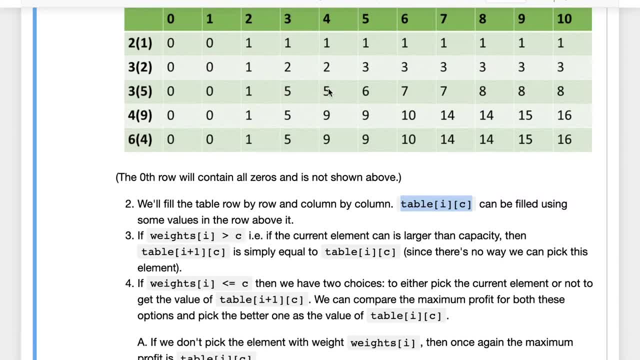 And that simply gives you the same highest profit as the previous set right. So you just consider these two cases, whether we choose the element or we do not choose the element. Now, if, if you do not choose the element, the value comes from above. 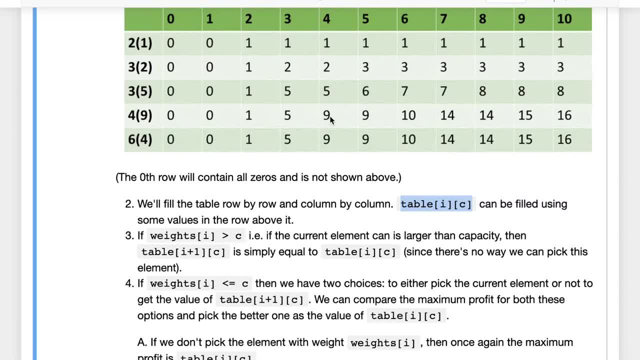 If you choose the element, then the value comes from where. let's see: If you choose the element, the profit of nine comes and you fill out a capacity for so you have no remaining capacity. but on the other hand, if the capacity was six and you choose the element, then you have chosen the. 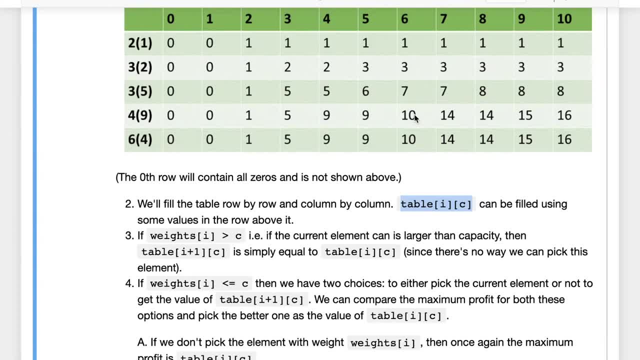 element and you've used up the capacity for. so you can still use the previous three elements to fill the remaining capacity, which is six minus four, which is your capacity of two. So you can go back to the previous row and check the capacity too and see how much was a maximum profit that you can obtain with. 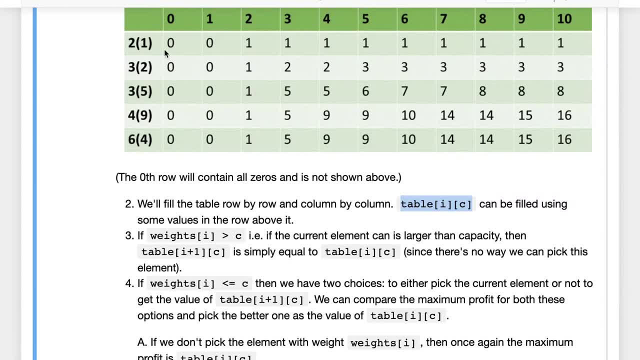 capacity too, And it turns out that with capacity too, Using the first three elements, you can obtain a maximum profit of one. So the maximum profit here, when you choose the element, is nine plus one, And similarly here the maximum profit that can be obtained. 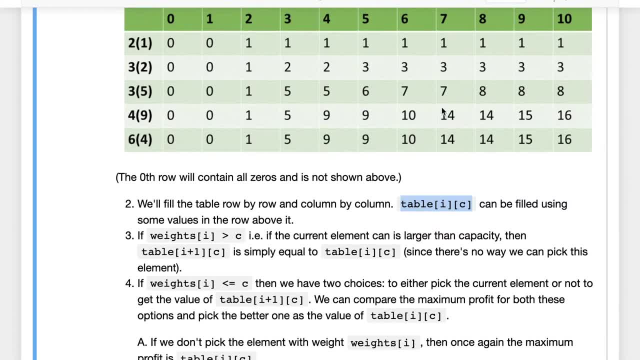 If you choose, the element is nine plus seven, minus a plus. from the previous row you pick the element with a capacity seven minus four, which is three, So nine plus five, 14.. Okay, So that's the logic here. Sometimes you choose the element. 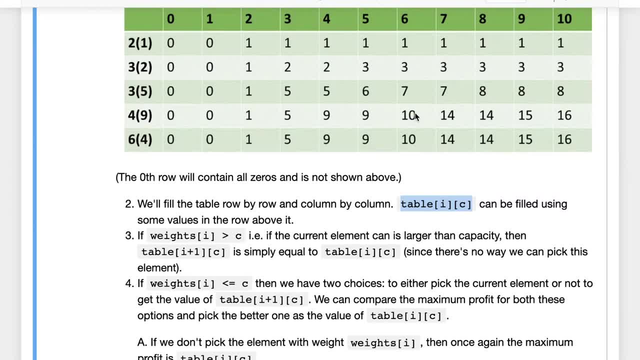 Sometimes you don't choose the element And, in fact, the solute, the result of the cell is simply the maximum of either not choosing the elements- the maximum of this cell- or choosing the element and subtracting the weight, which is six minus four two. 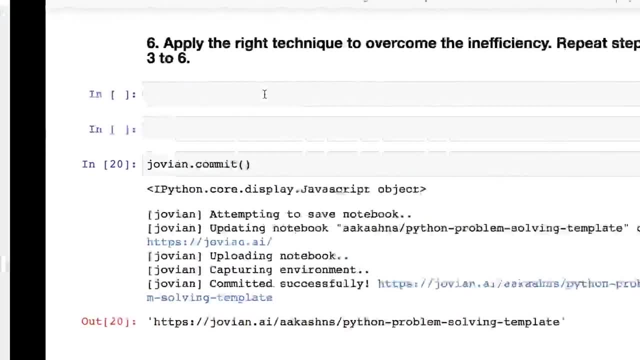 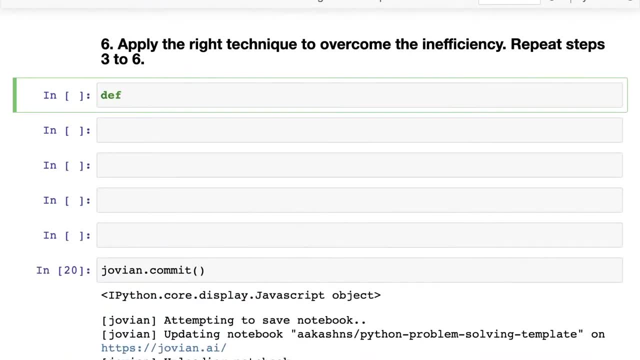 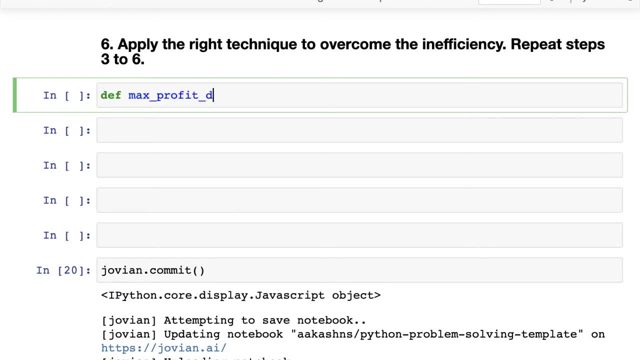 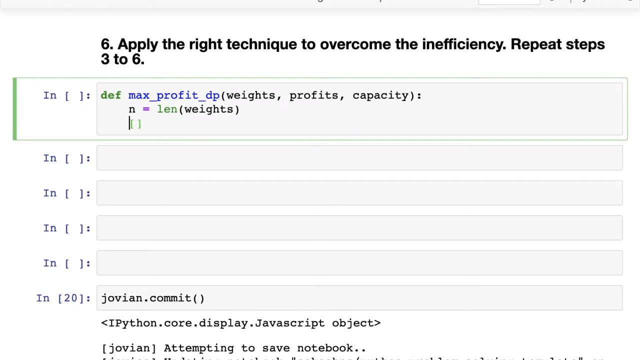 So we need to create a table. This is that table. A table contains end rows, So we have land in and then in. for each of the roles We contain, we have capacity plus one. Oh, we contain N plus one rows. 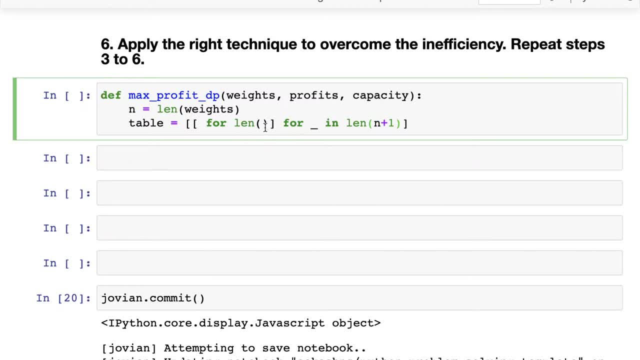 Remember, we also want to consider the case where we don't consider, where we don't take any of the elements, and it is filled with zeros And the number of columns is capacity plus one to check the values from zero to capacity. So that's a table right now. 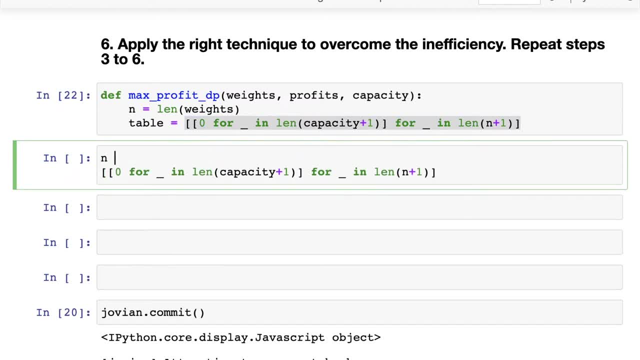 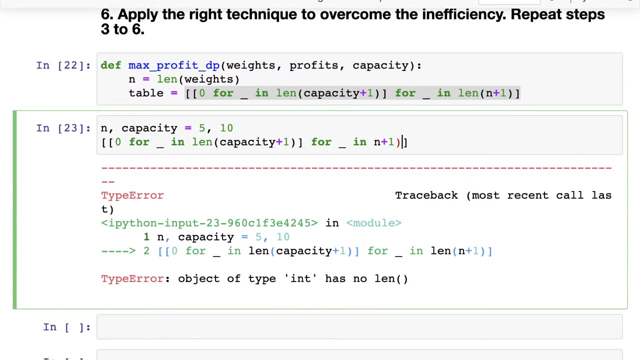 You can check what this capacity looks like. Let's say N has N and capacity have the values here. N, in this case is five and capacity is 10.. We don't need a line here. We don't need a line here as well. 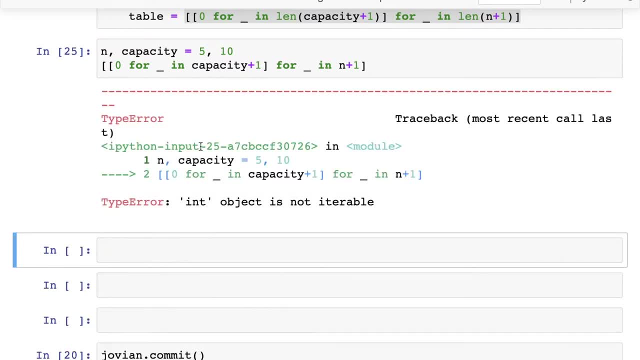 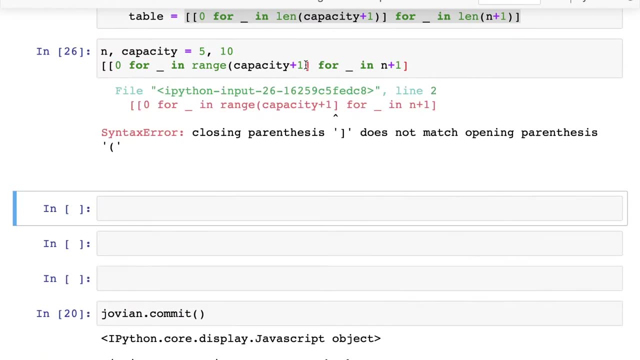 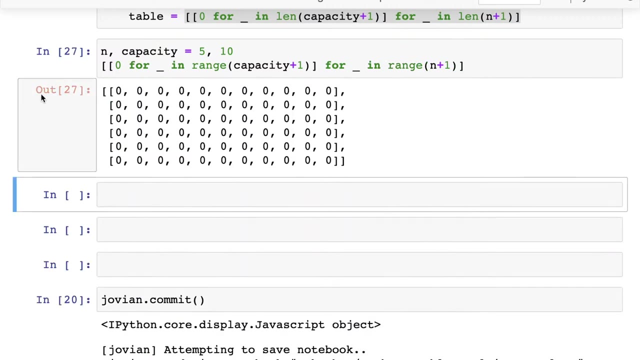 It's all perfectly natural to make these mistakes. This should be range, not Len, So this should be a range and this should be arranged to. yeah, now you can see that we have created N rows, or N plus one rows, So one for each of these and then one more row above containing 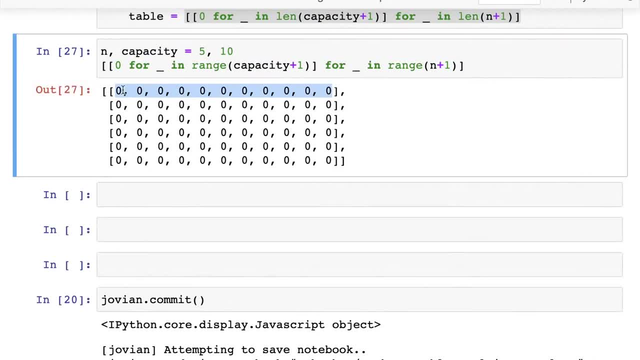 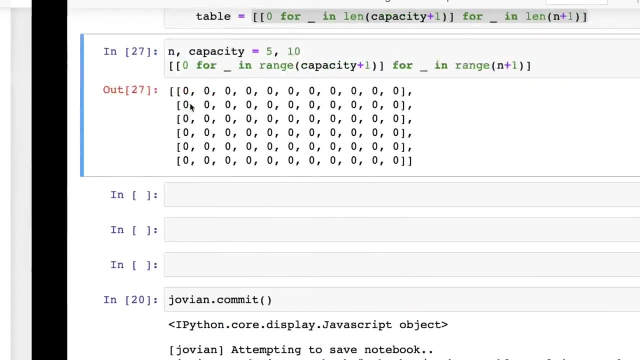 all, which will contain all zeros. This is in the case where we don't pick any of the elements and then we've created 11 columns. So this is for capacity zero. So, again, the first column will also contain all zeros, And this is something that you will often see in dynamic programming. you will 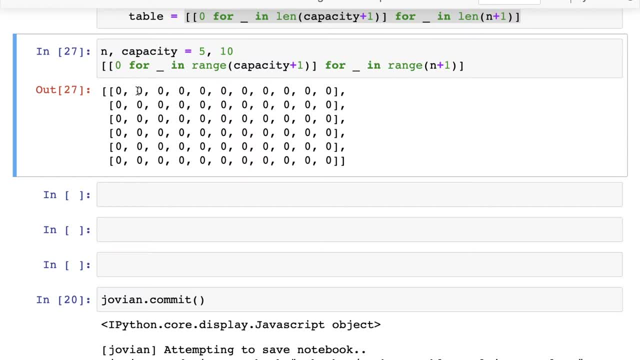 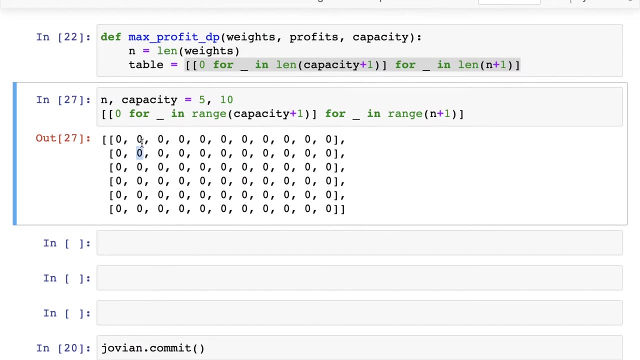 have an additional row at the beginning or at the end containing all zeros, And that is simply to make your calculations or computations easier, But what that will lead to is off by one error, So you need to be very careful while doing this, And now we'll fill out this value using either this value or by subtracting the. 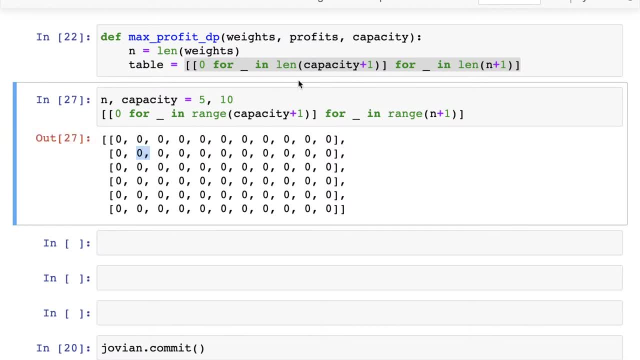 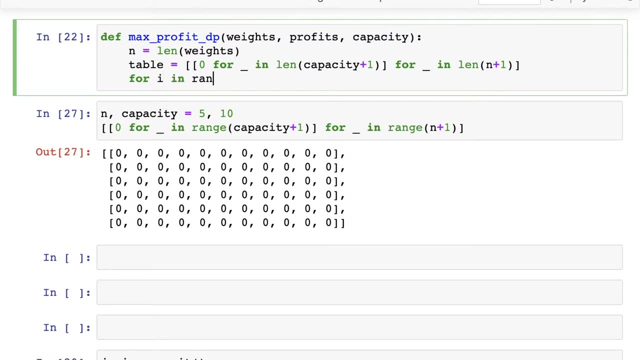 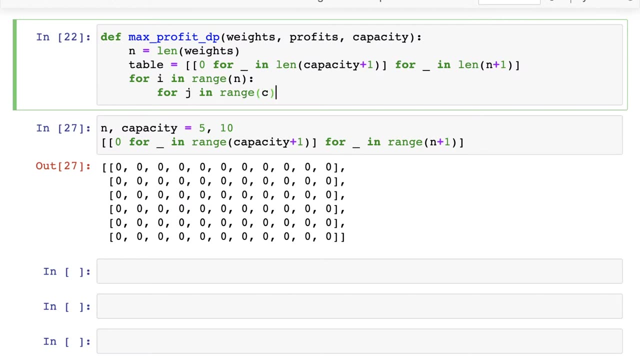 weight of the element that's here and getting a value from the previous row. So now we start iterating. So when now we say for I in range N and for J in range C, let's just say for C in range capacity. it should be. 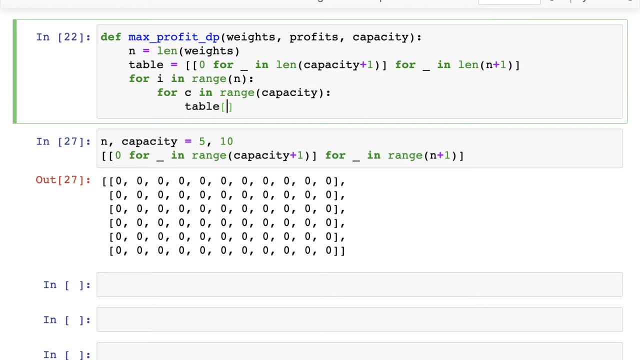 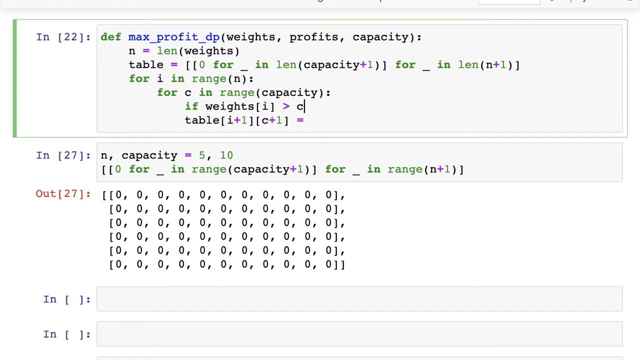 capacity table of I comma C. and it's actually going to be I plus one and C plus one because we have these additional rows and columns able to find I plus one comma C plus one is. there are two cases here. If weights of I is greater than C- the current capacity- then we can simply look at the previous row. 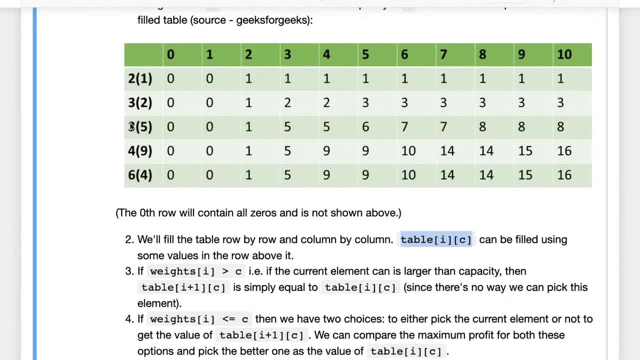 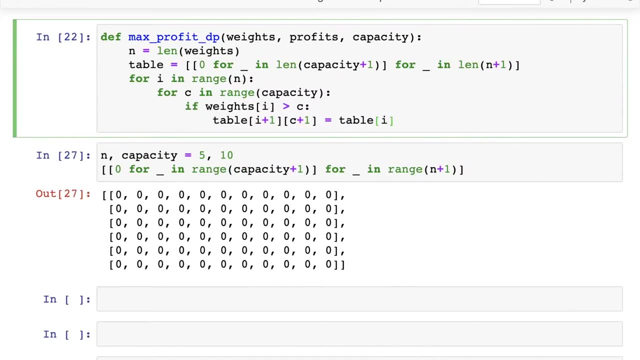 So, which is this case? let's say, the weight three is greater than the current capacity two. So then we simply copy over the value from the previous row, the same column. So we just say: table of I, comma C plus one. Well, this should be C. 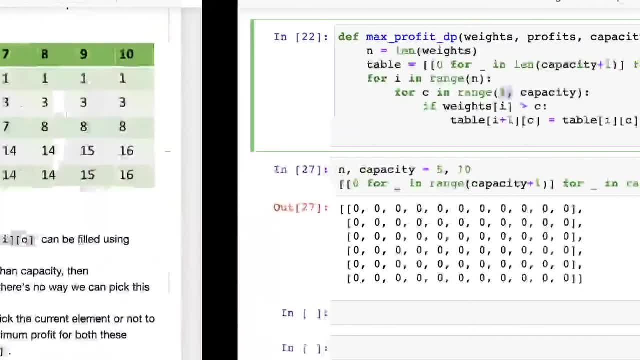 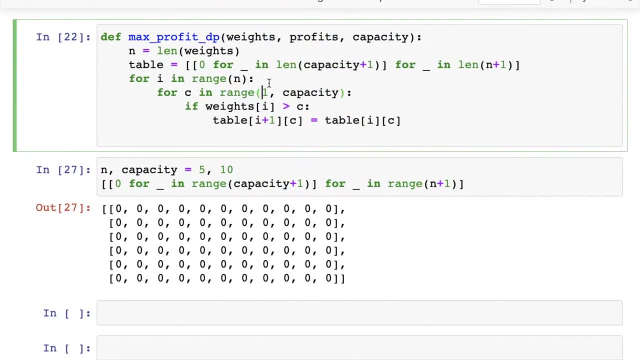 So our capacity should go from the value of one, because we don't want to affect the first column. So the our capacity. So our capacity goes from the value of one to a value of 10.. So capacity C goes from the range of one to capacity. 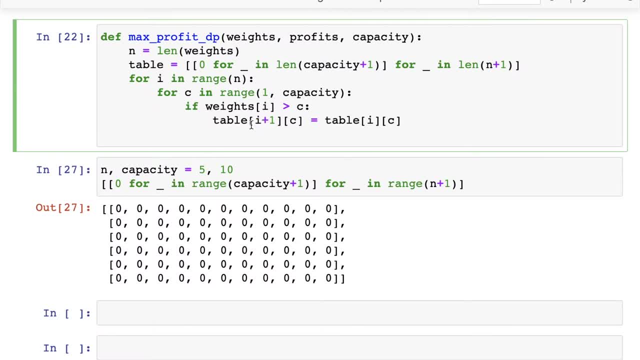 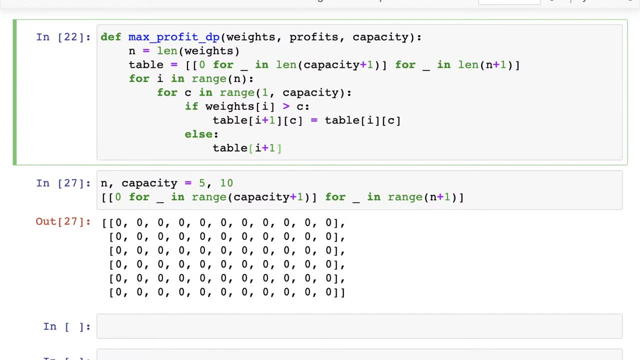 And if the weights I is greater than the capacity, then we cannot fill the table. On the other hand, if it is, if it fits within the capacity, then we have two options. The table of I plus one comma C has two options. 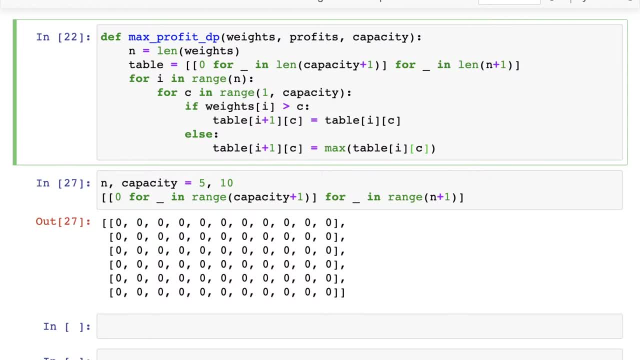 So one is: we don't use the current element. We don't use the current element And that gives us The table I see once again. the other option is: we use the current element, So we get profit from the current element, So profits I, but we do not get profits. but that reduces the capacity. 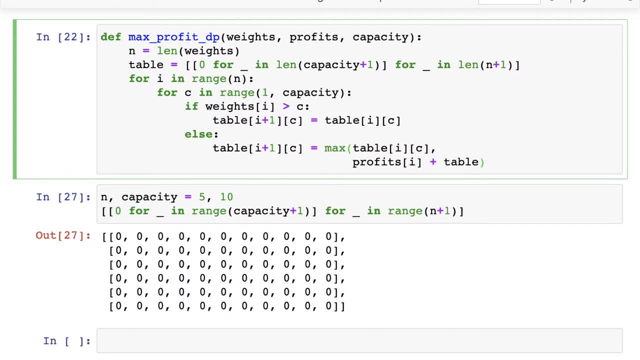 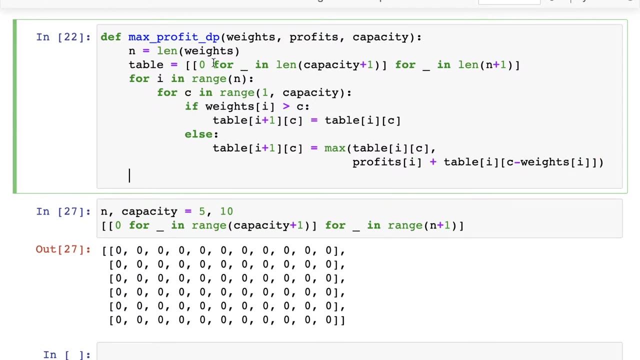 So we then have to pick table of I, but now we have to pick C minus weight, weights of I, okay, And that should fill out the entire table pretty much. That's a nice thing about dynamic programming. So we just have to write this one solution or this one recurrence and be careful about it. 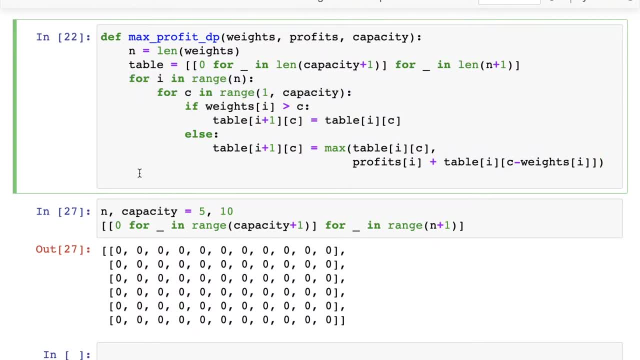 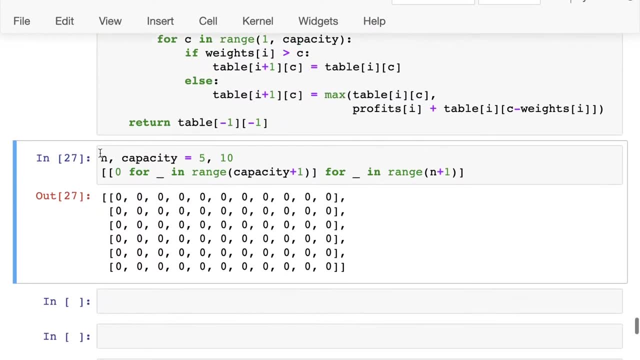 And everything else is taken care of by this loop. here And now we simply return table of minus one and minus one and let's see if that works. It's likely that there are some issues here, but let's see. we have test cases. 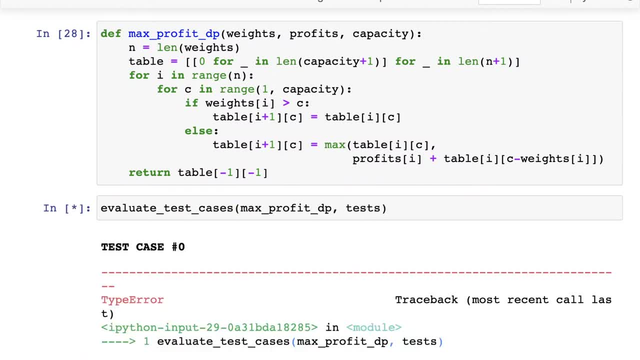 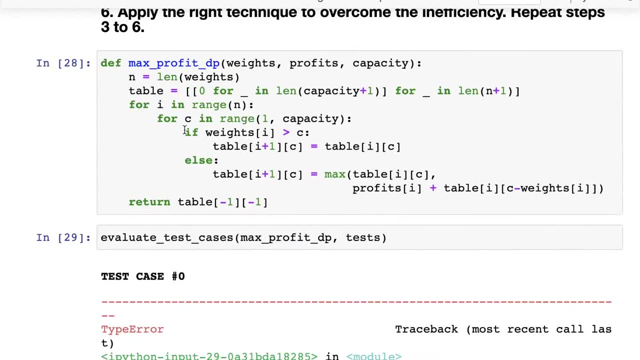 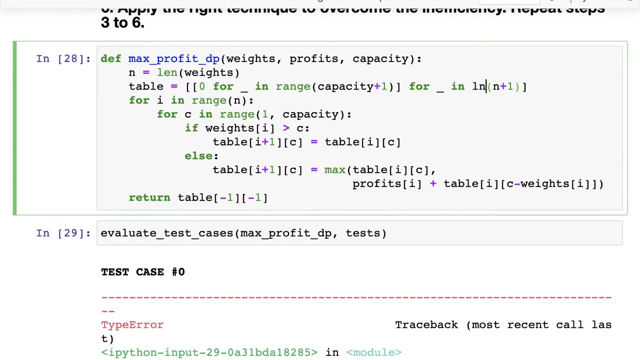 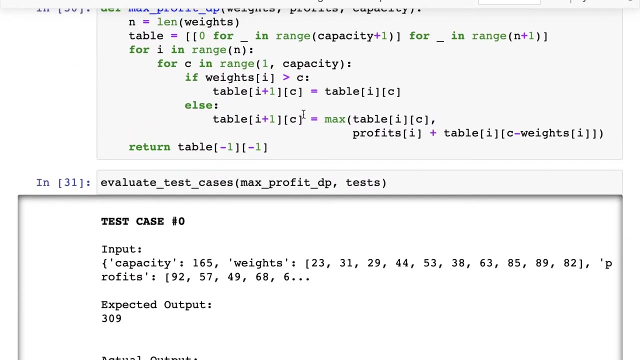 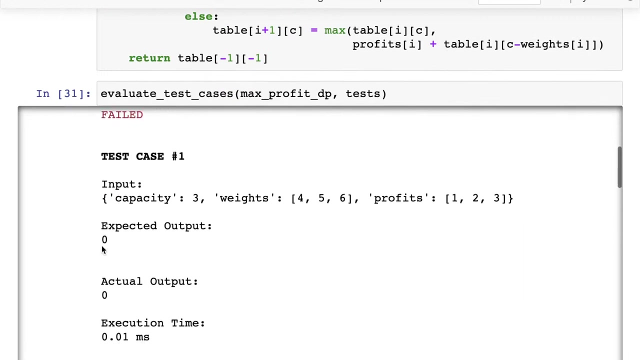 max profit, DP With the tests that we have- great. So we are seeing an issue already. I see here that this should be range and this should be range. Okay, One thing that we haven't done here is: well, it seems like. 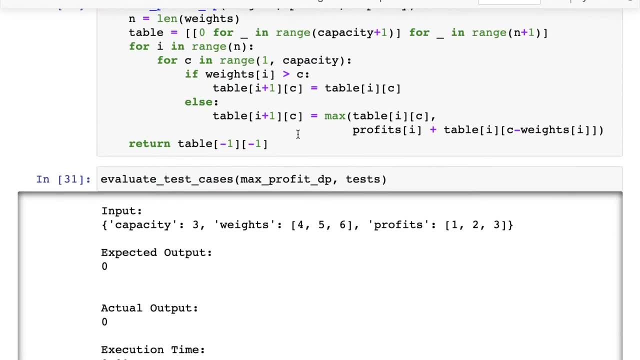 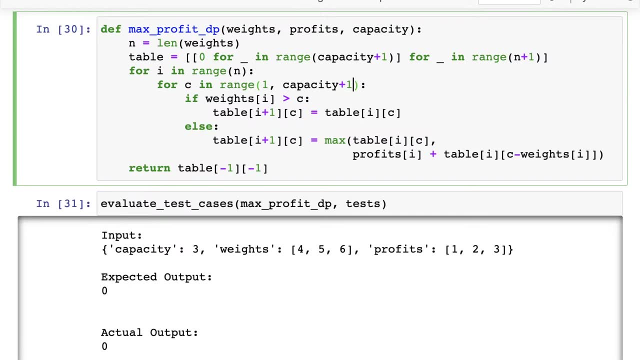 Our solution is always zero. This should be capacity plus one, So that we this takes all the values from zero to capacity, right? So see, the iterator should take the values from one, two, three, four, all the way up to the maximum capacity. 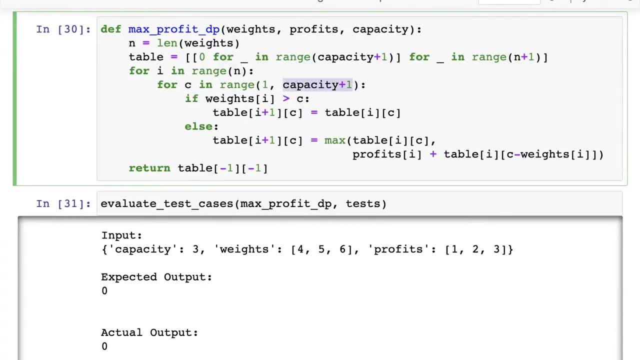 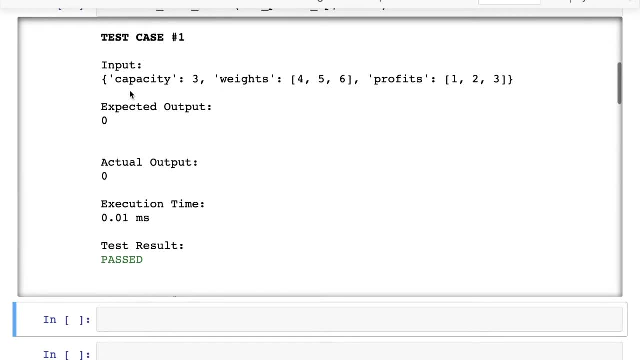 And the range does not end. Uh, so the range does not include the end value, So you need to put capacity plus one here. Okay, Now, with that out of the way, you see, once again, these off by one. errors are always. 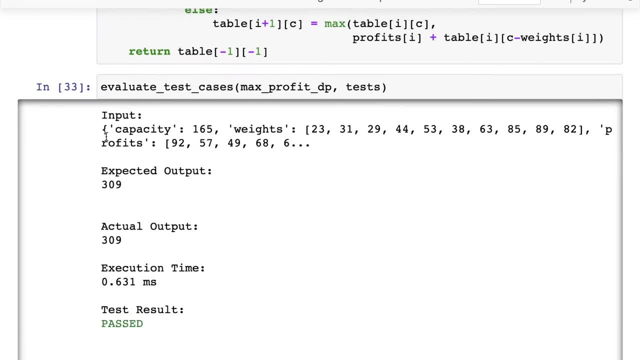 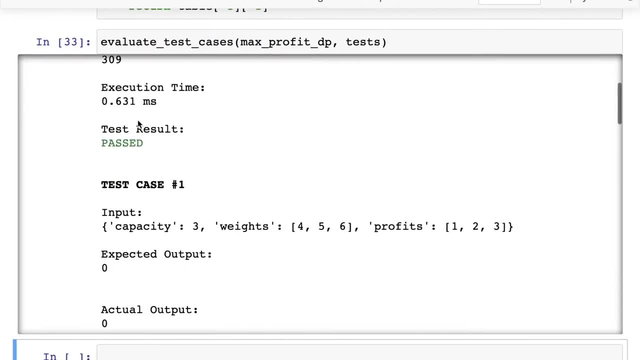 Going to bug you with dynamic programming. I've probably solved 50 or a hundred problems in dynamic programming, but I still make these errors. Um, but with that out of the way, you can see now that each of the test cases seems to pass. 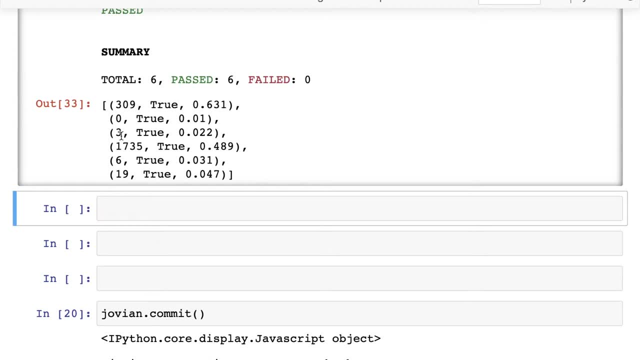 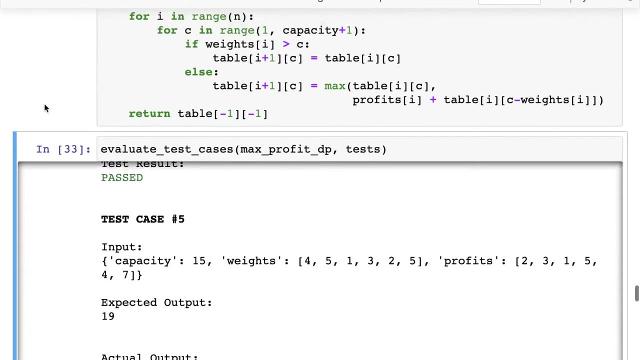 Now there may be other cases which you have not accounted for, but overall we've covered all the test cases here And we've ended up with now a dynamic programming solution, And I let you figure out the complexity here, but once again, it's pretty straightforward. 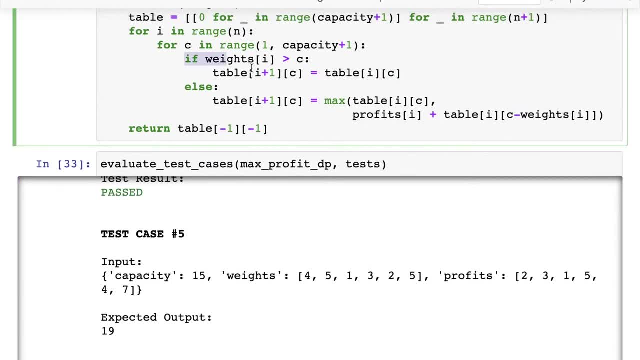 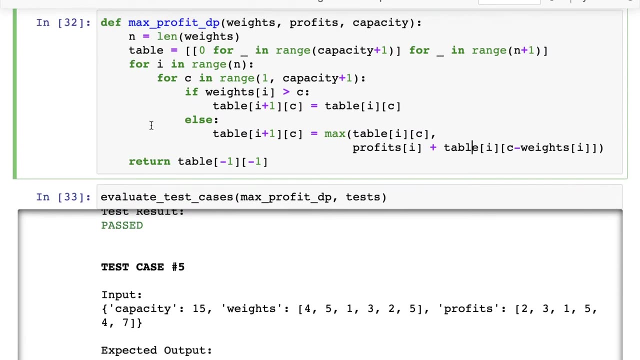 Because we are filling up this table, and filling up this table simply requires this constant amount of work, which is a comparison And then potentially another comparison and an addition and a subtraction, So like four or five operations. So you have this end times and you have this end times. get past, uh, end times. capacity, where N is the length of weights and capacity, or W is a total capacity. 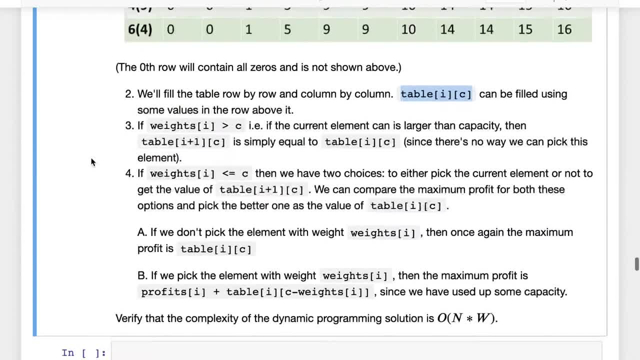 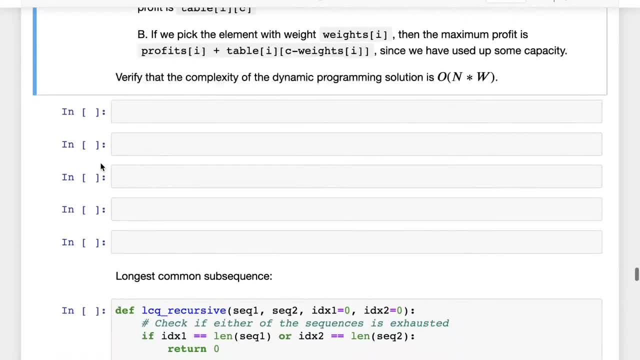 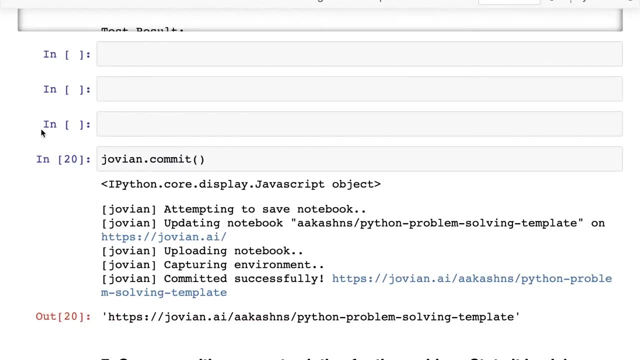 So N times W is the number of iterations And that Really also is the complexity, the time complexity of the algorithm. So that's the knapsack problem, And now what you can do is try and figure out not just what is the maximum value, but also figure out what are the actual elements that were chosen. 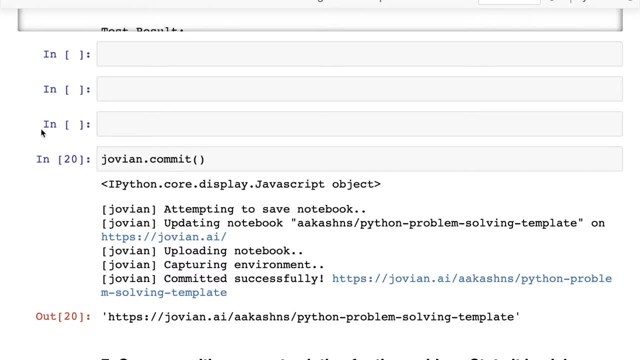 Now you can do this for the knapsack problem and you can do this for the longest subsequence problem. figure out the actual longest subsequence And it should be possible to do that with just a small modification. Now use the forum. 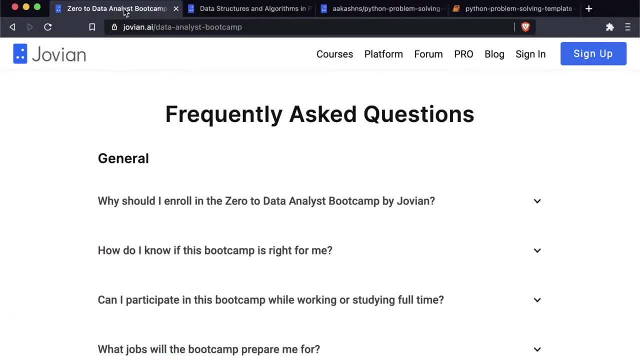 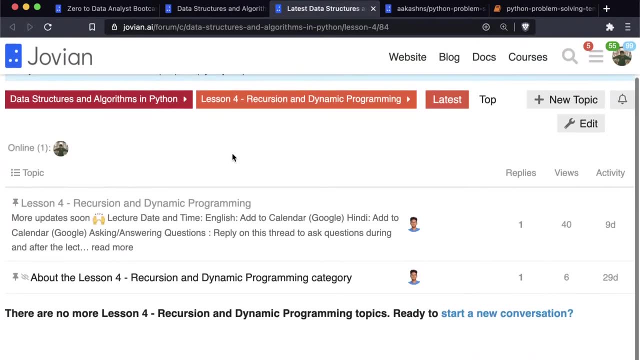 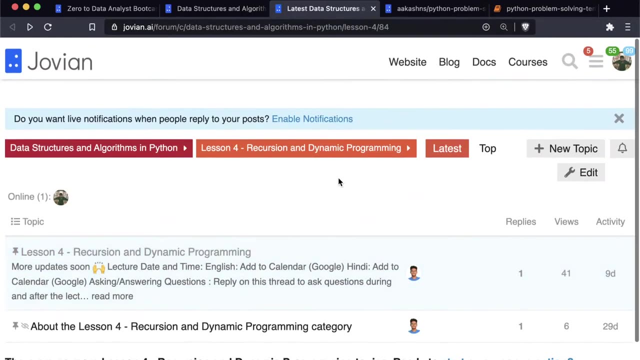 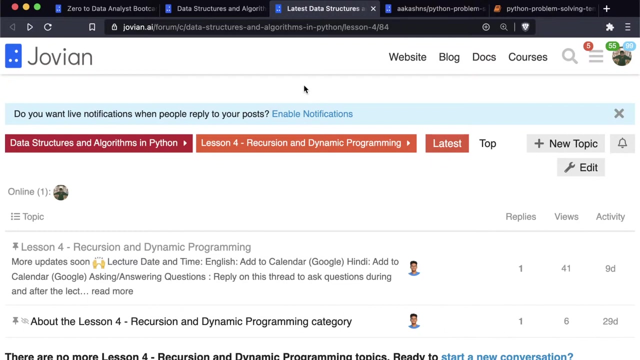 If you have any questions about the contents of this lecture, go back to the lesson page and open up the course community forum here. You can see here that, uh, this is the lesson for recursion and dynamic programming lesson. You can post your question here and you can also discuss ideas on how to figure out what the longest common subsequence is and what the best selection for the knapsack problem is. 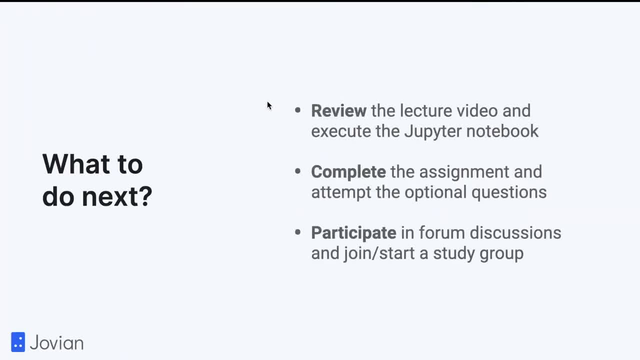 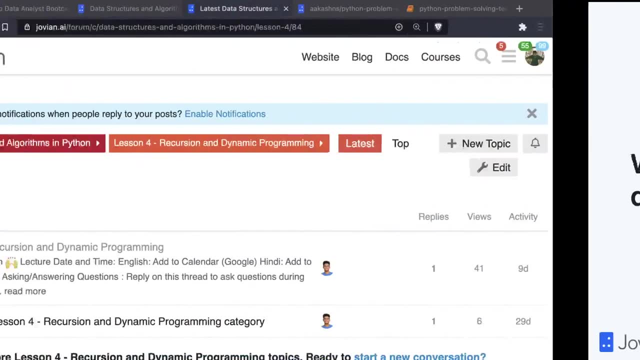 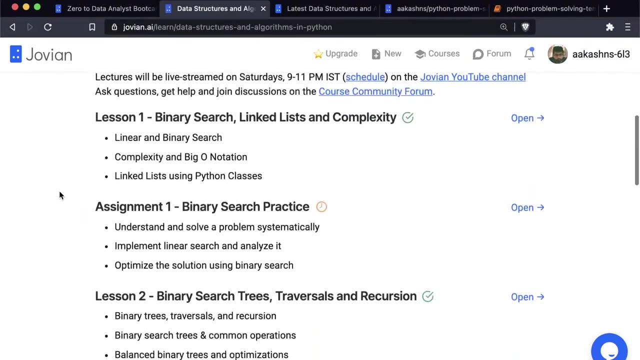 Okay, So what do you do next? Well, you can review the lecture video and execute the Jupiter notebook. The next step is also to complete the assignment. Now we have released assignments one and two so far. If you go back on the lesson page, you will find lessons, or you will find assignments one and two and you can work on them, and assignment three will be live soon. 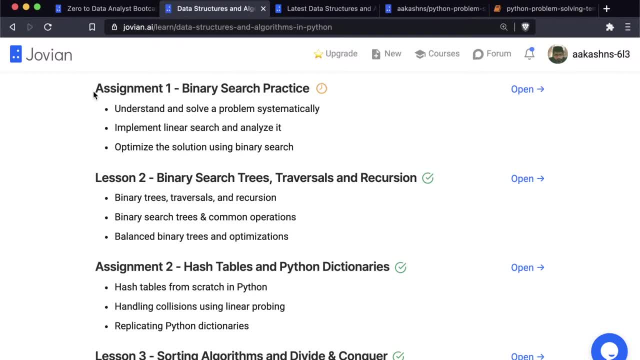 But since many of you have let us know that you are currently have exams or other commitments, we've extended some of these deadlines, So you have A lot of time. Now you have close to four weeks to submit these assignments, to do work on them. 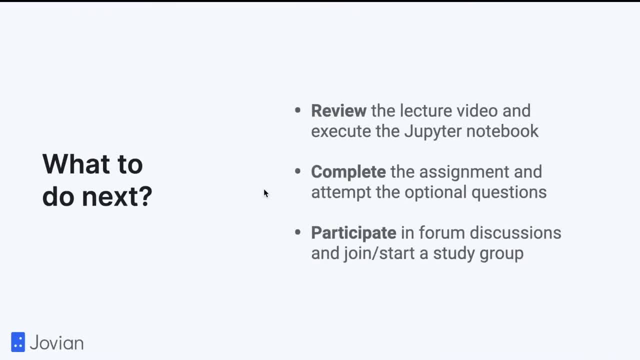 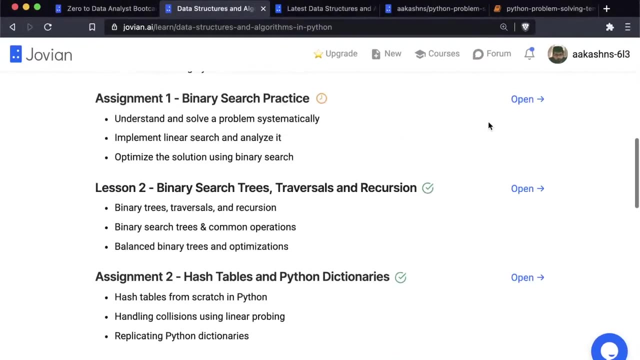 There is sufficient time and also work on optional questions and to participate in forum discussions and, if possible, join or start a study group too, And that's a great way to stay motivated. So we do have assignment walkthrough videos as well. If you open up assignment one, you can see here that this is a walkthrough. 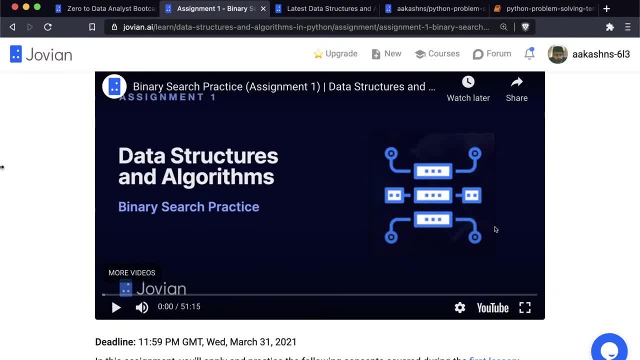 And this is a one hour walkthrough of the assignment. So if you just watch through this video and have the assignment notebook on the side, you will pretty much solve the entire assignment by the time you get to the end of this video. So it'll only take a couple of hours for you to solve the assignment. 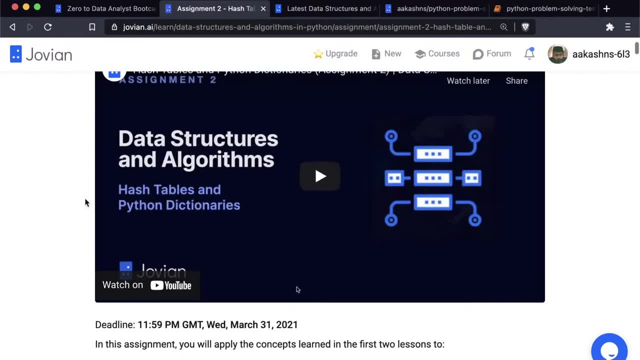 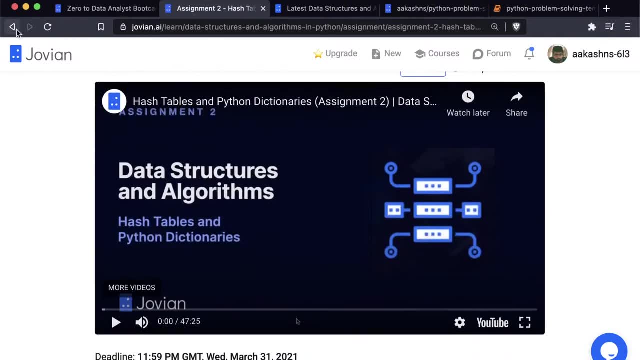 We don't show you the full solution here, but we do give you a whole bunch of hints and point you in the right direction. And similarly we have this 50, 45 minute video for assignment two as well, to make it easier for you to walk through this assignment and assignment. 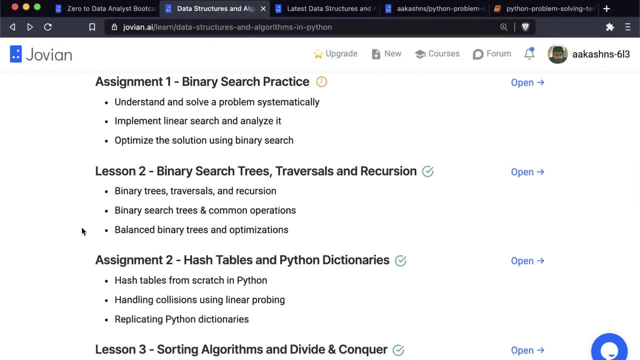 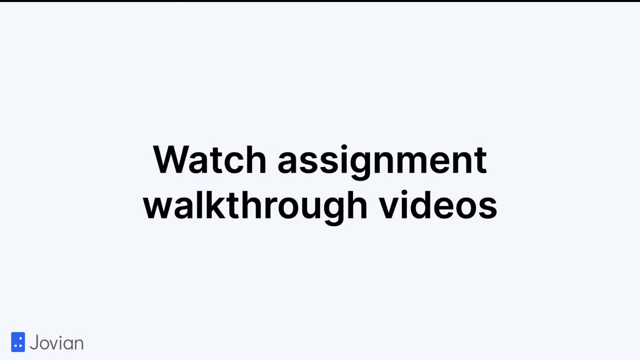 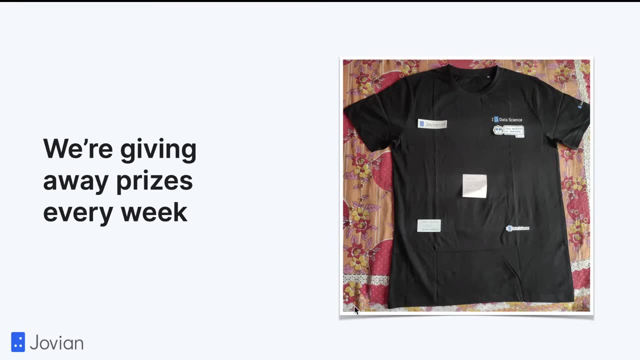 Three Live very shortly, So do watch assignment one and through walkthrough videos and complete the assignment. Thousands of people have already completed the assignment and we've extended the deadlines significantly, So you have a lot of time to work on the assignments and we are giving away some prizes every week. 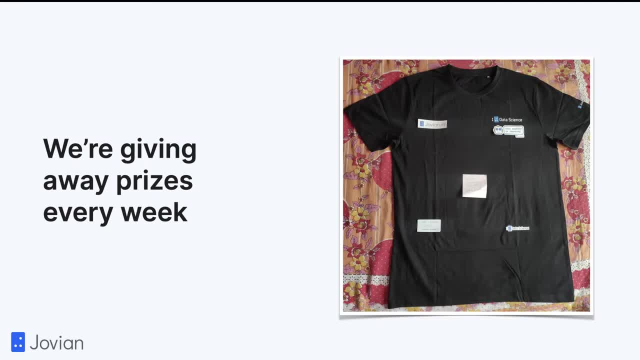 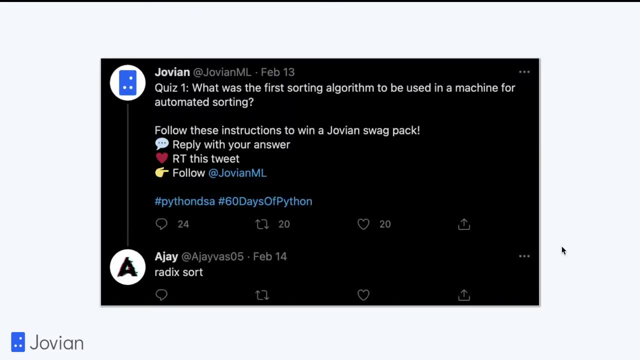 So we had five opportunities to win prizes last week, So I'm quickly going to declare the winners of last week. Now the quiz one winner. the quiz one was what? This is the first sorting algorithm to be used in a machine for automated sorting. 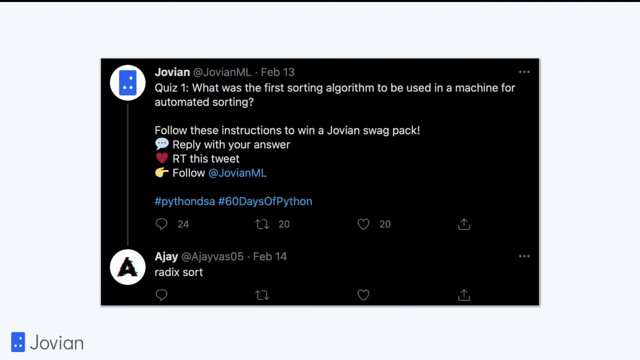 Well, this was Radek sort, and this was used way before we even had digital computers. This was back in the 18, late 1800s, I believe, And this was used to sort punch cards, if I'm not wrong. 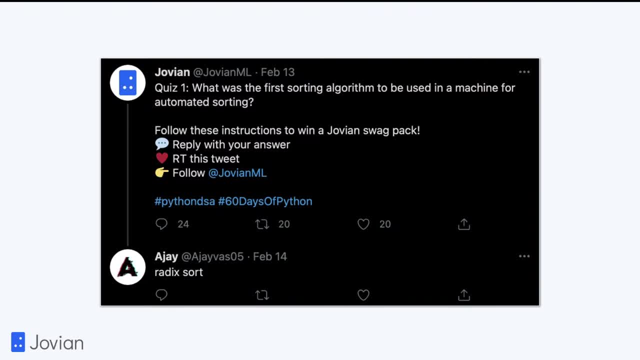 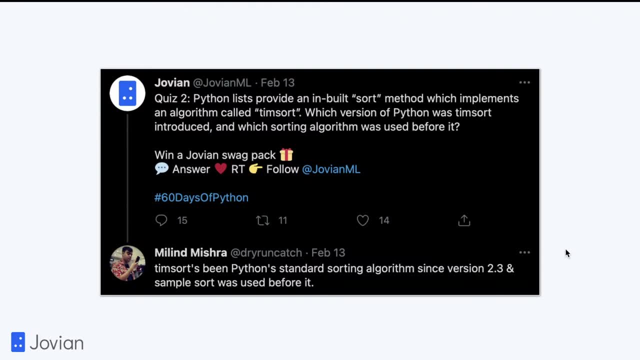 So Ajay is the winner. So congrats, Ajay. you will receive a swag pack from us: a t-shirt and some stickers. The second quiz was Python Bill A list. Provide an inbuilt Method which implements an algorithm called Tim sort. 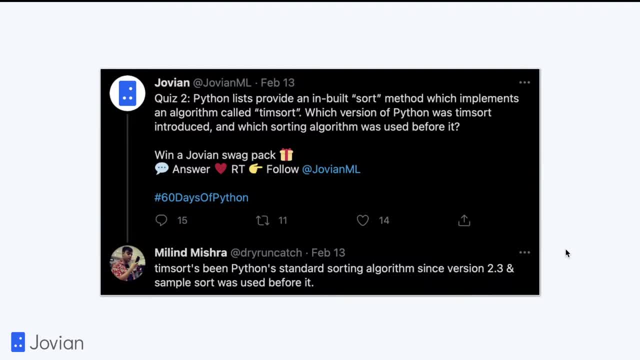 Now which version of Python was Tim sort introduced in and which sorting algorithm was used before it? And the solution is: the Tim sort was you introduced in version 2.3 and sample sort was the algorithm that was used before it. So million Mishra is the winner. 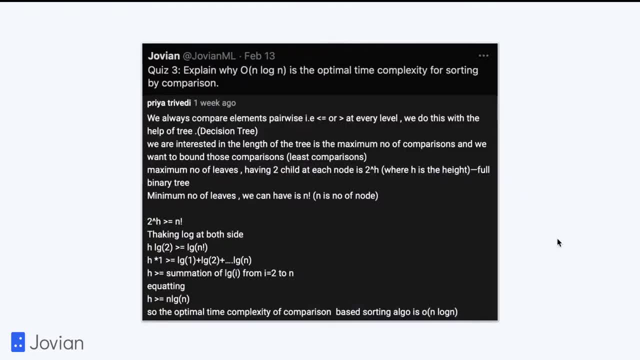 Congrats, Milan. You will receive a swag pack from us, And here's the winner of quiz three. The question was: Explain why order and login is the optimal time. complexity for sorting by comparison. Now, we can always come, We always compare elements. 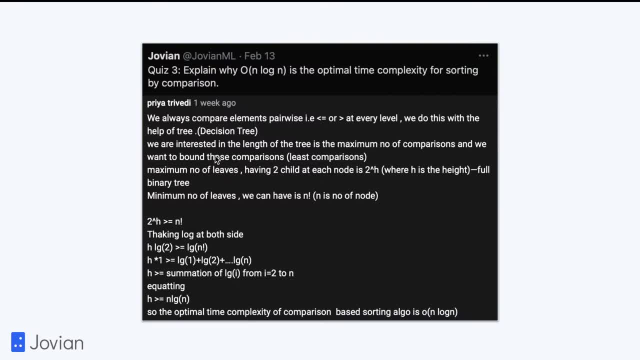 Priya, Priya says Priya is the winner. congrats, Priya. And the solution is that we always compare elements pair wise, and we do this with the help of a decision tree. Now we're interested in the length of the tree and the maximum number. 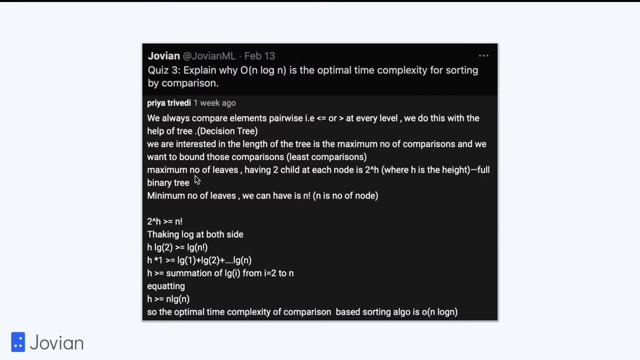 of comparisons that we need to make. So What Priya concludes Is that because we have two children at each node, so the height of the trees edge, then at the leaves, the leaf node, we have two to the power edge leaves. 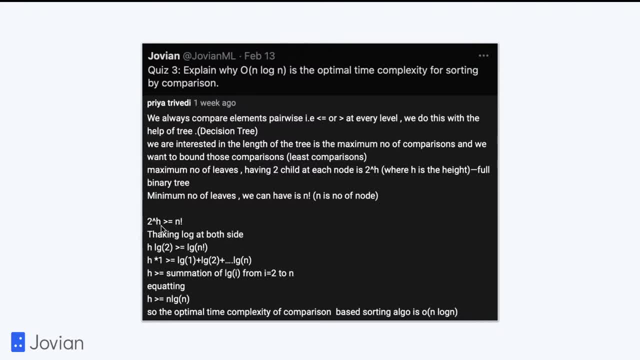 And because we have two to the bar edge leaves, So two to the bar edge will be greater than the total number of possible arrangements of an element. So two to the bar edge will be greater than N factorial. And what that means on Some, on simplification, is that edge will be greater than N log N. 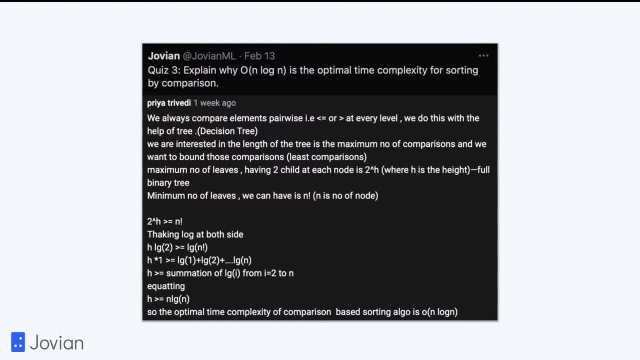 So the height of the tree that you, the decision tree that you create by doing a pair wise comparison at each level, is greater than N log N. So any sorting algorithm, We'll take At least N log N for some particular input, right. 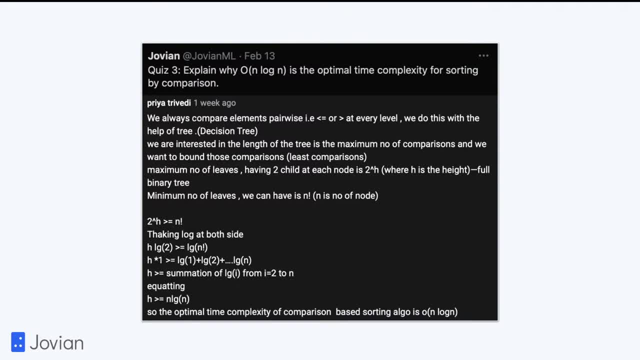 To go from the current set, the current organization, to the sorted organization will take- at least I will take and log in steps, not for all cases, but there will at least be one case among all the possible permutations which will take and log in steps. 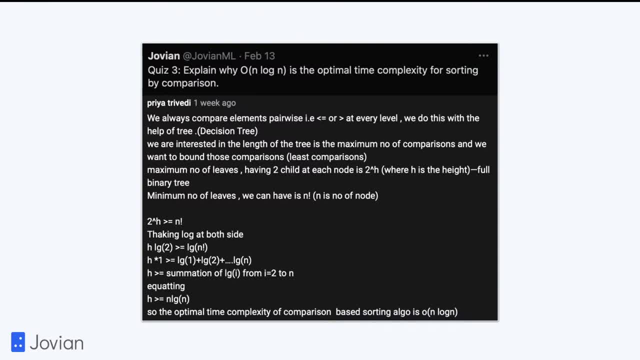 And in fact there will be far more than one case. Most, most of the cases, will take and log in steps. Okay, And that is why the optimal complexity of the sorting algorithm is in login. That's a great explanation, Priya. 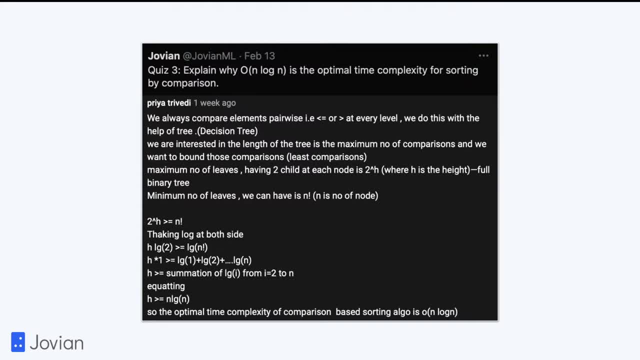 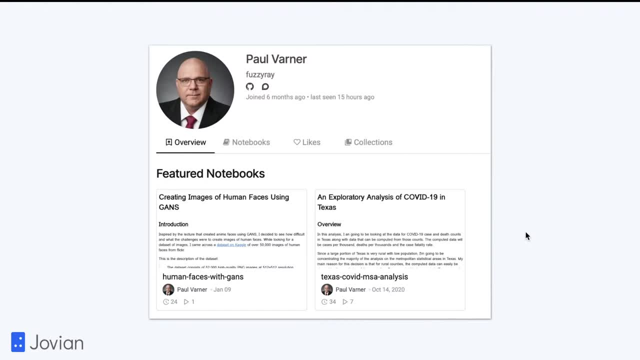 Thanks and congrats on winning the swag pack. And then the forum contributor of the week is Paul Warner, or Fuzzy Ray on the forum. Thanks, Paul, for all the questions you've been answering and for all your contributions on the forum, and you win a swag pack from us too. you will hear from us soon. 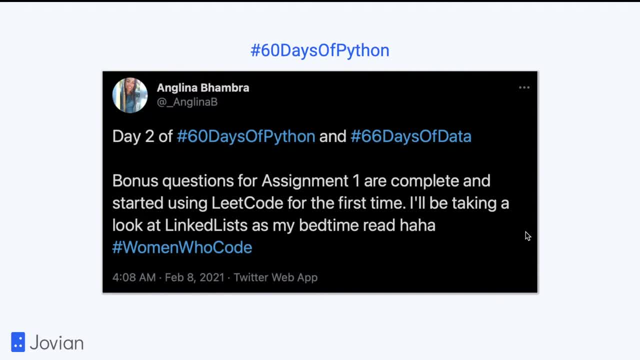 And finally, the winner of the 60 days of Python hashtag is Anglina, And Anglina has been sharing her update every single day on Twitter, almost So you can check out her Twitter profile underscore Anglina B. So there's a lot of it's a. it's a great way to hold yourself accountable and stay. 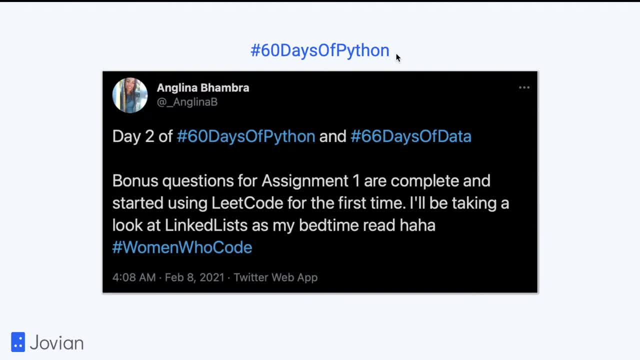 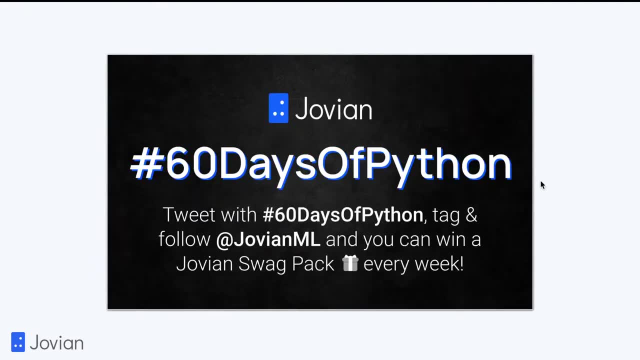 motivated throughout the course. So there's something that you should try out as well: Do tweet out what you're doing with 60 days of Python and also write a blog post, if possible. So for this week we have we're giving away one price for an interesting 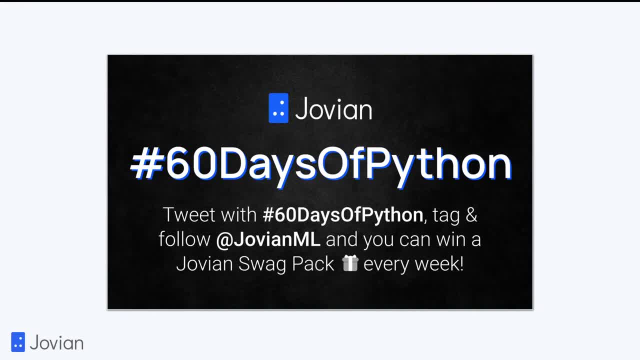 Notebook that you share with 60 days of Python, And I have a couple of suggestions: create a notebook to modify the dynamic programming solutions that we've created for the long, longest subsequence or the knapsack problem, to not just find the maximum number but actually find the longest subsequence or actually find the selected elements in the knapsack. 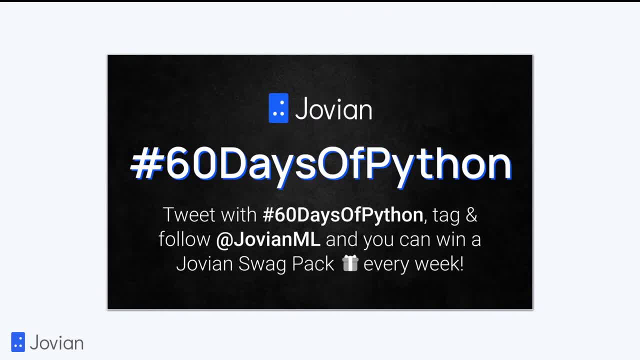 problem. Now, if you create a notebook like that and Tweet it out with Hashtag 60 days of Python and also make sure to make sure to tag us and follow us on Twitter, Then we pick a winner and you can win a swag pack from us. 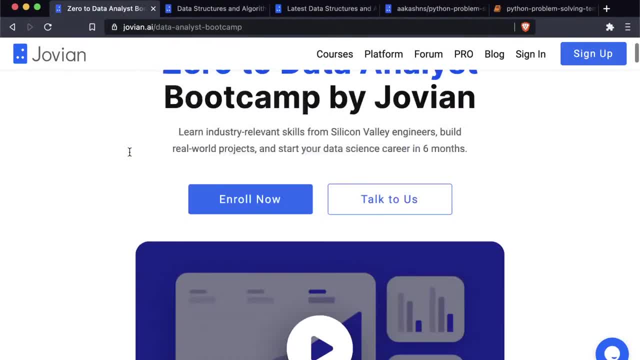 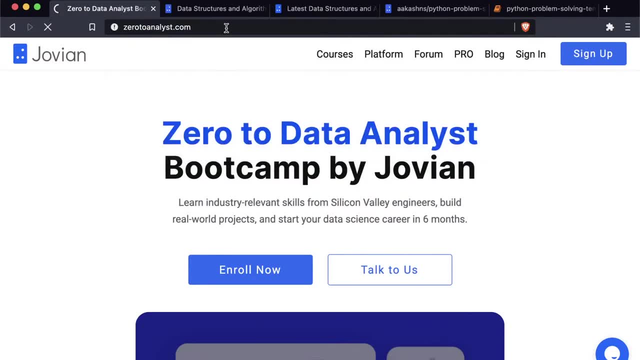 So with that, I'll see you in the forums, And, once again, I just wanted to tell you about the zero to data analyst bootcamp. This is something that we're starting on the 15th of March. You can find it on zero to analystcom. 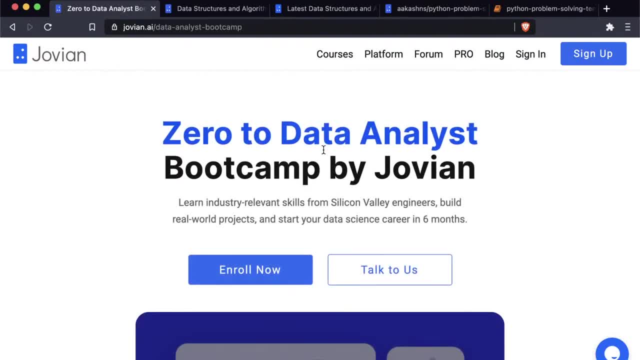 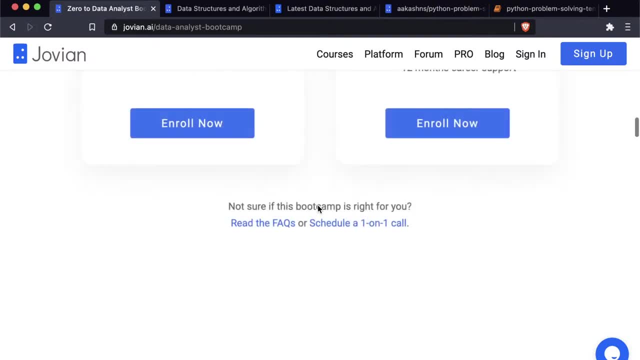 This is 16, we got a 20 week bootcamp where you can learn industry relevant skills And by the end you will be job ready to get hired as a data analyst. You can see all the benefits here. Now, this is a limited program. 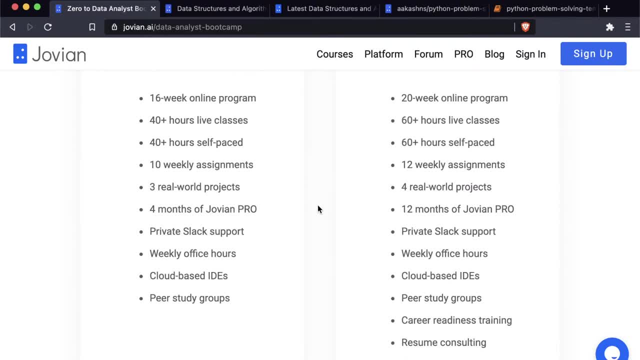 We are only accepting a batch of hundred students starting next month and you will have several hours of live classes on weekends. You'll also have a lot of self-paced content. You will solve 12 weekly assignments, You will build for real world projects and you will also get access to a 12 full months of Joe. 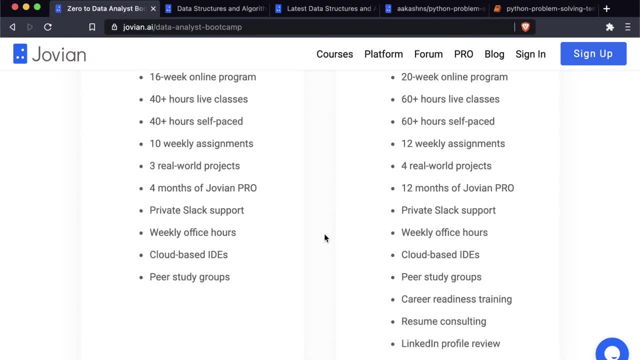 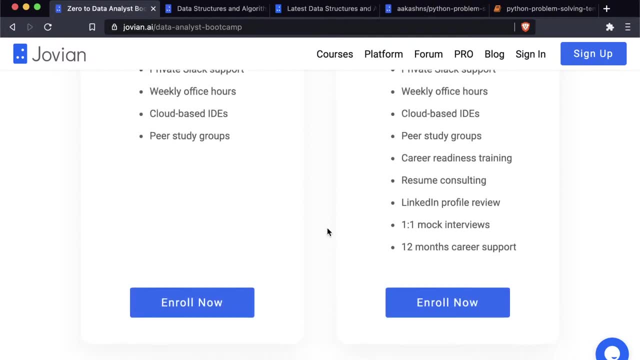 Yeah, And you will have private slack support, a weekly office hours, cloud-based programming environments, a peer study groups, a career readiness training module, resume consulting, LinkedIn profile review, a one on mock interviews and 12 months of career support. 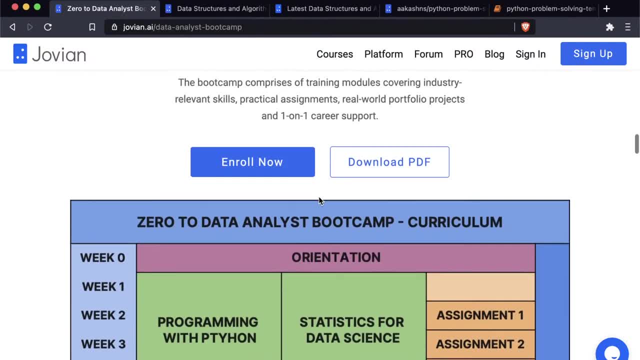 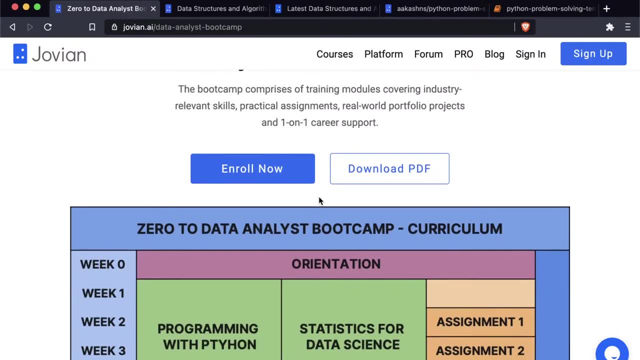 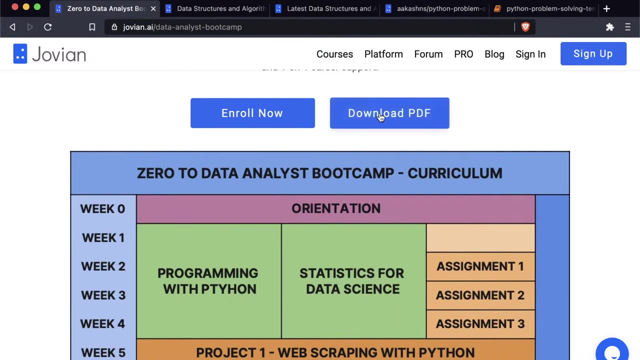 So to keep it in mind and it says: and this is the curriculum, this is focused towards data science and machine learning, So this will prepare you for jobs like data analyst, machine learning engineer and even data scientist, Although that may require a little more work. you can see a curriculum here or you can also. 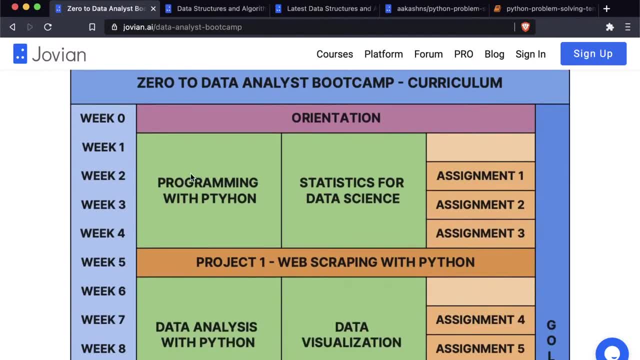 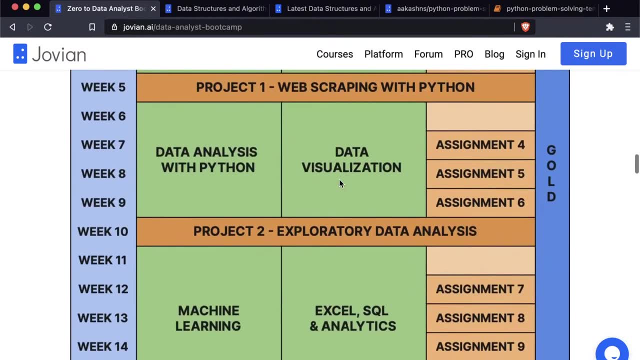 download a detailed PDF with a full list of topics that we are covering: programming with Python, statistics for data science, and you will build a project and work on some assignments. And then you have data analysis with Python, a data visualization assignments- four, five, six. 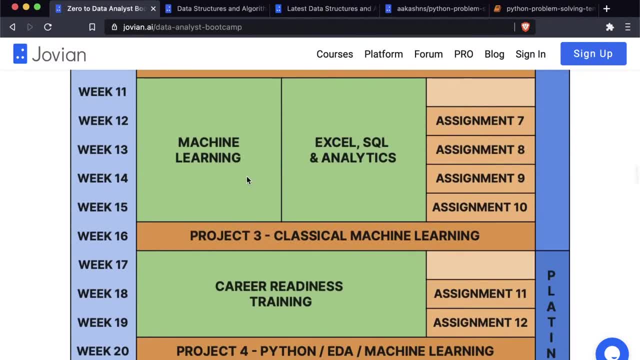 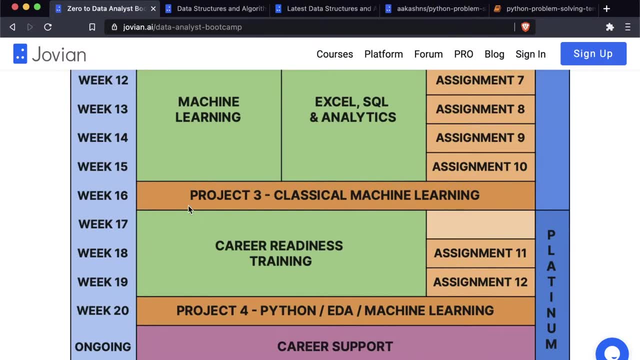 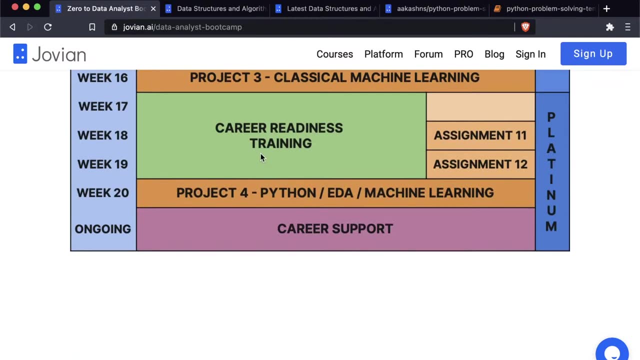 and you have a second project on exploratory data analysis. Then you we will cover machine learning, Excel, SQL and analytics and another four assignments over four weeks And you'll have a project on classical machine learning. And finally, we'll focus on career readiness training, where we'll work with you to create a rock solid resume and 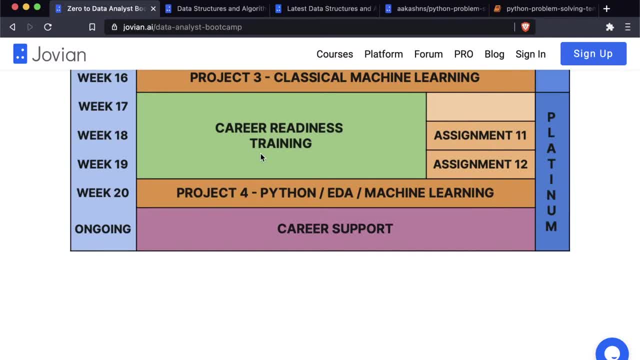 LinkedIn profile, help with the interview preparation, conduct mock interviews and help you find jobs. And it will also include a final fourth project that you will include or that you can put up on your portfolio. And once the bootcamp ends, the association doesn't end there.